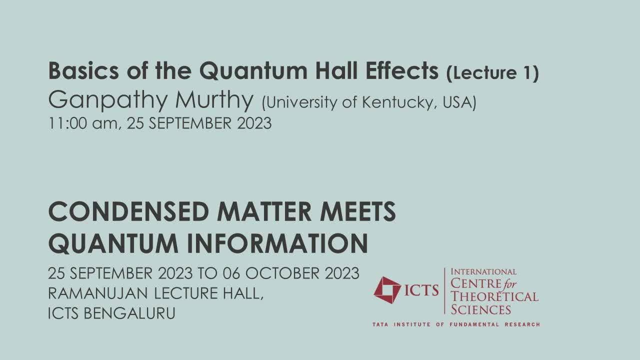 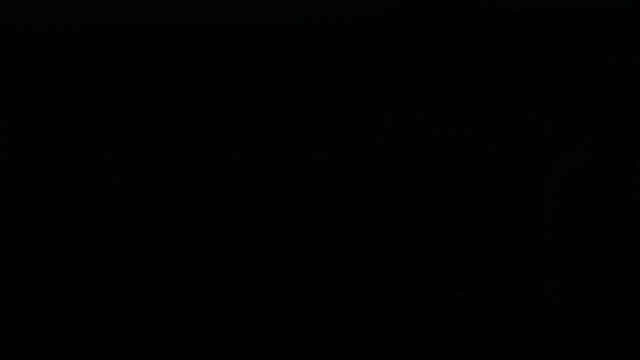 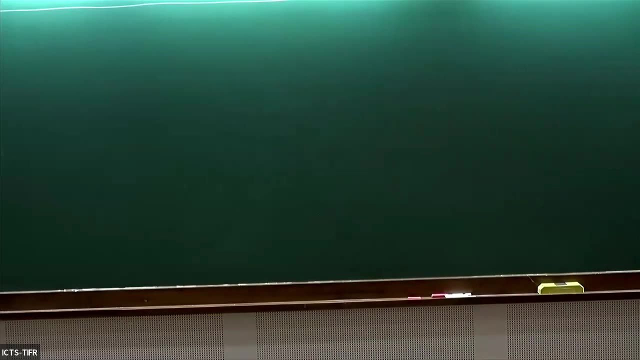 So I hope you guys will all ask questions during the talk. Okay, I'm going to try to make it as pedagogical as I can, And I have to warn you that sometimes, if I don't get enough questions from the audience, I start picking out particular people and asking them questions, You know. for example, 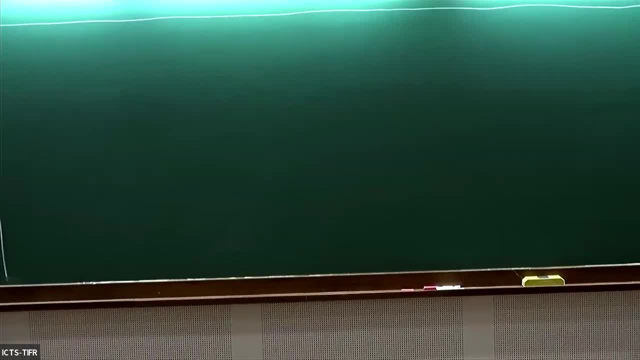 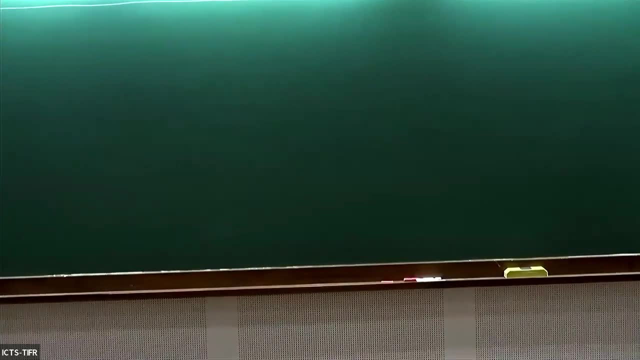 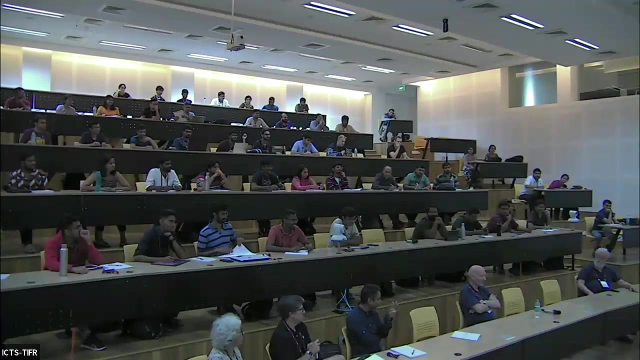 I might say the person in the purple shirt. you know and you'll have to answer. I'm not going to ask Sam, So okay. So please ask lots of questions, All right, Dissent on what, Of course, they can. 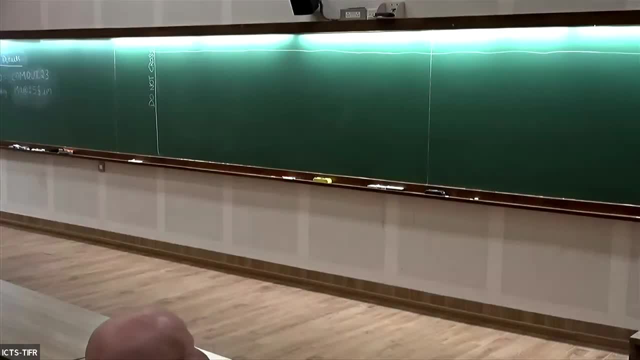 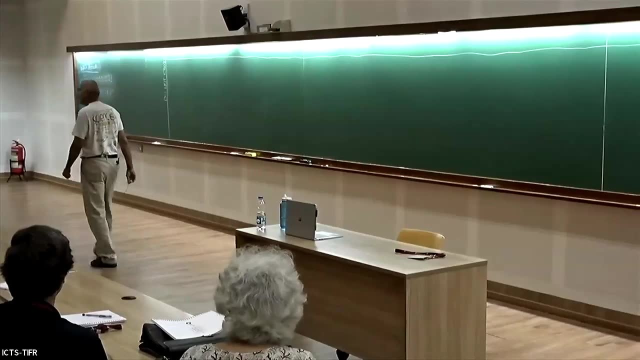 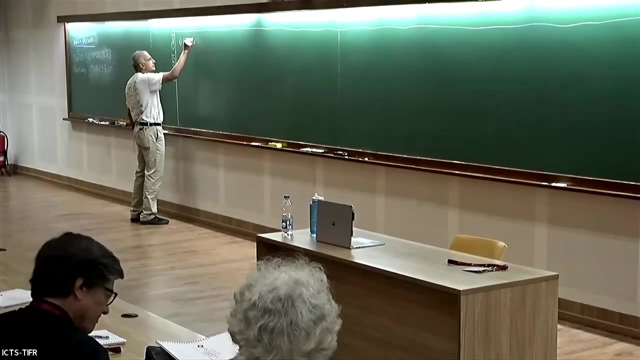 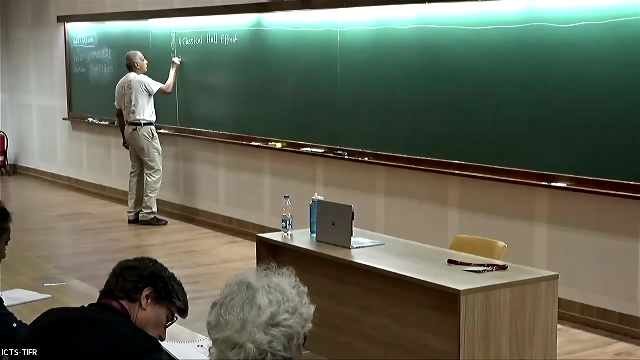 not answer. They can choose not to answer. You have the right to remain silent, So okay, So here's the plan of my talk. So what I'm going to talk about is first the classical Hall effect, And then I'm going to talk about the phenomenology. 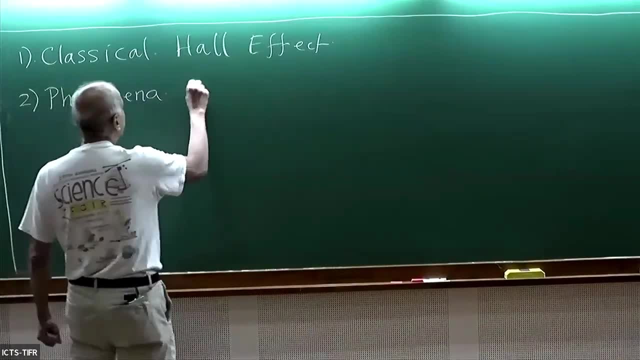 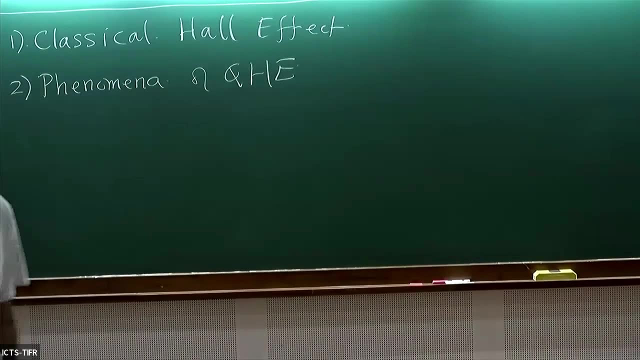 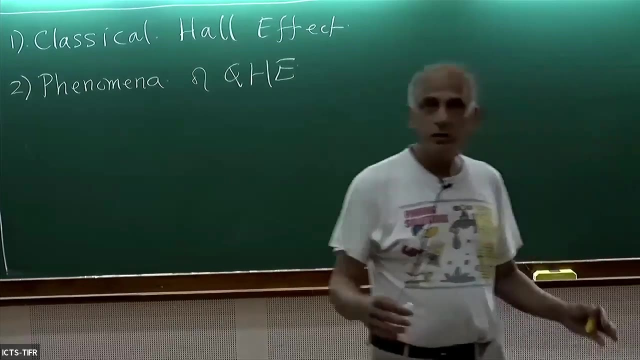 of the quantum Hall effect. Now please tell me if I'm writing big enough that it can be seen from the back And if I'm speaking loud enough. usually the loudness is not a problem, Actually it's a problem, But it's a problem the other way, But anyway. so if you cannot hear me, then please tell me. 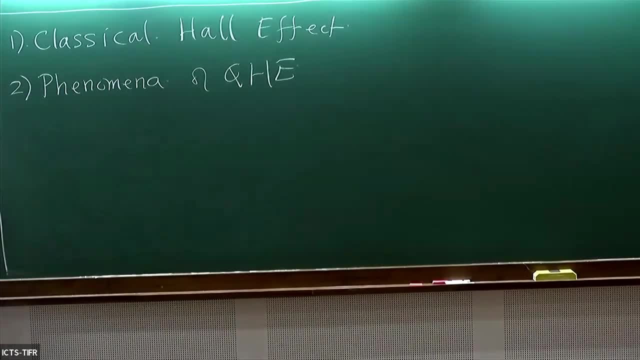 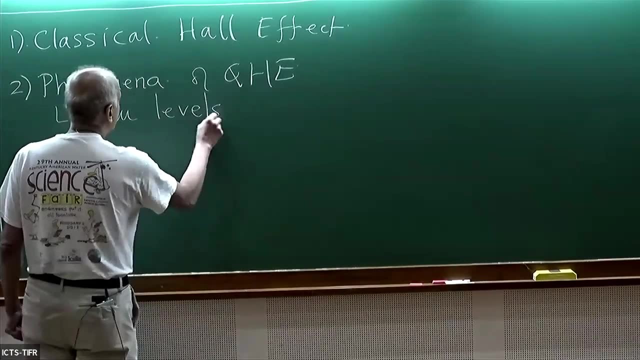 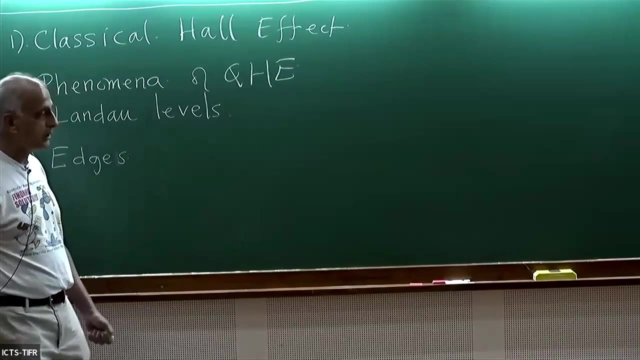 Okay, So I'll tell you what the phenomena are, what is surprising about these phenomena, And then we will talk about Landau levels, And then we'll talk a little bit about edges. These are very important, especially for this particular conference, because a lot of the platforms that are based on quantum Hall systems. 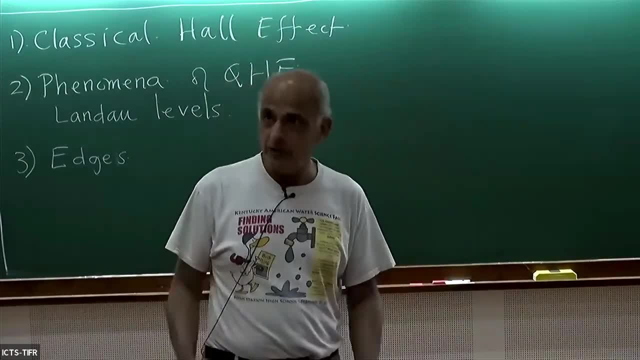 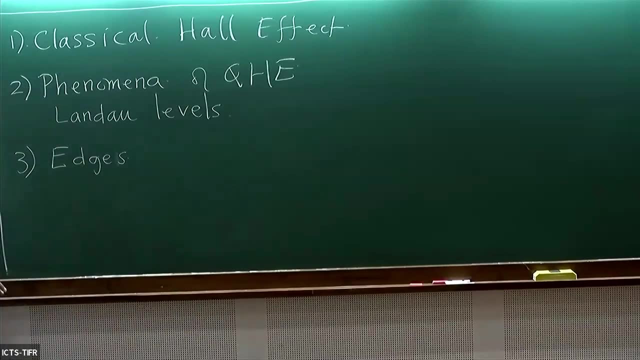 for quantum information processing are based on edge modes of quantum Hall systems, And so we'll talk a little bit about edges, And this entire lecture will be about the integer quantum Hall effect. The next lecture will be our diffraction of quantum Hall effect from two. 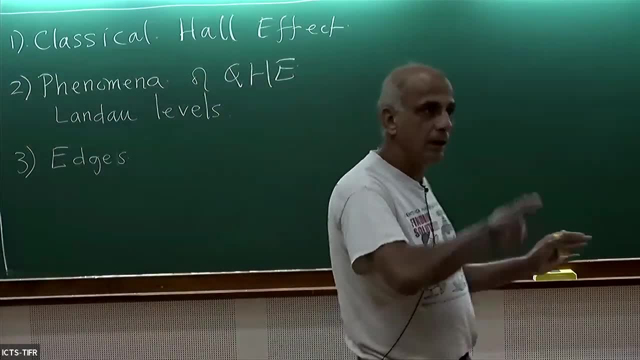 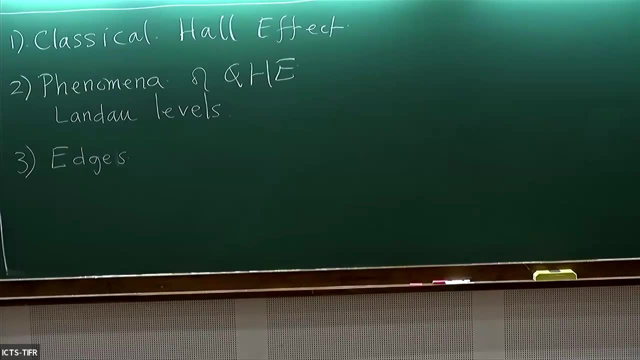 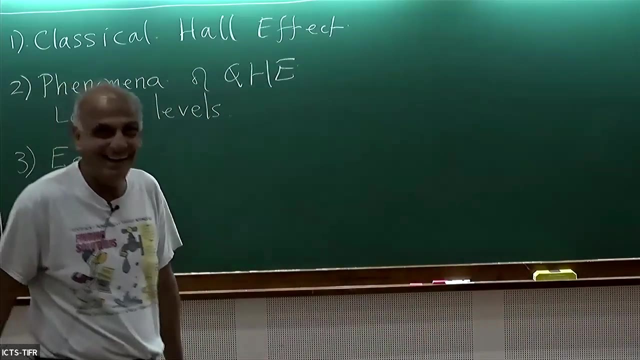 different perspectives: wave function perspective in the first half, and then the Chern-Simons perspective, of whom the originator is sitting right here. So if you have any questions, don't ask me. ask Eduardo and the third one, and then the third lecture will be about actual son-simons theory itself. 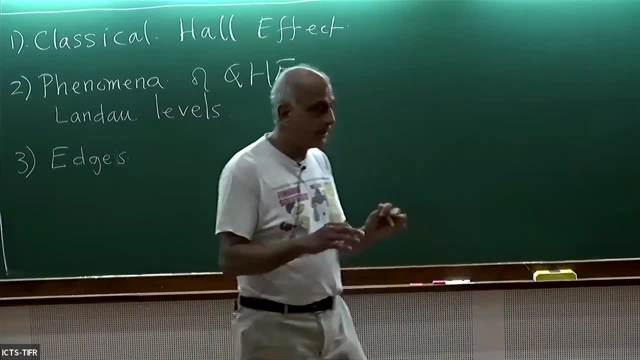 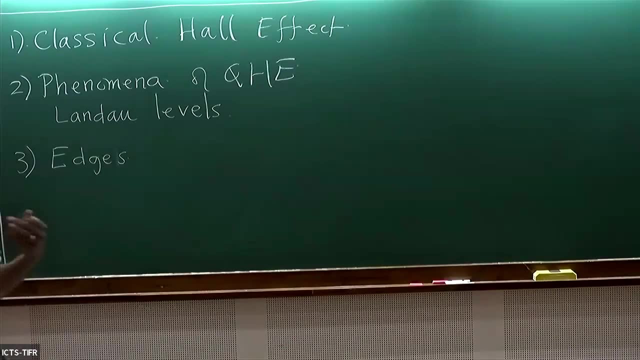 without involving any fermions, effective theory of abelian quantum hall states. and then eduardo will continue with non-abelian quantum hall states, which are actually more interesting and more useful for quantum computation. so and then, finally, no discussion of the quantum hall effect is complete without talking about disorder. so i'm going to tell you this is the only time i'll. 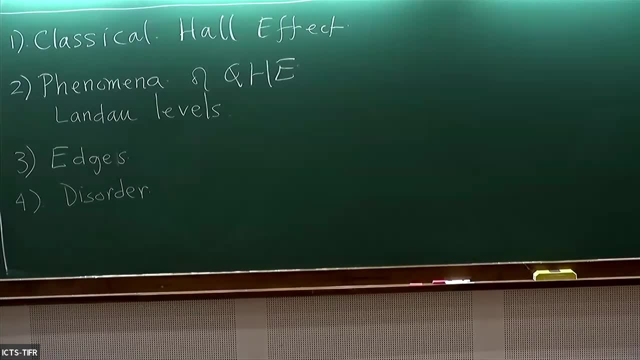 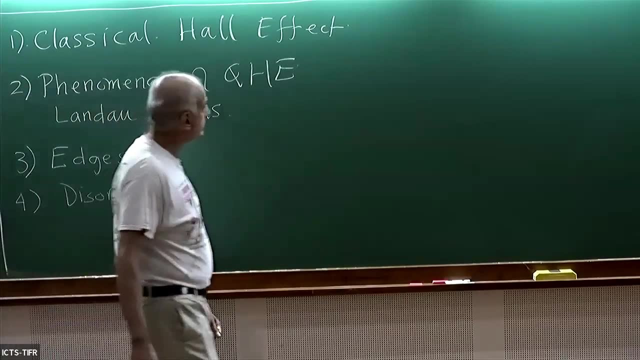 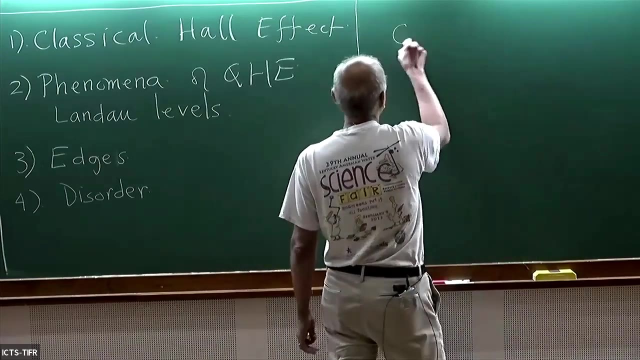 really be talking about disorder, and this is only the like the end of the first lecture. but you have to know that disorder is extremely important. without disorder, there is no quantized hall effect. okay, we'll talk about that, all right, so let's begin so. the classical hall effect: 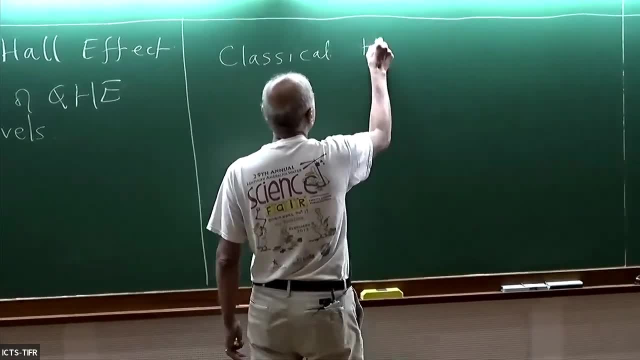 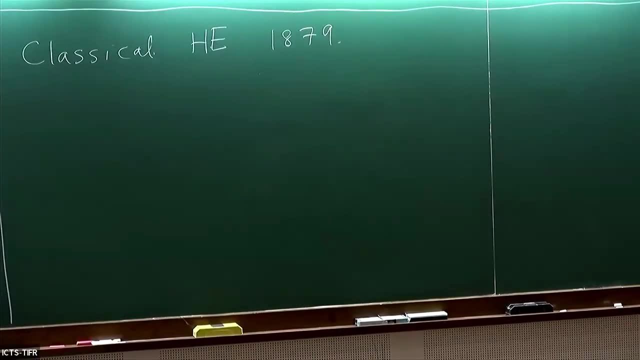 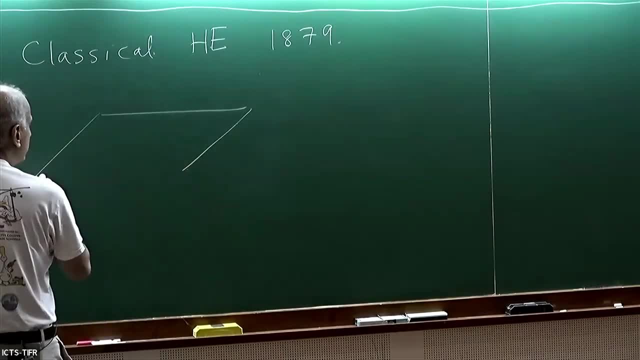 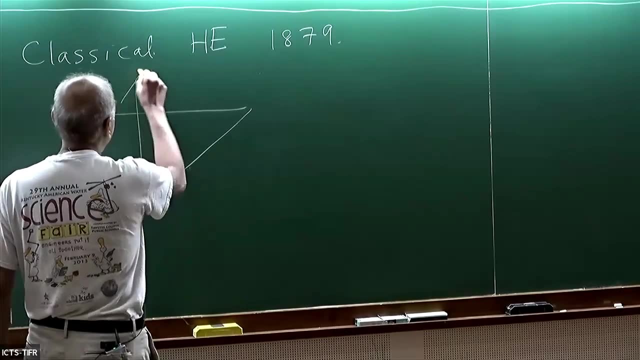 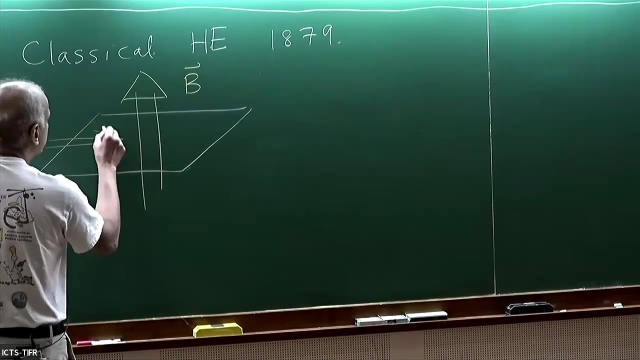 And very simple experiment. you just take a two-dimensional metallic sheet, you put some perpendicular magnetic field through it- let's call it B, right- and then you drive a current in that direction. and then you ask yourself if I measure the voltages of different? 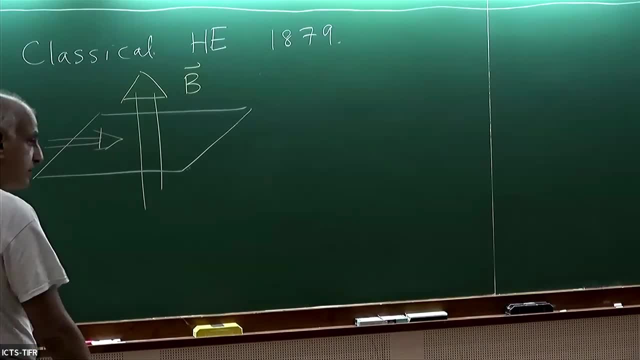 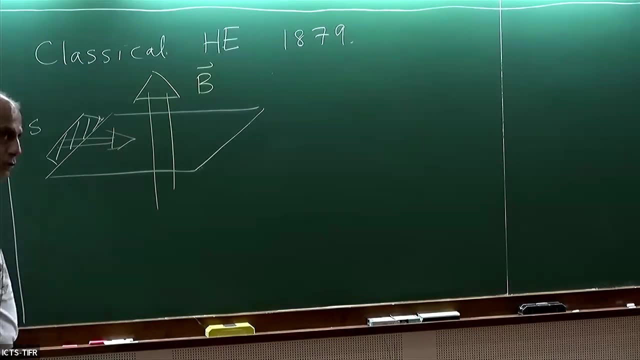 kinds. what do I measure? Okay, so there are two kinds of voltages I can use. So typically what happens is that you have some contact here. this contact is called the source S. there's another contact here that's called the drain, and then there's 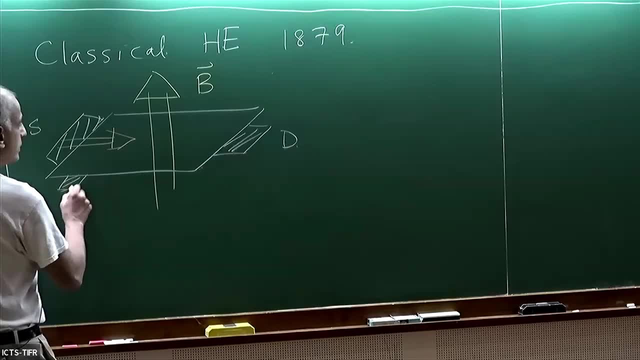 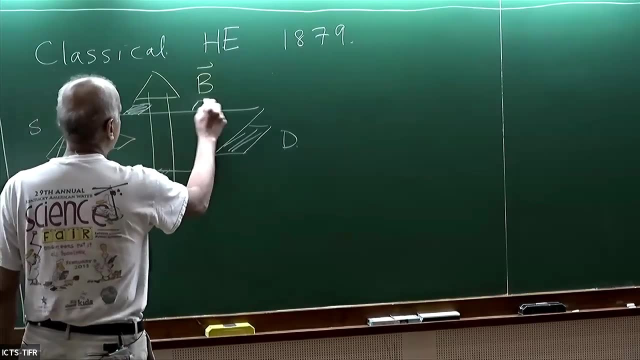 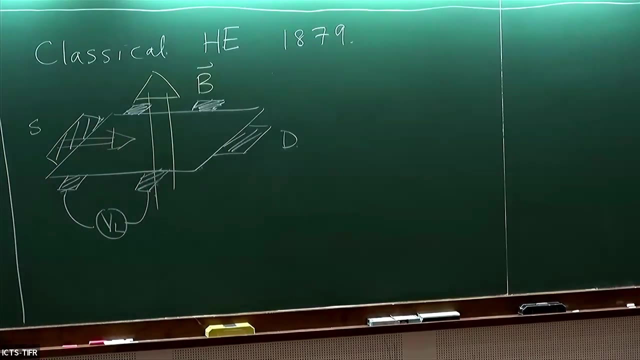 a bunch of other contacts that you will use to actually measure voltages. okay, So these are two contacts along this edge. there are two other contacts along that edge, and this voltage here is known as the longitudinal voltage. This is what would measure the normal resistance, the usual kind of resistance that you measure. 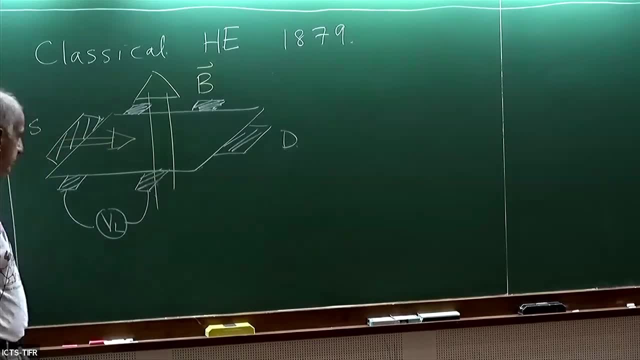 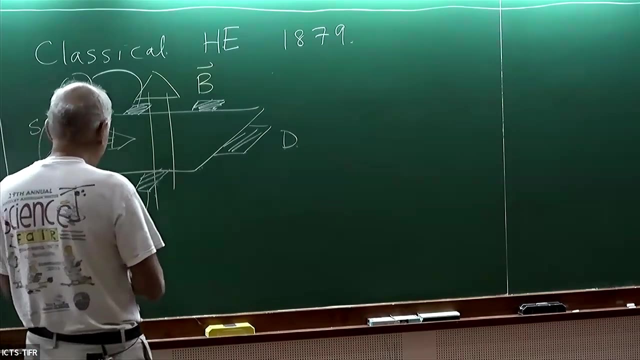 in a wire in your lab would be measured by this longitudinal resistance. And then there's something else, which you can call the transverse resistance, or, in this particular field, it's called the Hall resistance or the Hall voltage, And the Hall voltage divided by the current that you put in here, this is the current. 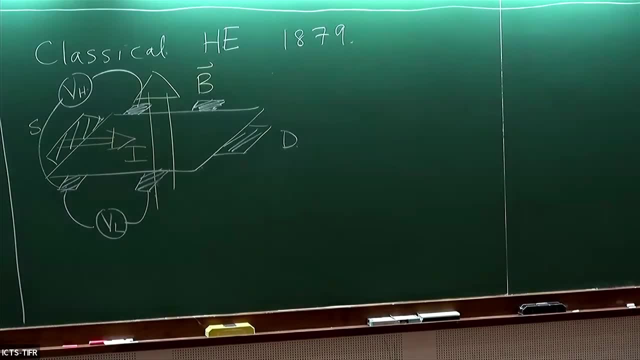 is known as the Hall resistance, And that is what we will be talking about, and that is what. that is one of the quantities whose behavior is very surprising in the quantum holotype. Okay, so how does this go? classically, Let's ask. 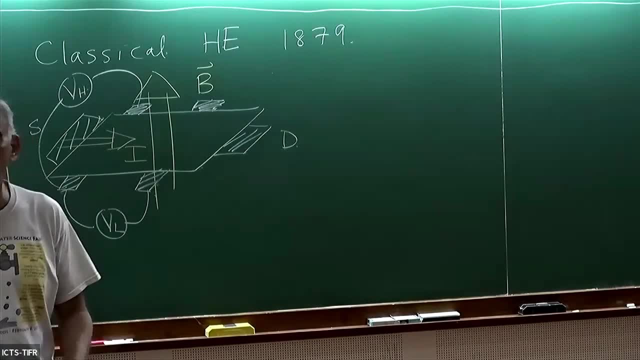 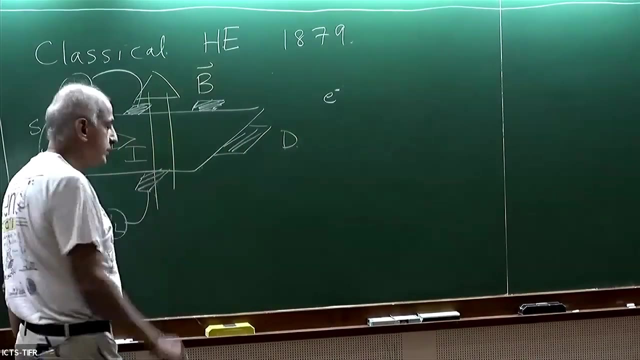 It depends a little bit upon whether the charge carriers are electrons or holes. You probably all know that in solid-state physics you can have either the charge carriers being electrons or the carriers being holes. so let's think about the carriers first being electrons. So let's say these are electrons, okay. and then the electrons you turn on the current. 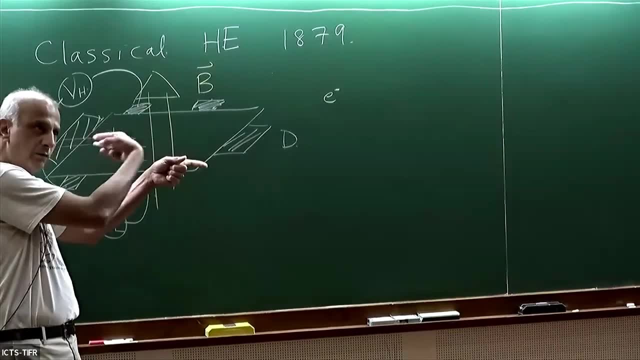 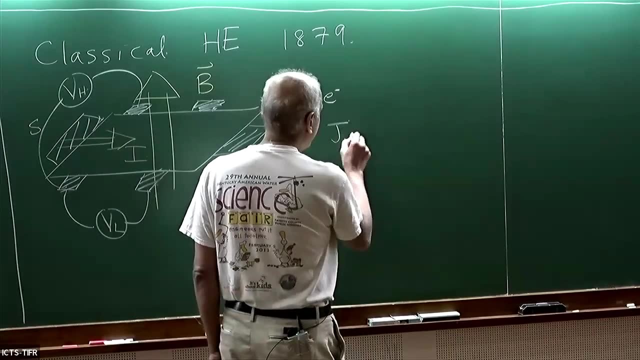 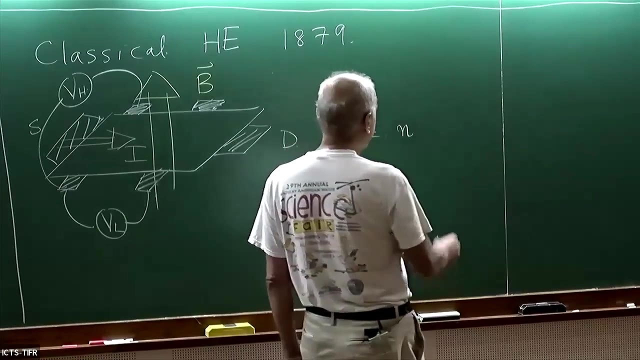 the electrons. the current is this way, so the electrons are obviously moving that way, right? So you know that the current density, this is going to be the x component of the current density, right, It's going to be equal to the number. density of charges. 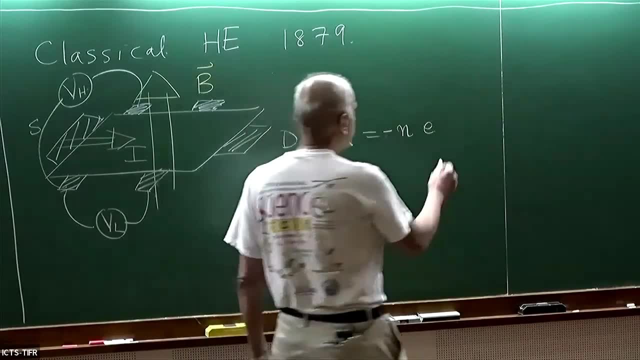 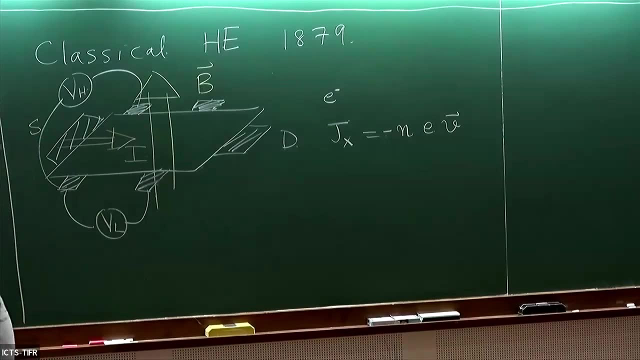 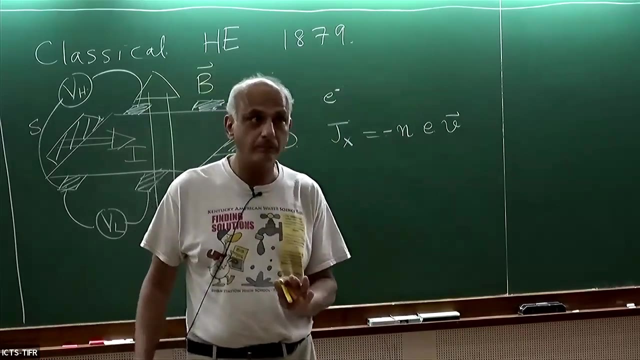 Okay. Times the charge. times the drift velocity: all right, this is like the standard formula for the current density. All I want to remind you of here is that we are working in two dimensions, so this is a number per unit area, okay. 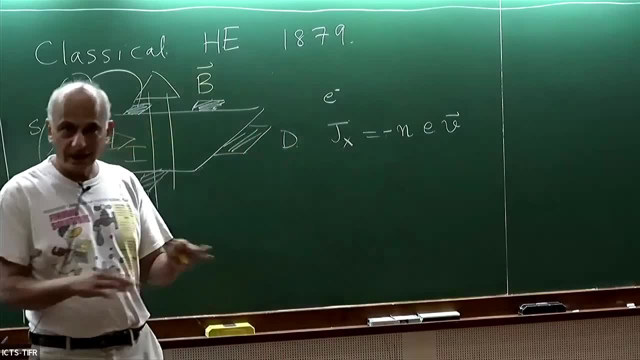 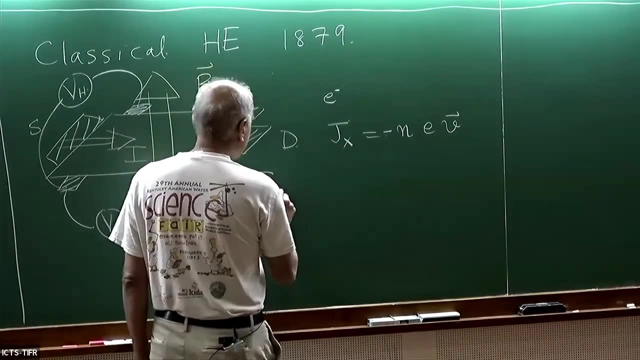 And this current density is the current per unit length. this is all in two dimensions. Okay, great. So the current itself, the current that you're driving, The current that you're driving is going to look like. so let me put some dimensions. 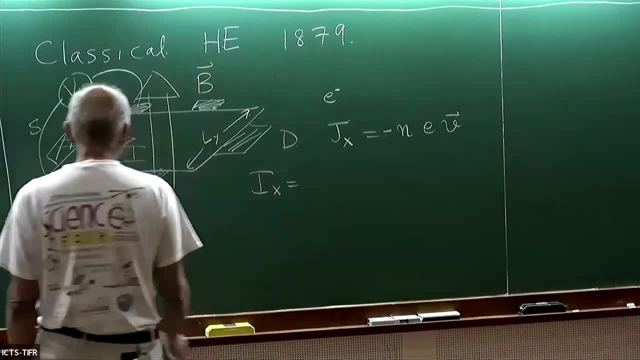 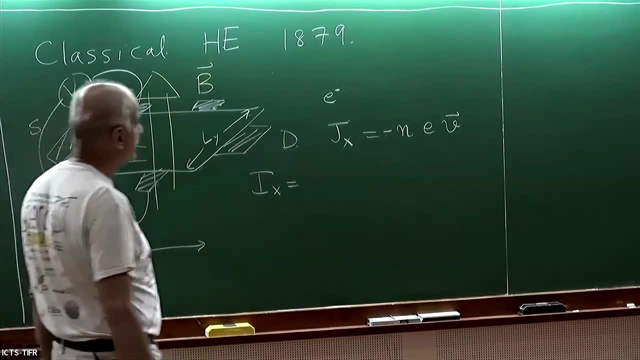 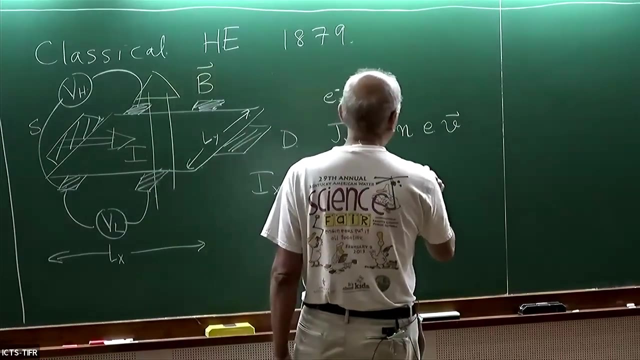 here. So this side is ly. we will not need the other side, but let me put it anyway. so that is lx. okay, So the current itself is going to be equal to jx times ly, right, And that will be minus nevx times ly. 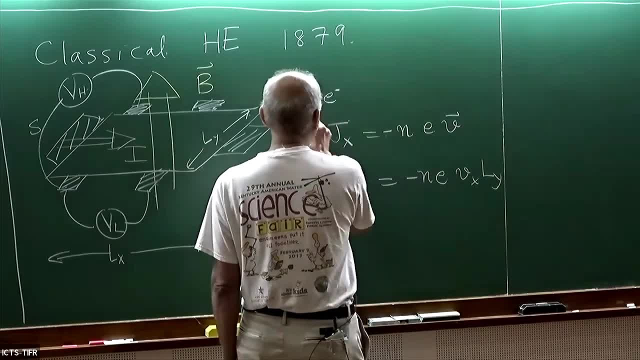 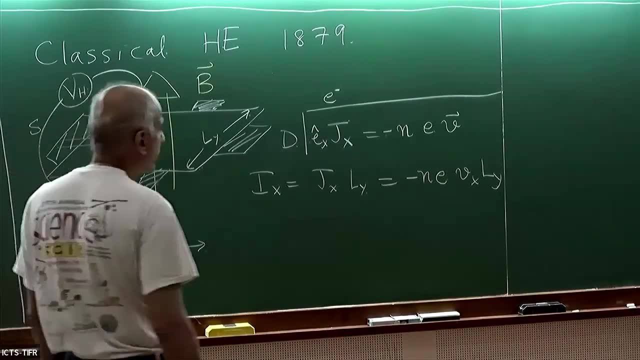 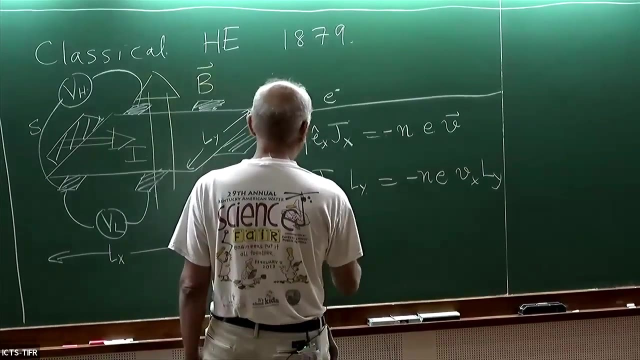 I did something bad here. I should have put a vector, okay. So there's that. So from that you can figure out what is the drift velocity of these electrons. okay, The drift velocity of these electrons is going to look like minus ix over nely. 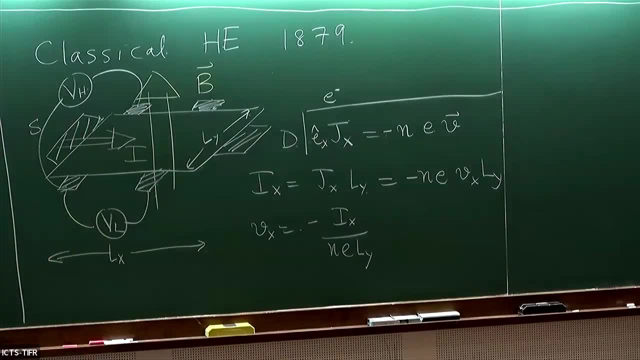 Okay, so these electrons are? they start out moving in the negative x direction then? so this is the velocity of the electron, Okay, And of course there's a Lorentz force, there's a perpendicular magnetic field, so there's. 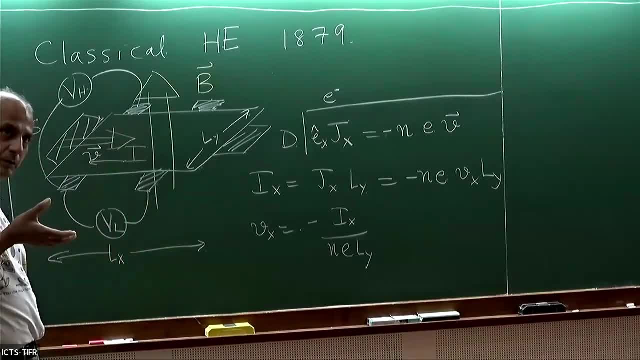 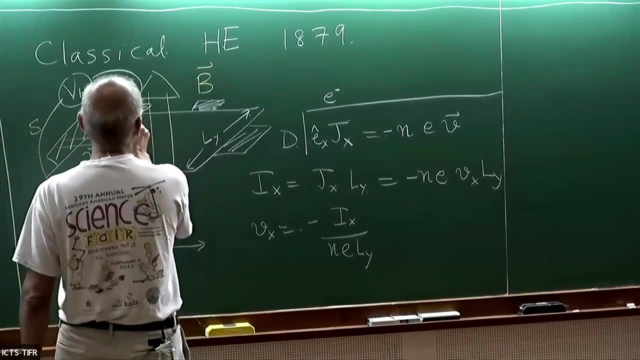 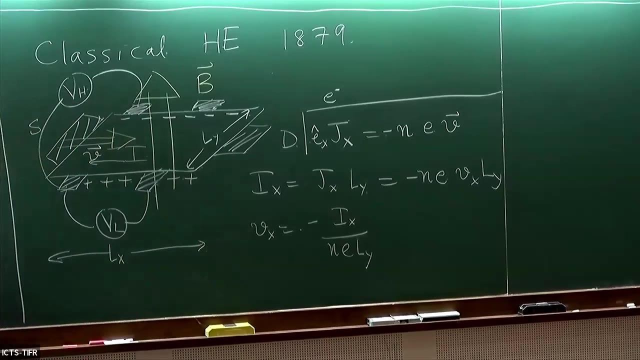 a Lorentz force. so the v cross b is coming out of the board, so the electrons charge is negative, so the force in the is into. So these guys, these electrons, start accelerating in the plus y direction and they start piling. 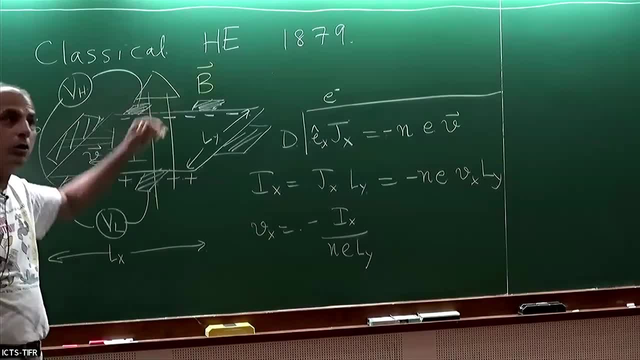 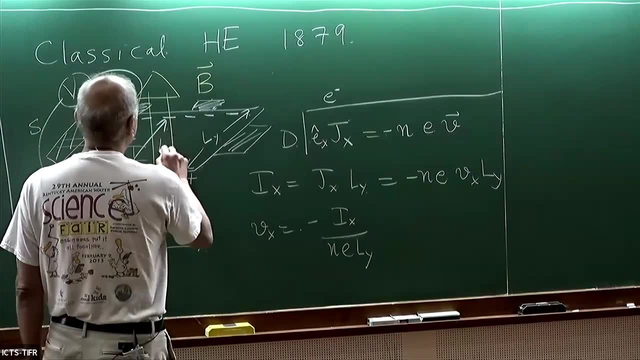 up against the edge. okay, because there's nowhere for them to go Once they pile up. What happens is that they create an electric field that's in that direction. ey, because it's like a parallel plate capacitor in some sense. right? 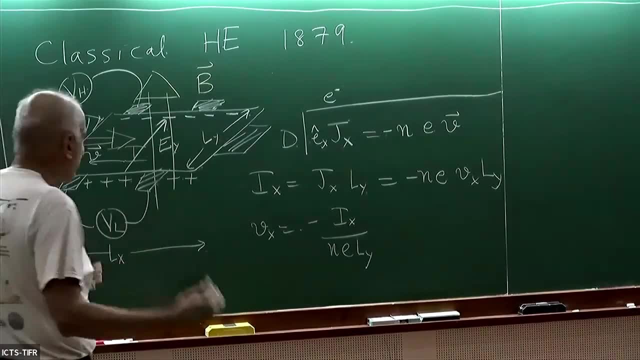 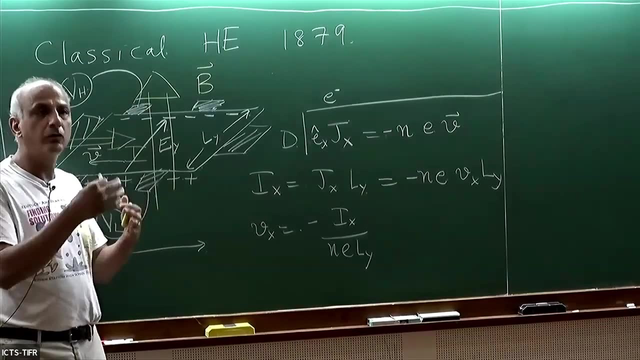 So they create an electric field and this electric field will build up and build up until such time as the force of this electric field exactly cancels the Lorentz force of the magnetic field that's trying to bend the electron up in y. Okay, is this clear? 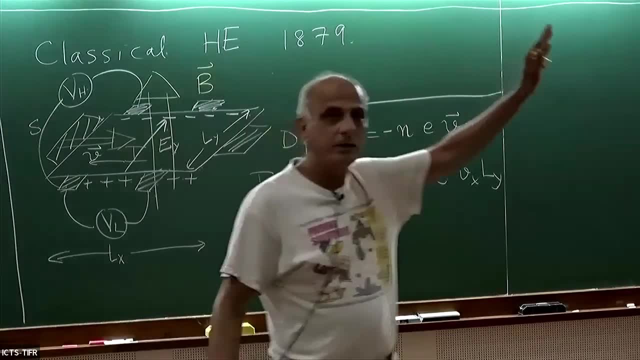 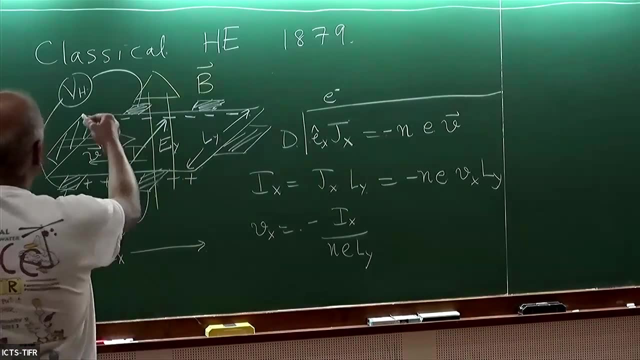 In your undergraduate, this is known something like this: Okay, Okay, So this is the. this is the, sometimes the velocity selector. yeah, This experiment was done at room temperature in 1881, and this experiment can be done at any temperature. Okay, in those days maybe the magnetic fields they had were just maybe a fraction of a Tesla, or maybe they had electromagnets that could make a Tesla or two Teslas. Nowadays we can go up to 40,, 50 Tesla and we can go down to, you know, milliseconds. 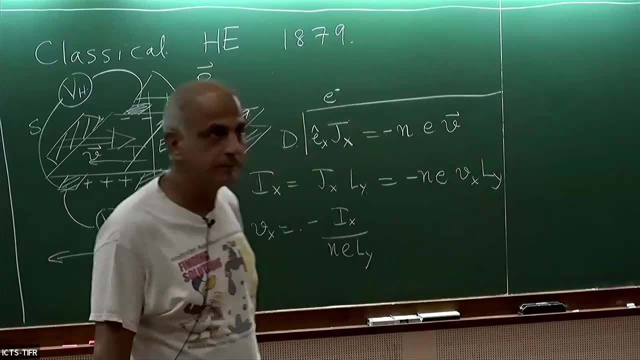 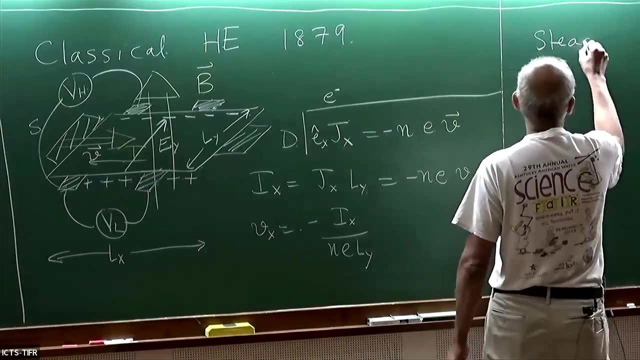 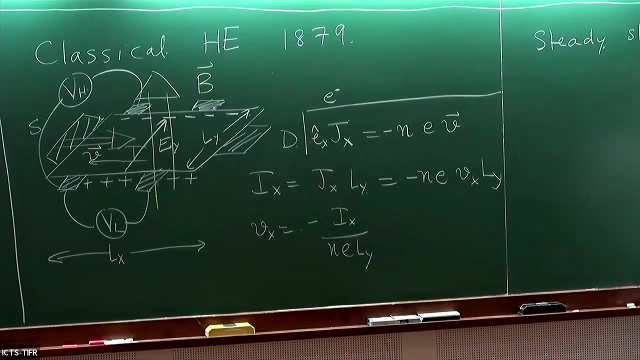 Okay, But this is all about the classical volume, Okay. so therefore, what you want in the steady state is that this E- y should be equal to V x times B, V z. right, Because Q e should be equal to Q V b. 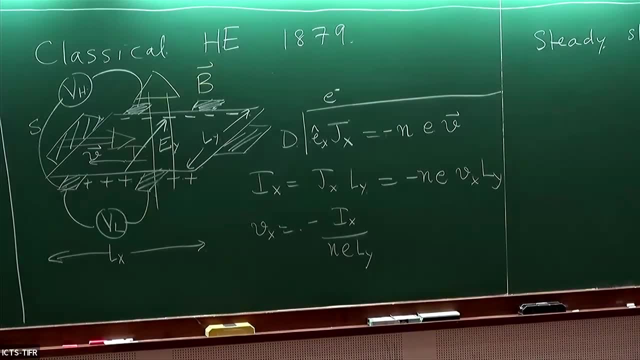 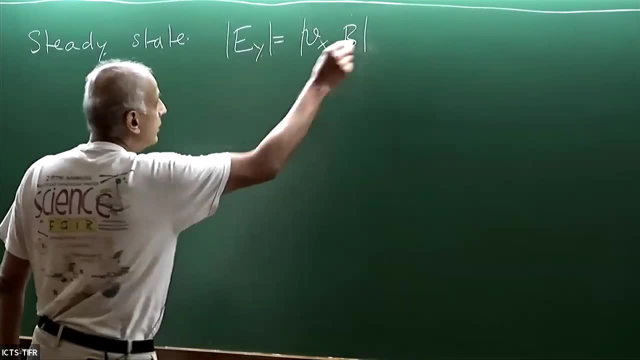 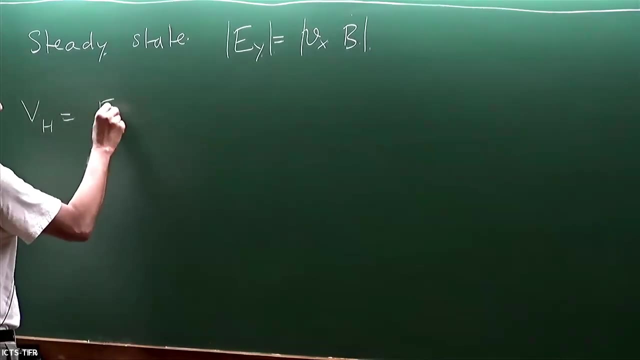 right, That's what should happen in order for the electric force to cancel the Lorentz magnetic force And therefore this in the steady state. so let me just talk about the magnitudes here of all these guys. right, And the voltage, the Hall voltage, is simply going to be E, y. 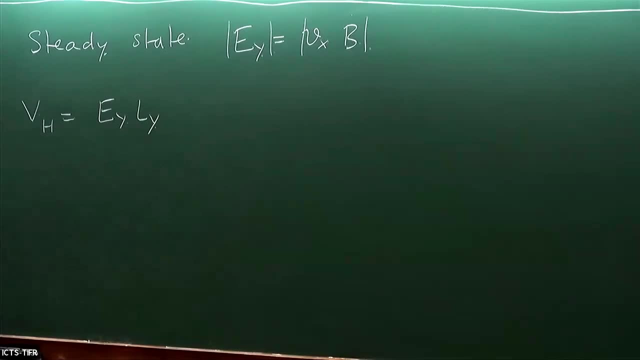 times L, y. right Again, the voltage is simply E times the distance in the y direction. If you don't follow it, please stop me. okay, I do have a tendency to talk a little fast, So if you find that I'm going too fast, 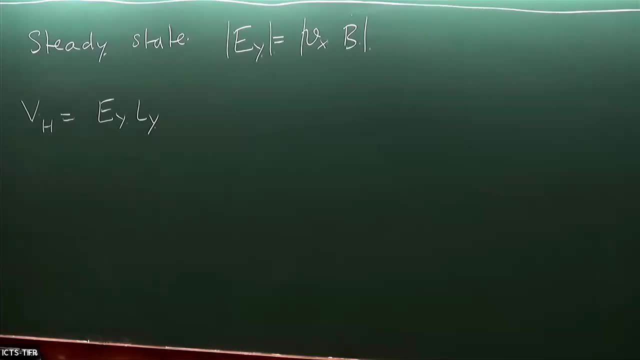 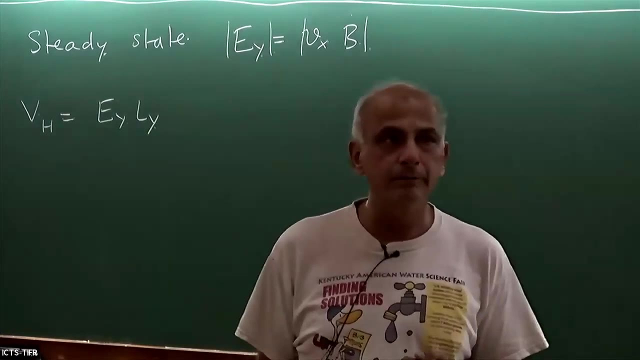 stop me and ask me to go over something. Let me also remind you that there is a tutorial session I'm going to give you. Guru Prasad has already given you some homework. I'm going to give you some more homework. It's all fairly simple, but we will be there in the evening between 6, 30 and. 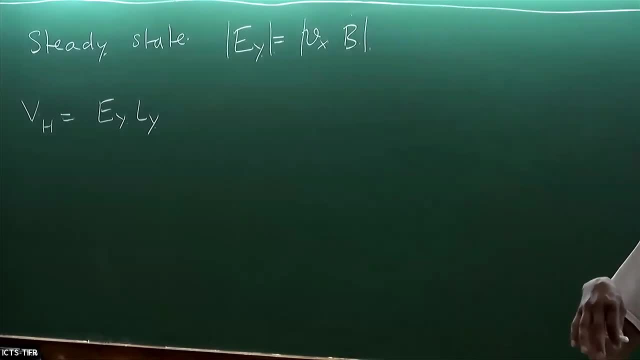 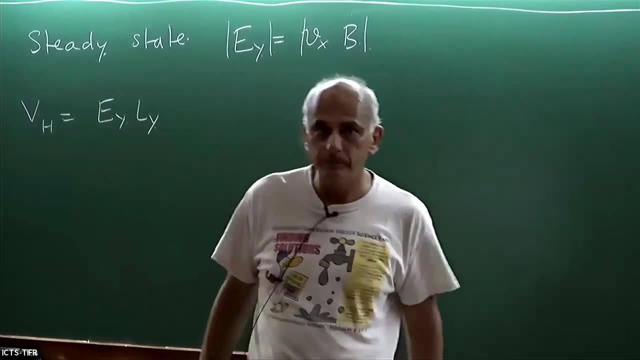 7- 30. Do we have the room here, Sumati? Okay, so we'll be here and we'll be here to answer questions, But really what we want is for you guys to do it, to solve it okay. 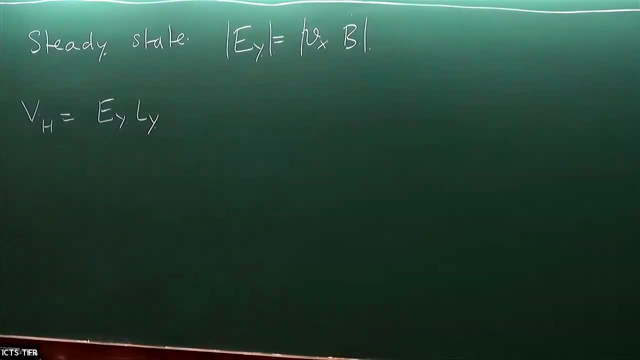 Any questions? so far? None. All right, so this is going to be equal to- let me just borrow all those things over there. So this is V x times B times L, y, and that is going to be equal to. what is it? I x. 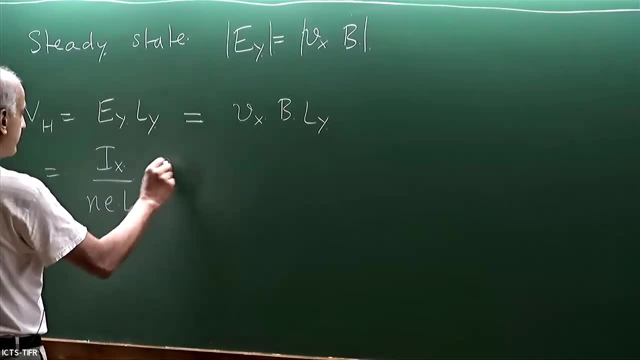 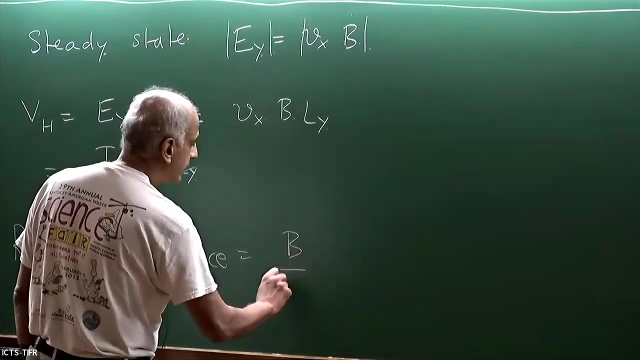 over N? e, Y, of x times- sorry times- B and Y and you can see that this cancels. Okay, so this quantity, very important quantity, known as the Hall resistance, is simply equal to B over N? E. I'm using MKS units Sometimes in the literature, you'll see. 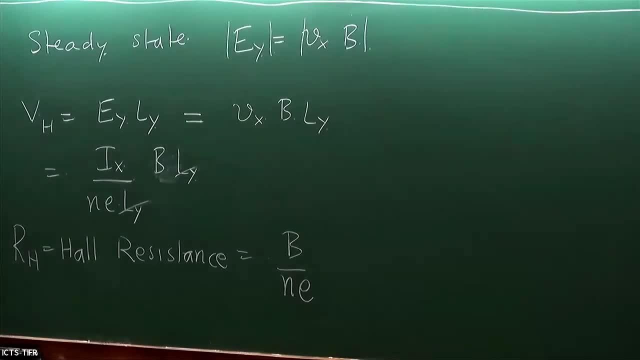 CGS units being used, and so there will be a C and at the bottom of that, but let's stick to MKS units here. So the situation is you have this, this sheet, with some constant number- density per unit area, and then you vary the magnetic. 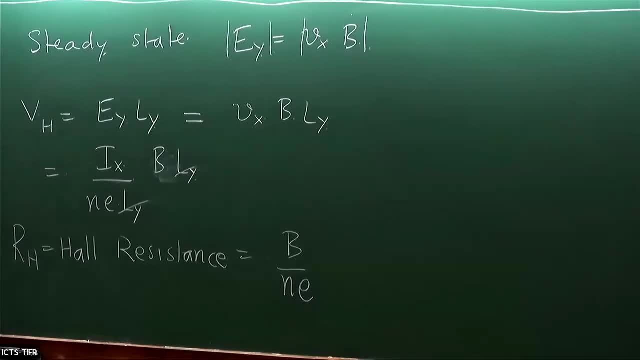 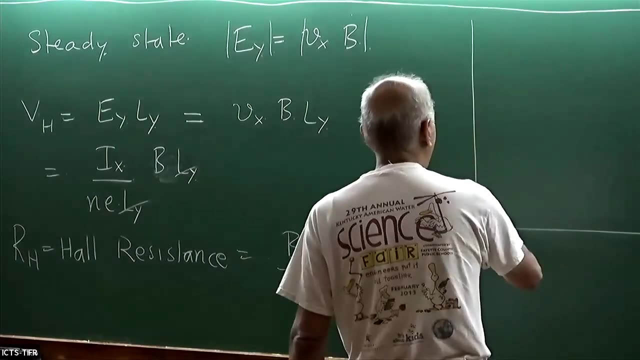 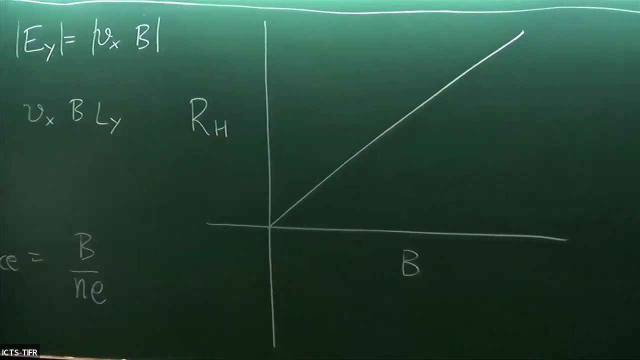 field and you ask yourself: what does the Hall resistance look like as a function of magnetic field? and what you will find is something that looks like that This is the magnetic field, This is the Hall resistance and this is the magnetic field, The slope of this guy. 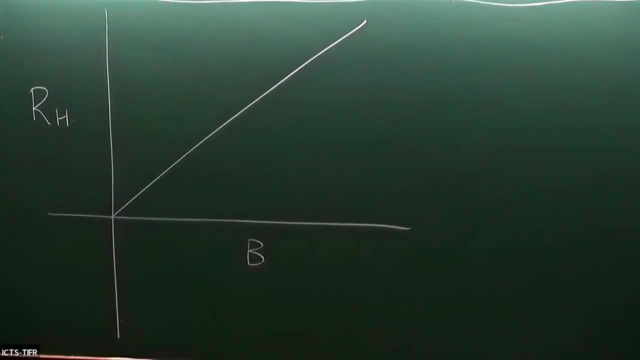 tells you the number density. So in fact, in a lot of condensate metal labs when you first make a material, you dope it. This is one way to find out what is the density. of charge carriers is to actually do a classical Hall measurement. 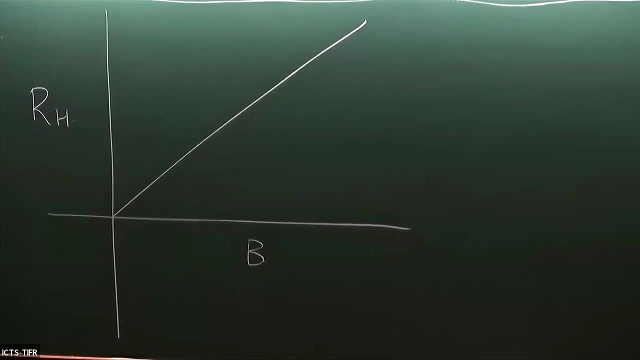 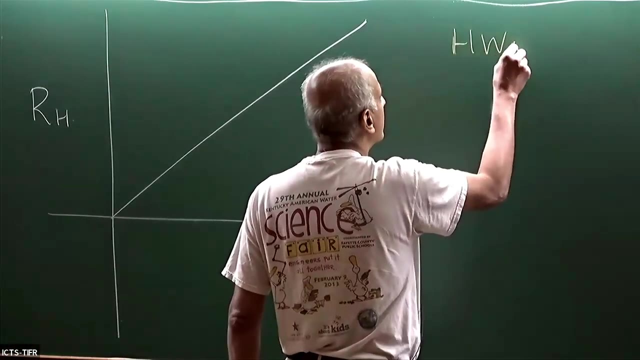 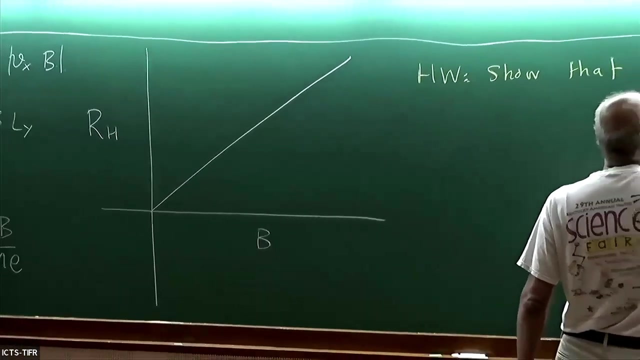 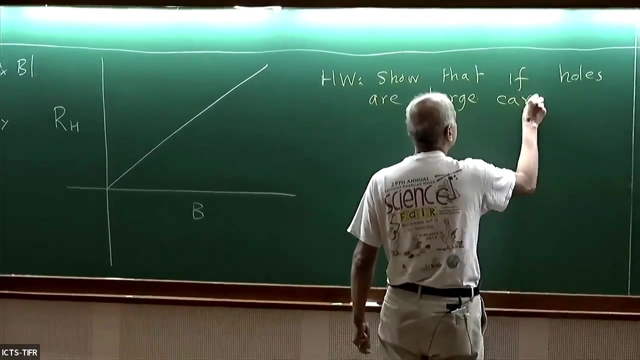 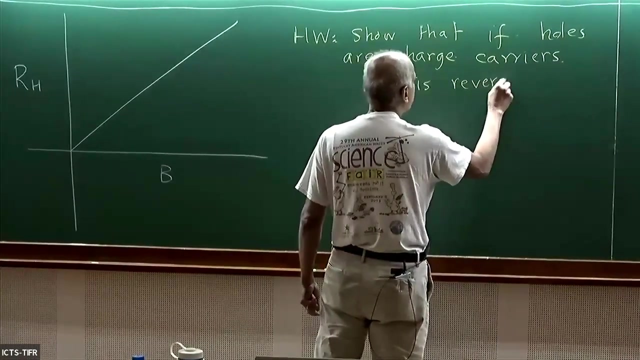 and look at the slope That tells you 1 over N. In fact. the homework, so let me say homework- show that if holes are the charge carriers, then the Hall is reversed, So the sign changes. It's very easy to show, So go. 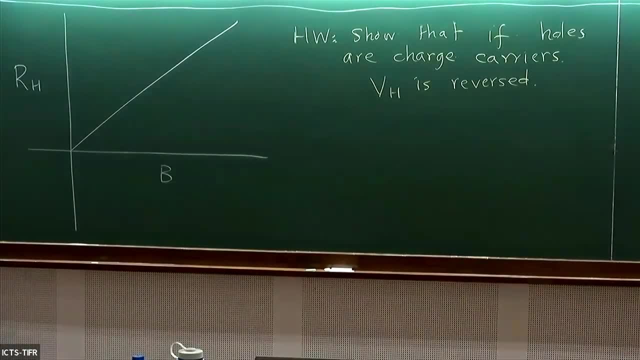 ahead and show it and if you have trouble, then then come to the. well, anyway, come to the tutorial anyway, because even if you don't have a question, somebody else will have a question and that may help you to understand other stuff. Okay, so this is what is observed at room temperature. Okay, very good, So that was. 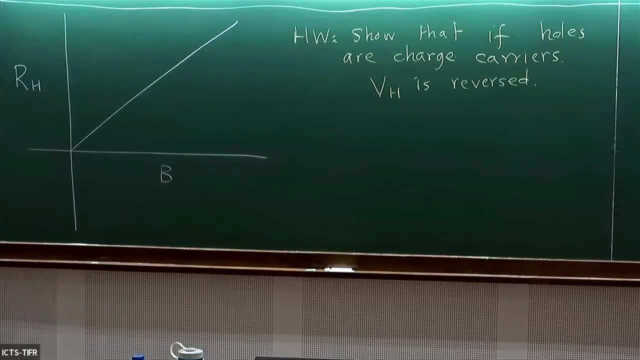 the classical Hall effect. What about the quantum Hall effect? The quantum Hall effect is the following observation: that if you reduce the temperature, you make the systems really, really clean And you reduce the temperature to, let's say, a fraction of a Kelvin. 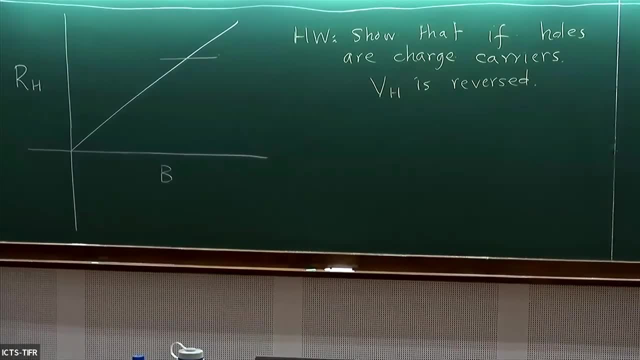 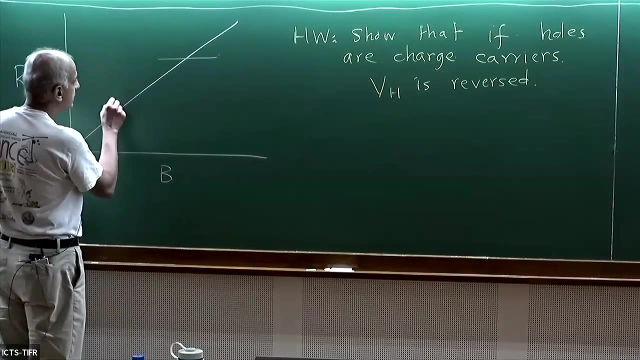 You make the magnetic field really large, Then what you start seeing is a deviation. So at high temperatures, this is indeed what the Hall resistance looks like as a function of magnetic field. But as you reduce the temperature- if your system is good enough- then you will start seeing some stuff that looks like this: 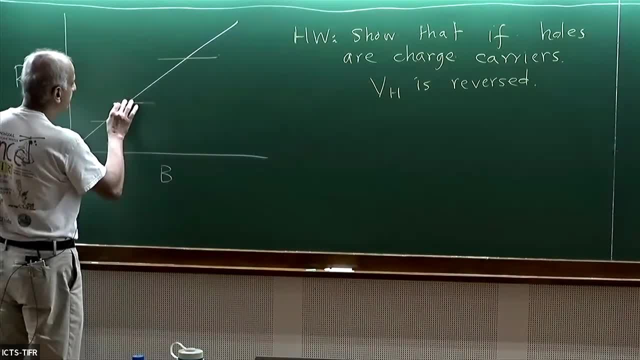 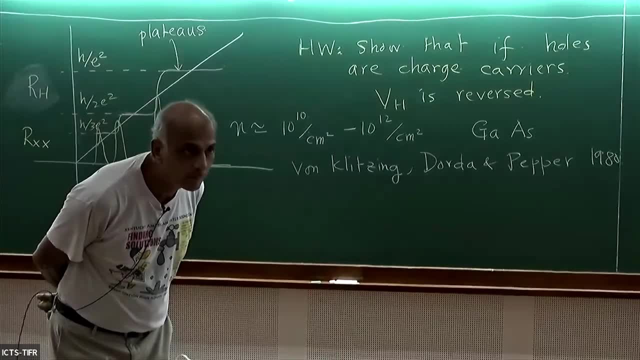 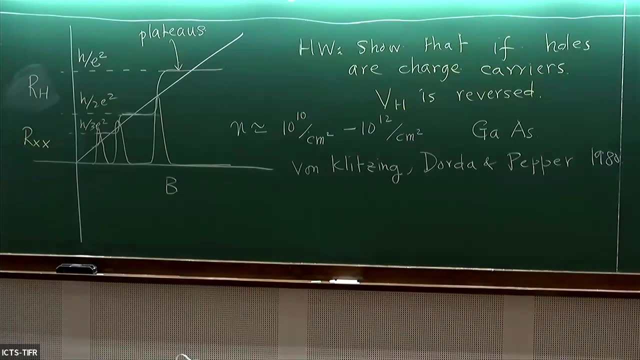 Okay, And you know there's a very nice picture that I copied from. Yes, yes, you will see. okay, You will see in due course of time what it is. you're right, there is some energy scale that you have to go below in order to see the quantum model. yeah, 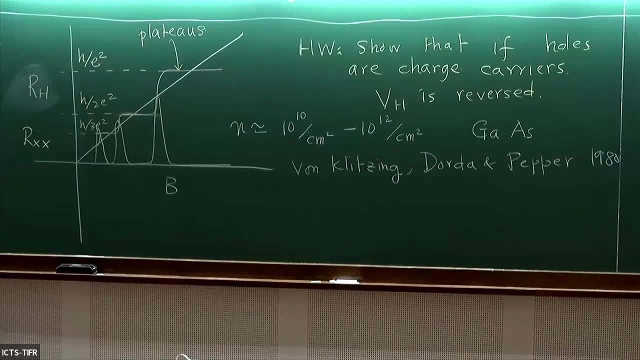 Well, as far as steady fields are concerned, I think people have gone up to 35,, 40 Tesla. Now, if you want temporary fields, okay. there's some kind of an explosive device, okay, where you destroy the sample but then for some fraction of a second, you take data while 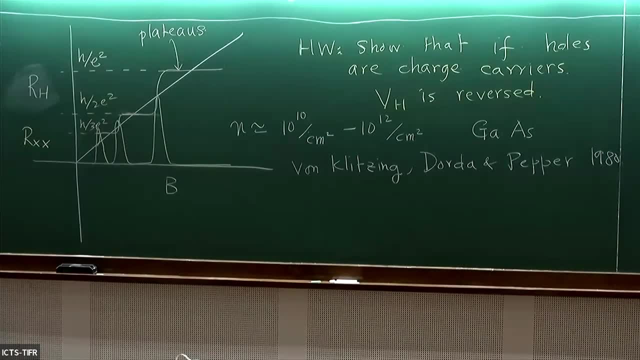 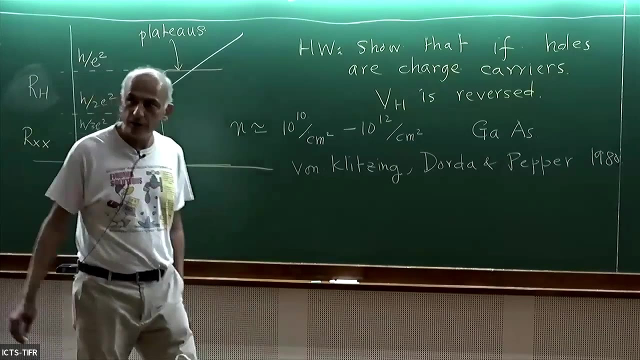 you're, you know, and you can ramp up the field. so I believe, like of the order of 100 Tesla, The peaks here depend upon the amount of disorder in the sample, They depend on the temperature, They depend on many things, okay. 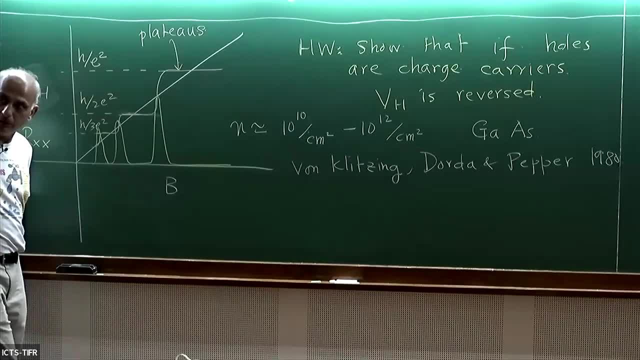 So what is universal in every sample is the fact that there are these plateaus, the fact that these plateaus are at quantized values, okay, of h over e squared, some rational multiple of h over e squared, and whenever the Rxy or R Hall Hall resistance is on a plateau. 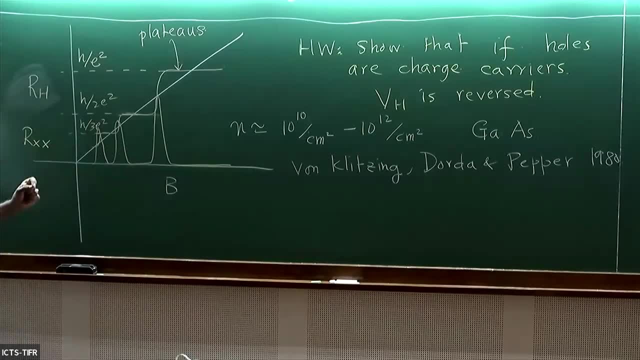 the Rxx is zero and as you reduce the temperature, the quantization of this guy- how close is it appears to h over e squared or rational multiple- becomes better and better. In fact, this is now the standard. The resistance standard is a quantum Hall resistance. okay. 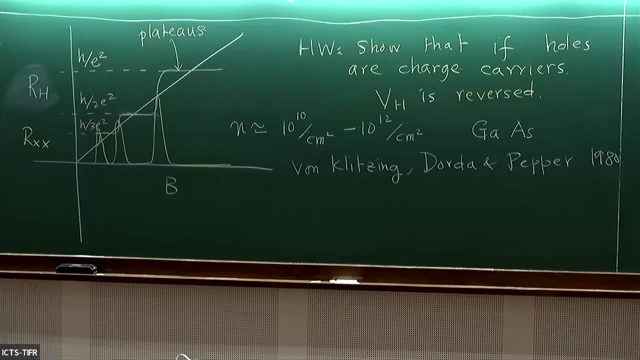 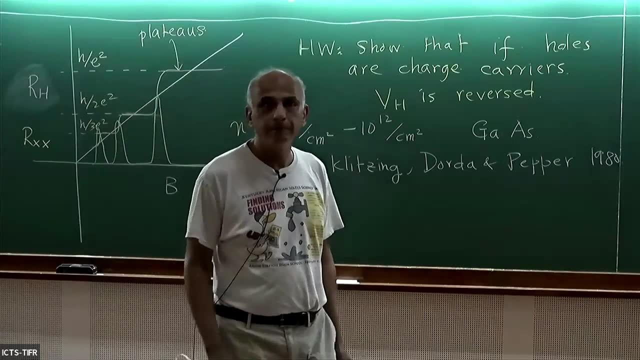 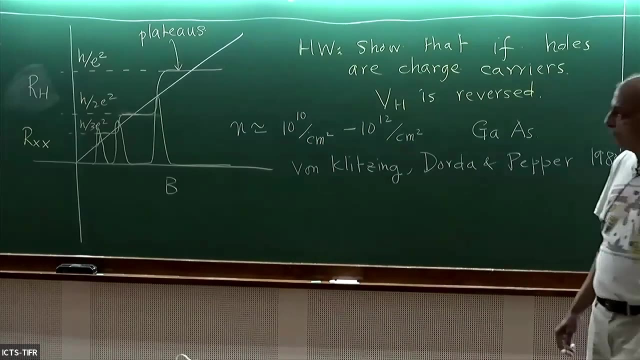 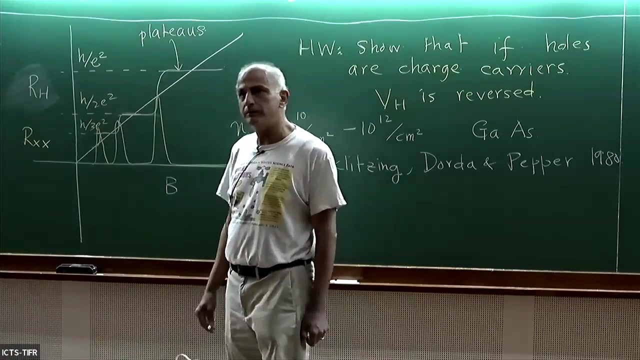 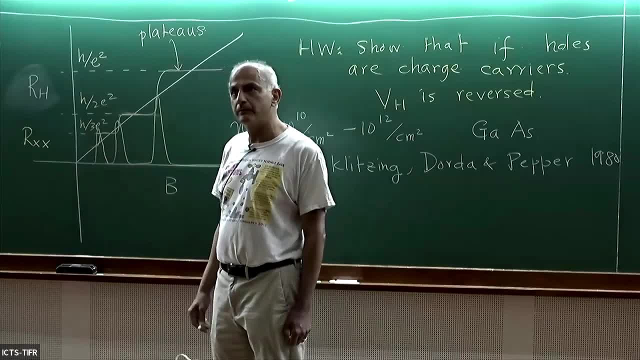 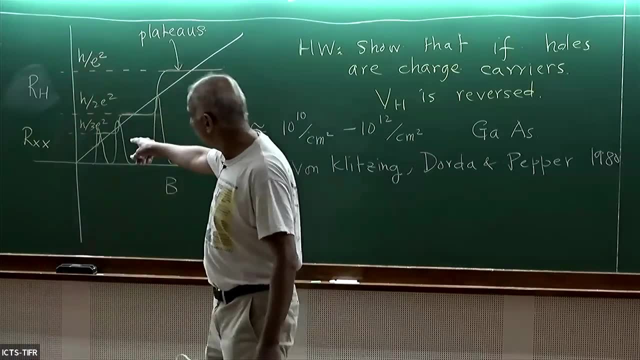 There are a lot of plateaus crowded in here that I'm not showing you. If you look in the picture that I have in the notes, okay, you will see many more peaks, many more plateaus of Rxy. This picture is actually a lot more complicated than I'm making it out to be. 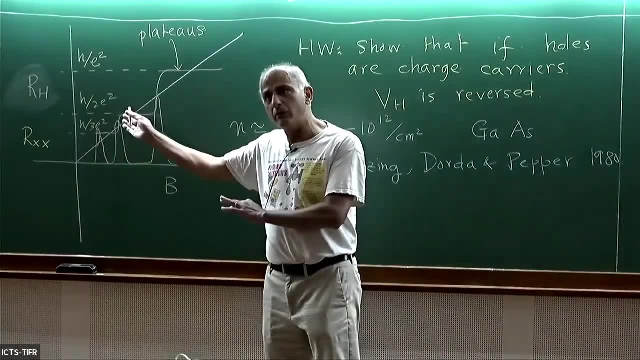 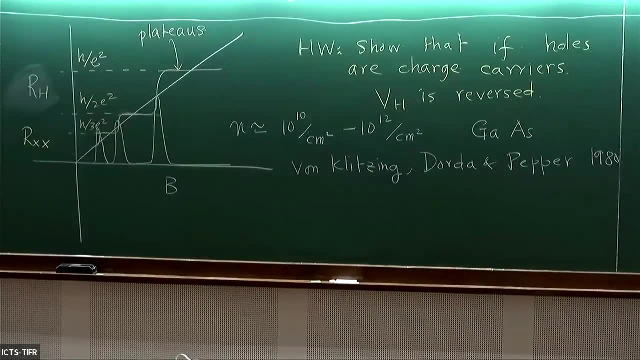 In between these two. there are other plateaus that I'm not able to draw for you because my drawing is not good enough. As you raise the temperature, Very good. So as you raise the temperature, let me draw a. If I raise the temperature. 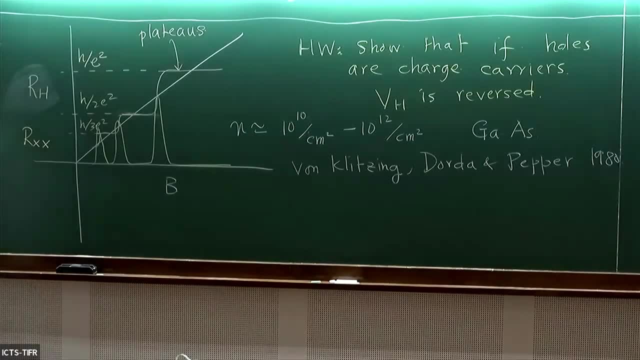 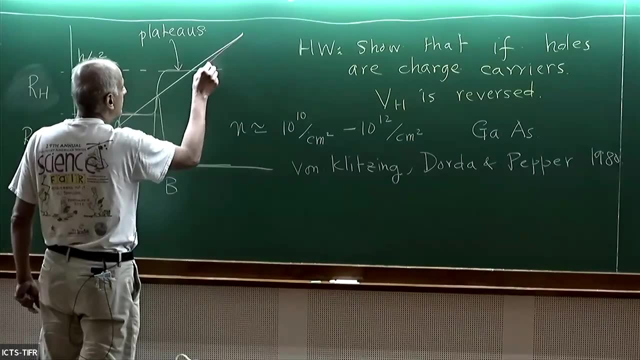 So this is at some temperature, let us say some very low temperature, let's say a few millikelvin. If I raise the temperature, then what's going to happen is that this plateau is going to become something like that. These plateaus are going to become very small. 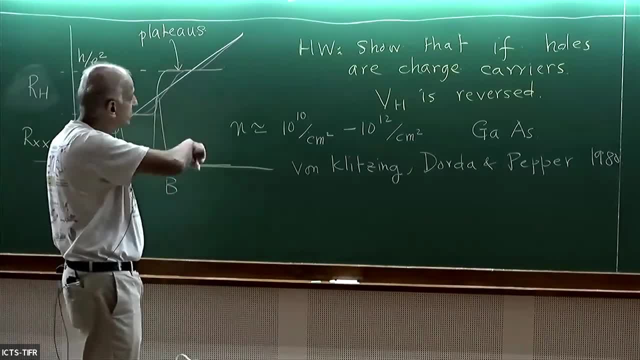 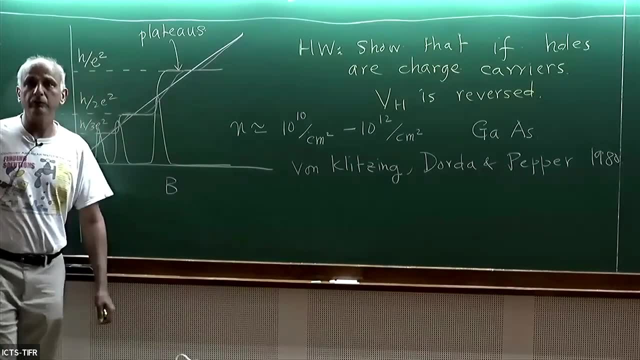 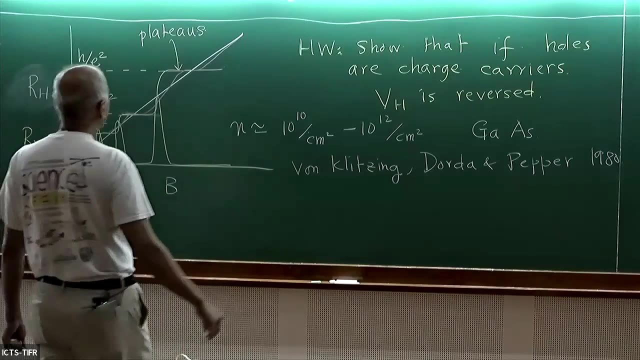 They're going to become less broad And these peaks are going to become more So this Rxx will not touch zero. instead, it will just oscillate, maybe never touching zero. It will tend to more and more towards the straight line that you see at high temperature. 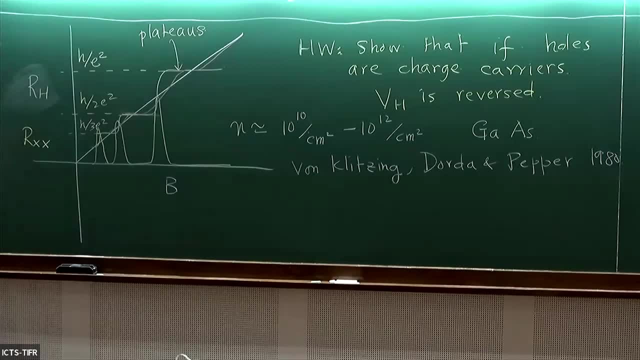 Okay, So the white straight line is what you see at high temperature in any sample that's metallic, So it will go towards that as you raise the temperature. Other questions? Yes, So the thermal transport also has been done very recently. 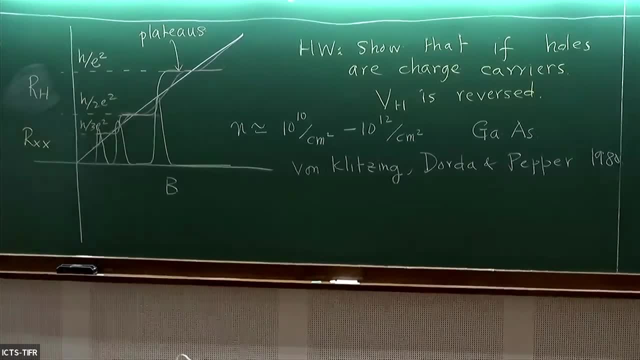 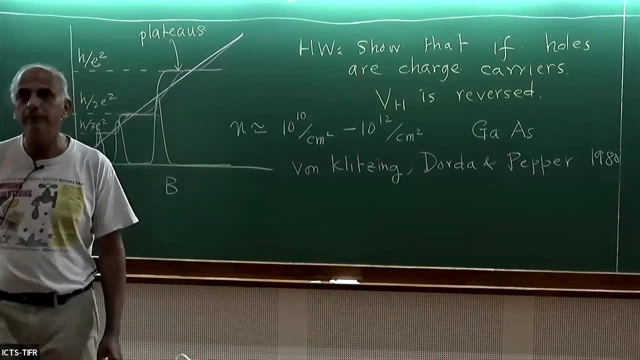 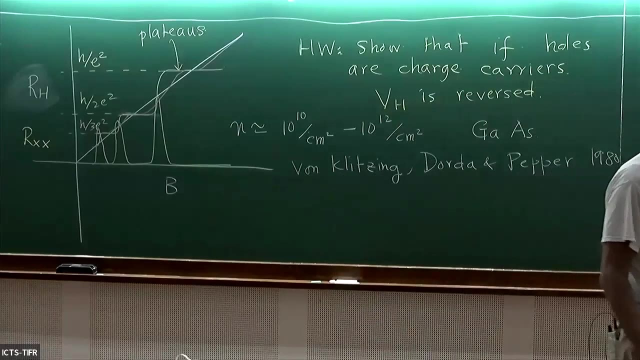 We will talk about that later. There is some quantized thermal transport also. that happens. We will not talk a lot about it, but if you ask me at that point, okay, Yes, That is a very interesting question. We don't actually know what happens. 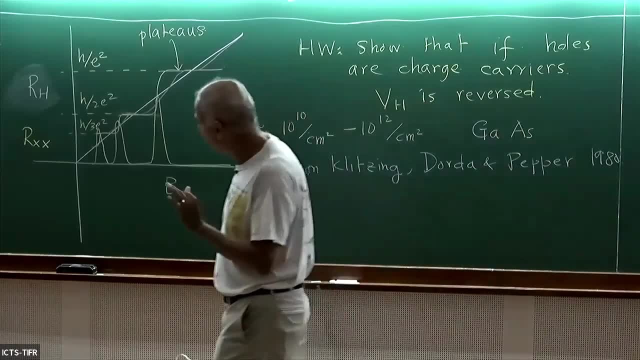 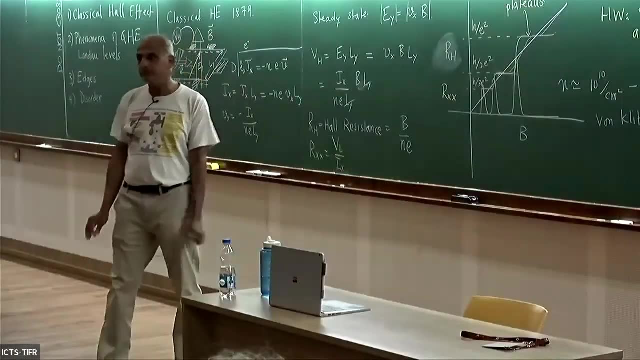 Okay, What happens? It depends upon the degree of disorder in the system. So in between these integer plateaus there are other fractional plateaus that occur. Okay, And so especially between, let us say, this guy and that guy, there are several fractional. 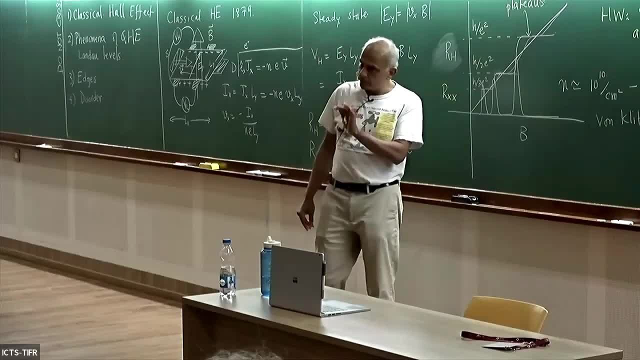 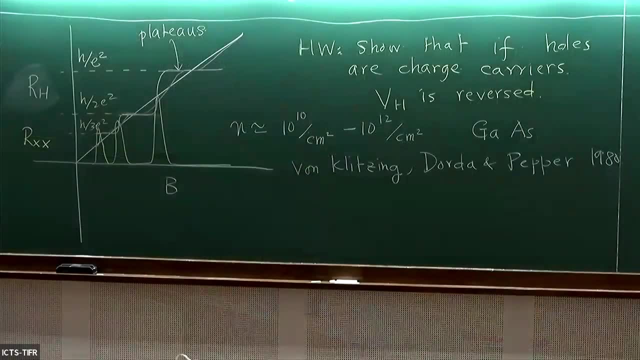 plateaus. So if the system is very clean, then you'll see a lot of fractional plateaus between the two integer plateaus. Okay, But yes, eventually you expect to see a bunch of steps of different heights and different Okay. 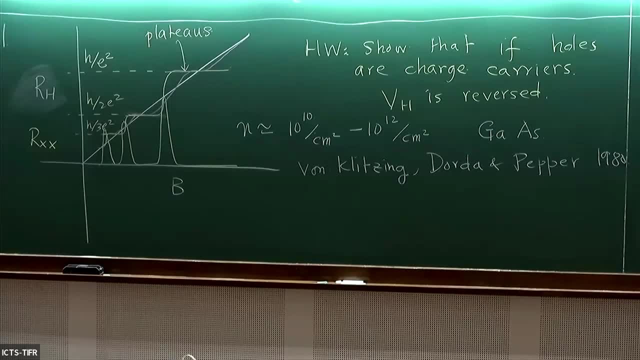 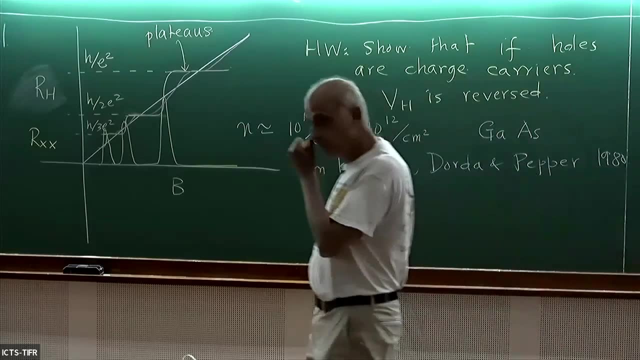 Other questions. Okay, This is good. There are lots and lots of questions. Yes, Yeah, Which one? Right, Right, Right, Right. So all I'm saying is that, because of the Lorentz force, when I switch on the current, 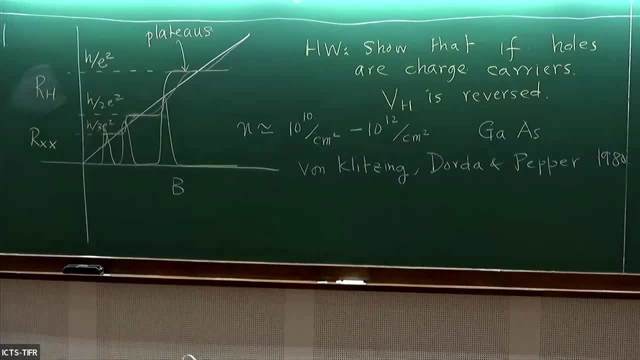 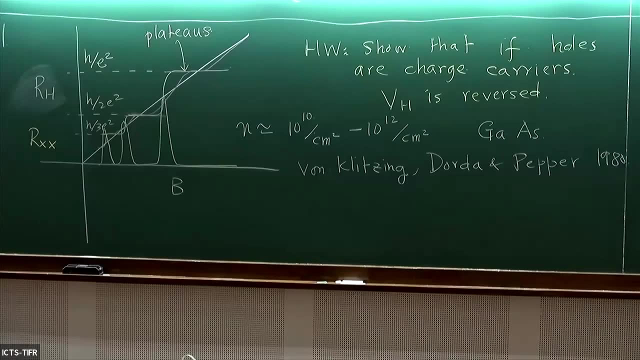 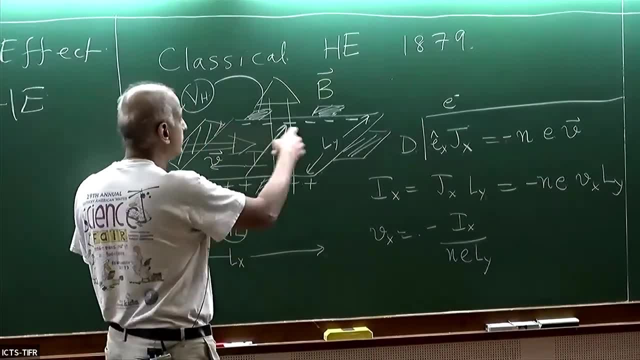 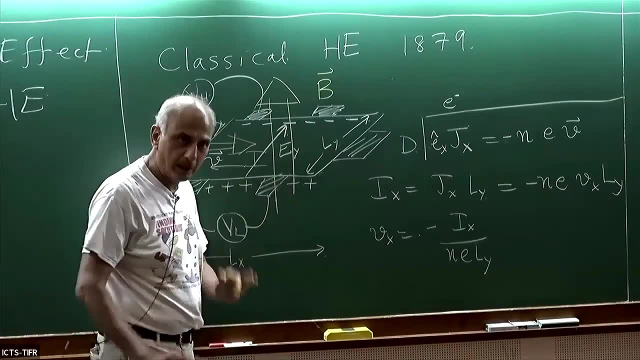 Yes, They go there. Yes, Successful, Perfect. At some point the electric field force will counter balance, the Lorentz force and the electrons will move straight and no more charges will pile up there. Okay, So when I say It's localized, 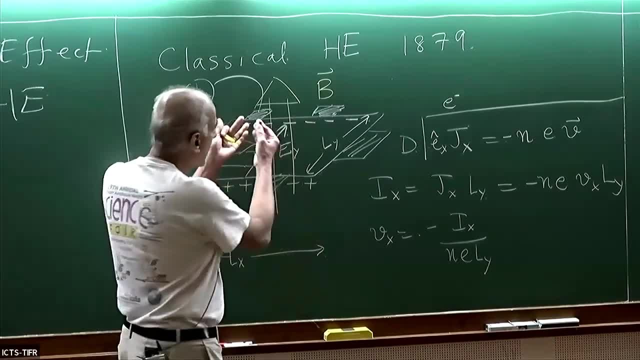 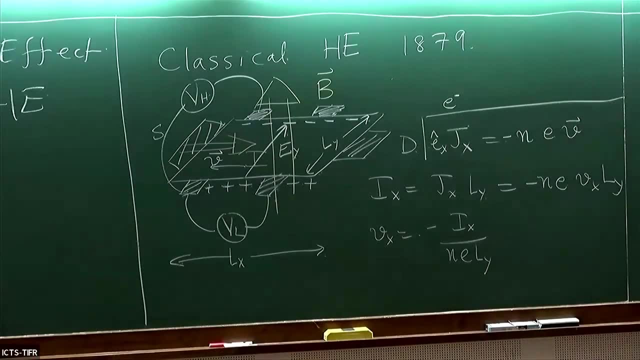 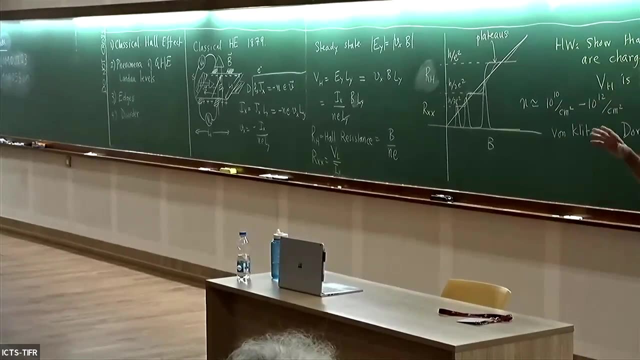 No, they're not localized. These charges may be moving, they may not be moving, but there is some excess negative charge here and there is an excess positive charge there. Okay, Good, All right. So now let's get to the quantum Hall effect. 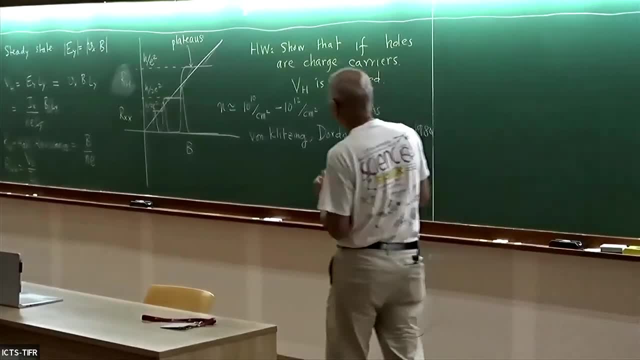 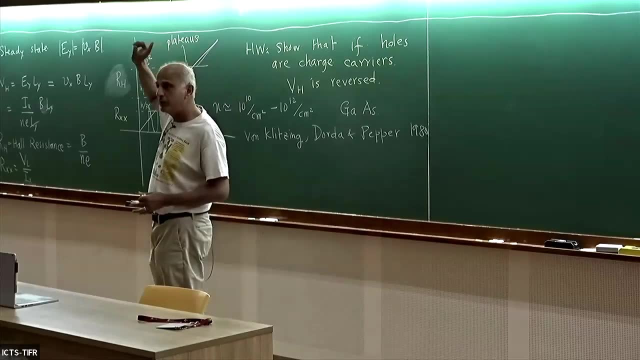 Okay. so this it turns out, even though it appears very strange, this phenomenon, you know, not counting this other stuff that I'm telling you about- at 3 h over e squared, and so on, this phenomenon was understood within two or three years of its discovery. 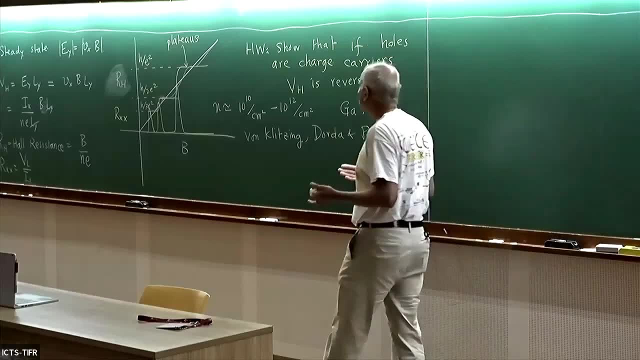 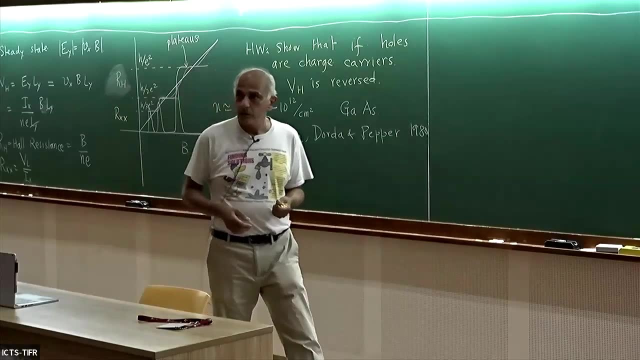 So let's understand what it is. So first of all, you know, just from the fact that the h appears, Planck's constant appears, that this must have something to do with quantum mechanics. So we start with our basic quantum mechanics and we say: you know what is the quantum mechanics of electrons? 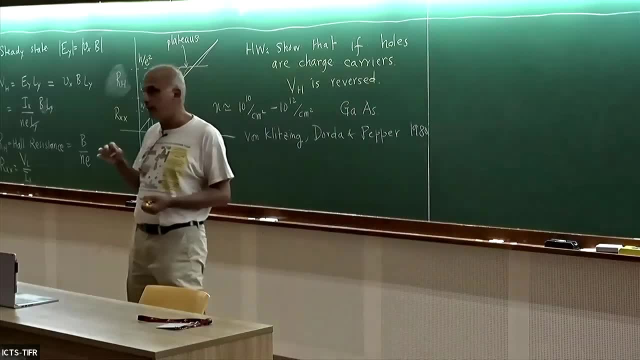 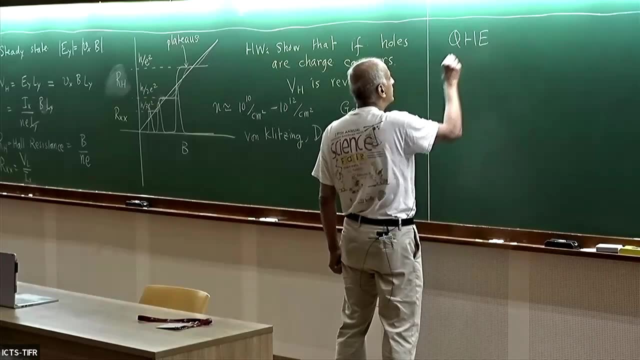 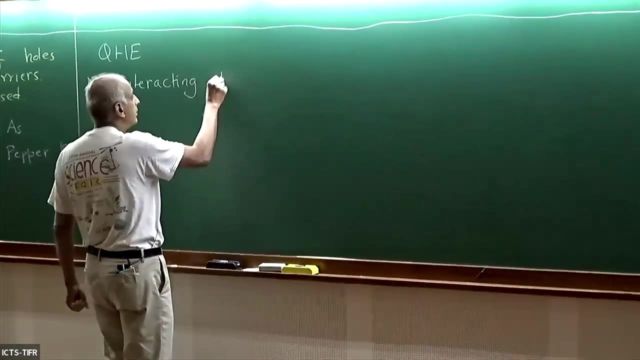 moving in a plane subject to a perpendicular magnetic field, right. So we want to set up the quantum mechanics of that and the simplest level. what we want to do is non-interacting electrons And a lot of it, the integer quantum Hall effect. 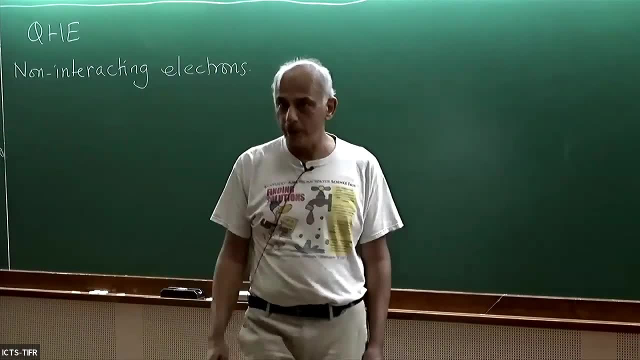 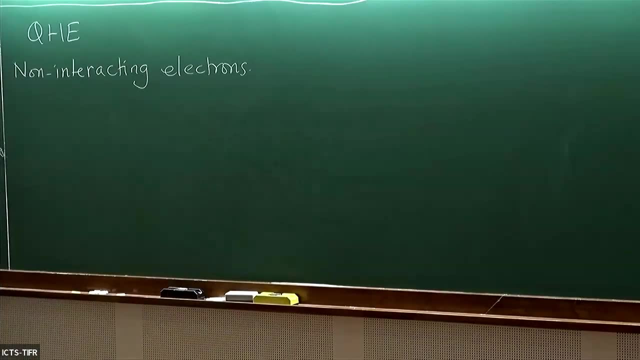 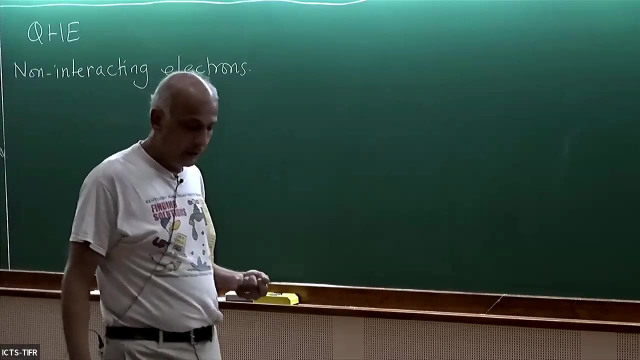 can be understood by thinking about non-interacting electrons. So let's do that first, and then we'll turn on the interactions, and then we'll see what extra stuff they bring out. Okay, So you probably all know that when I do something, so when you do quantum mechanics, you have to do it in the Hamiltonian formalism, right? 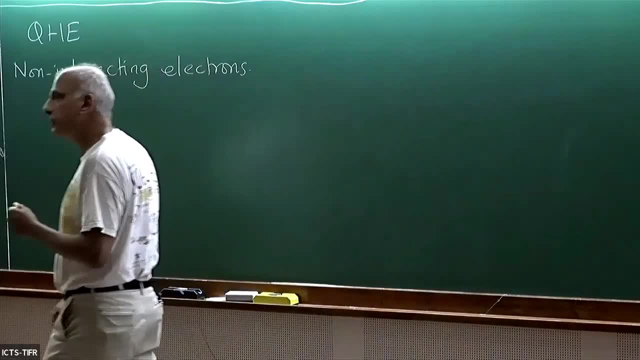 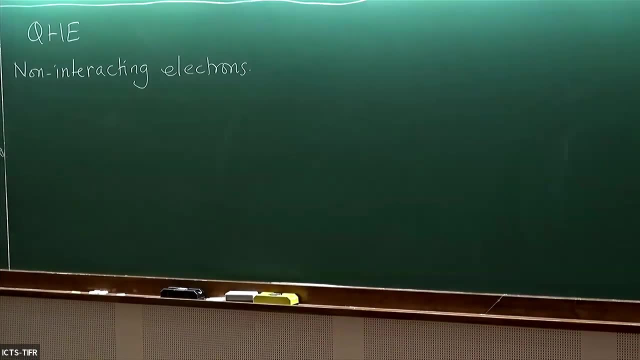 And when you do even classical mechanics, in the Hamiltonian formalism, if you're talking about charged particles, they don't talk directly to the electric and magnetic fields. In fact they talk to the vector and the scalar potentials. That's how in Hamiltonian formalism you couple charged particles to electromagnetic fields. 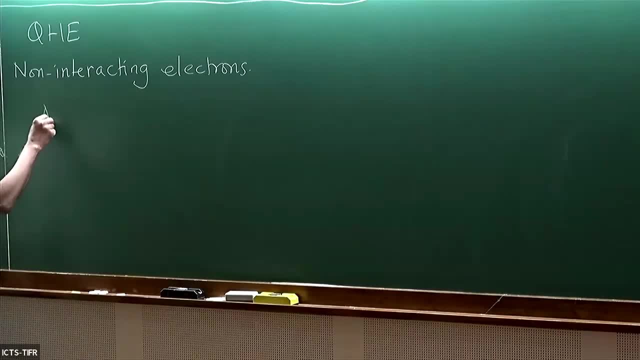 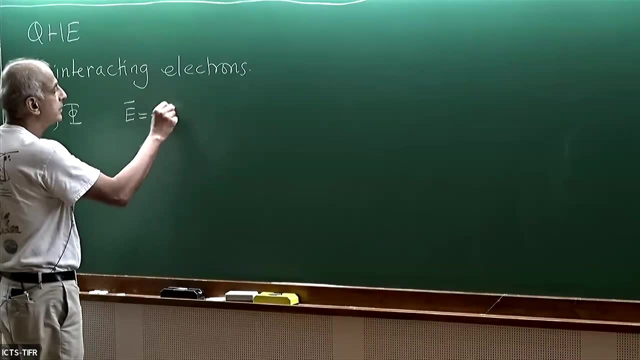 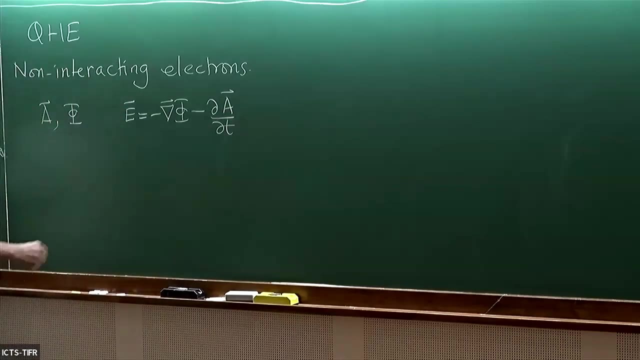 So how does it work? So there is a vector potential and there is a scalar potential. They're connected to the electric and magnetic fields by these relations. again, I'm using MKS. okay, and B is simply the curl of A, and given this, the way that 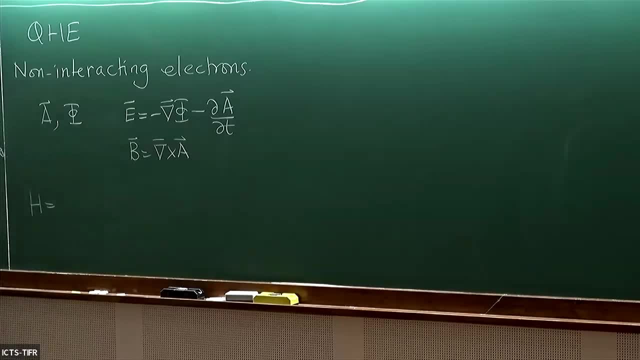 the Hamiltonian is written down. so let me first write down the classical Hamiltonian. so if I have a particle of charge Q, then I will write down the Hamiltonian as P minus Q times A plus Q times Phi. this will be my classical Hamiltonian and the way that the coordinates of the particle appear. 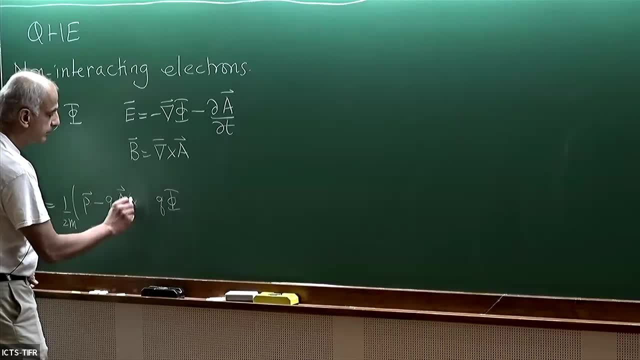 inside here are in these things here. so there's some X and T squared. this X is the coordinate of the particle itself. that is how X. so the Hamiltonian should be a function of X and P. that's how X appears here. and then of course in the 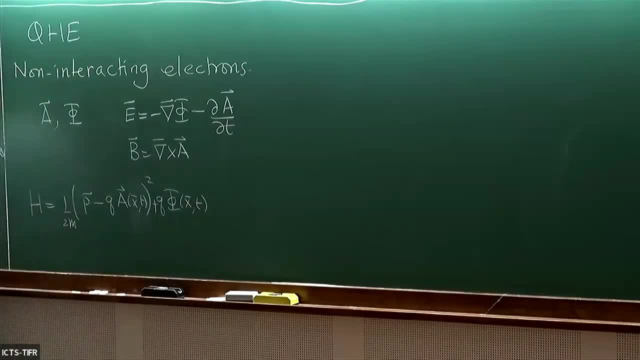 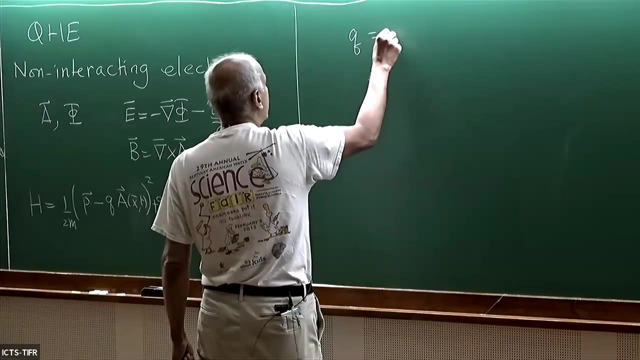 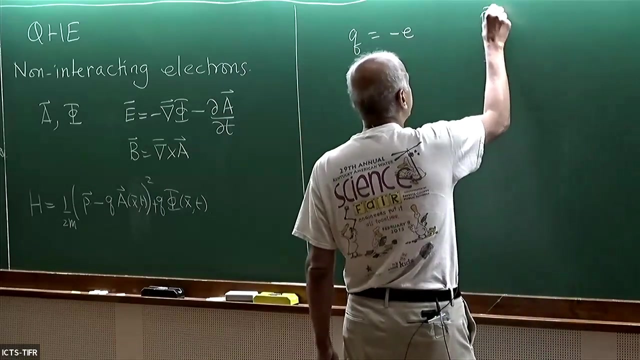 scalar potential also, it may appear okay. so that is what the Hamiltonian of a charged particle looks like. okay, so now we are going to take an electron, so it's minus E. and to make my own life simple, okay, I'm going to choose a magnetic field to be pointing along. 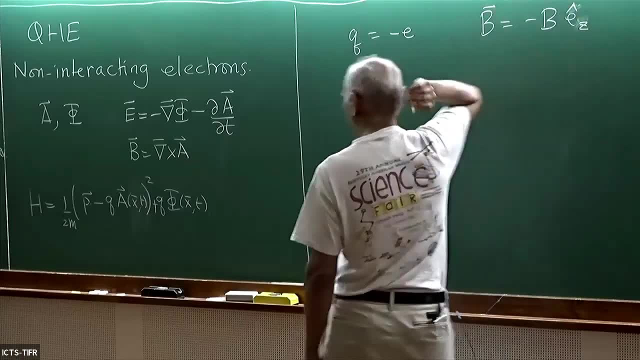 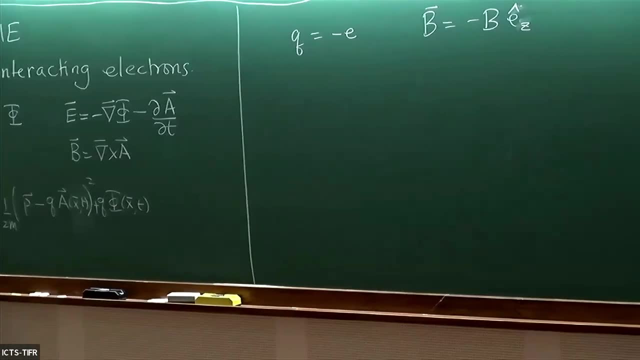 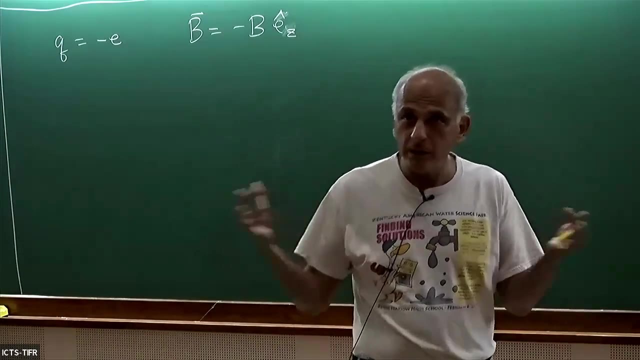 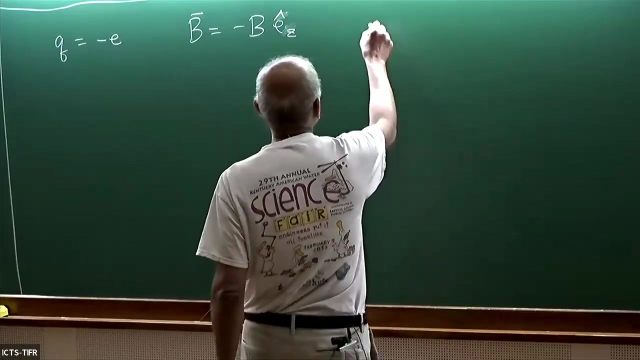 the negative z-axis. okay, because it'll make something simple for me eventually. okay, all right, so I have this, and now there is no electric field. at the moment, I'm taking the simplest possible situation where there's only simply a magnetic field, and so therefore I don't need a scalar potential, so let me set Y equal to zero. 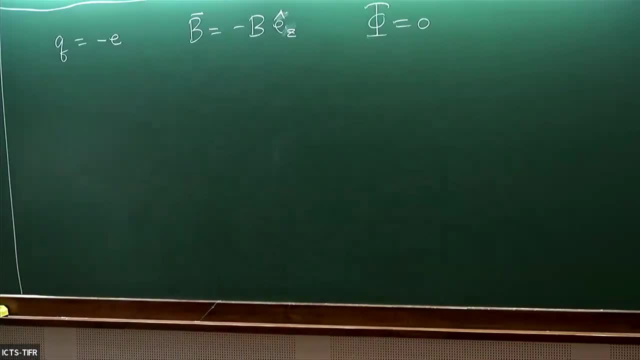 and this B is a constant. there is no time dependence. I get some time independent Hamiltonian. now there's one thing that you have to worry about whenever you talk about quantum mechanics or even classical mechanics of electromagnetic, of charged particles, which is gauge transformations. so you know that E and B don't uniquely specify a and Phi. right, you can always make a. 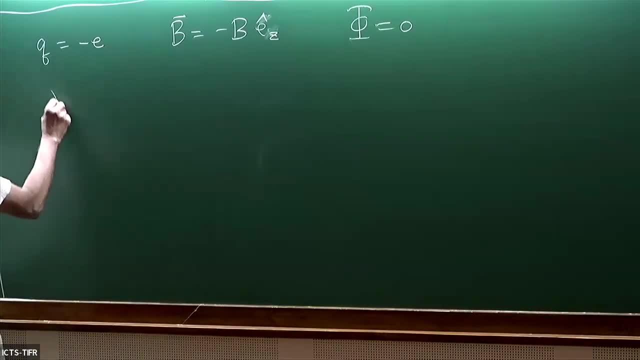 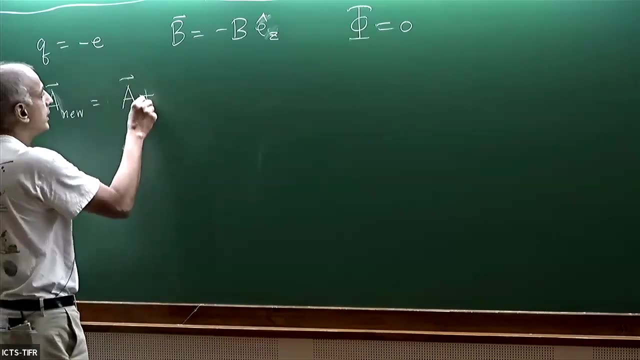 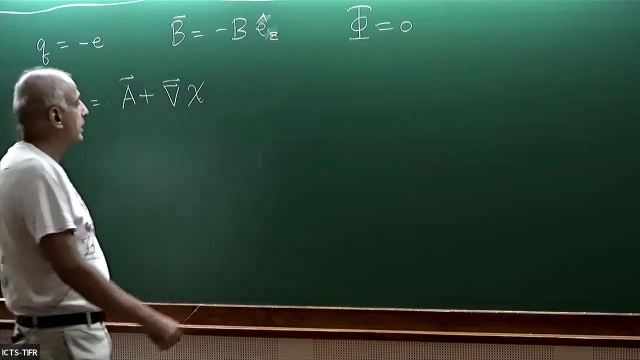 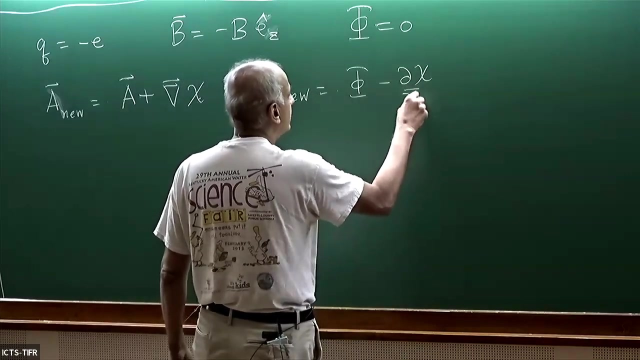 gauge transformation and it will look something like this: you take some, so you take some, some a new, let's say, and this would be some a plus the gradient of some smooth scalar, some function of space and time, perhaps okay. at the same time, if you let Phi go to Phi minus B, Chi by DT, then E and B remain unchanged. 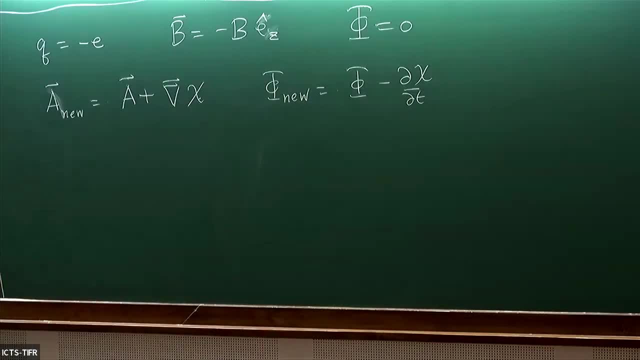 and therefore the physics should remain unchanged. so when you solve for the quantum mechanics or even the classical mechanics of a charged particle, you have to pick a gauge in which to do business. so what we are going to do is we're going to take a rectangular sample first. so let me take a rectangular sample. I'm 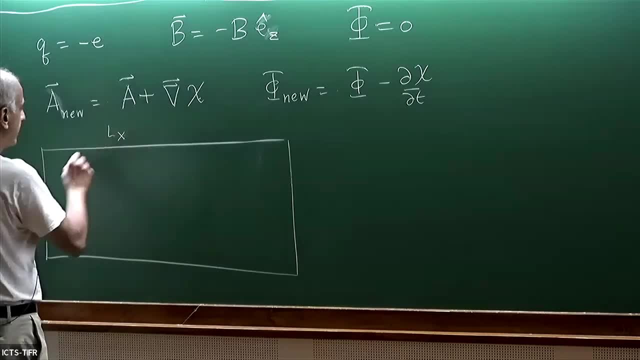 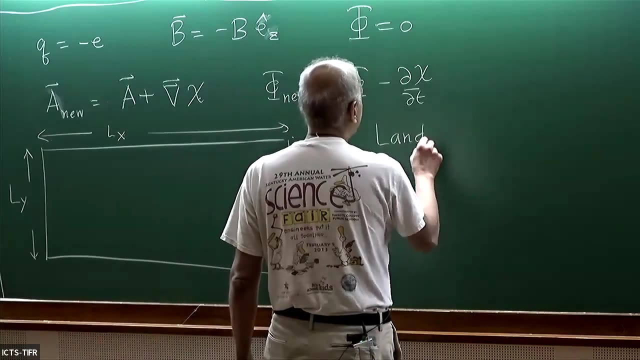 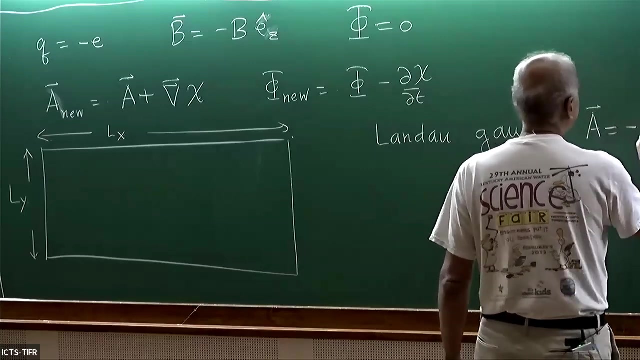 going to do some more stuff to it in a minute, but let's start with the rectangular sample. I have L X and I have L Y and for this particular geometry of sample the most convenient gauge is something known as Landau gauge. so I'm going to choose Landau gauge and my Landau gauge will look like A is minus B. 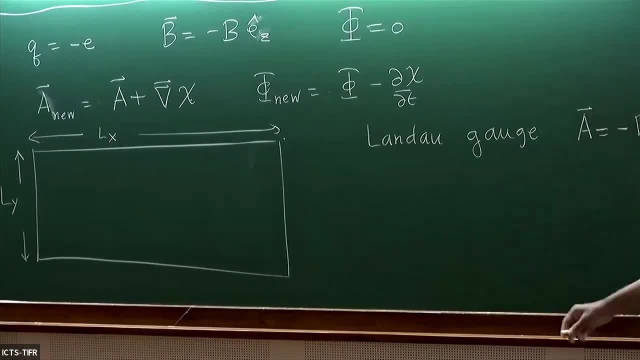 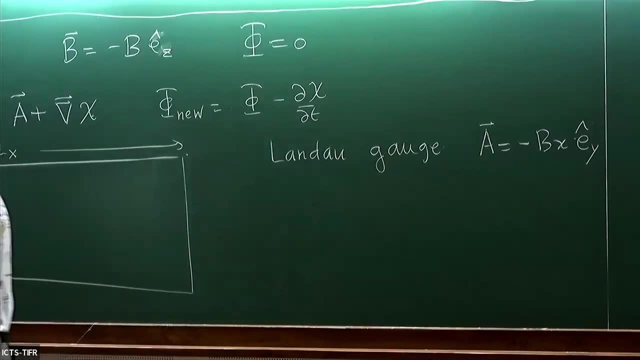 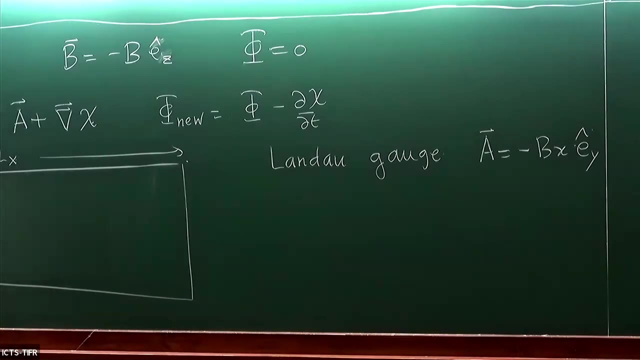 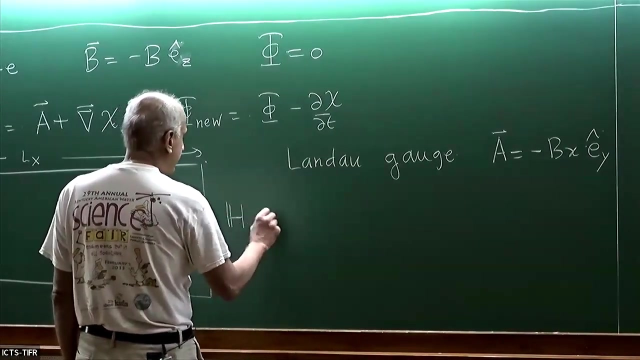 X, E, Y. okay, and you can easily convince yourself that the curl is of A is in fact this minus B in the Z direction. so that'll be my vector potential. and now let me write down my quantum Hamiltonian. okay, so my quantum Hamiltonian will look like this: so when I write an operator, I'm going to put a. 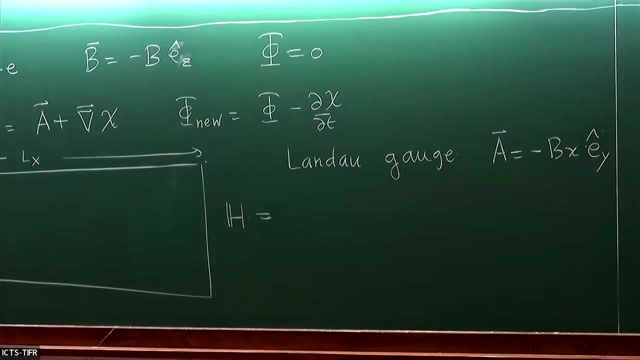 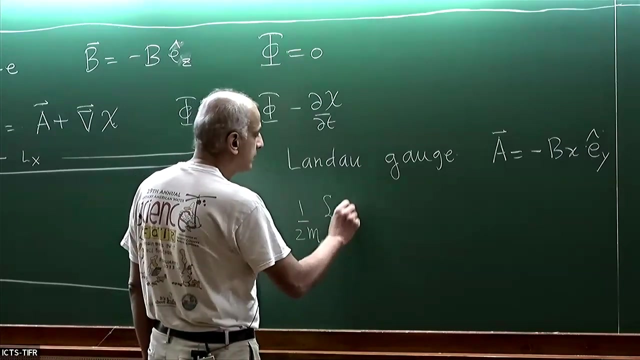 double line on one side of it to indicate that it's an operator, because often we'll have operators, we'll have eigenvalues, we'll have numbers, and to distinguish between them I'll put that double line there. so this means it's an operator, and so it will look something like 1 over 2 M. so there is a. 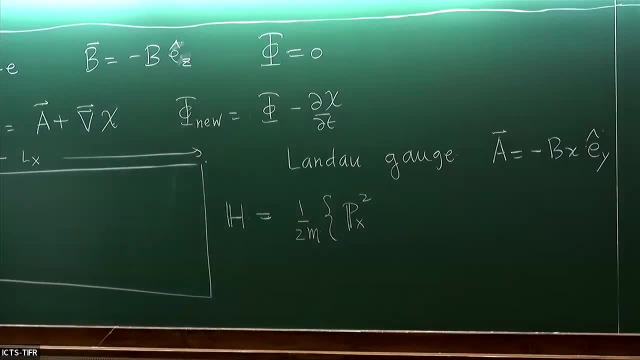 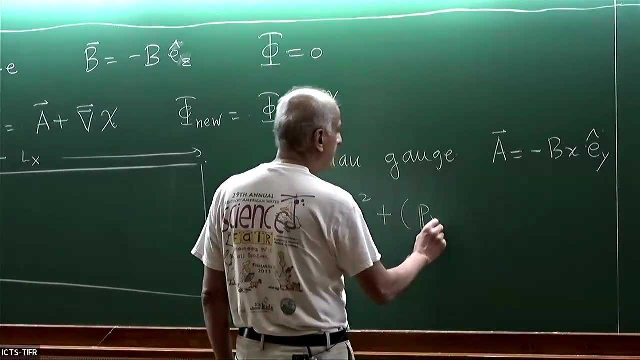 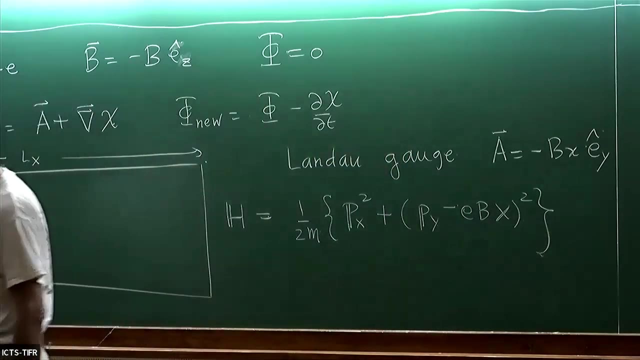 P X squared, because there's no vector potential for that right, and then there will be a E Y minus E B X. of course X is now an operator as well. that is why I chose the magnetic field to be in the Z direction, the negative Z direction, because I wanted to cancel the negative sign of. 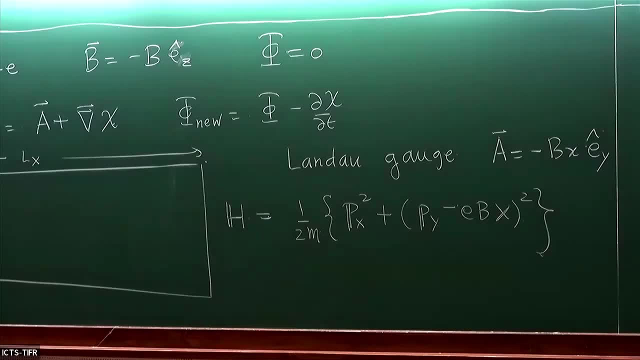 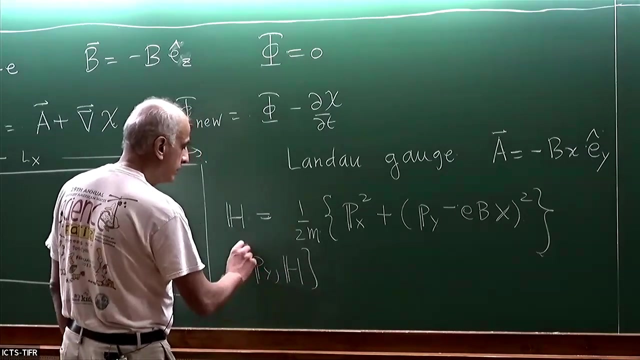 the electrons charge. so all right, so this is what I have, and now I want to diagonalize this Hamiltonian. I want to find all the eigenvalues, I want to find the eigenstates and then, and then we'll see what happens. okay, so this Hamiltonian, you can see immediately by inspection, that it commutes with P? Y. 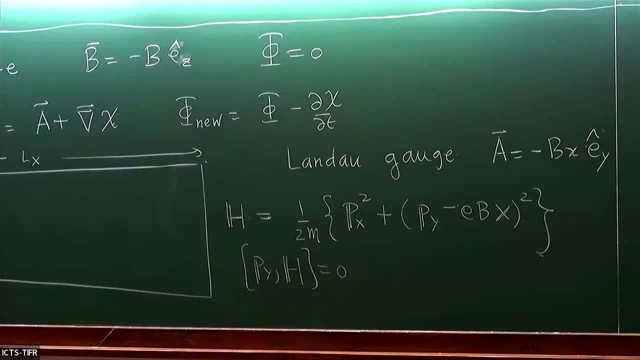 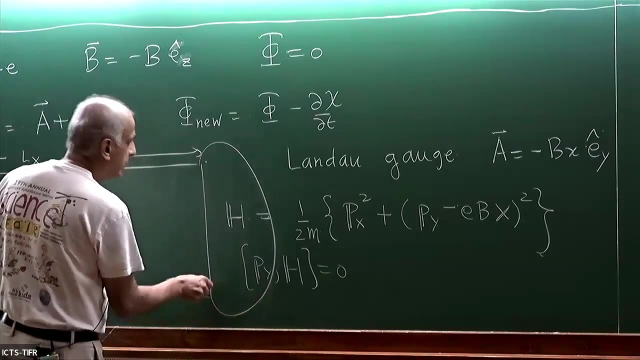 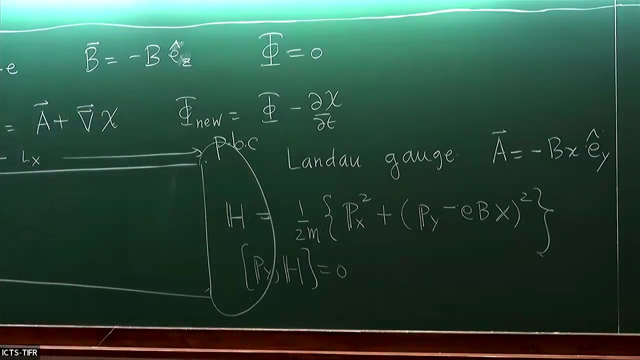 so, therefore, I can simultaneously diagonalize P Y and the Hamiltonian. in order to do that, though, I have to make sure that P Y itself is a good farm number, right. so what I do for that is, I put periodic boundary conditions, so let me say P B, C, over here. so you imagine rolling this guy up into a tube, okay, so 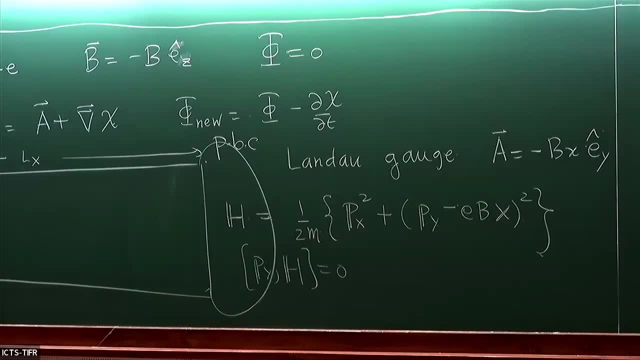 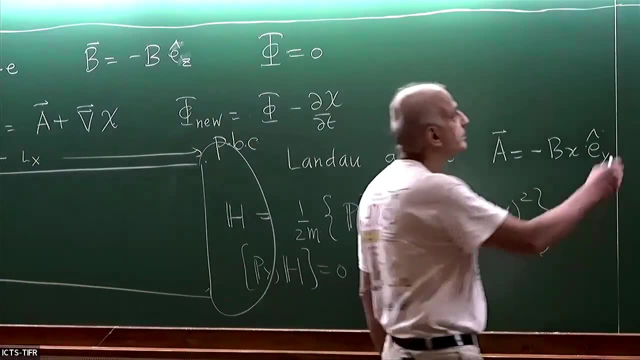 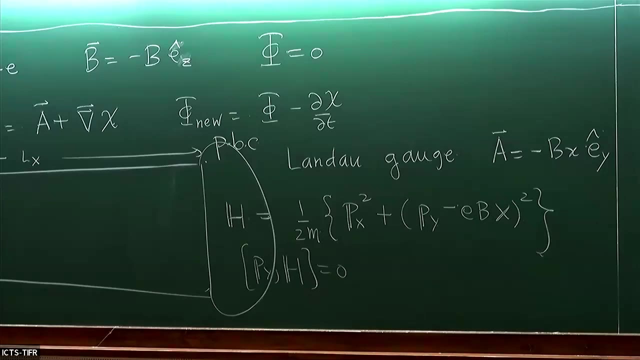 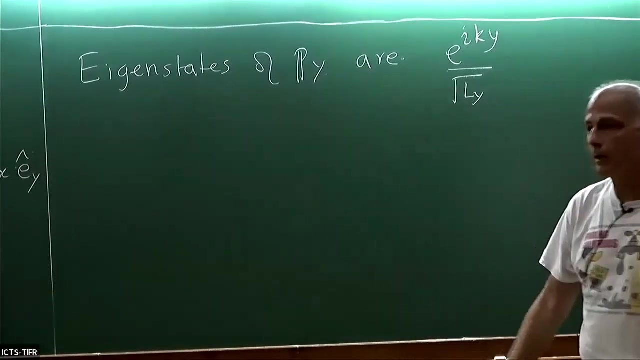 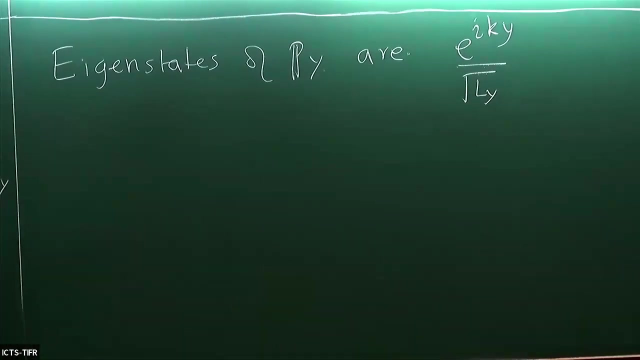 there's periodic boundary conditions in the Y direction. so P? Y is a good farm number and you have the eigenstates of P? Y are simply plane waves. I've even normalized okay. so these are the items. all right, so now I'll have to solve some differential equation, but fortunately it's a differential equation. 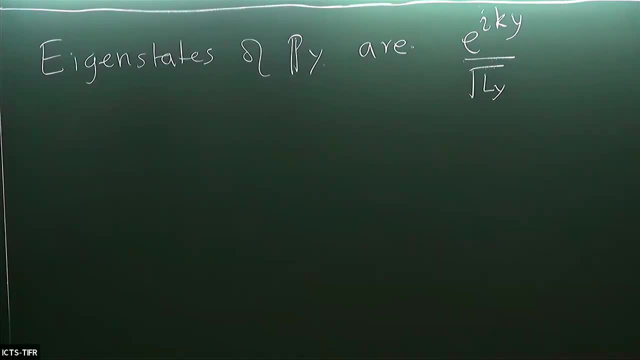 that's not going to work, but fortunately it's a differential equation that's going to work. but fortunately it's a differential equation that's going to work. I already know from from many, many years ago and suddenly I've done what that differential equation looks like now: my Hamiltonian, acting upon my psi of 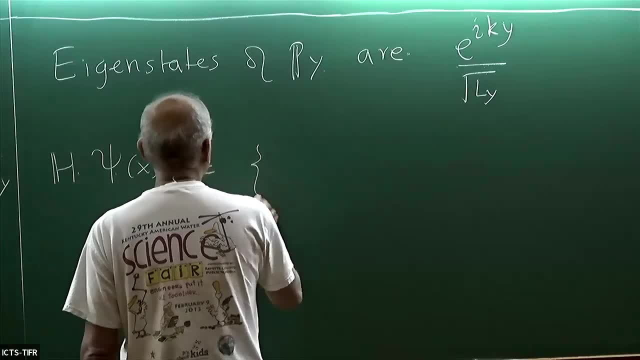 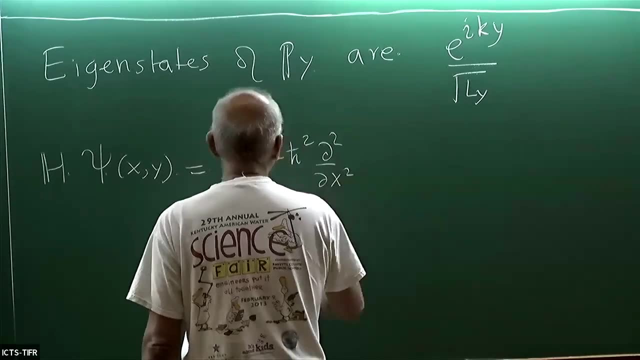 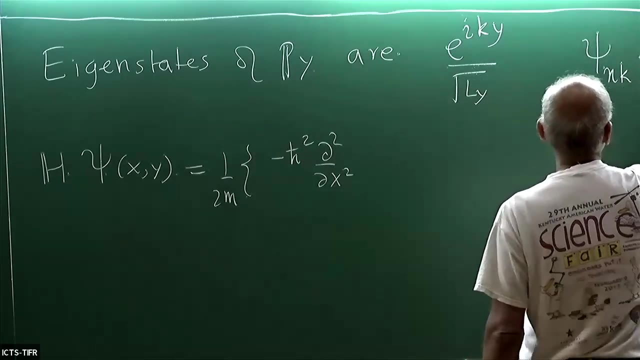 X and Y is going to look like 1 over 2 M, and there's of course a minus h bar squared B, squared DX, squared right. there's that and then. so, so let me say my psi n K is going to be equal to e, to the. 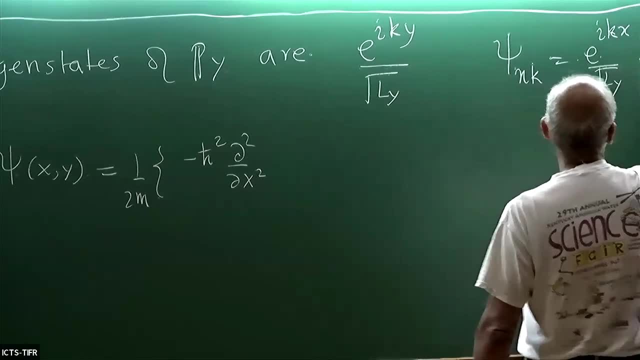 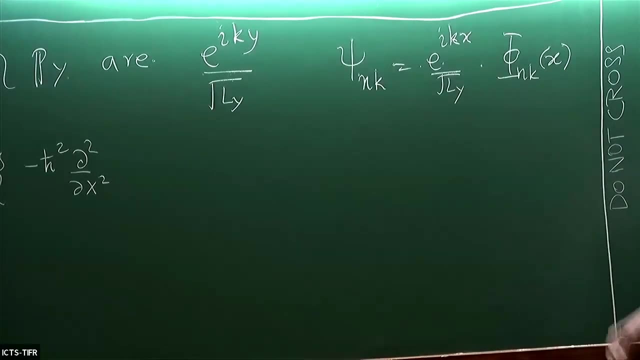 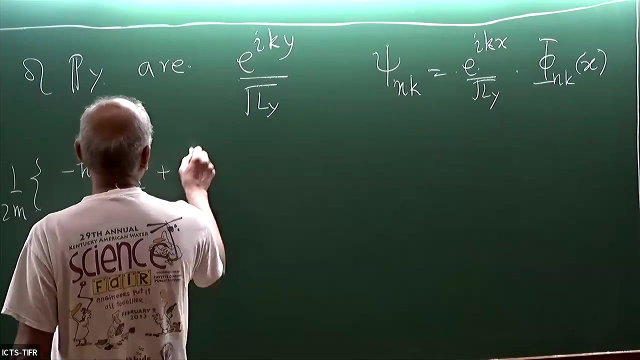 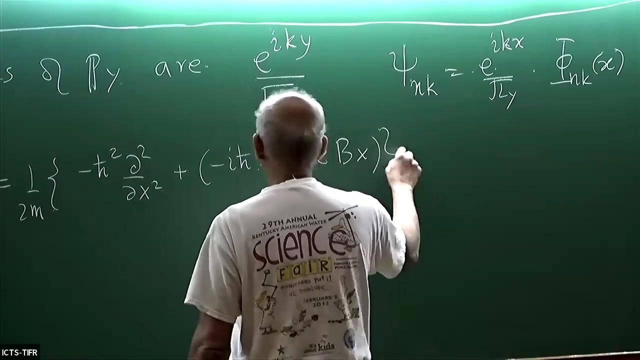 y, k, X over square root L Y time some phi n K of X alone. okay, this particular geometry, I can factorize the wave function like this, and what it looks like is: of course there's a plus, minus i h, bar d by D Y minus e, B, X acting. 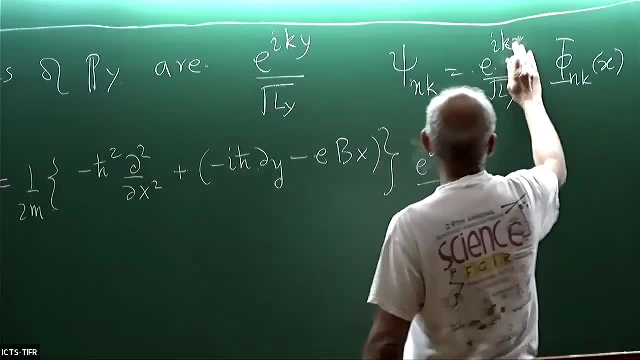 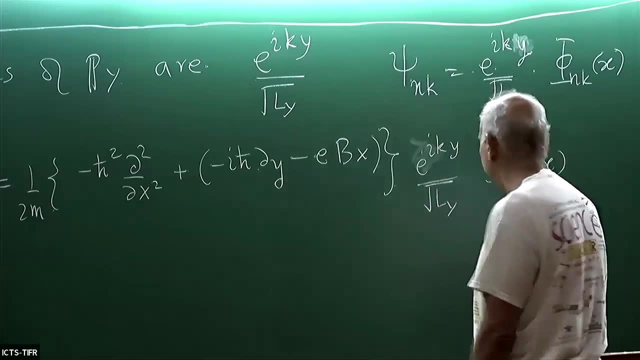 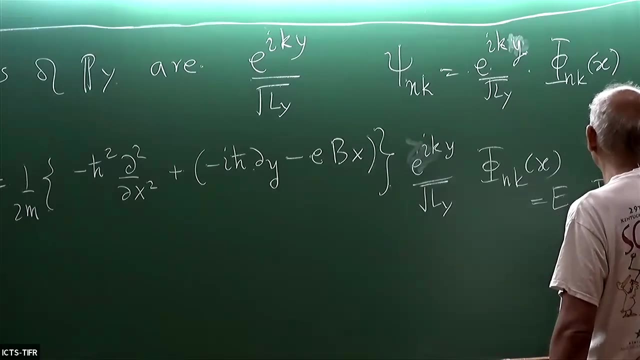 on e to the i k y. sorry, this is przykład y suffering to Genau is a y, square root of ly y and k of x. That's what it looks like and I want to solve this. I want to find all the eigenstates. I want to say: this is the equation I want to solve. 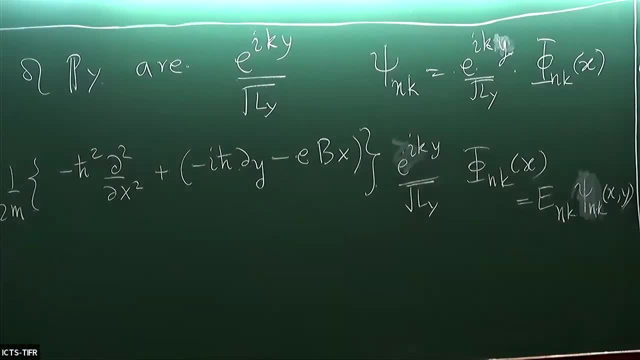 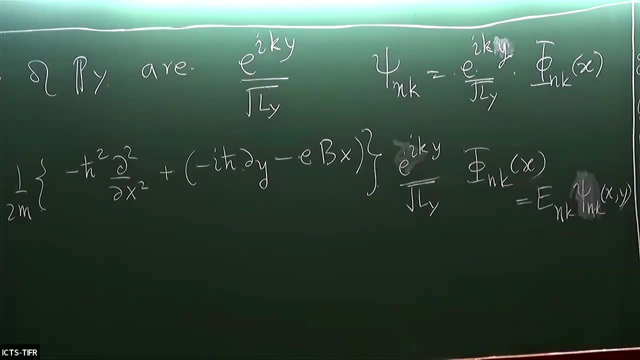 I already put in the fact that py is a good quantum number, so I plug that in. and then I got a differential equation for y of x. So I find 1 over 2m minus h, bar squared, d squared by dx squared now, because it's only acting on one variable. and then there is 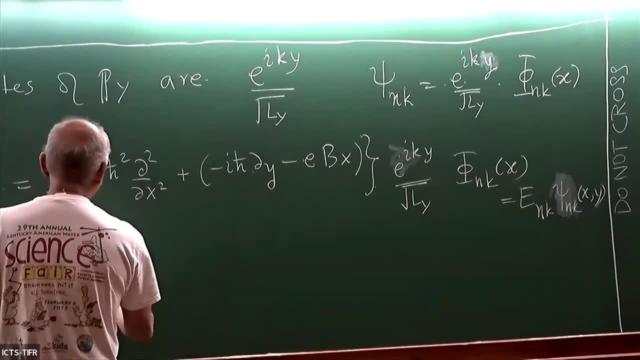 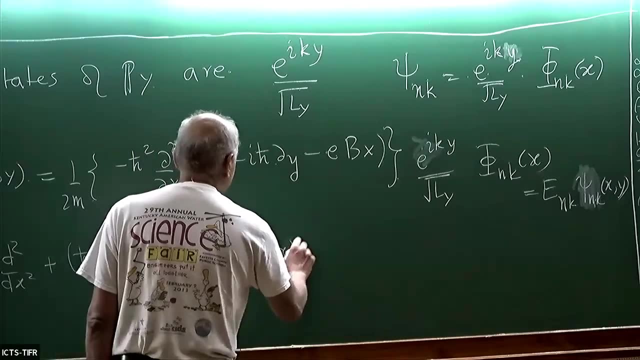 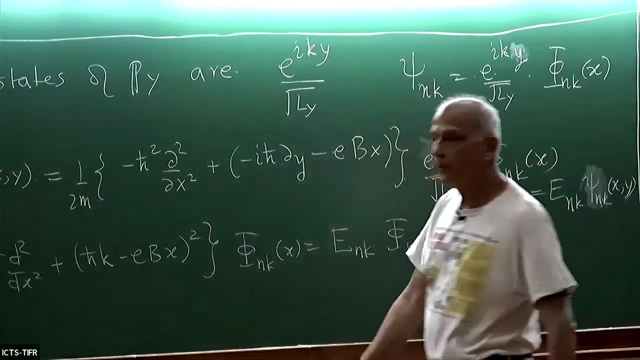 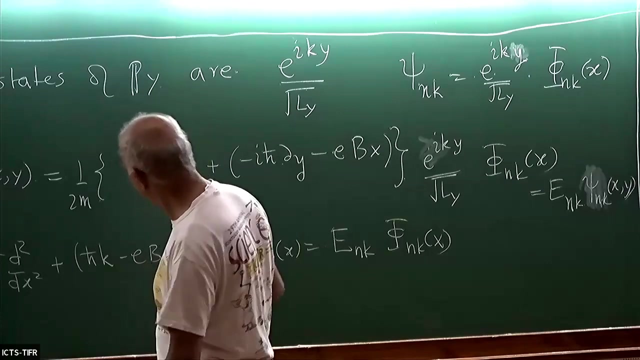 plus h bar k minus e b x. squared y n k x is e n k y n k of x. Okay, so this is the equation I want to solve. This equation is simply the harmonic oscillator in disguise, because all you have to do is you have to shift x by something. okay, and? 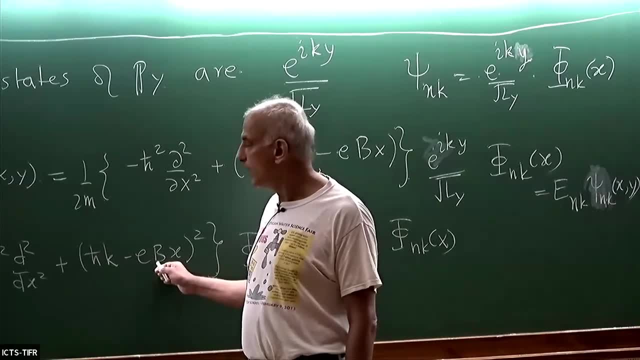 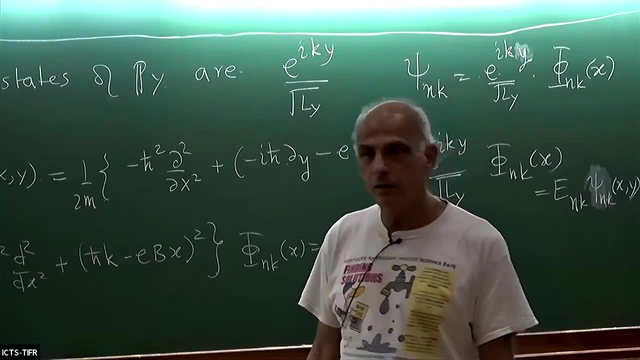 then, once you shift it, it looks like x squared and there is a d squared by dx squared and there's an x squared. That's simply the harmonic oscillator. Okay, that's all it is. So, in order to do that shifting, let me go over there. 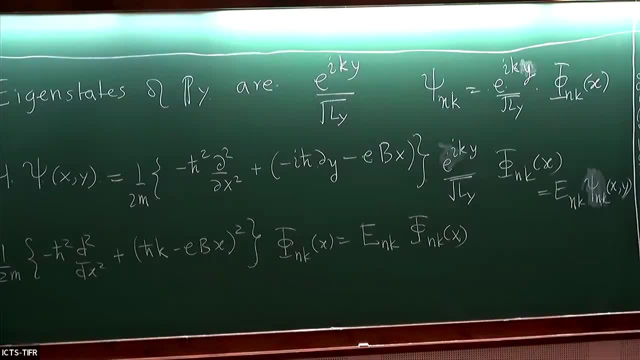 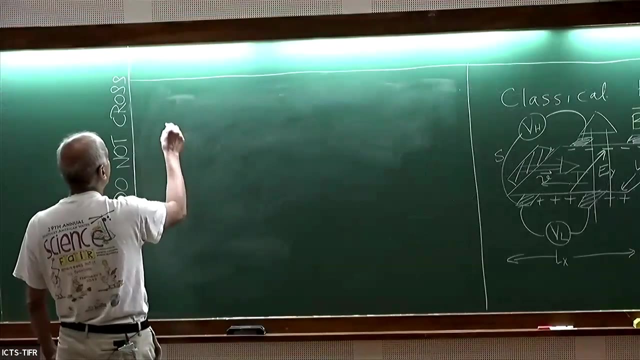 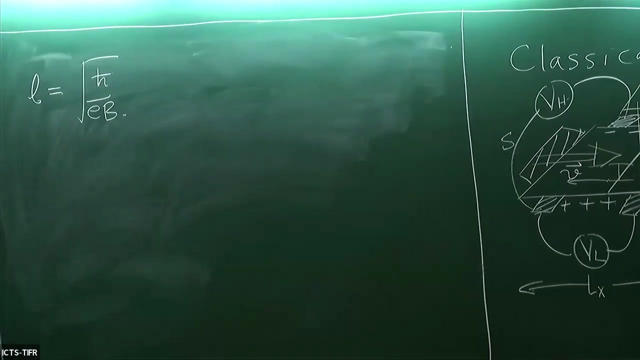 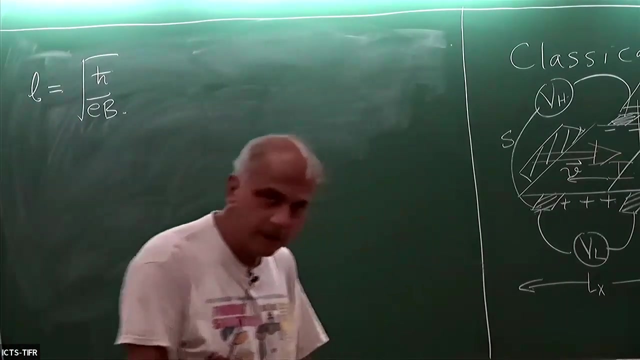 Let me go over here and define something known as the magnetic length. This is a very important length scale Whenever you have an orbital magnetic field. okay, this defines for you the length scale over which you get one flux quantity. Okay, so there are many ways of thinking about. 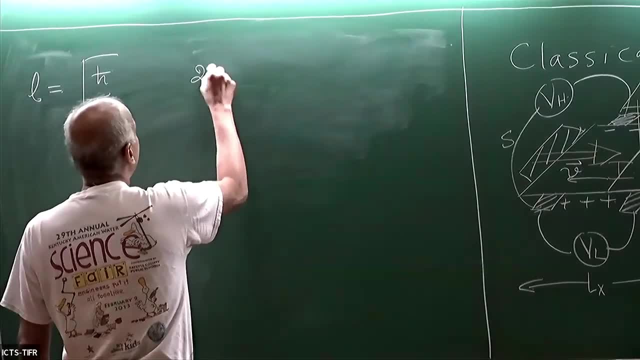 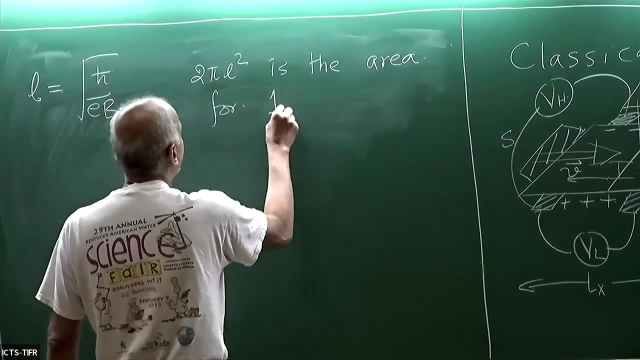 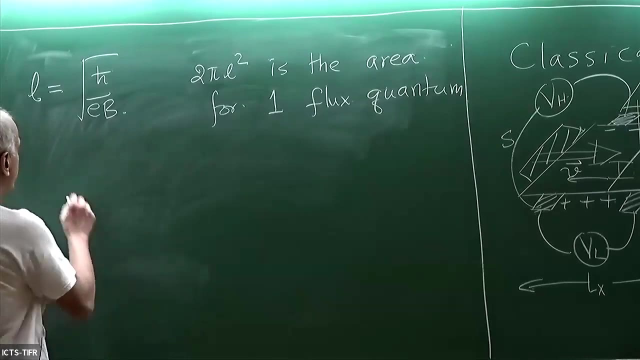 this. okay, but one way to think about it is that 2 pi l squared is the area for one flux quantum. Okay, what is one flux quantum? A flux quantum is phi naught. is h over e in mks units. Okay, what is this guy here? Anybody know what a flux quantum is Up there in the back? 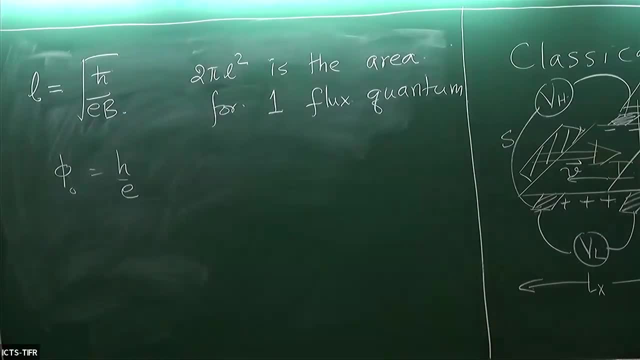 benches, Okay. a superconducting ring would have half of that flux, Okay. but why? Why is this called the flux quantum? Is flux quantized No only in a superconductor, it's quantized In general. it's not quantized right? So why is this called a flux quantum? This was. 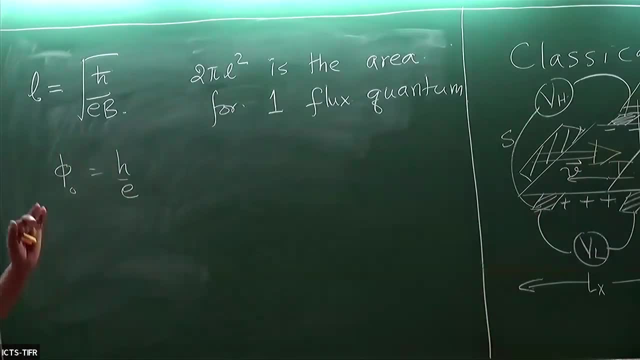 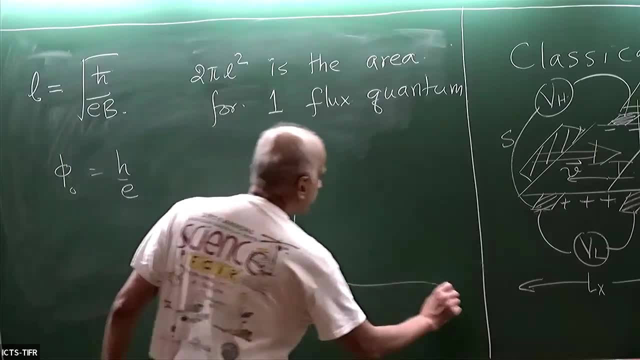 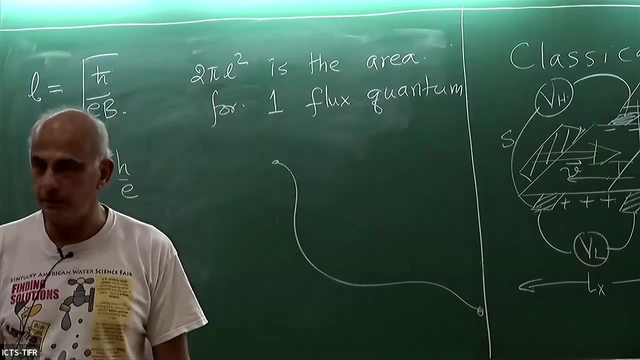 and he said: if there's a monopole here, then I have some string and then there's an anti-monopole somewhere else. but in order to really be a monopole, I should not be able to detect this string. When can I not detect a string? Well, supposedly I make a loop around this. 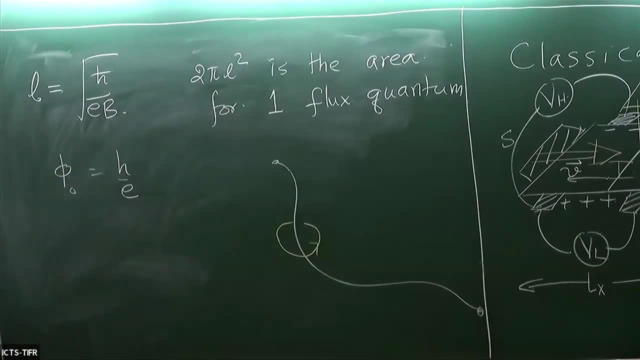 thing. I take an electron in a loop around it and I ask: how much phase does the electron accumulate? There's an Aharonov-Bohm phase which is Ie over h-bar, the integral of A dot dl. You guys know about this. How many people have seen this before? How many? 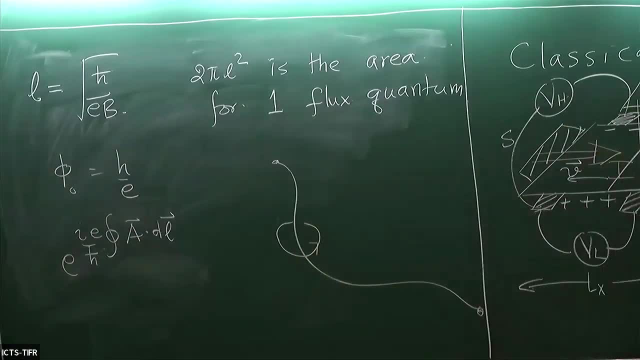 people have never seen this before The Aharonov-Bohm phase. Okay, you've seen it now. Okay, so I'm going to do the same thing. So, whenever you take an electron around some magnetic flux, this is the amount of flux that it accumulates. Okay, so Derac said: all right, if I should. 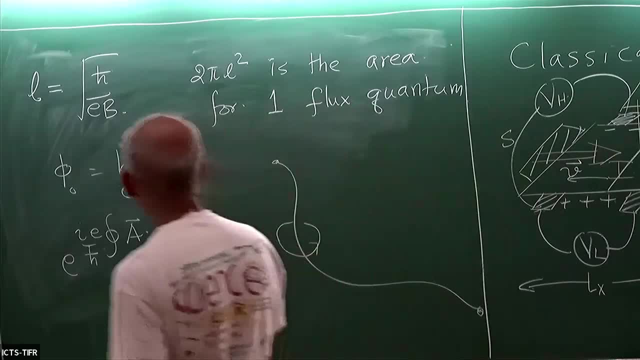 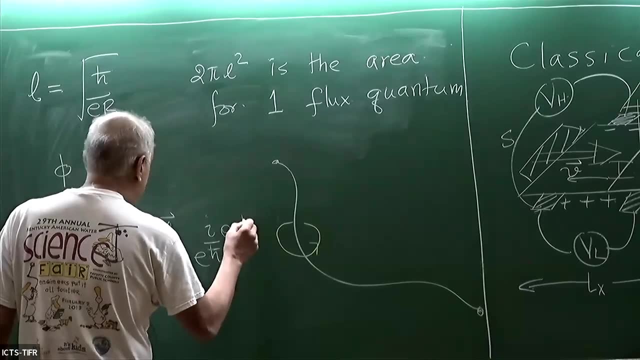 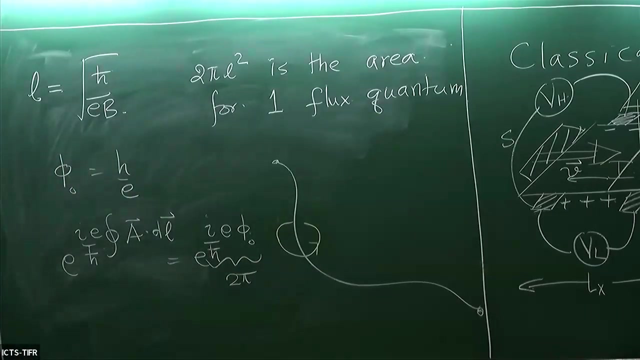 not be able to detect this solenoid, then this should be e to the i, h-bar e. This is this flux, This is the flux quantum that I'm talking about. Should be this: this number should be two pi. Okay, because e to the i, two pi is one, and 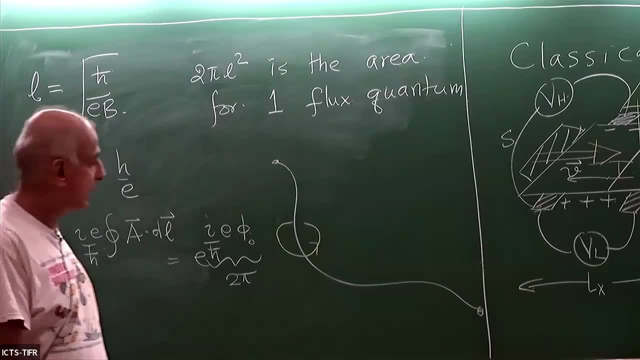 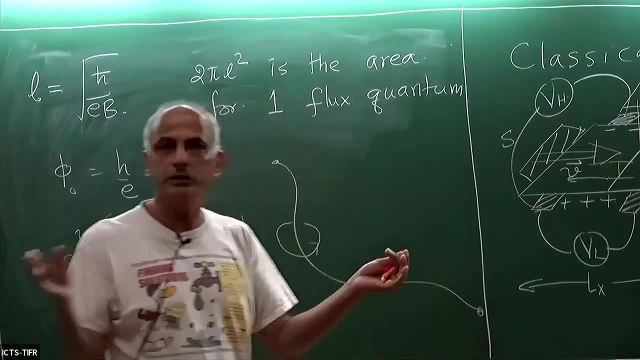 doesn't know whether it's there or not. Okay, and then it appears as though this monopole and the ankyl monopole are completely separate objects, because nobody can tell that there's this thin solenoid. This is not the way we think about. 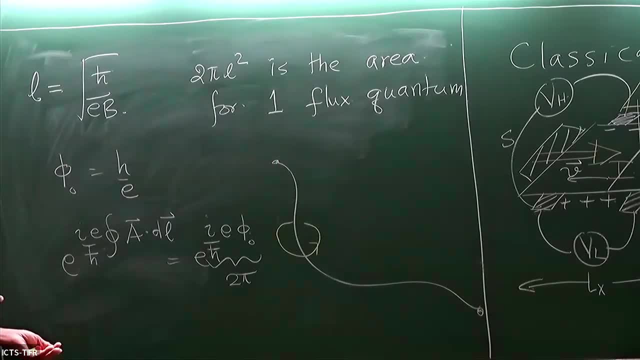 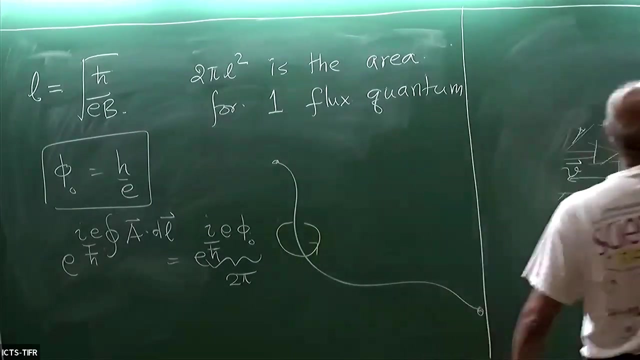 monopoles nowadays. but this is the way Dirac thought about in those days. Okay, so that's where this flux quantum comes from. Okay, so now, so that 2 pi L squared is the area which encloses one flux quantum. and now let's put that in there. 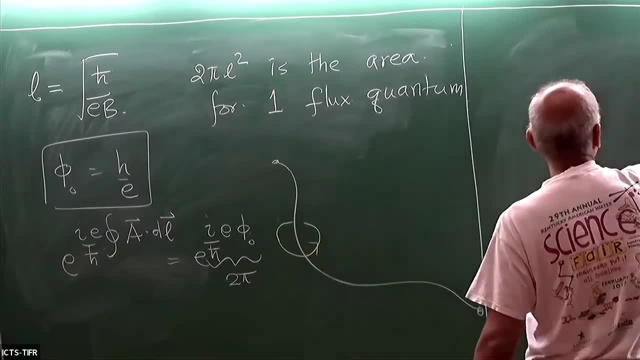 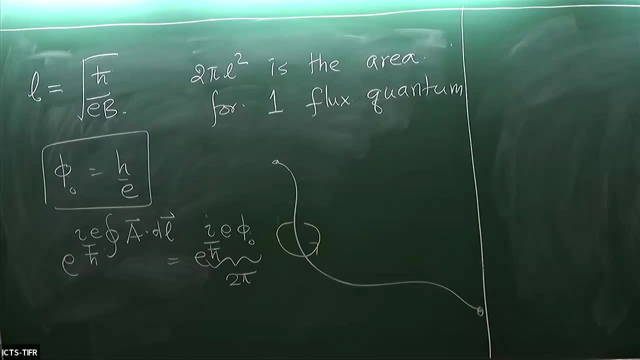 this length, scale L, and what we're going to do is de-dimensionalize everything. Okay, and now I can go through it. So anytime people think that I'm going too fast, please tell me. Okay, and I will slow down and I'll explain the steps to you. 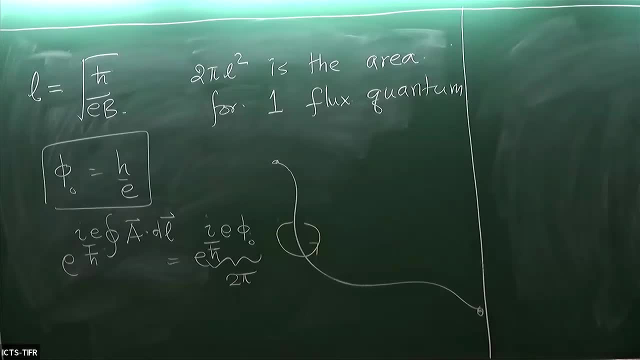 But really think about it, Think about it. Think of this as each of these little steps. If I skip over a little step, think of it as your homework. Okay, and just try to fill in all the steps. So I'm. 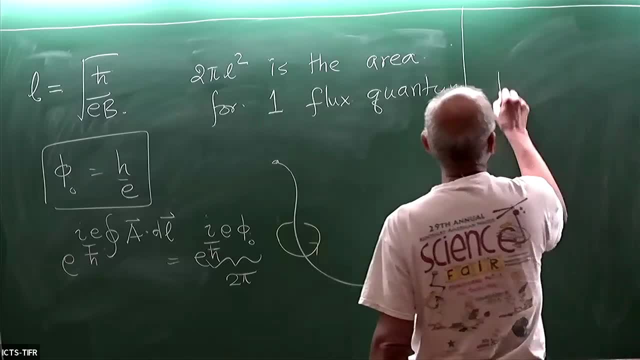 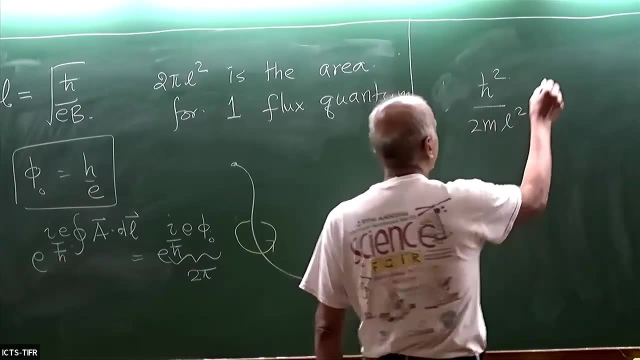 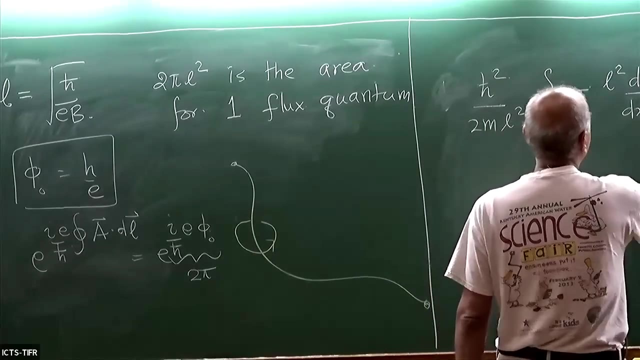 going to write down the Hamiltonian now and it's going to look like this. So it's going to look like h bar squared over 2 m L squared. Okay, it's going to look like minus L squared d squared by dx squared plus 1 over L squared. 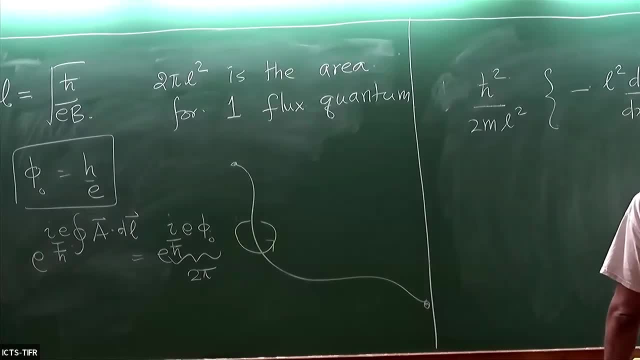 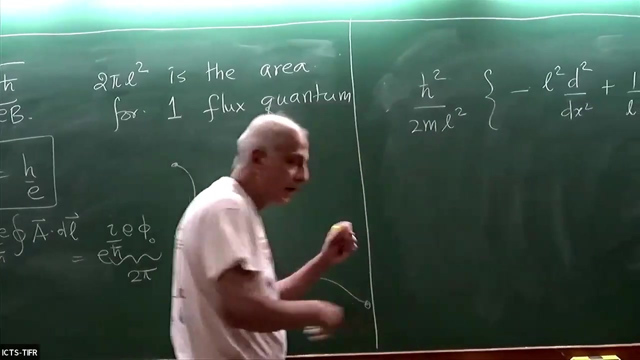 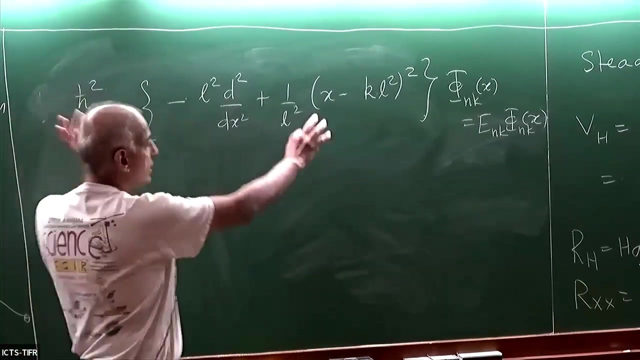 x minus k L, squared, squared, Okay, and that on pi n k of x is e n k, pi n k of x. So I've sort of factored things out, I've put things back, something, something, Okay, but really this thing is now dimensionless. Okay, the operator sitting inside the curly braces is dimensionless. 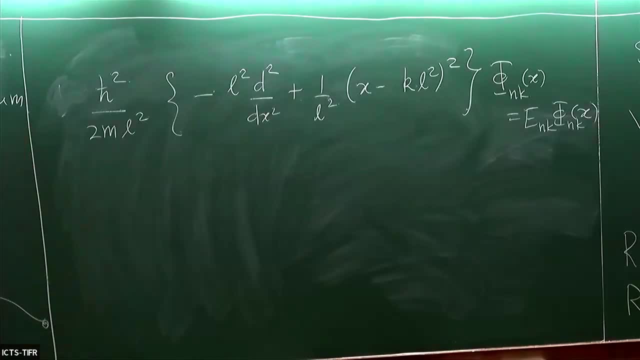 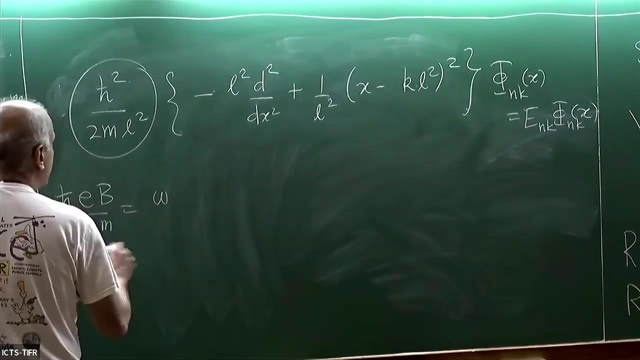 Just go home and verify that this is all correct. So this guy here, if I put in this L squared, is, you know, h bar over e b. this one looks like e b over 2 m, which is simply the cyclotron frequency. h bar times the cyclotron frequency divided by g. 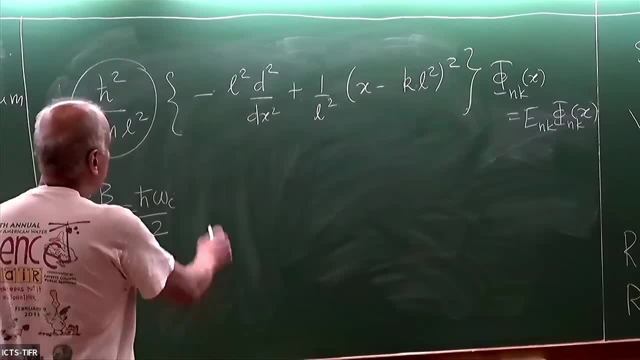 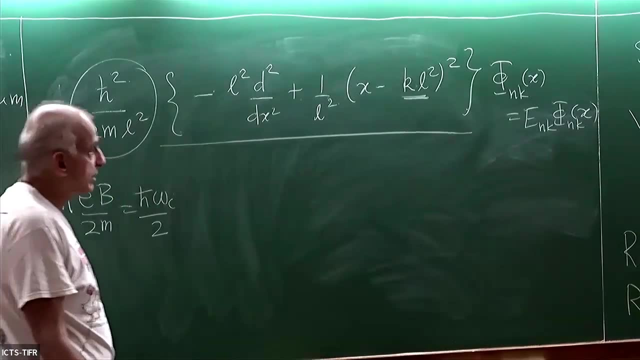 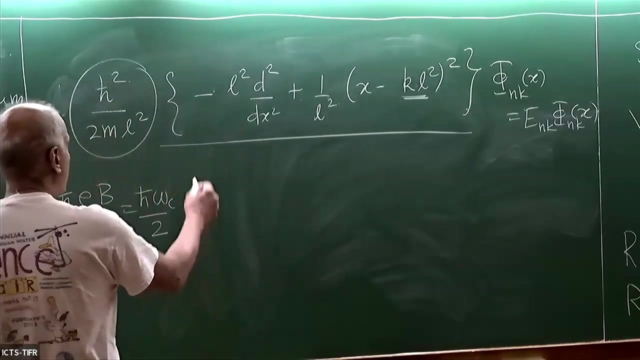 That's what it looks like. And now this is simply the harmonic oscillator shifted to this origin, And the energy, of course, doesn't depend on the choice of origin, And so, therefore, the energy will only depend upon n. The eigenvalues of this are simply n plus a half right. 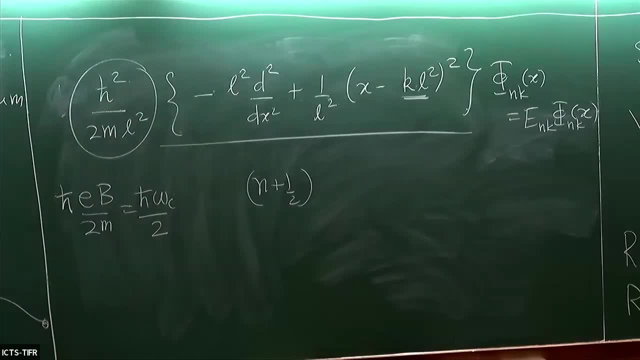 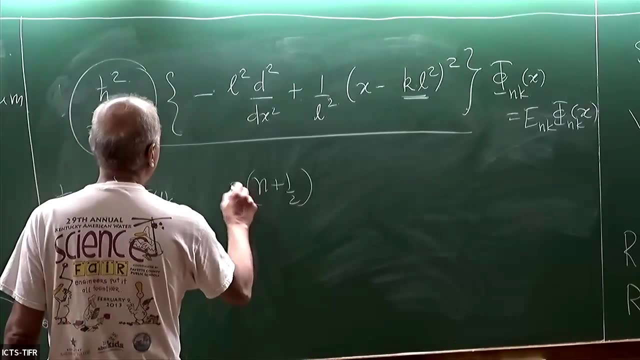 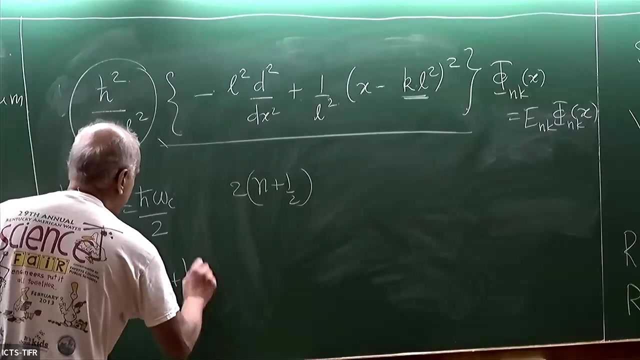 This particular operator here in the curly braces. eigenvalues are n plus a half And so this is: I guess it's 2 n plus 1 here, because there's a half sitting outside. So you get e n. k is n plus 1 half h bar omega c. 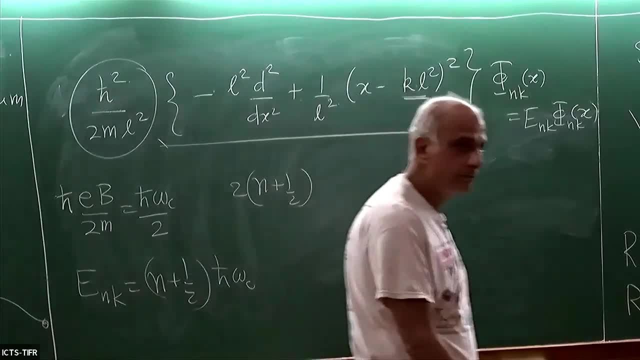 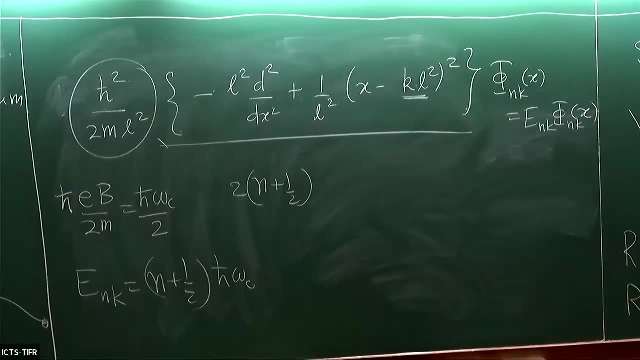 Okay, it's independent of k. All right Questions. What conditions do we have on k? Very good, So if I want my, my boundary conditions to be to be periodic, okay, so let me do the simplest thing And let me say that I'm going to impose. 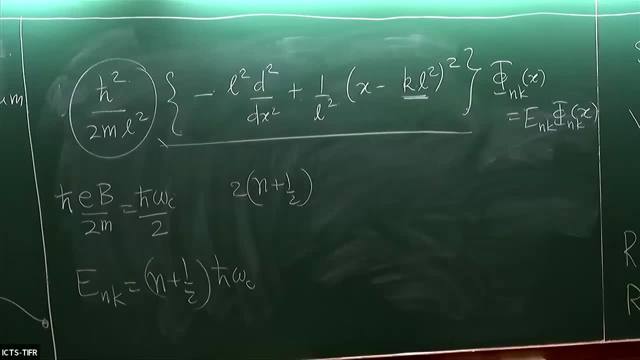 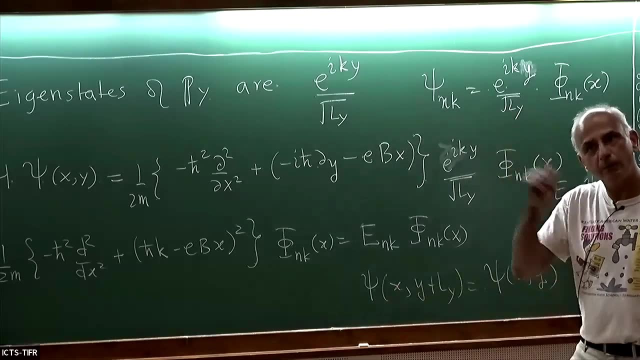 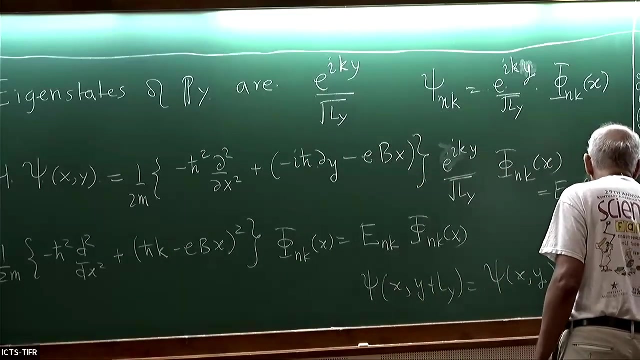 psi of x, y plus l y is psi of x and y. Okay, Suppose I impose periodic boundary conditions, Then the value of k is going to be given by 2 pi j over l? y, And we're going to come to that in a minute. 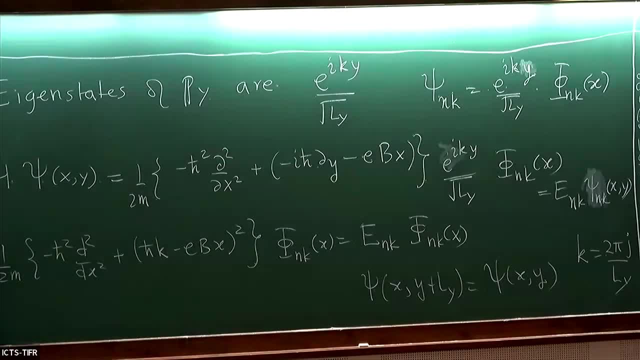 Sorry, There is no boundary condition in the expression. I'm not specifying anything. Yes and no, You'll see. Okay, I mean I can. I can actually put some some hard wall boundary condition. I'd rather not. I will in a few minutes when I talk about edges. 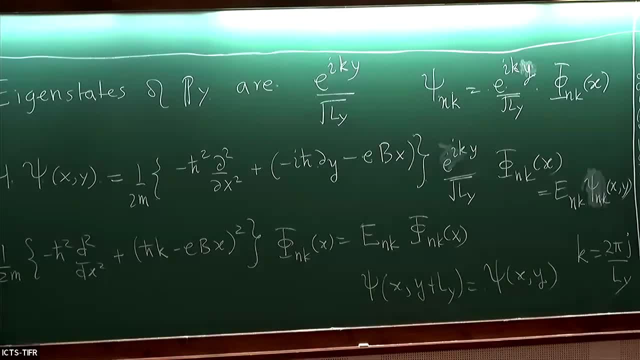 But at the moment I'm talking about the bulk, So I would rather not specify what happens On in the extraction. I will soon, Okay, Hmm, Then there will be something shortly, Okay, All right, Just wait for it. Other questions: 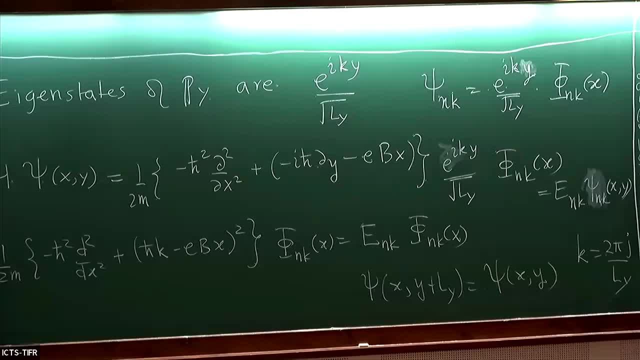 Yeah, Very good. Okay, That's another very good question. So So, as usual, what we theorists do is: we try to solve problems we can solve right, So we solve this. and then we say, okay, what do interactions do to this? And now, you're asking what is the strength of the interactions compared to something else, right? That's really what you're asking. Now, that depends a lot on what is the density of electrons compared to the magnetic field. So that's how I'm not. 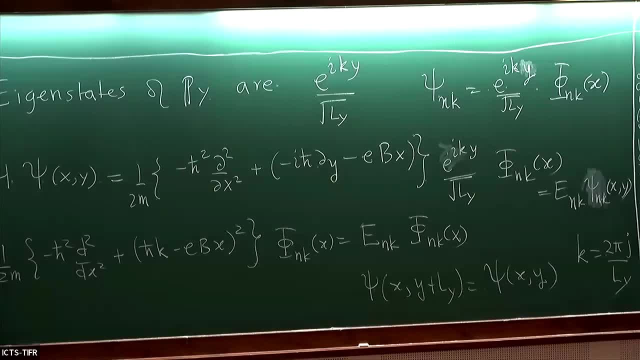 getting into it right now. okay, If you have the right amount of density, such that an integer number of these Landau levels- these guys, by the way, are called Landau levels- okay, So this n starts from 0,, 1,, 2, and so on, and these are the. 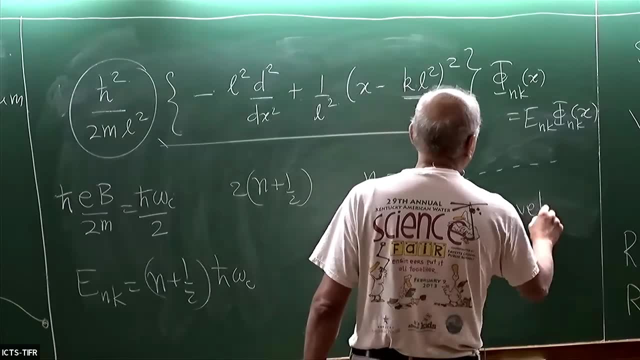 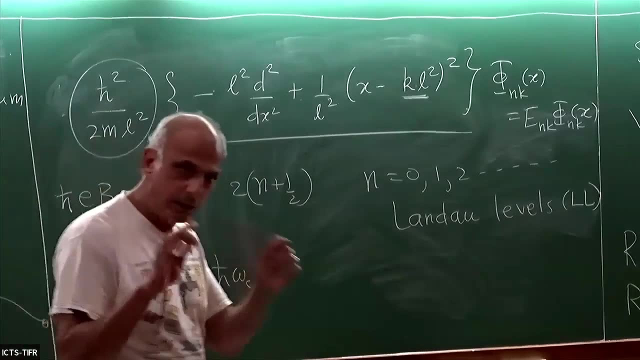 Landau levels. I'm also going to call them simply LLs. okay, If you have the right density to fill up exactly an integer number of these Landau levels, then the interactions are going to be the same. So if you have the right density to fill up exactly an integer number of these Landau levels, then the interaction 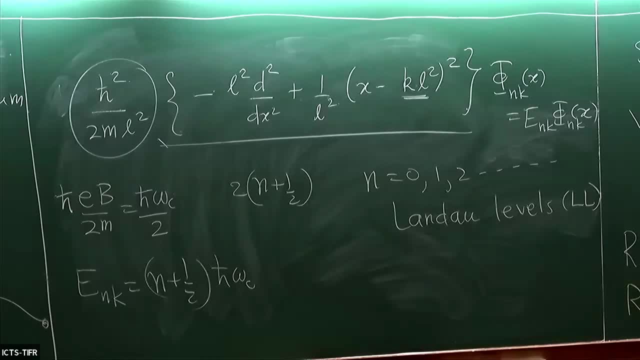 are not that important If it's not the right number to fill up an integer number. if you have a fractional number, then they're extremely important. They're more important than anything else. It's related to the filling. actually. We'll come to that, okay. So, yeah, these are all very good questions. 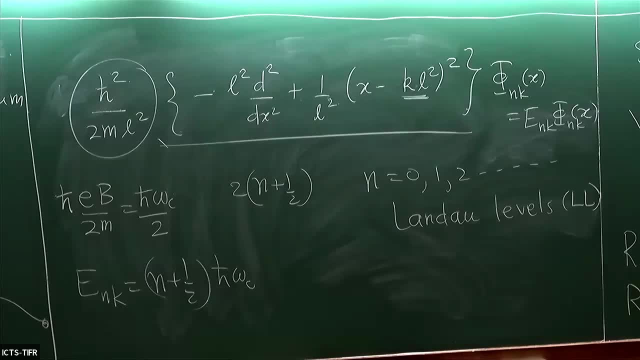 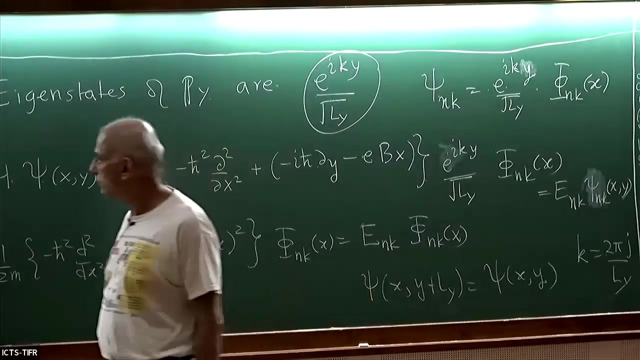 They're anticipating something that will happen shortly. okay, Maybe not in this lecture, but in the next Other questions. Yeah, Yeah, Yeah, Because we already know the eigenstate in the Y direction. Very good, So the question was the first equation with: 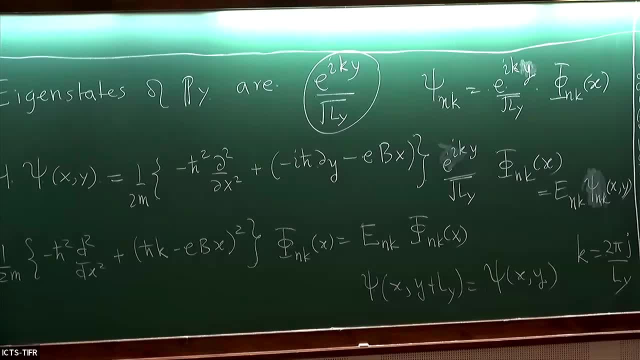 this H with the double symbol, double line, was in two dimensions, but suddenly it became one-dimensional equation. That's because I factorized it. This is what is, I think, mathematically called the separation of variables, or something. 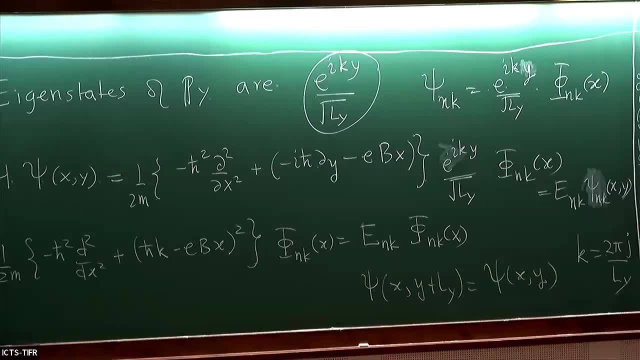 In this geometry I can separate out the Y component of the wave function from the X component. With the degeneracy, it will, it will, it will shortly. So this geometry is very nice because you can do everything okay analytically. 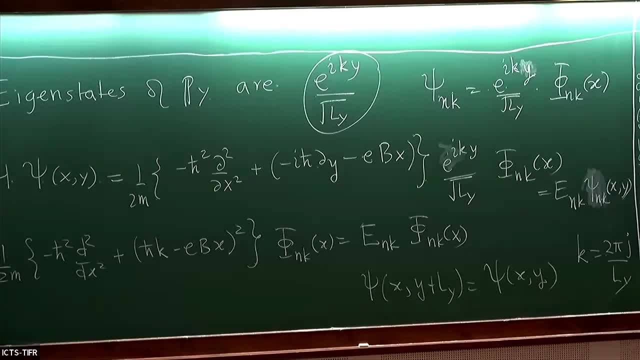 Other questions? Okay, so let's carry on. So now these guys don't depend upon K. all right, So there is a lot of degeneracy. So how much is the degeneracy? Well, let's compute it. 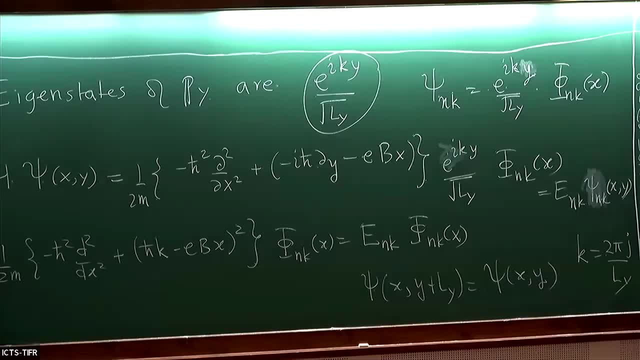 Again, this geometry is very nice for computing what the degeneracy of the of each Landau level is, And to do that, I'm gonna write it as a tube. I'm now gonna explicitly draw a tube and I'm gonna draw some. 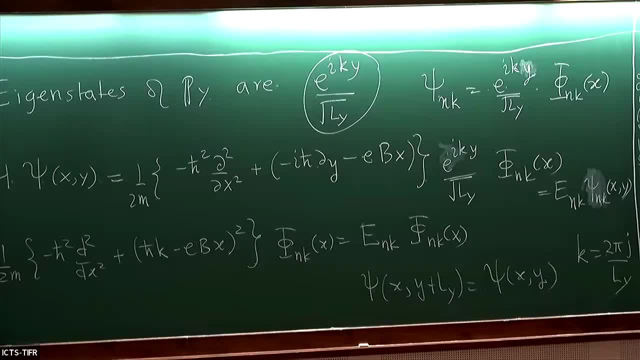 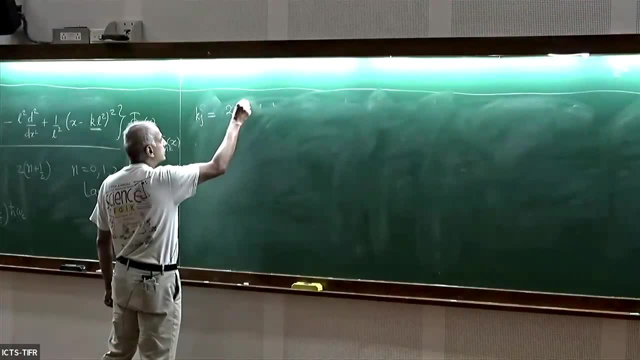 let me, let me gather some key facts. So we know from the bottom of that very last rightmost panel that K is quantized because of periodic boundary conditions in the Y direction. okay, This, this putting a finite length, actually helps me count. 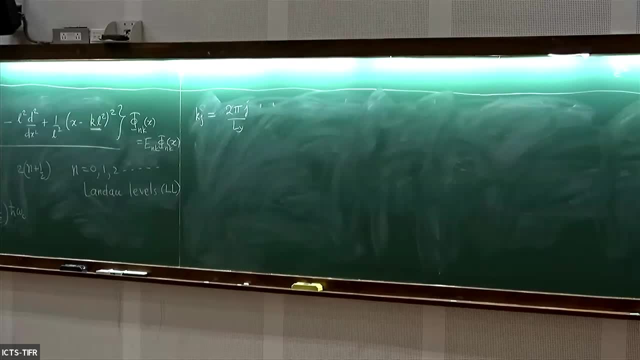 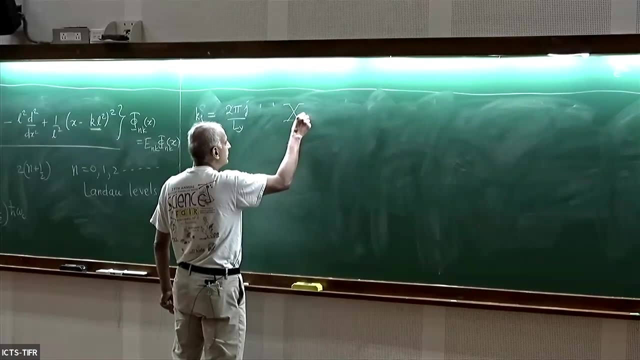 This, this putting a finite length actually helps me count. This, this putting a finite length actually helps me count, Because everything becomes finite. So that is, those are the values of K. For every value of K, there is something that I can call X sub K. 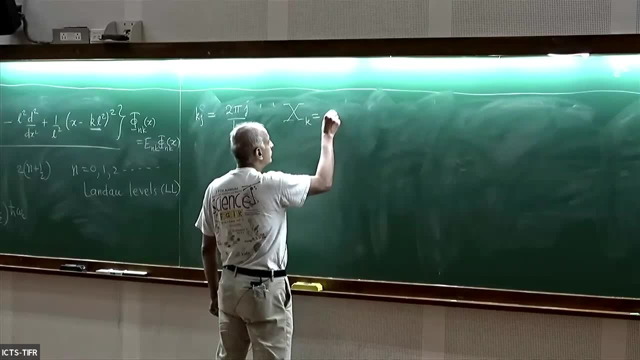 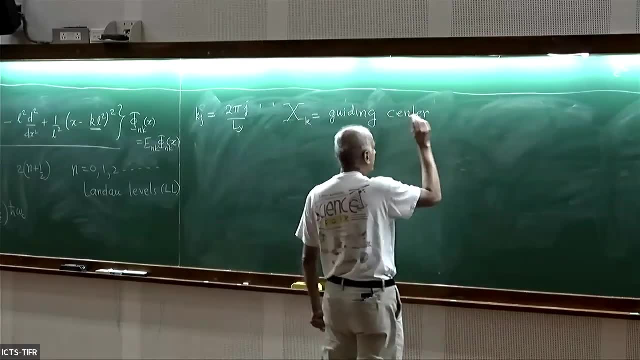 which is called the guiding center- okay, This is a word that you will you will hear again- Guiding center of that particular orbit, And this is simply K sub J, L squared. okay, So this is the center around which? okay. 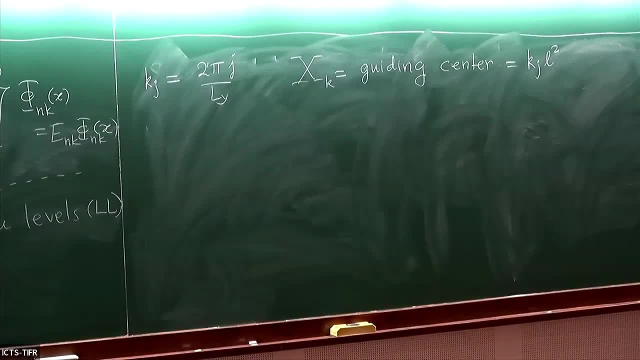 So this is the center around which? okay, This is the center around which. okay, this harmonic potential is being felt by the electron. okay, this harmonic potential is being felt by the electron. okay, So an electron with a wave number in the Y direction of K. 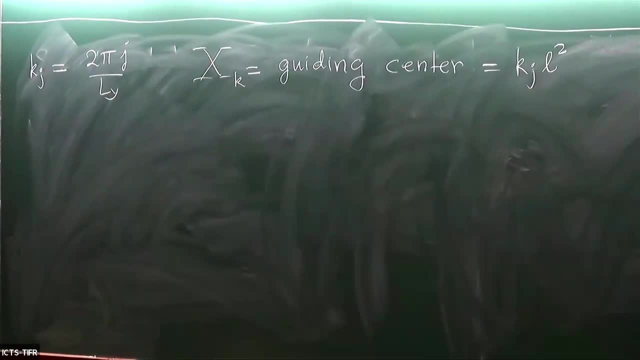 So an electron with a wave number in the Y direction of K will feel that it's confined to a region around capital X sub K. Okay, that's what it feels like to the electron. Okay. so now I'm gonna draw this tube. 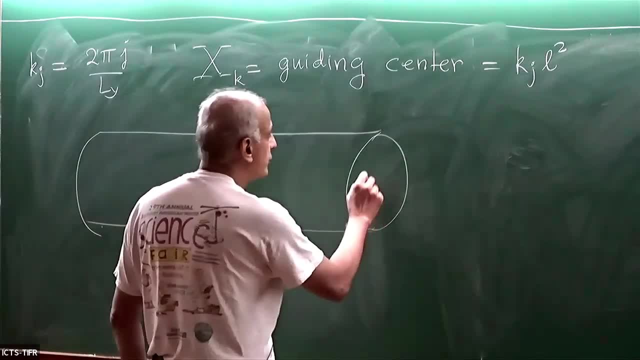 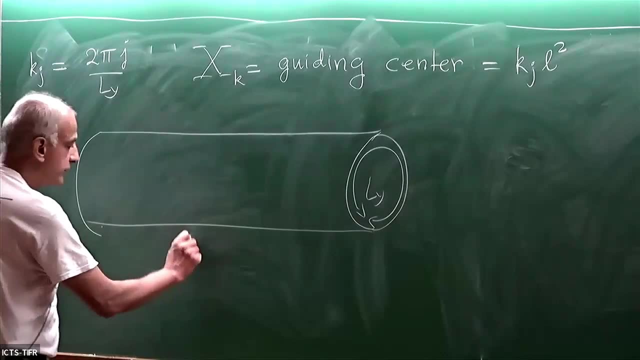 So here's my tube, right, The circumference of this tube is L Y, The circumference of this tube is L Y and the length of this tube is Lx. So I'm going to draw these lines here. okay, These x sub k's. 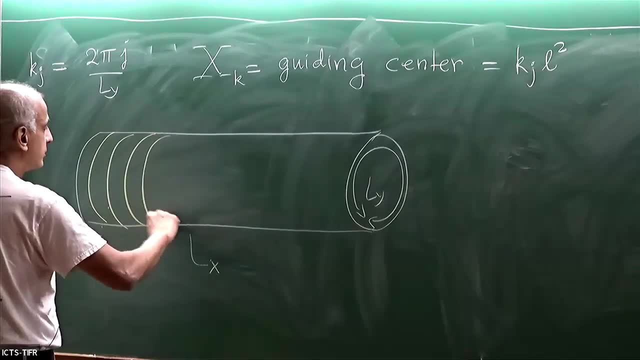 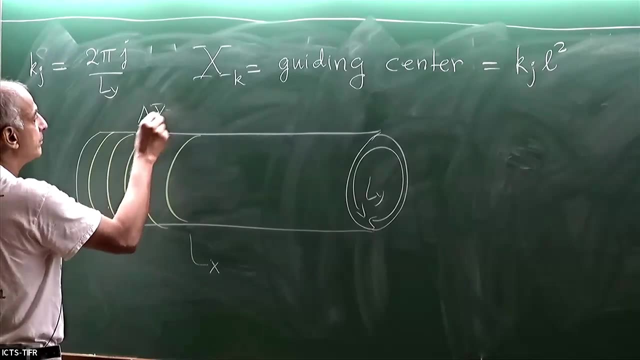 So there's some lines like this: okay, And so on and so on. What is the separation of two of these lines? The separation is simply between k sub j and k sub j plus 1, right, And their separation is 2 pi over Ly. So the smallest separation is simply 2 pi L squared over Ly between two. 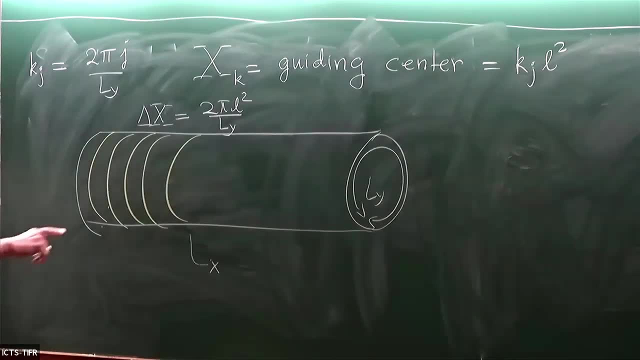 successive orbits. When I draw this line here, I don't intend to say that it's completely localized on this line. It spreads out, okay, around this line, but its greatest, you know, density is around that line. Of course it depends on the density. It depends on the density It depends on. 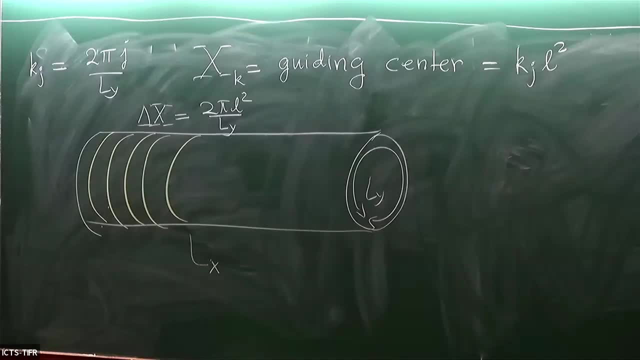 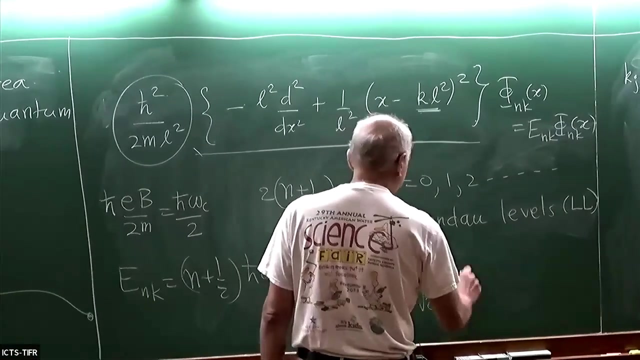 which Landau level you're talking about. I can also write down the wave function, So let me write down these wave functions here as well. So there's a phi and k that looks something like you know, 1 over some stuff. okay, Some stuff here, some stuff there and some more stuff here. 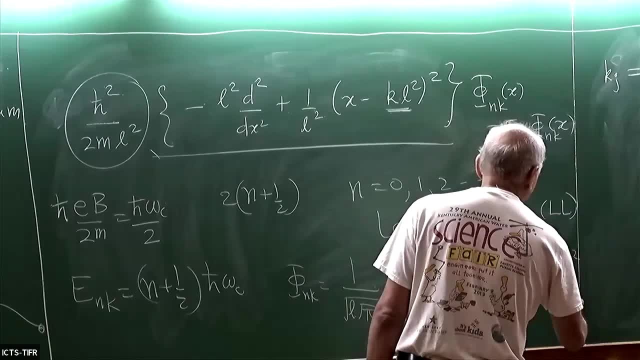 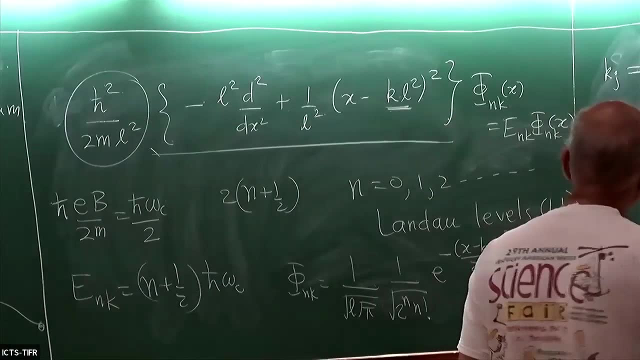 Okay, these are the Hermite polynomials that you know about from your harmonic oscillator solution. okay, So that's what the wave function looks like, but it doesn't matter, okay, The important thing is that it's spread out, you know, around the 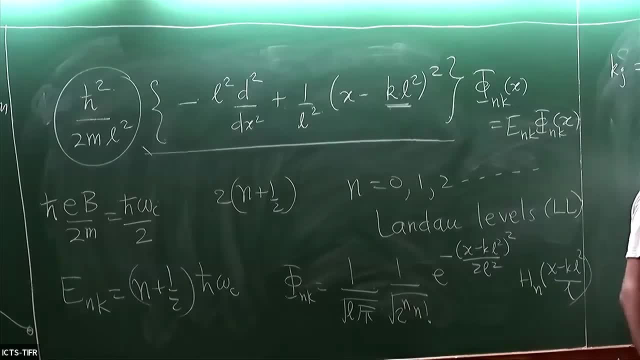 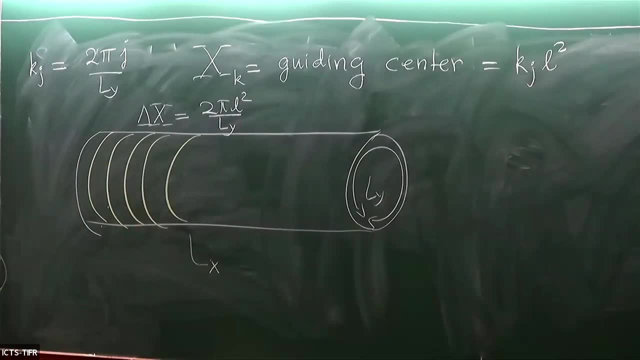 center, which is this x sub j. okay, All right, But each of these guiding centers marks the location of a particular orbit. okay, So now I ask myself: how many states are there? Now I say okay if I take some of these states. how many states are there? Now I say okay, if I take. 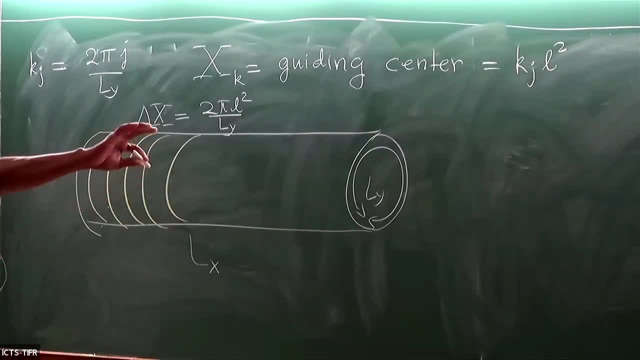 some of these states. how many states are there? Now I say okay, if I take some of these states length Lx. So now I'm assuming that this is continuing okay, beyond my Lx and this continues in the same old cube. I'm asking myself: how many states are there in this range of Lx And the 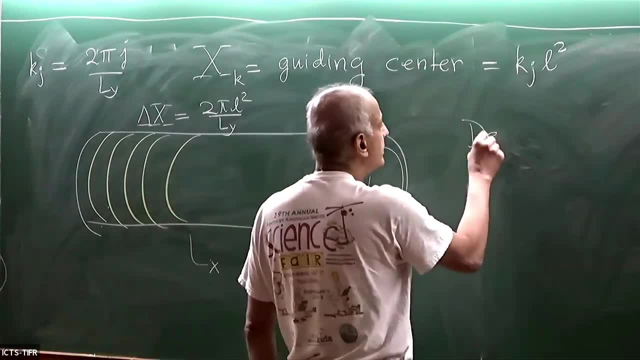 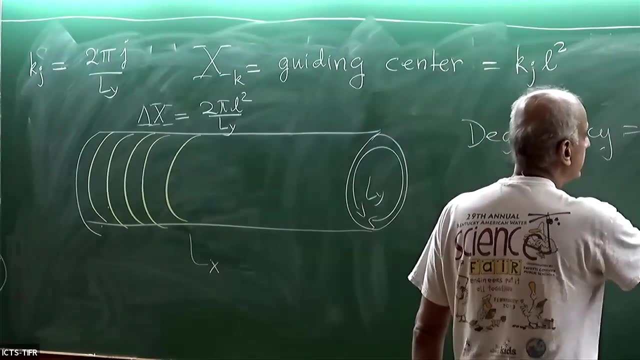 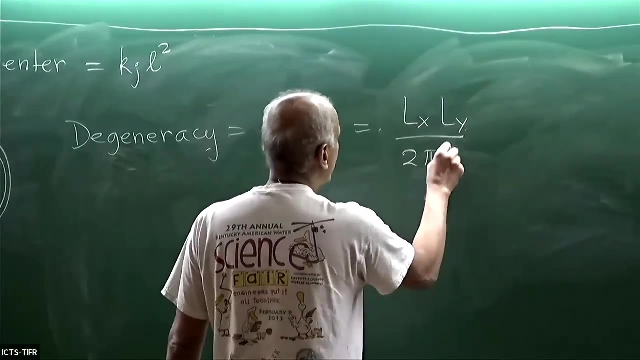 number of states will simply be so. this is the degeneracy. is Lx divided by delta x right, And that is simply Lx, Ly, And that is simply Lx over 2 pi L squared? I already told you that 2 pi L squared is the area. 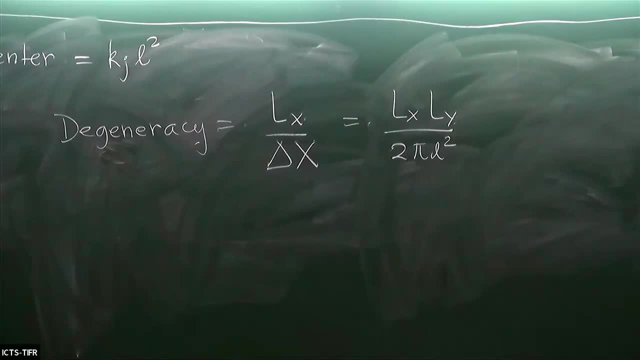 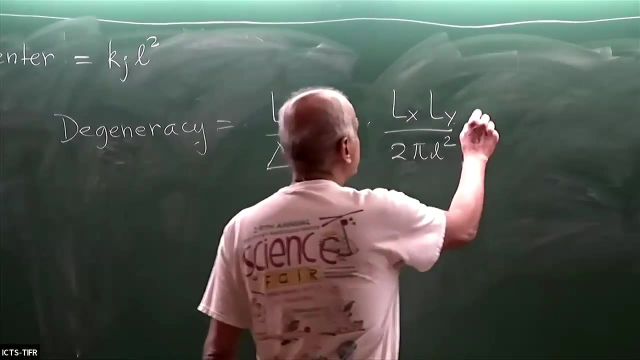 that it takes to have one flux quantum at the particular field that we're talking about, B. okay, So this, you can think about it as the number of flux quanta that go through the sample, And this is we're going to see this. 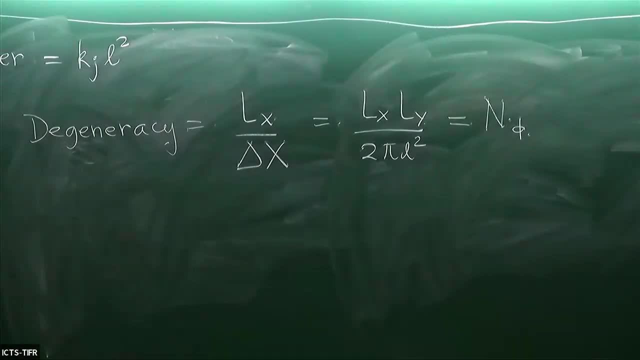 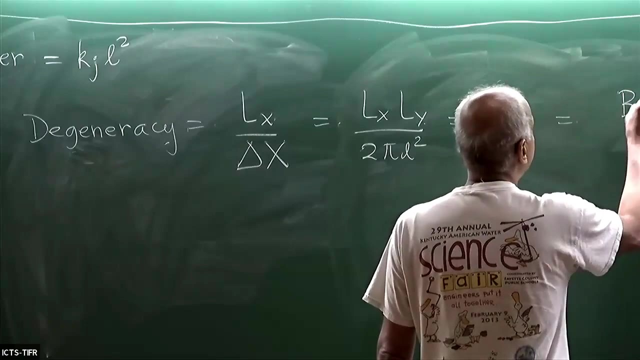 number again. so I'm going to give it a name and I'm going to call it n sub 5, okay, So you can perhaps expand this and you can write it like this: B, Lx, Ly over H over E. Make it completely. 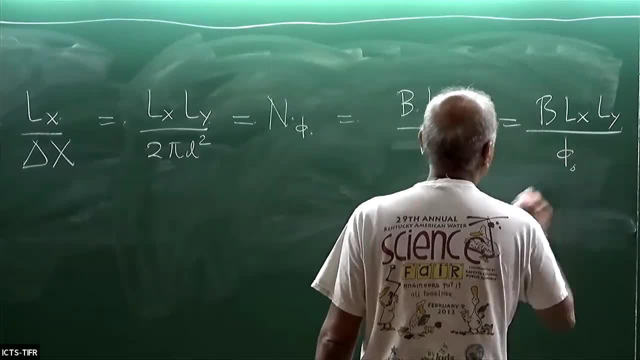 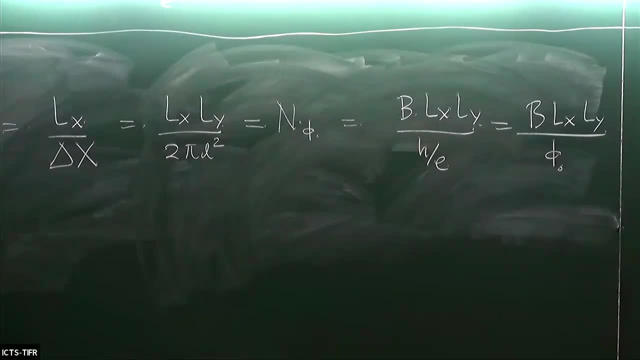 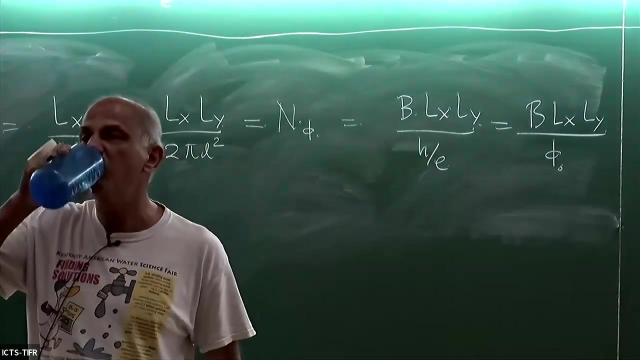 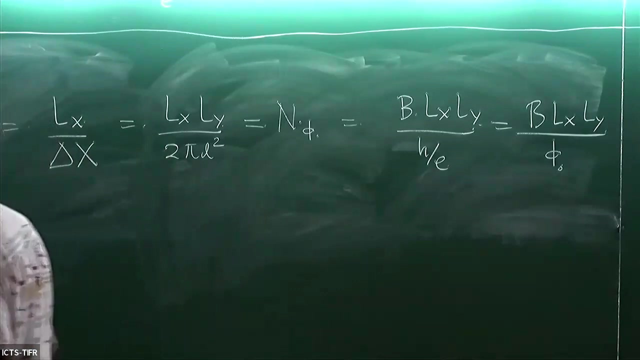 explicit. This is the total flux going through the sample divided by pi naught. That's what it looks like. So that is the degeneracy. Yes, you are. Yeah, Each wave function, Excellent point, Excellent point. So what you are saying is that this delta x is goes down with Ly. okay, So typically. 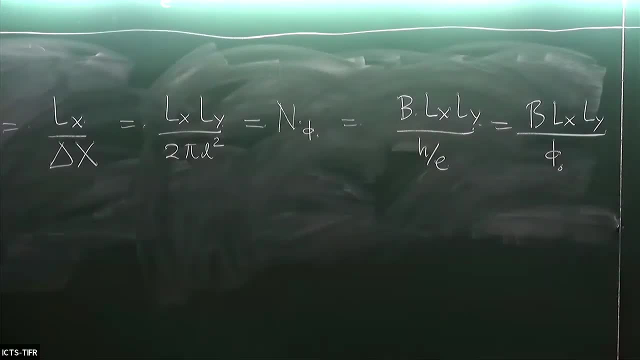 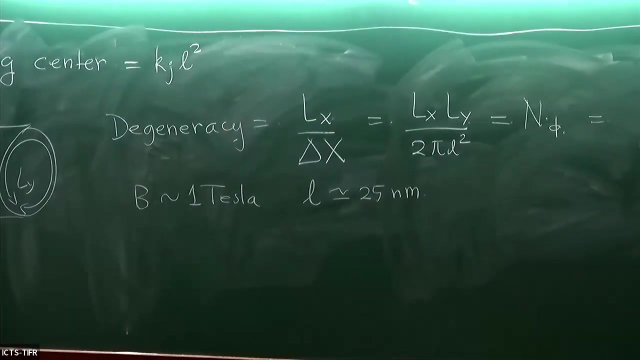 what you have in a sample, that's of the size of microns. let me give you some rough length scales. So if you have B, approximately 1 tesla, the magnetic length is about 25 nanometers. okay, That's a very tiny length And the higher you make the B, the smaller this. 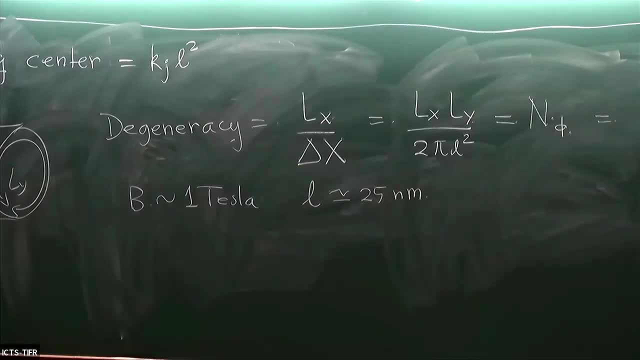 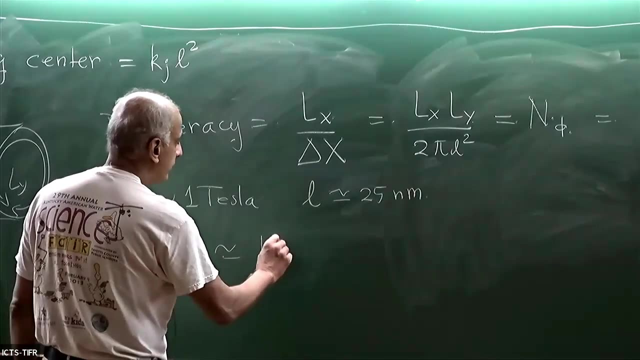 length will shrink because it's H bar over Eb square root right, Okay. Whereas the size of a sample Lx and Ly- is of the order of 10 microns. okay, That's typical size of a sample, maybe. 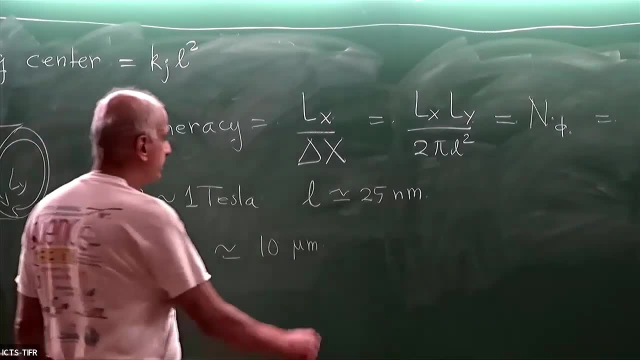 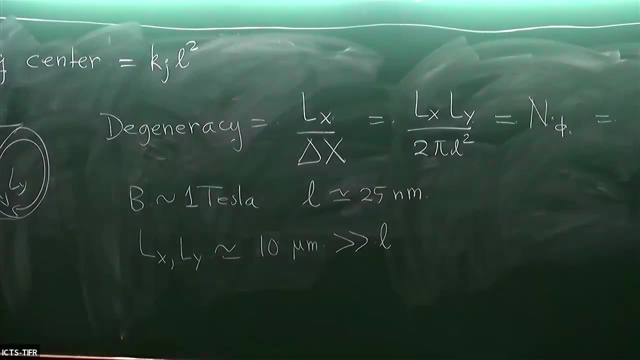 even bigger. So, therefore, typically, you will have this Lx and Ly much, much larger than little L, And so, therefore, what's going to happen is that this delta x is going to be a very tiny length indeed. okay, Because it is L times the ratio of little L by capital Ly. 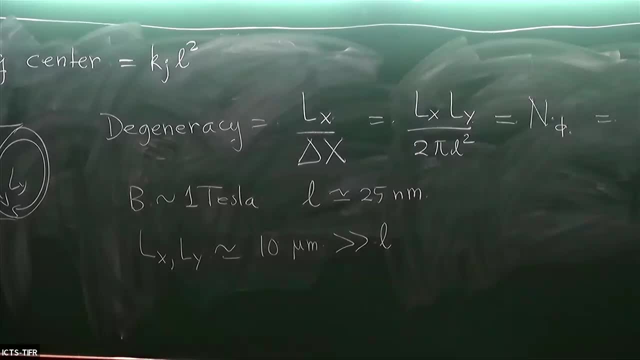 which is a very small number. So these guys are extremely closely spaced. And if I draw the wave function itself of one of these guys- let's say this guy- then it will actually look like this: There'll be some Gaussian centered at this point. There is huge, huge. 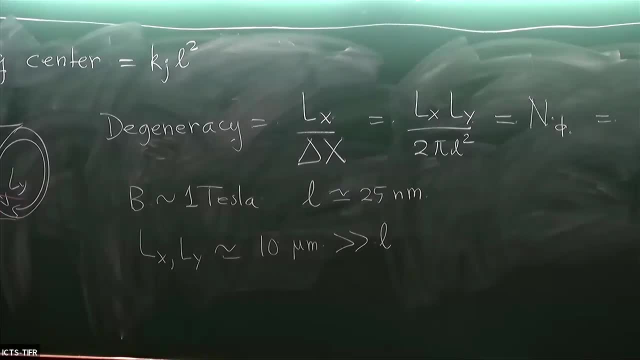 space And if I draw the wave function itself of one of these guys, let's say this guy, then it will actually look like this: There'll be some Gaussian centered at this point. There's huge. It passes many, many, many, many guiding centers, But nevertheless they're all orthogonal. 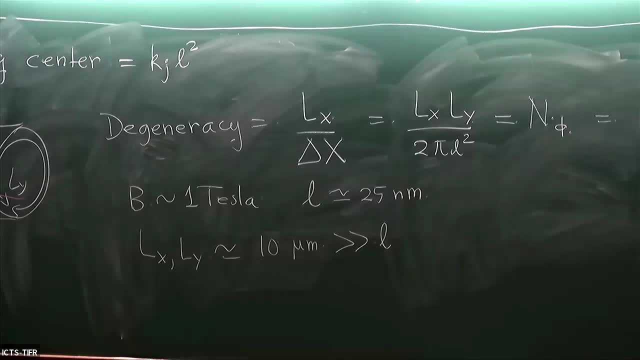 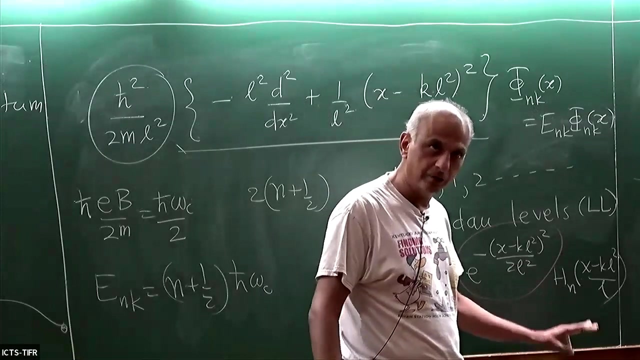 because they have different wave numbers in the y direction. So this is y-orthogonality. Yeah, It doesn't have to be a Gaussian. I'm just drawing this part of it. If it's the lowest Landau level, then it's indeed a Gaussian. If it's n equals zero Landau level, it is. 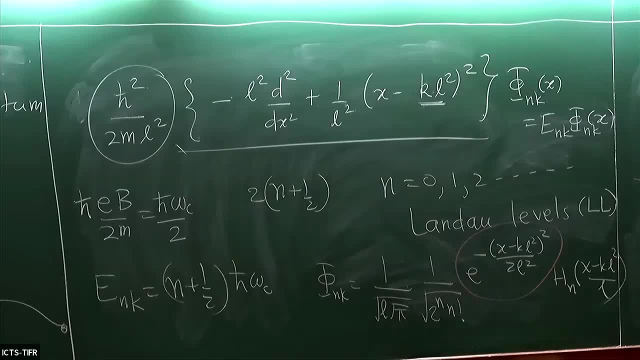 a Gaussian. If it's a higher Landau level, it won't be a Gaussian, It'll be something else. Why am I saying what, Flatter? You just speak about the guiding center, but the width of this thing is of the order of. 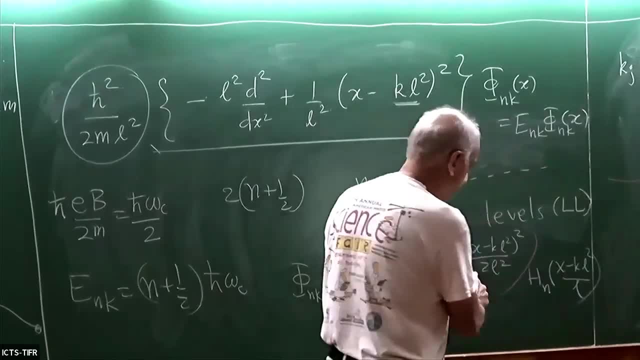 the magnetic plane. Just look at this Gaussian here. Okay, Whereas the distance between these two is that much, which is much, much smaller than the distance between these two. It's much, much smaller than the distance between these two. It's much, much smaller than the. 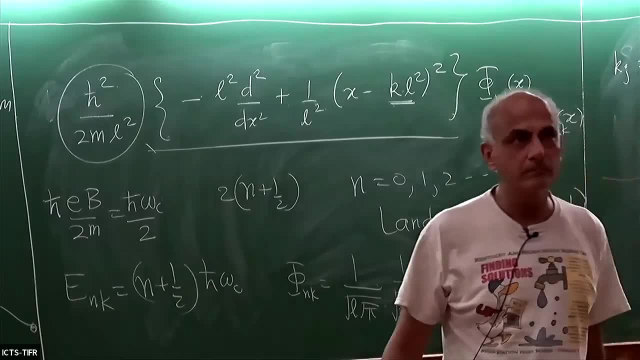 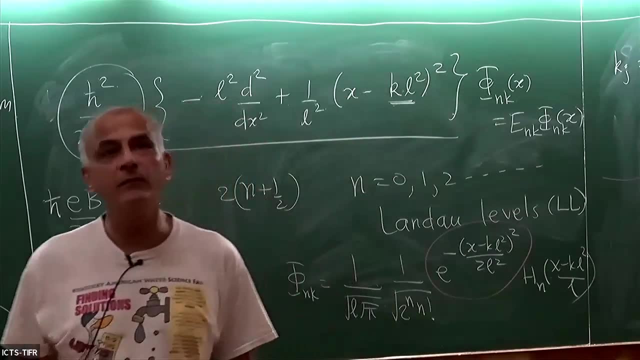 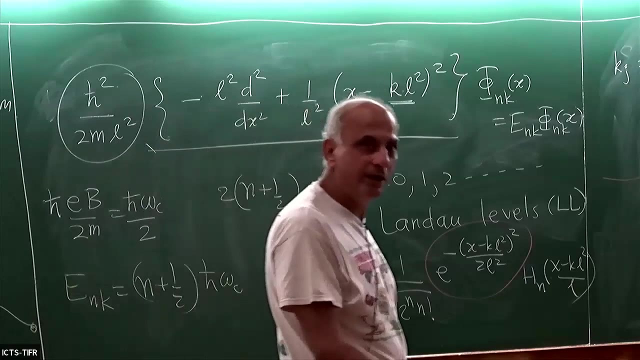 magnetic plane. Okay, Yeah, Nothing, It's not a big deal. They're overlapping a lot. Actually, there are some implications. So the point is that the fact that they overlap means that they sort of behave like itinerant electrons in terms of their spin exchange. 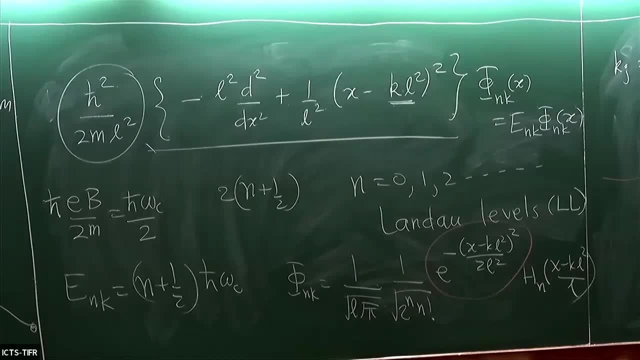 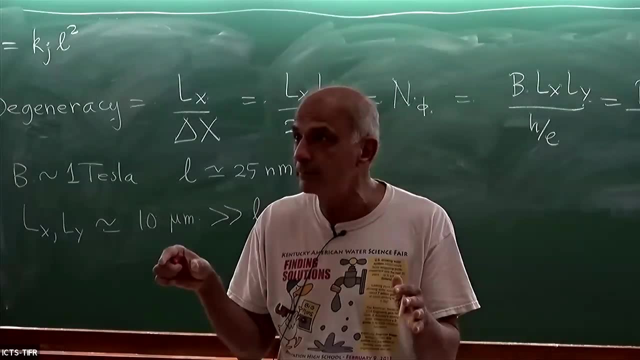 Properties. Okay, So if you have localized spins, then if the wave function is completely localized, there's no overlap between wave functions, then the Coulomb exchange integral is very small Right, Whereas if they're heavily overlapping, then the exchange integral is: 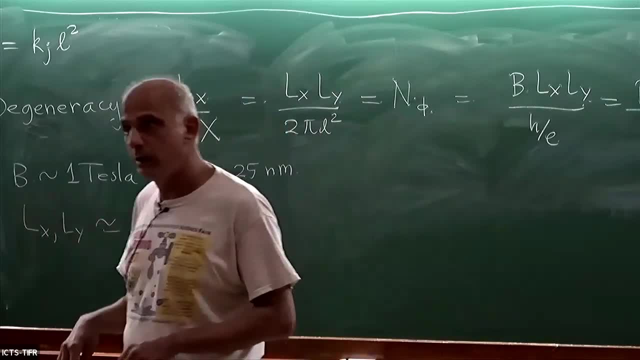 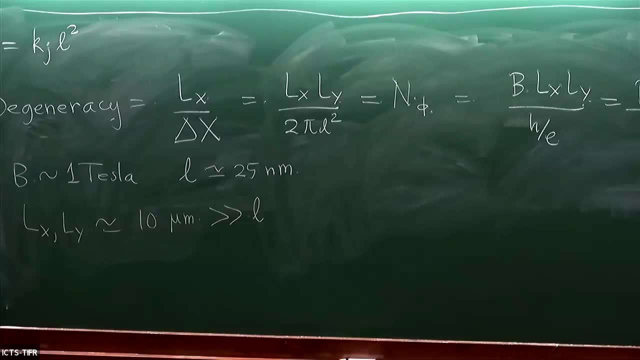 very big and displays a role in some of the phenomena, in even an integer quantum hall system in some case. Yeah, I cannot hear anything. Speak up, Hello, Yeah, So what if we consider the case where Lx is less than Ly? 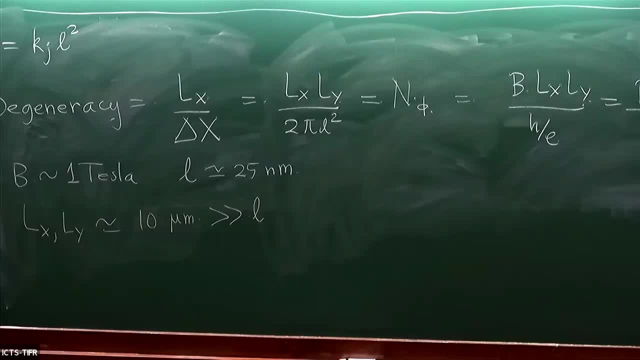 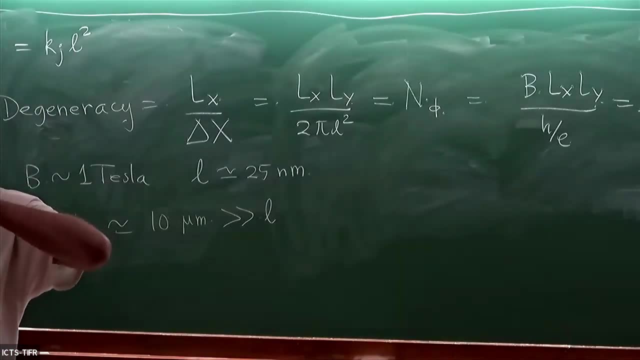 Lx is less than Ly, then it's a very weird case. I would say that that you know a lot of the phenomena that you expect, for the bulk of a quantum hall system will not be seen in such samples. Okay, Or you can think about situations where Lx or Ly become comparable. 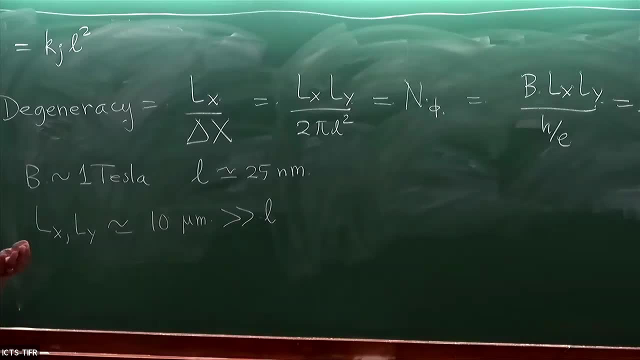 to L, little l. Again, you will not see any difference. There's no difference in the not see many of the phenomena. they will look very different. okay, yeah, In one Landau level this many electrons per spin, right, so if there are two spins with 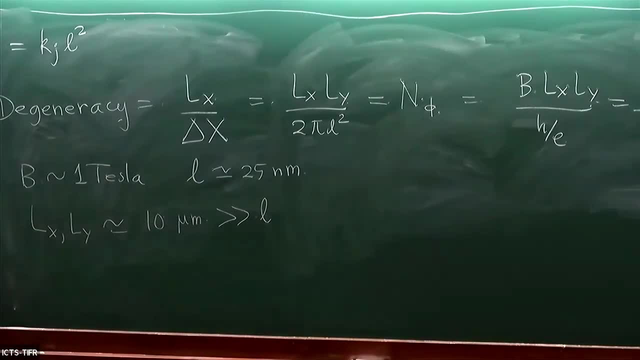 a non-entracting electrons. so in a particular Landau level you can fill up two times n sub phi electron, because up spin and down spin At the moment, yeah, no, no, not just a possibility, there's definitely a coupling, there's a Zeeman. 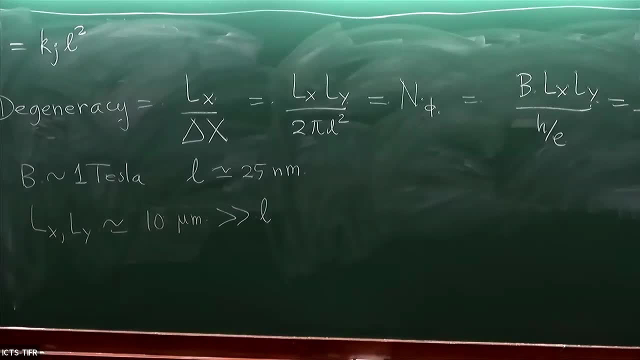 coupling to the spin. we're not talking about that. yeah, that's correct and there's a reason for that. the reason is that the Zeeman coupling in this material, gallium arsenide, is actually very small, so compared to, let's say, the cyclotron energy, which is h bar. so there are things. 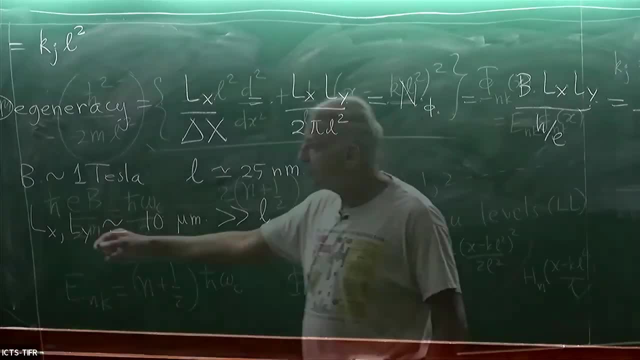 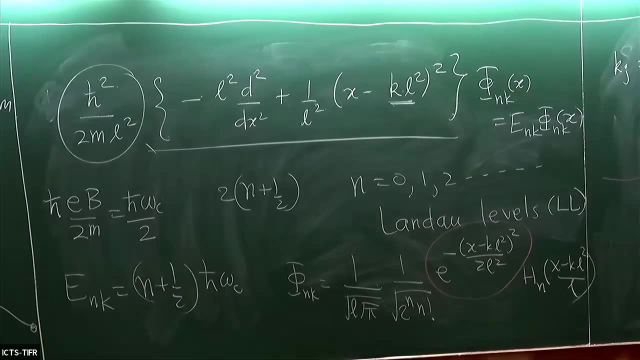 that I'm not telling you. For example, this M Here is not the mass of the electron in vacuum, it's the effective band mass of the electron inside gallium arsenide. it turns out to be very tiny compared to the mass of the electron. 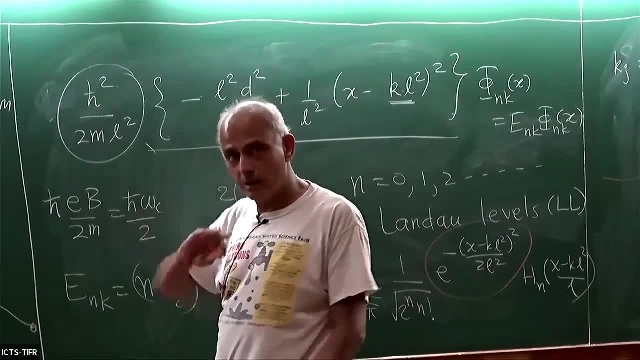 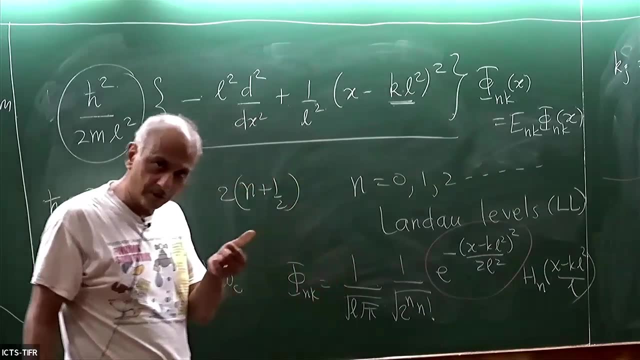 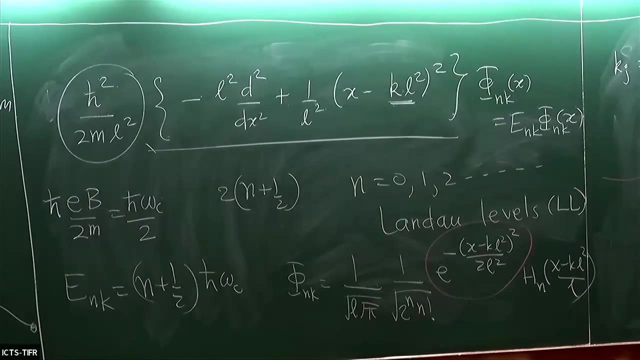 so this scale, this energy scale, is much larger than what it would be in vacuum. At the same time, the Zeeman coupling: there's a g factor coming from the spin orbit coupling of gallium arsenide, which actually shrinks the importance of the Zeeman. okay, so the 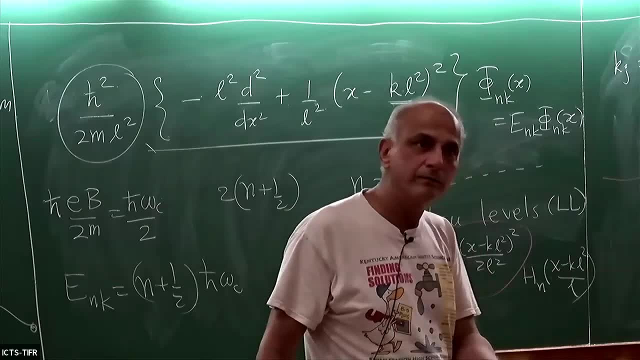 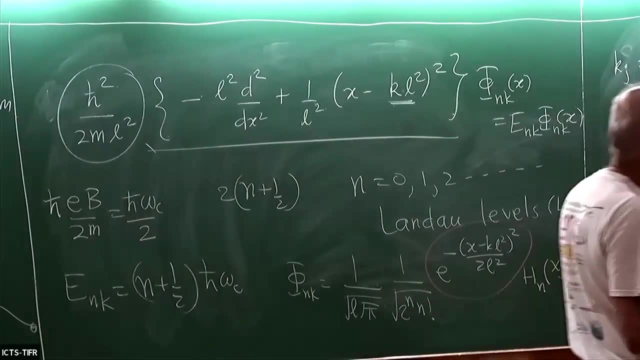 Zeeman, energy is much, much smaller than the cyclotron energy, so that's why it's a reasonable approximation to think about the electrons- as you know, the Hamiltonian- as being almost spin independent. I'm sorry, the degeneracy again. okay, so what I'm saying? 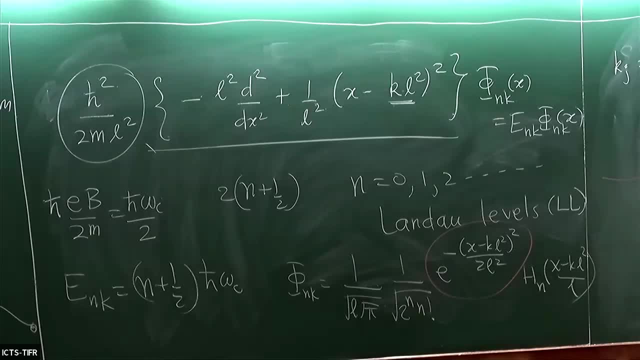 is that each of these positions is this: Okay, K, L squared K is quantized by the periodic boundary conditions, so each of these represents a state. okay, Now you ask how many states are there within a length of L sub x? 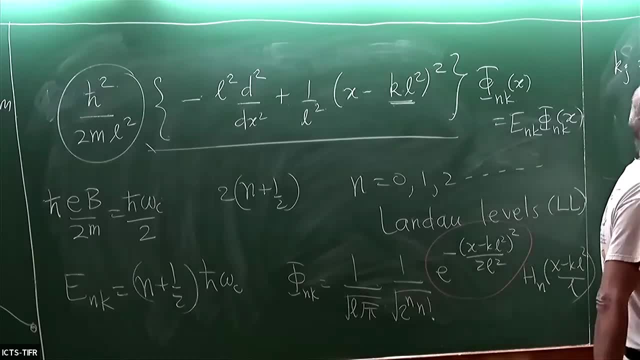 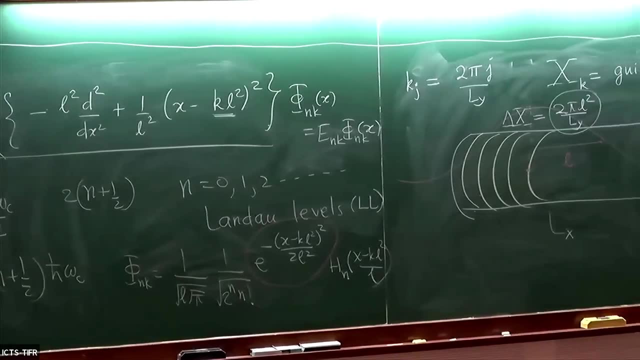 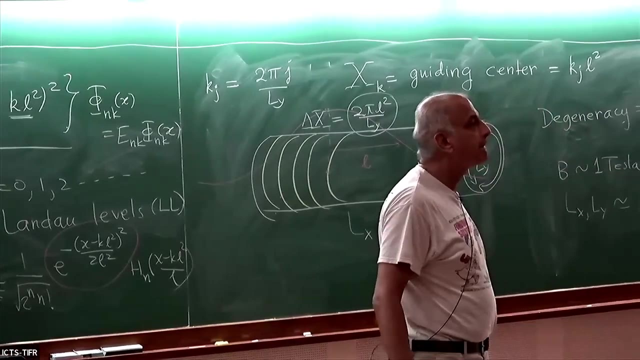 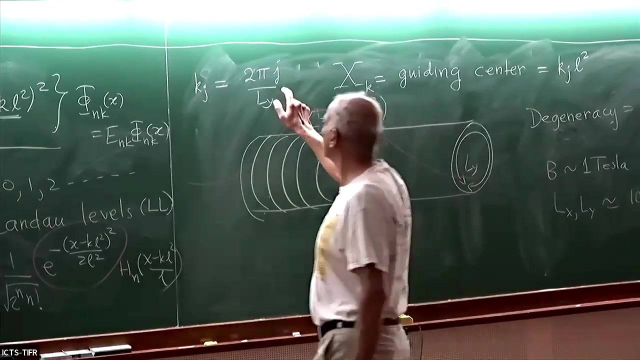 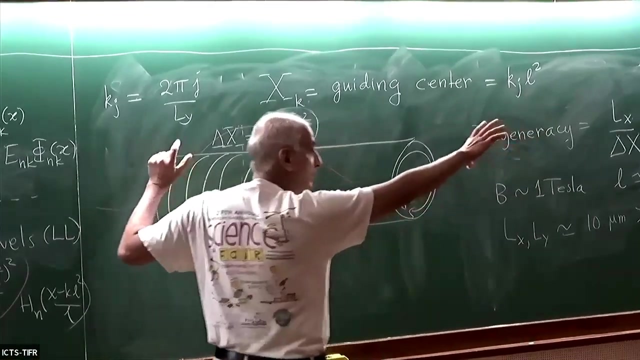 Okay, that will be L sub x divided by the spacing between these guys. Sorry For a given value of k y, there's only one orbital state. These are the choices for k. Okay, so if you take this tube to be from minus infinity to infinity, yes, yes, but every. 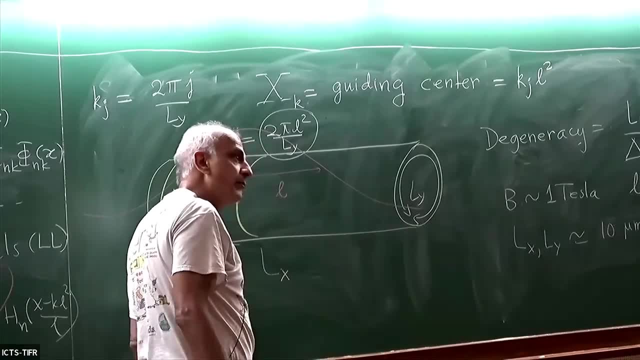 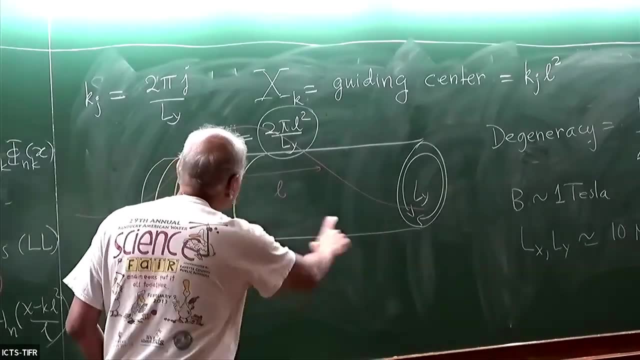 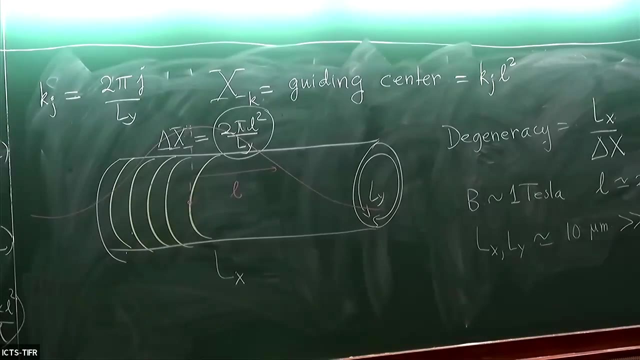 one of these guys has a position in x. If I ask myself, what are the Landau orbits that lie within my L sub x? That's these guys. There are other guys lying outside Here. They're all quantized by this right. 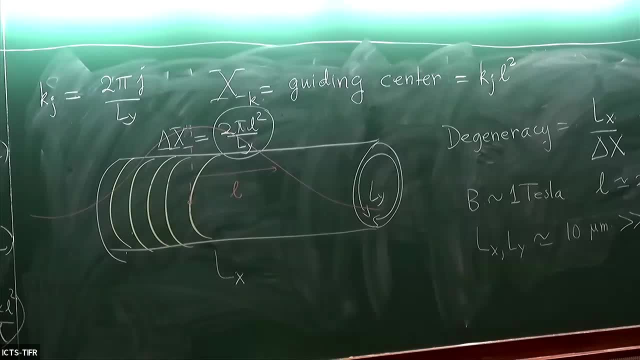 Yeah, j can be anything. You're right, j can be any integer. Most of those orbits will lie outside my sample. Okay, their wave functions will not have support inside my sample. You can also have many Ns, But we're talking about a single N. 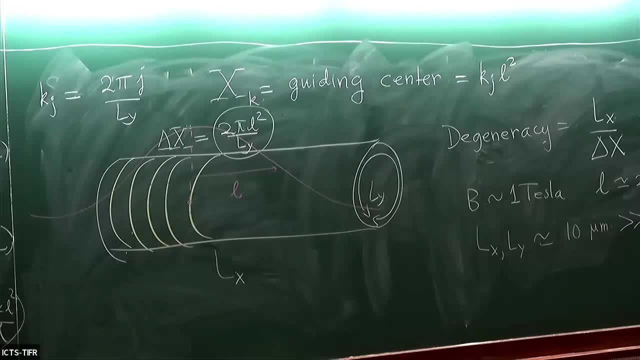 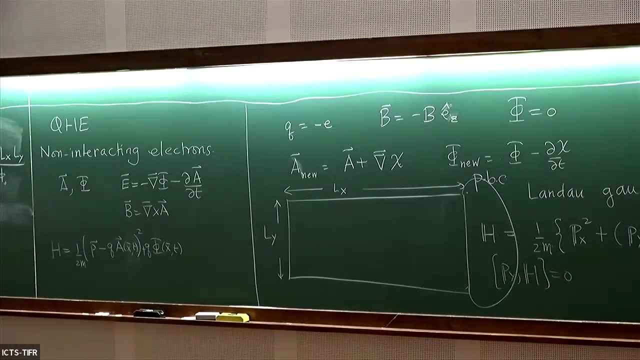 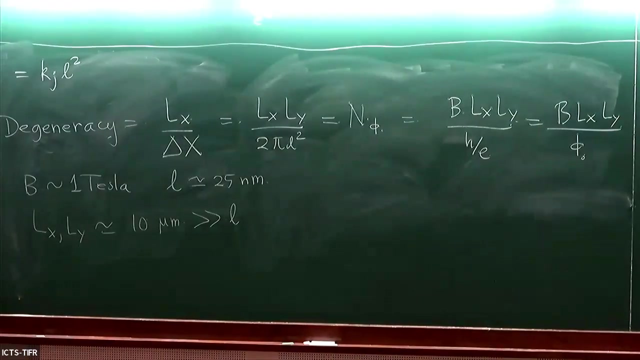 will end right now. I hope. Okay, was that the question? Was it n or it was k? The question was about k, not n. Okay, yes, Other questions, Yeah, Yeah, Very good. So if it has any component. 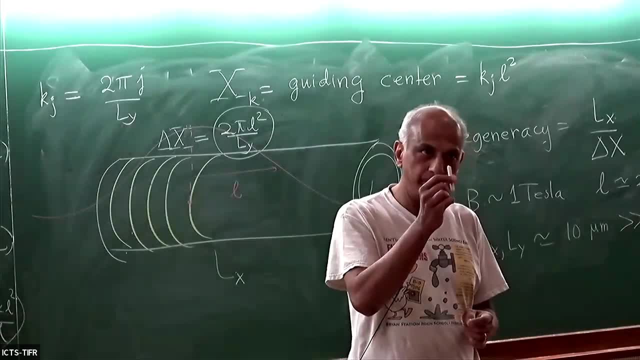 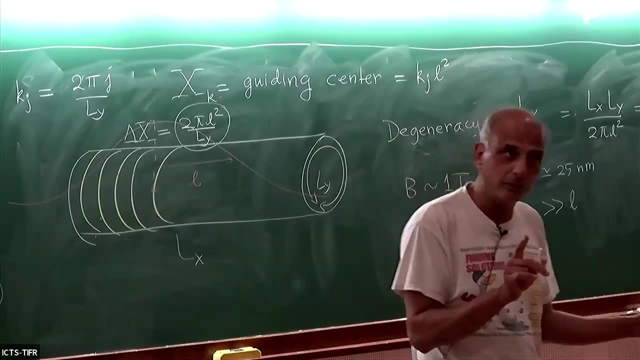 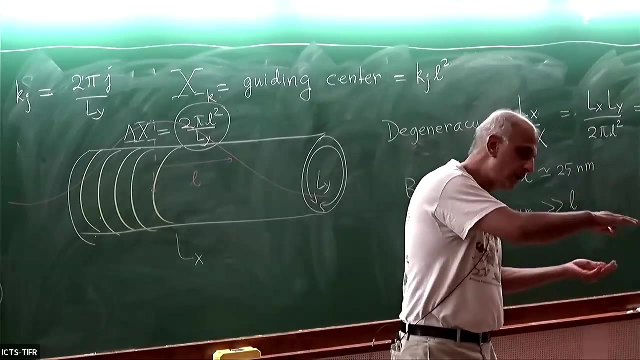 in the perpendicular direction. the perpendicular component will come into the orbital part of the Hamiltonian. The non-perpendicular, the parallel component, will come into the Zeeman part of the Hamiltonian. There are other second-order effects that it does in gallium arsenide because the field in the plane can somehow alter the wave function. 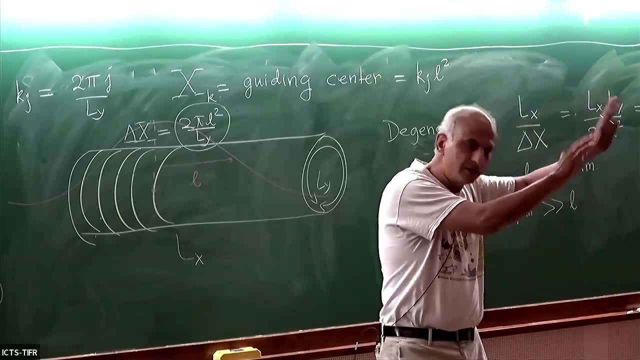 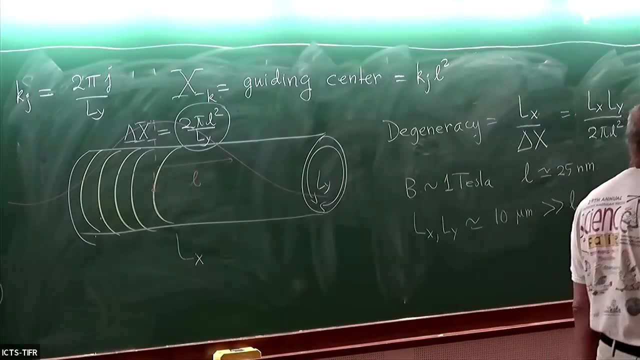 of the 2-DEG. But let's leave all that aside. That's complicated stuff. If you did what? No, there won't be. There will be a finite degeneracy. No, no, no, Because then it will be the same state. right, Because the case, even though you can come back, they. 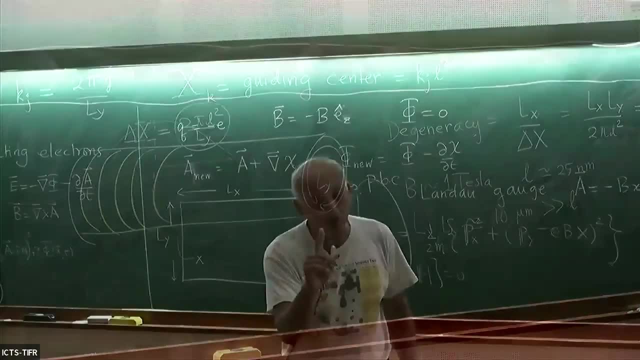 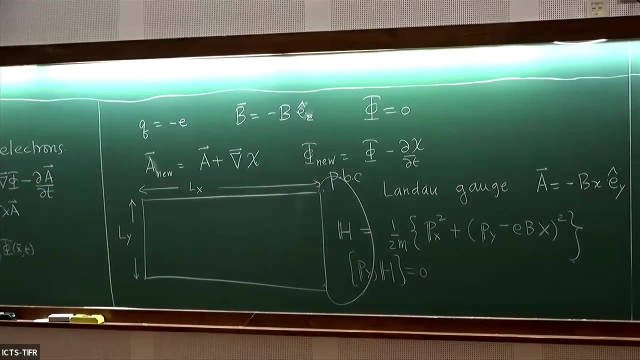 will start repeating themselves. Those states will no longer be orthogonal to each other. Okay, Let's talk about it offline. Okay, So per Landau level, there is a finite degeneracy. It's equal to the area of the surface area of the torus divided by the number of flux. 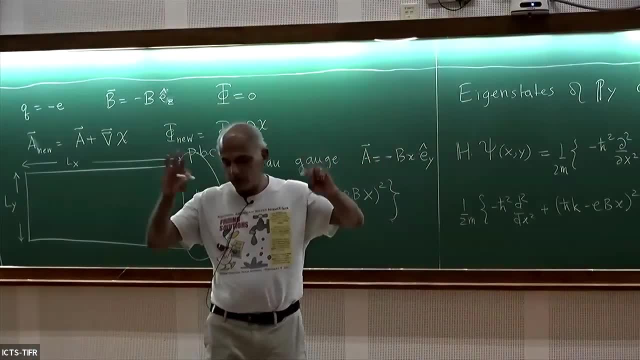 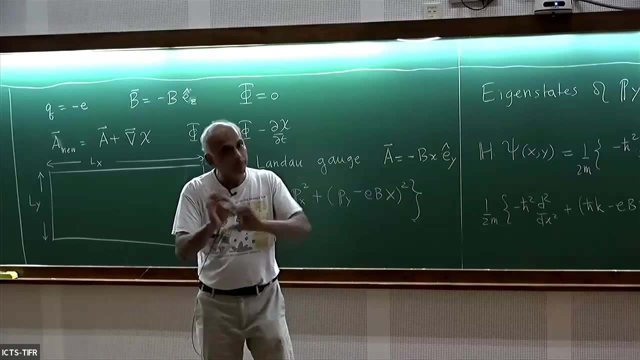 quanta. Okay, You have to make sure of a few things, Like you have to make sure that the, that degeneracy is an integer. Okay, When you quantize it on a torus, you have to make sure of that. 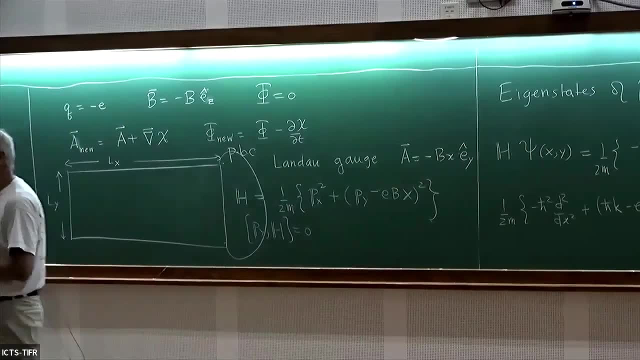 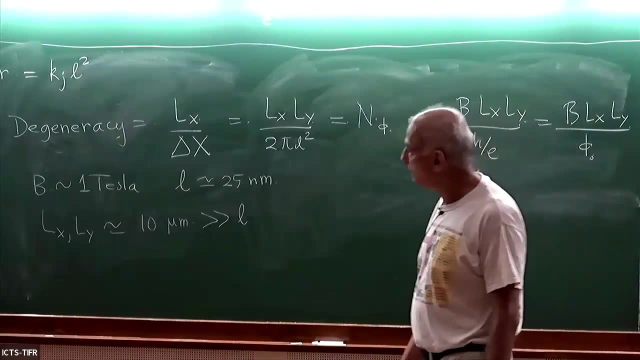 But given that it's There's a finite degeneracy, Okay, Yes, Add disorder in this. now, How do I add disorder? I mean, adding disorder in a real system is very easy, right? You just put in some impurities and some potential and stuff like that. Okay, Sorry. 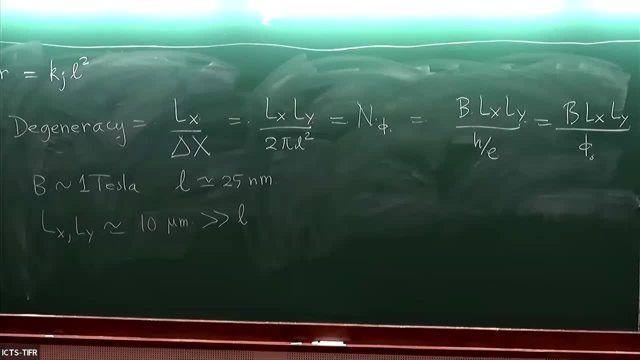 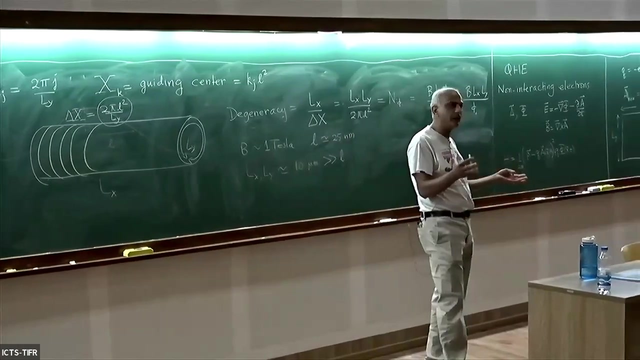 I mean in the analysis, In the, In the Hamiltonian. how do you model disorder? We'll talk about that in a few minutes. Okay, You have to do it approximately. You can't do it exactly Or you can, but it'll be heavily. 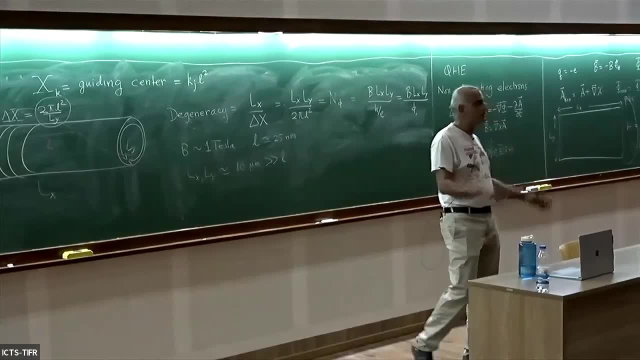 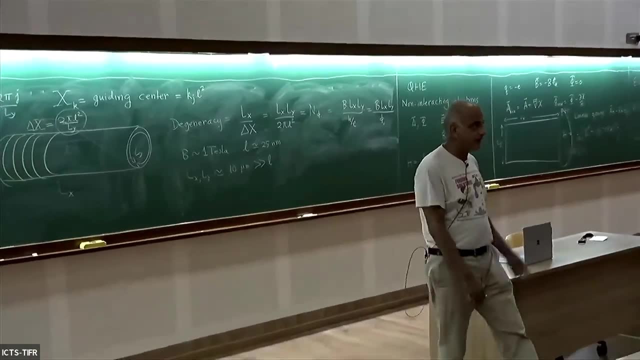 numerical. Well, hey, this is great. Lots and lots of questions. So at least you guys are not sleeping. But I warn you that if somebody starts sleeping, including Yuval here, I will call them out. Okay, So, all right, Great, So let's proceed. 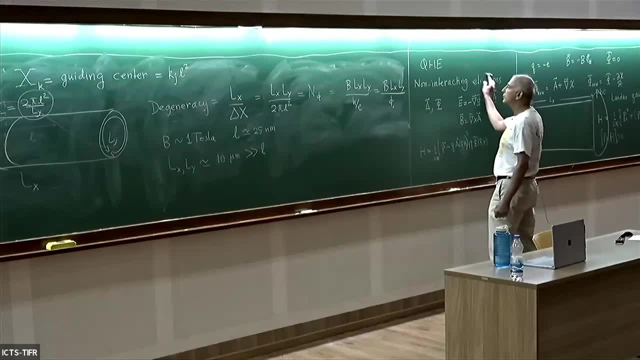 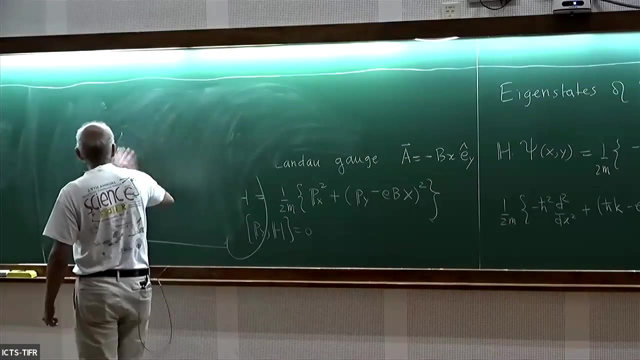 And now we're going to talk: Okay, Okay, Okay. So what does the spectrum now look like? So what I'm going to do is I'm going to draw something known as the density of states. So this is the number of states per unit energy interval. 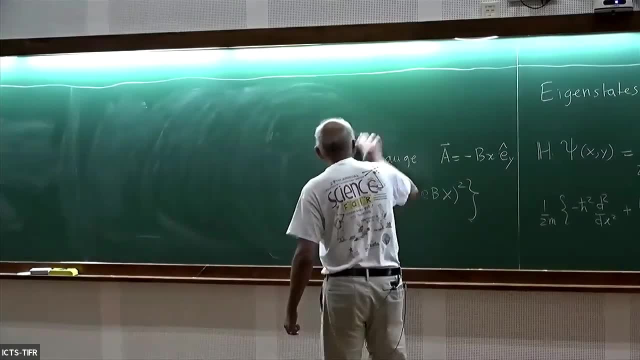 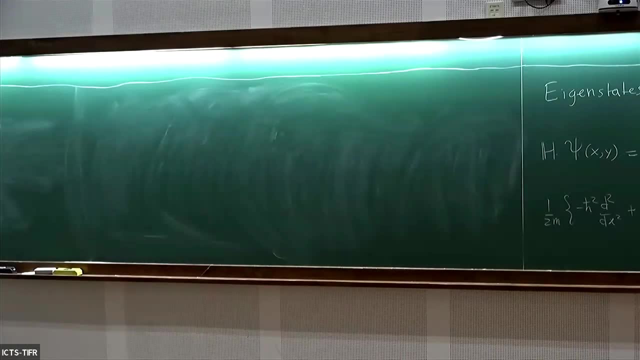 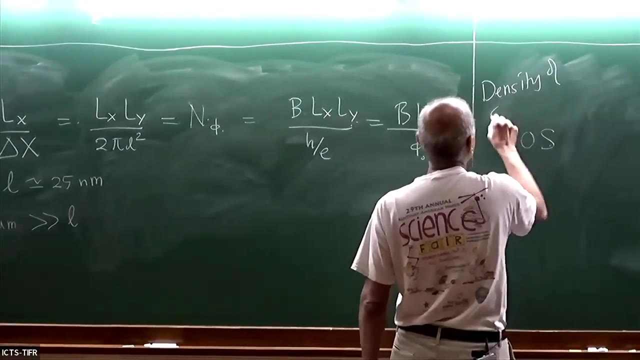 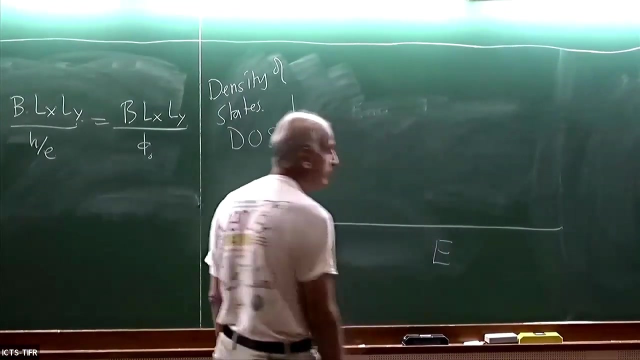 Okay, It's very commonly used in condensed matter for all kinds of materials, So let me plot that, So I will call it DOS. Okay, So density of states. Very good, So here is the energy, And there on the vertical axis is the density of states. 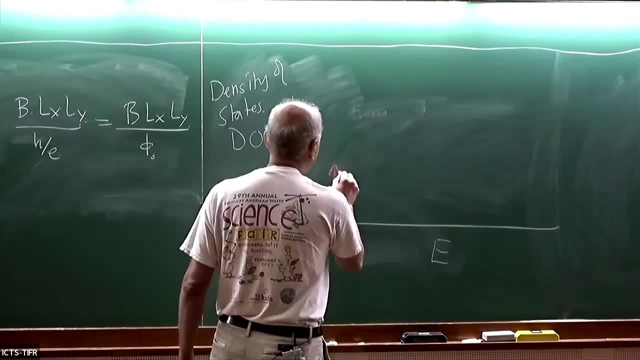 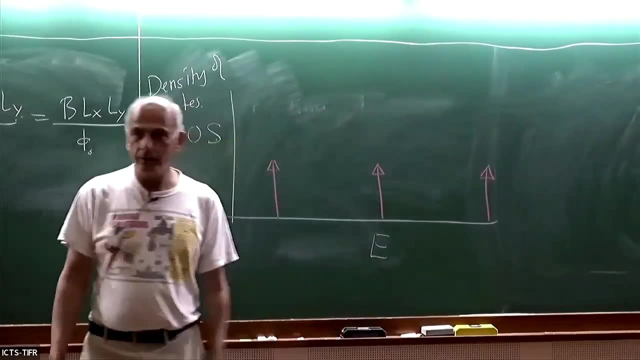 So I'm going to draw something that looks like that, Something that looks like that. Whenever I draw a vertical line with an arrow like this, it means the delta function Okay, And the height of this arrow represents the degenerate. It represents the degeneracy. 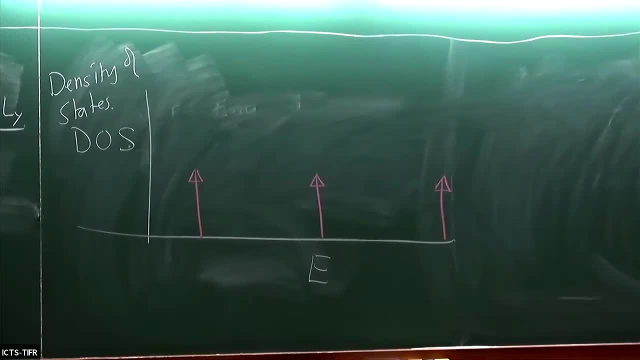 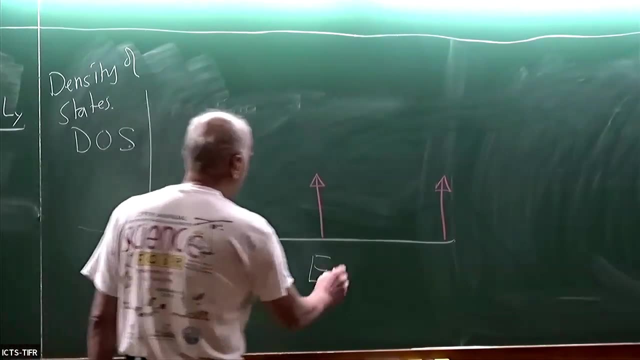 The number of states that are contained in this delta function. Okay, Delta function means it's just a particular energy. This particular energy is H bar omega C1 over 2.. This particular energy is 3 by 2 H bar omega C1, and so on. 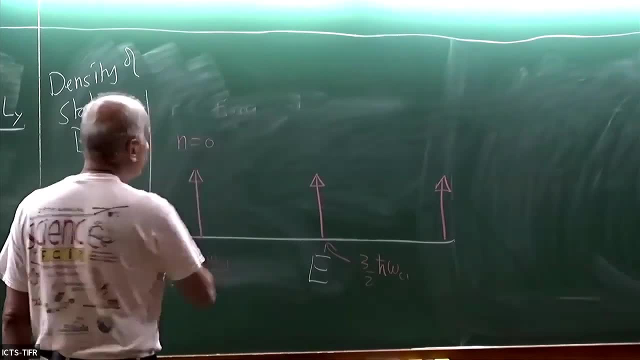 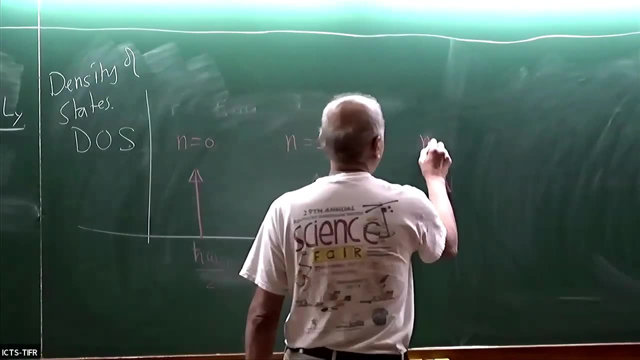 So this would be called the N equals 0 Landau level of the red field And this would be called the N equals 1 Landau level. This would be called the N equals 2 Landau level, 2 Landau level, and so on. 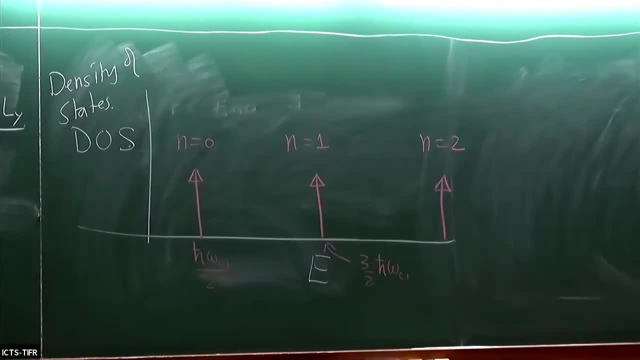 They're equally spaced. Okay, If I increase the field, suppose I increase the field to, let's say, I don't know, one and a half times this Right. So what will happen? Two things happen. First of all, omega C grows up, goes up. 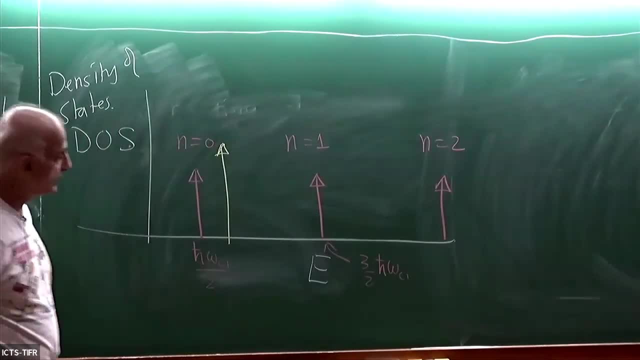 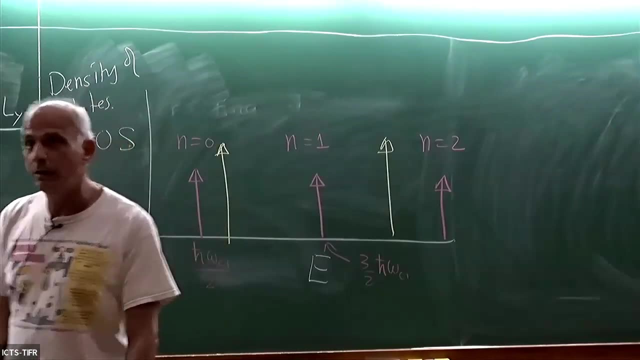 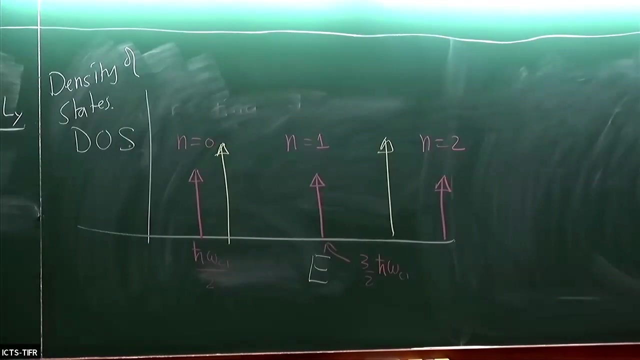 Right, So these things are spaced further and further apart, And this guy will come here, And then the height of this thing also increases, Because the degeneracy of a Landau level also grows With the magnetic field. Okay, So that is what happens. 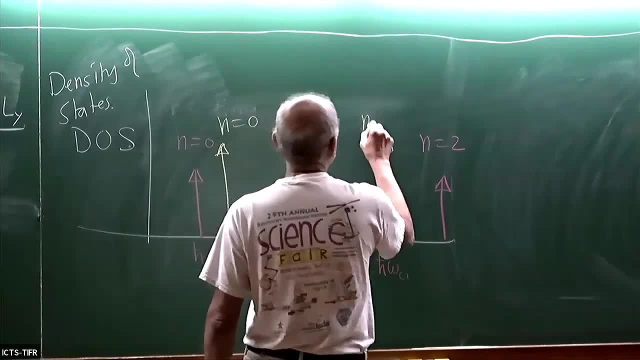 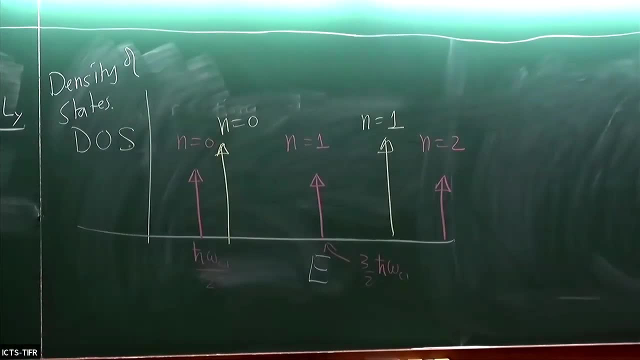 So this is N equals 0 of the yellow field, This is N equals 1 of the yellow field, and so on. So this is what is happening. So you have some fixed number of particles in your system And you're sweeping the field. 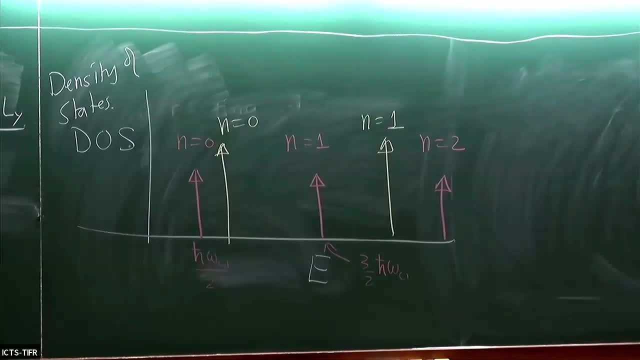 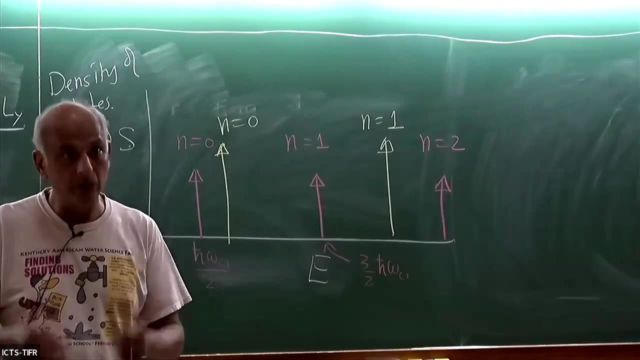 So something very complicated is going on. Okay, So typically you will have a certain number of Landau levels full And some Landau level partially full. That's what will typically happen As you sweep the field. you know all these things. the degeneracy will increase. 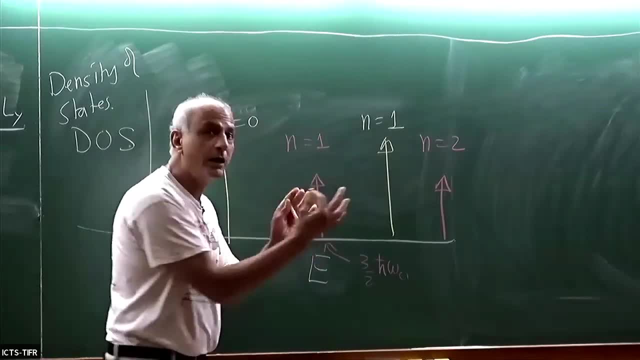 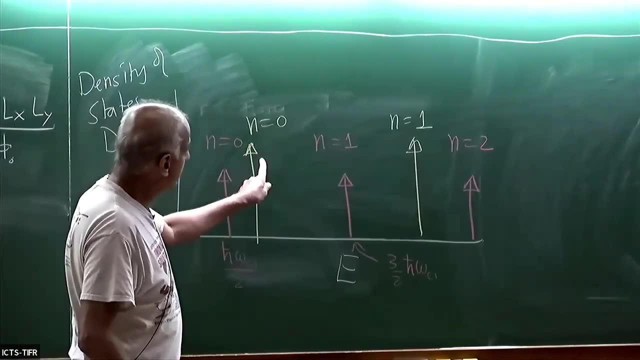 And at some point you'll have just two- let's say Landau- levels, exactly full, Okay. And then you increase the field a little bit more And then the degeneracy here goes up, And here it goes up. So therefore this guy will become full. 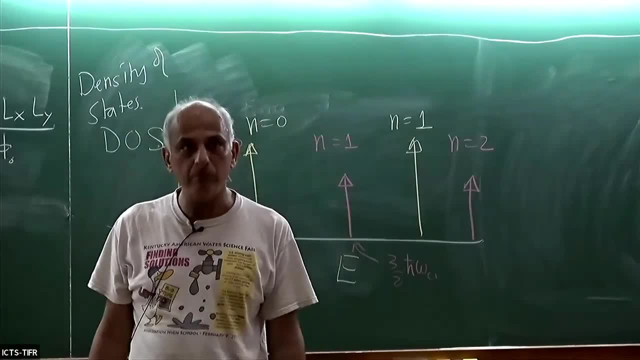 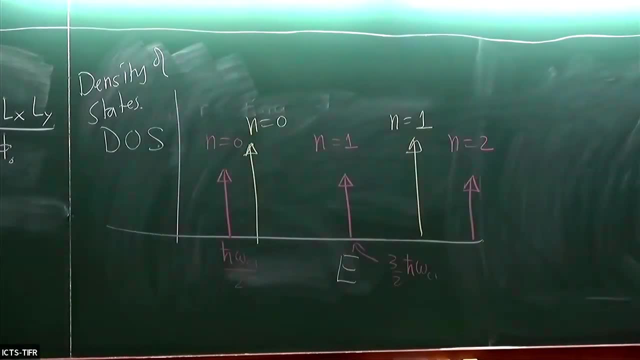 This guy will become slightly less than, And so on. Some very complicated stuff happens. This was actually all worked out. The reason this is called Landau levels: It all worked out by Landau in the 1930s. There's something called that you do in statistical physics, or somewhere called Landau diamagnetism. 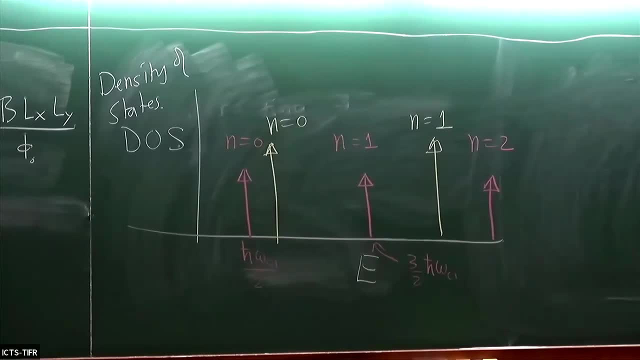 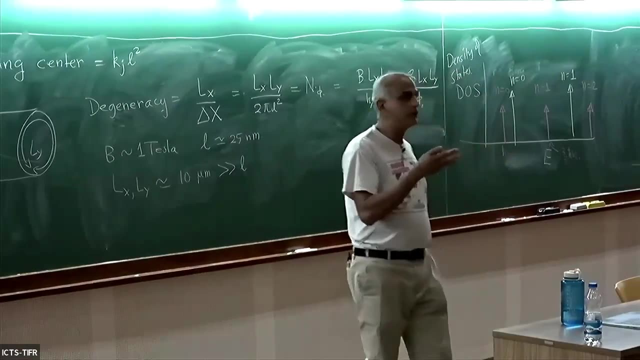 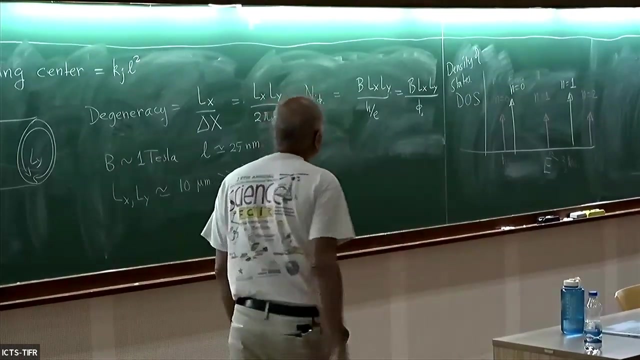 Have you guys done it? Only one person has done it: Landau diamagnetism. I think I should have a word with your STATMAC teachers. This is something that you should know about Something very basic. Okay, So that's what it looks like. 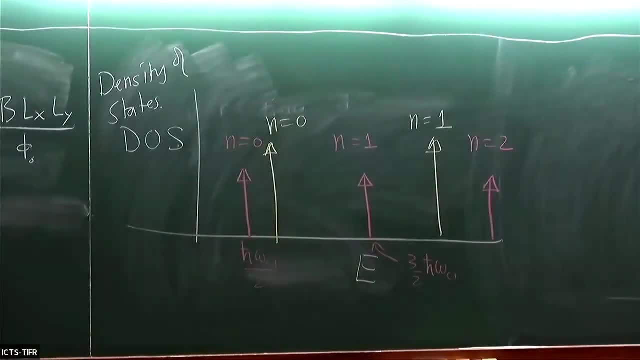 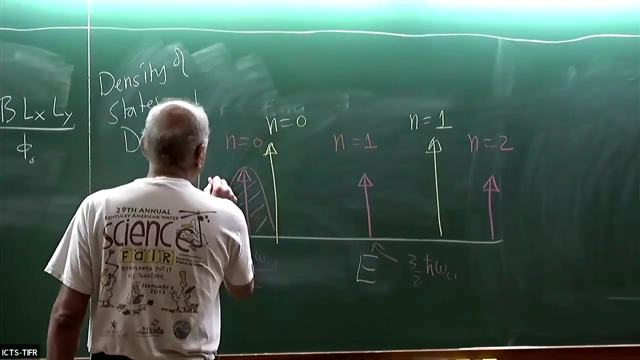 Okay, Now we're going to talk about disorder in detail in a little bit. I have 20 minutes, But first we're going to talk about edges. But let me say what happens with disorder. So what will end up happening is that there will be localized states around the center. 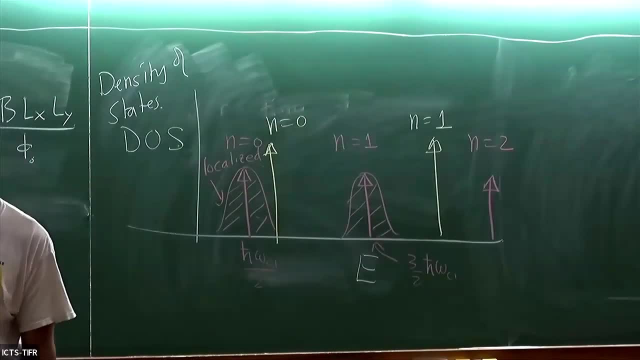 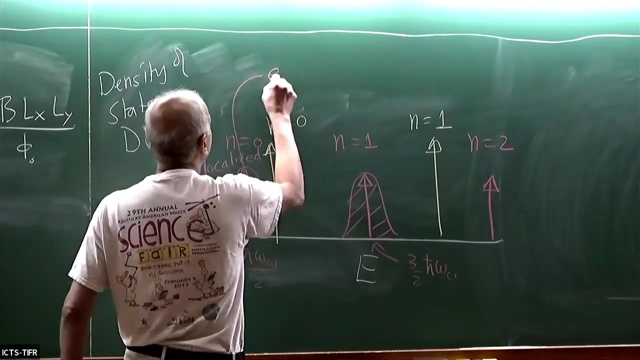 of each land. In other words, the Landau level, which used to be a delta function, now broadens out into a bunch of states that are spread out over some finite energy range, And most of these states are localized, But there is one state in every Landau level that's extended. 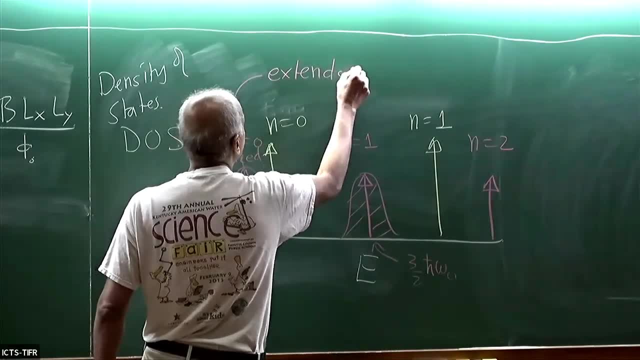 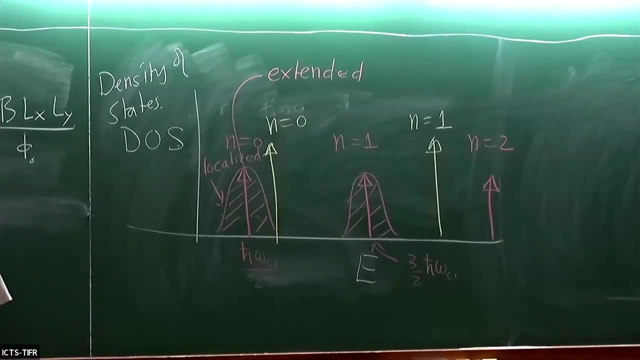 I'm going to show that to you. That is the picture with disorder. But let's get to it in due course of time. First we want to talk about edges. Extended means that the state has one single state has support from one edge to the other. 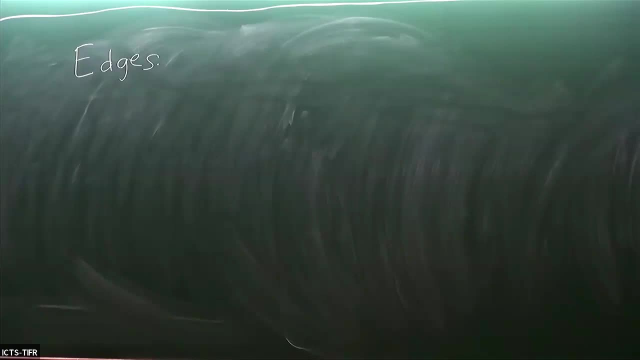 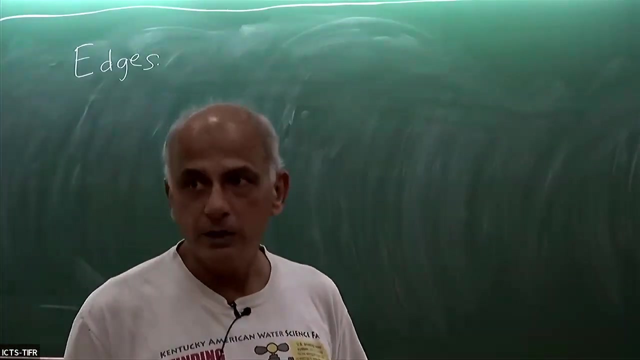 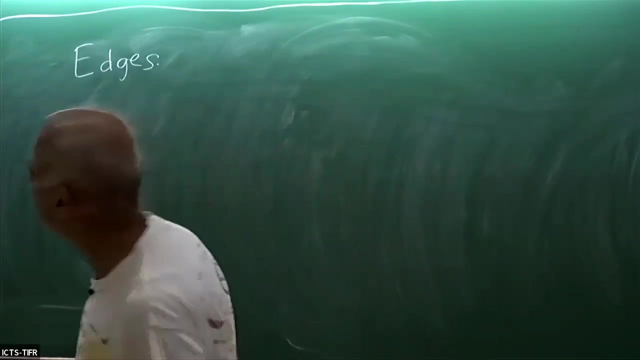 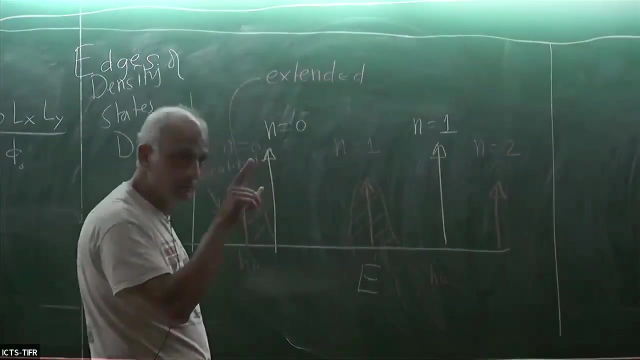 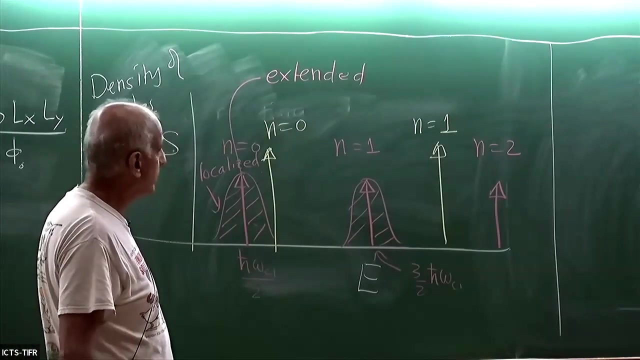 edge. That's what I mean by extended, Sorry. Yeah Yeah, The spectrum is gauge independent. Which one goes up and which one goes down. The degeneracy depends on the field, the strength of the field, Yeah Yeah. 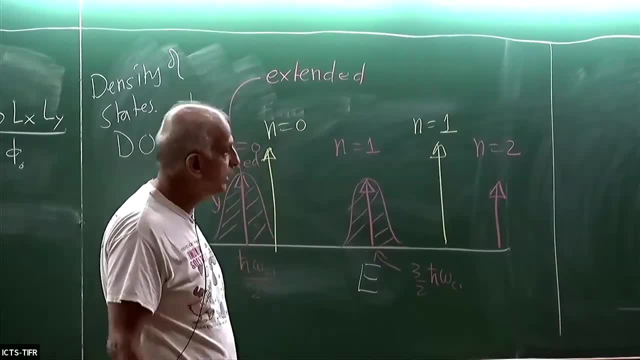 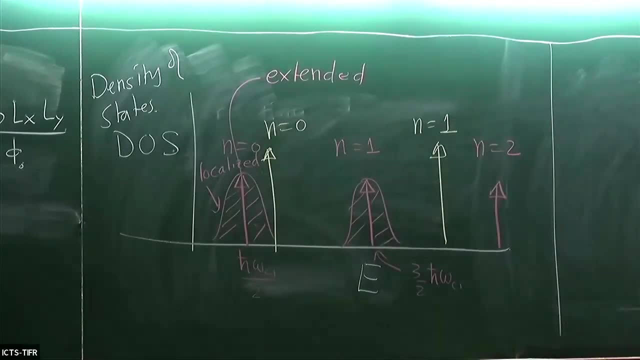 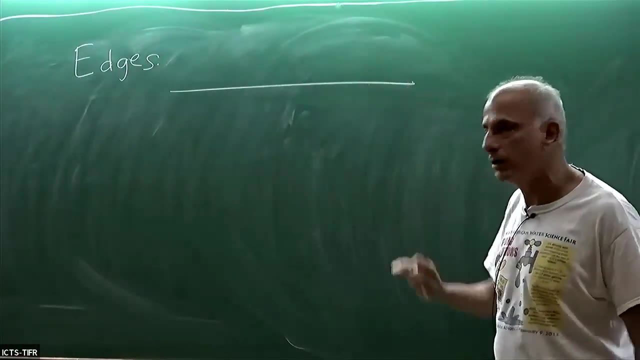 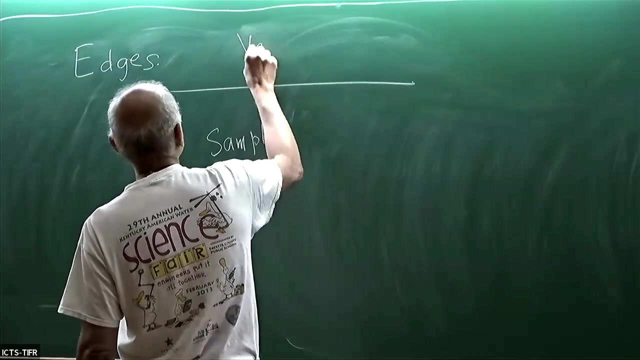 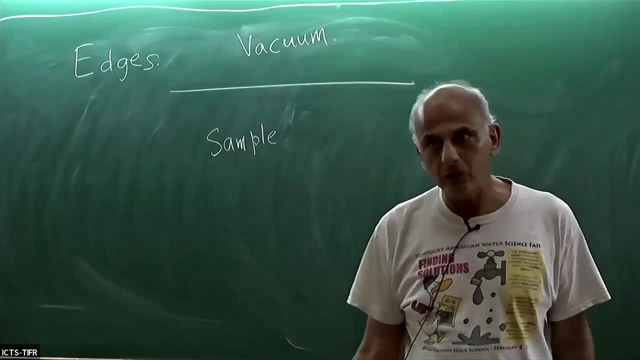 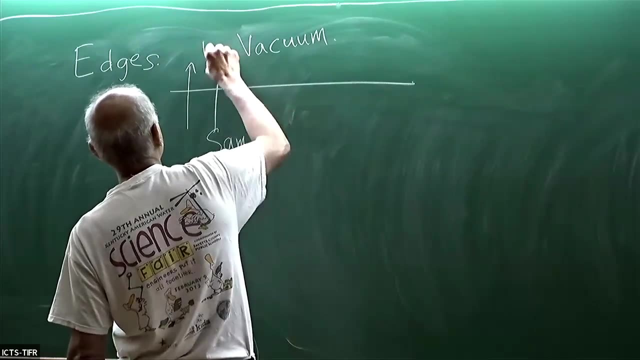 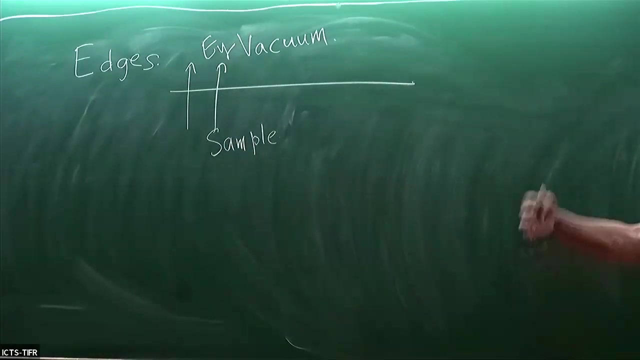 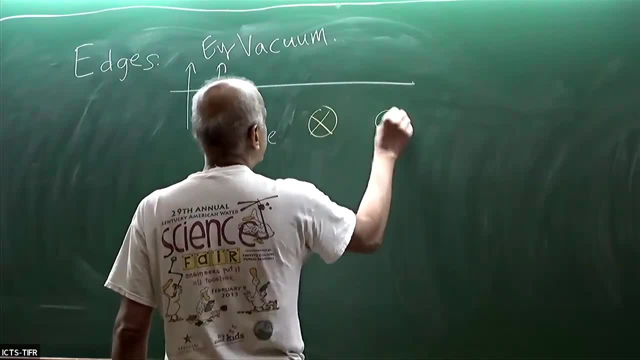 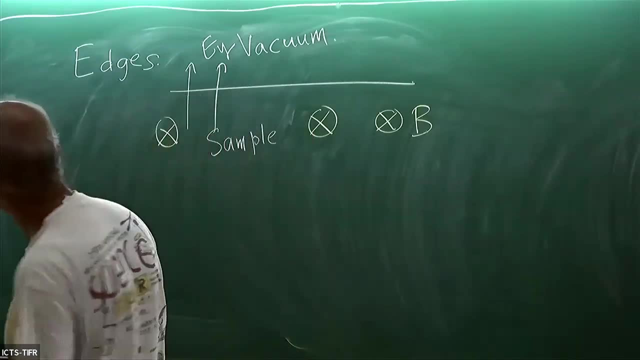 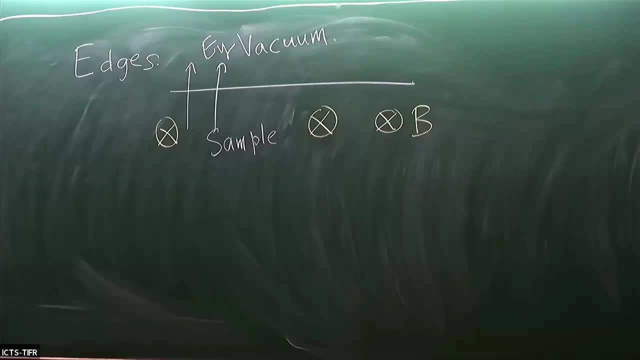 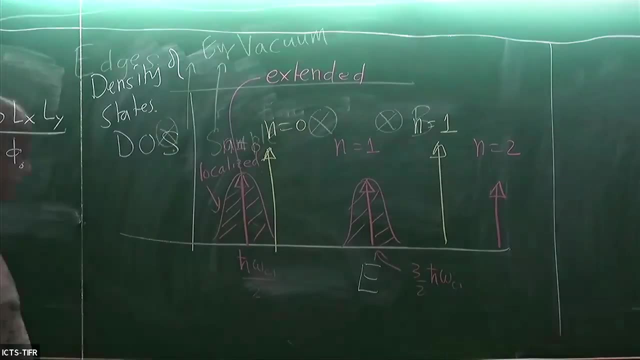 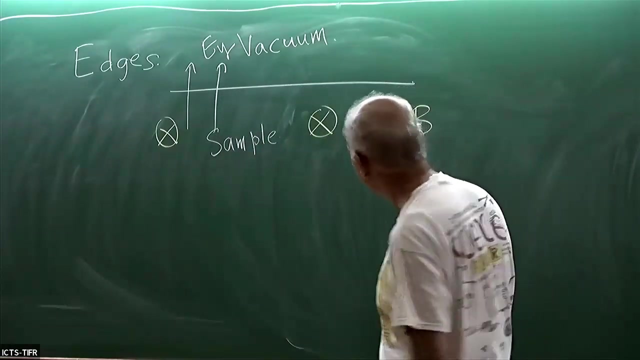 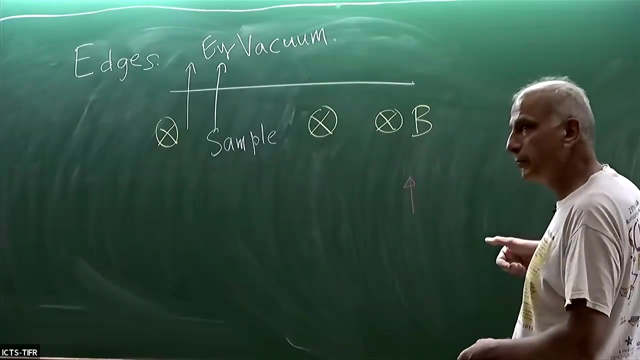 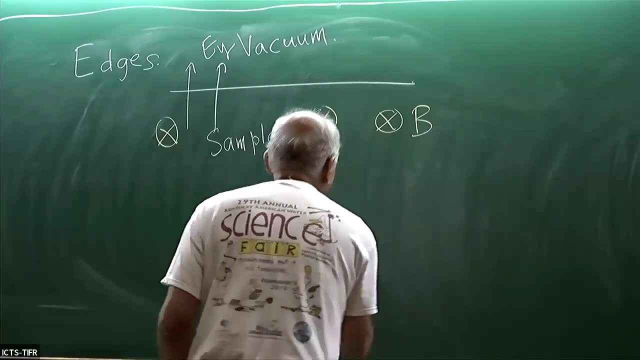 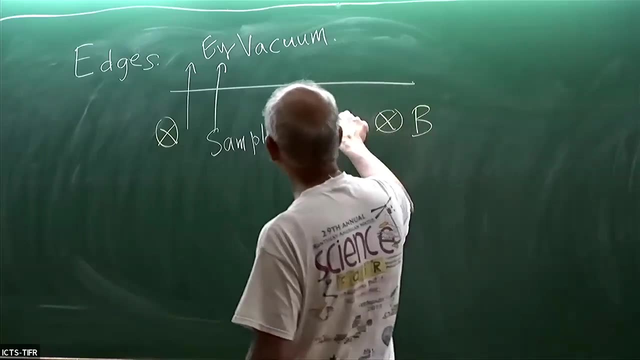 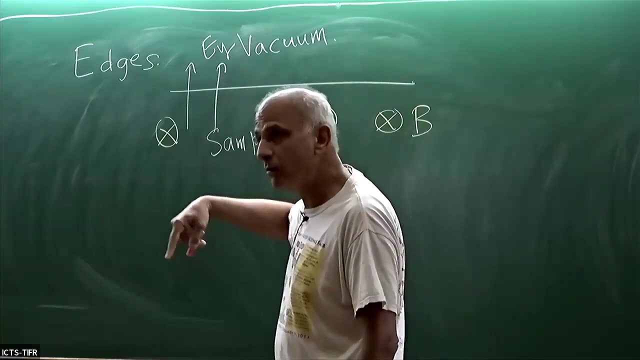 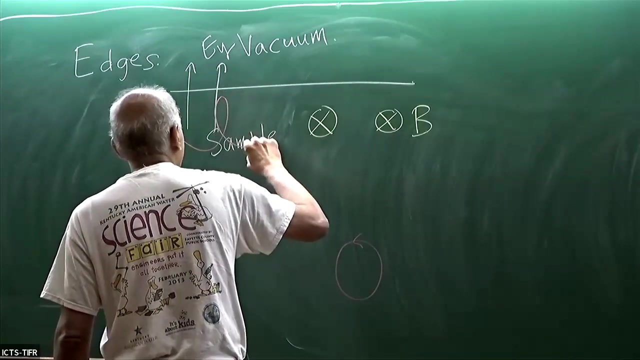 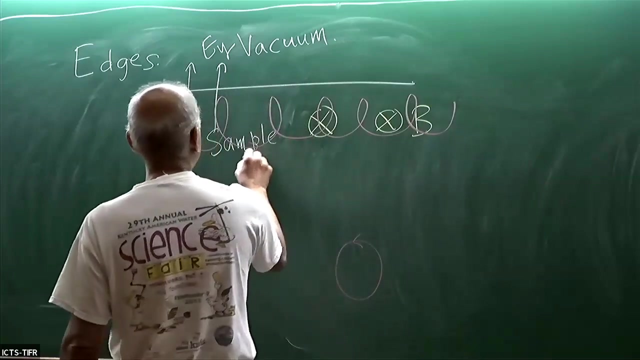 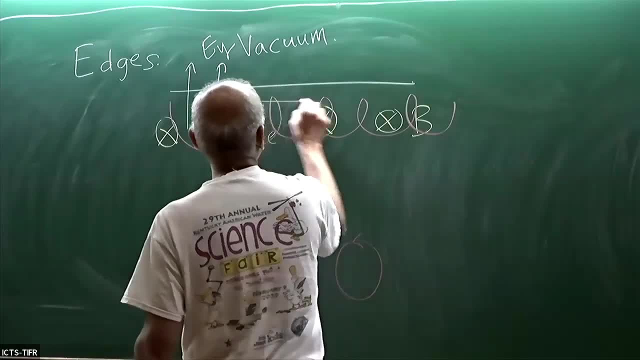 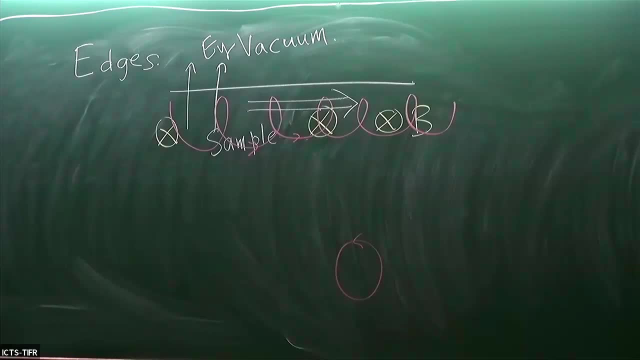 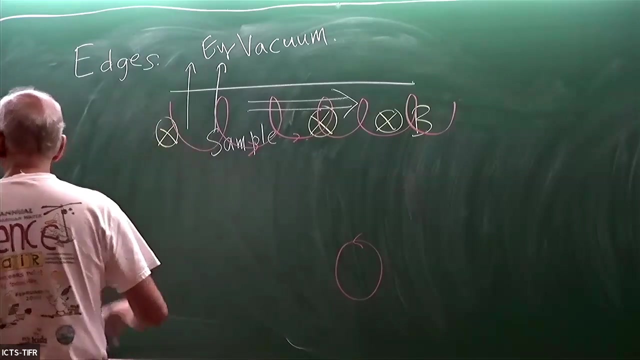 going. So overall, it's actually going in that direction. That is a semi-classical picture of what an electron does near a quantum Hall edge, But I'm going to give you a slightly better, better point of view. Okay, so let's take, instead of this electric field, let's take a hard edge. 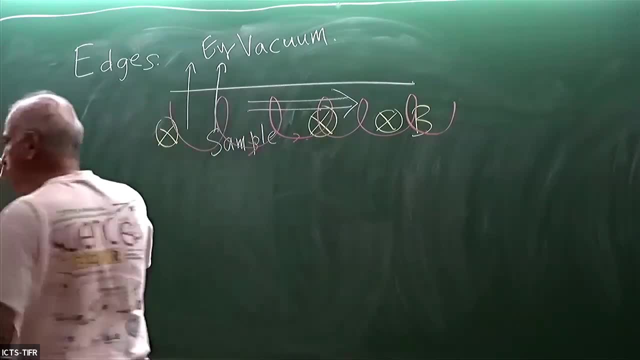 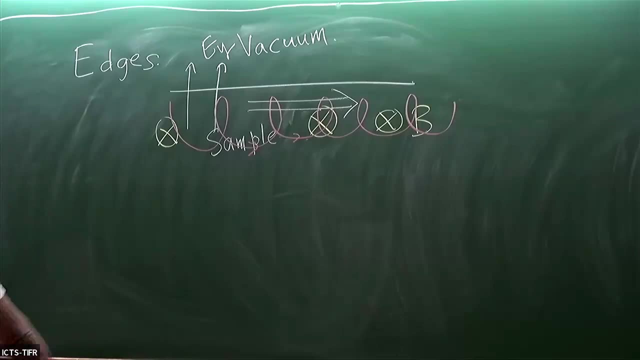 So once again, I'm going to go into this tube picture, right, But then I'm going to put infinitely hard walls at the edges of the tube. Let's focus upon one edge of this tube and then here's. here's how it looks. So this is V equals infinity. This 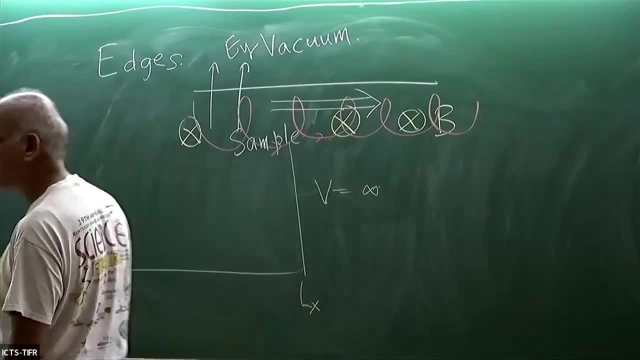 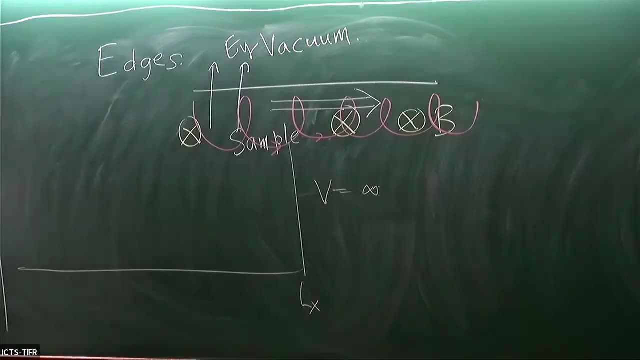 is the edge, and let's say, this position is L sub X. Okay, so now along here, I have all these guiding centers, right, Because L sub Y was finite. So there's, there are all these little guiding centers. So let's say this: 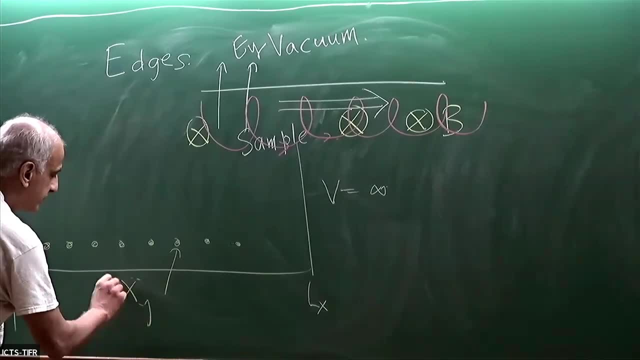 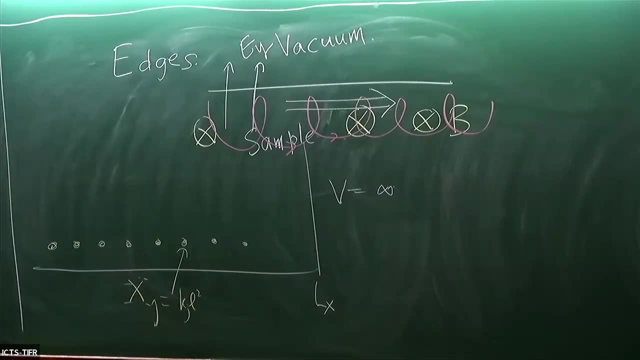 guy is J. So there's some X sub J, which is K- L squared, K sub J- L squared. Okay, very good, Now you go back to that Hamiltonian sitting there. So there's a harmonic potential that is centered at K- L squared. 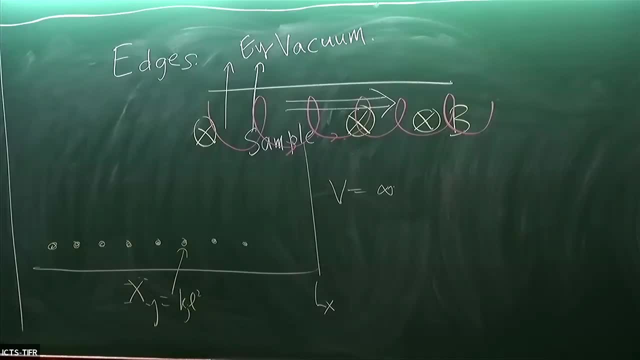 Now deep inside the sample. Okay, supposing I'm at this guiding center, the electron feels some harmonic potential that looks like this: Okay, and it's wave function, if I'm in the lowest Landau level, is going to do something like this. It doesn't even go to the edge. 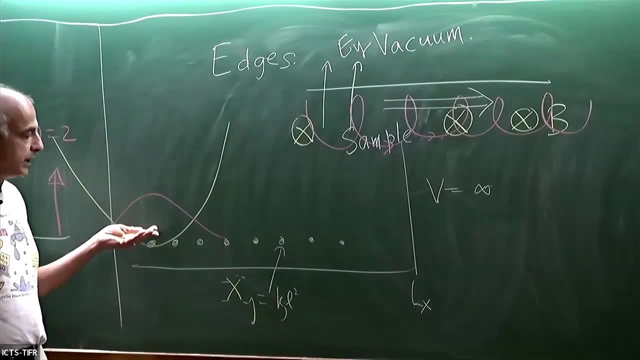 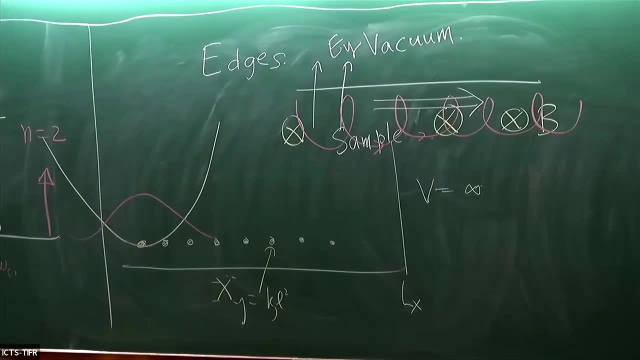 It doesn't feel that infinite potential. So here the energy is going to be the same as what was in the bulk, It's just going to be N plus a half H bar Omega As the electron, as the guiding center, approaches the edge. Suppose I'm here, Then you see it. 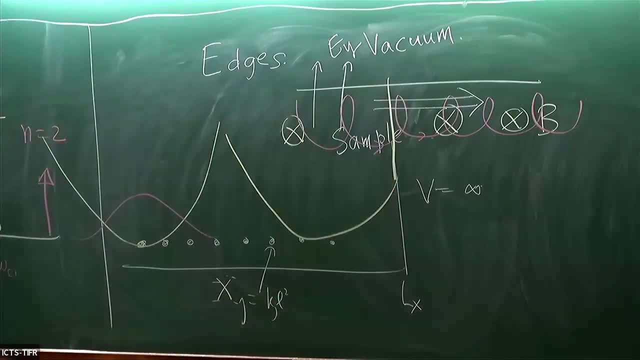 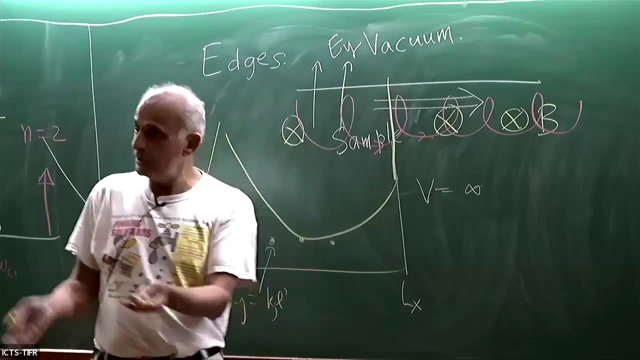 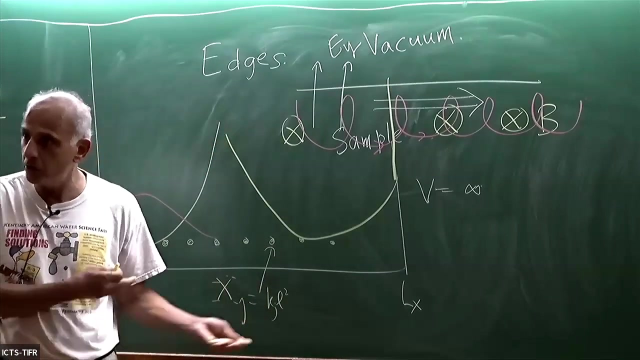 does this, And now this electron is experiencing a different potential. Obviously, this potential is increased, So the energy must have increased right from its bulk value. How much, we don't know. You'll have to solve the differential equation to find out. But 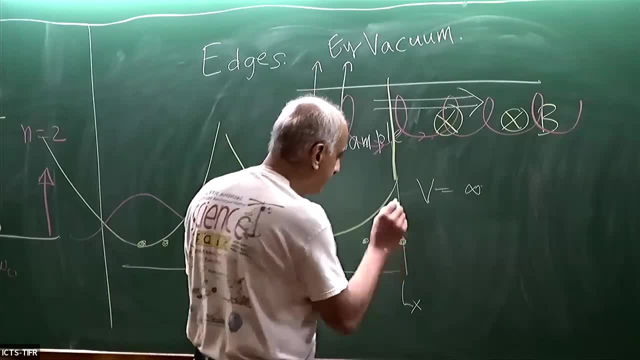 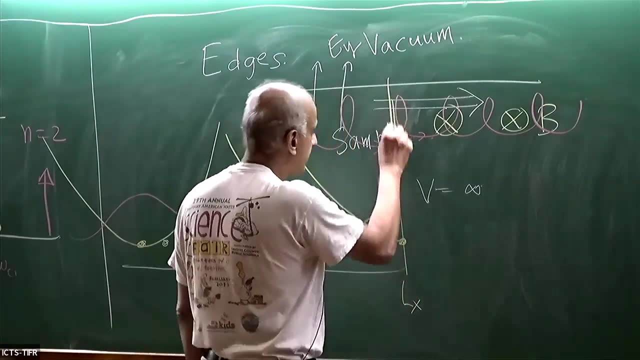 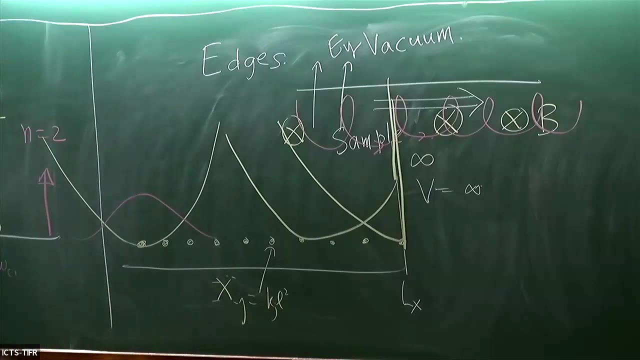 let's keep going. So let's say there is a guiding center right here, at the very edge. there The harmonic oscillator potential looks like this: Okay, it's half a harmonic oscillator, and then there's infinity on the other side. That we know how to do. 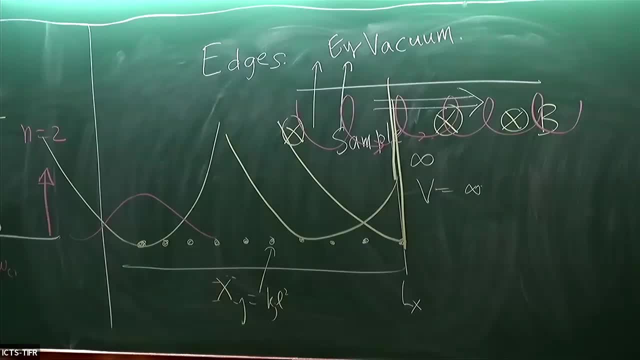 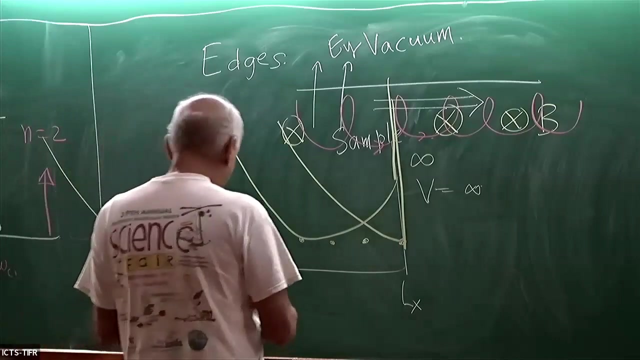 We know how to do this. How do we do this? Variational principle says somebody, Okay, Somebody else. I want an exact answer. Just take the odd wave function. Odd wave functions, Right, Okay, great, So we know for here. now let me draw this, this picture now. 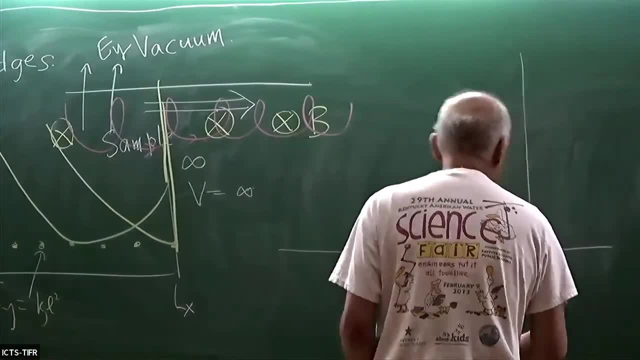 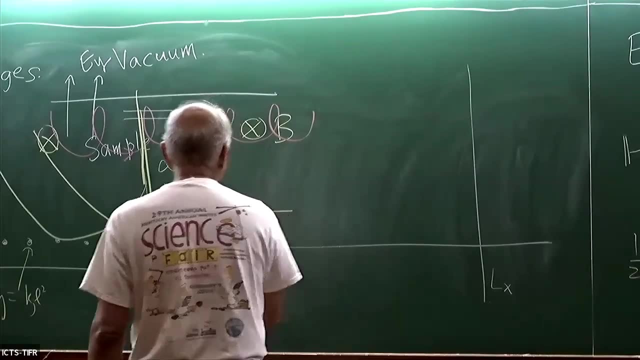 Okay, So this is else of X, and now I'm going to draw the energy as a function of guiding center. Okay, so deep inside the bulk, The n equals zero land, our level is one half H bar Omega, and it remains like that. okay, 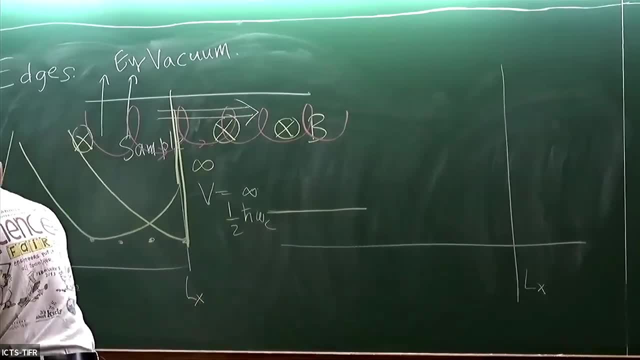 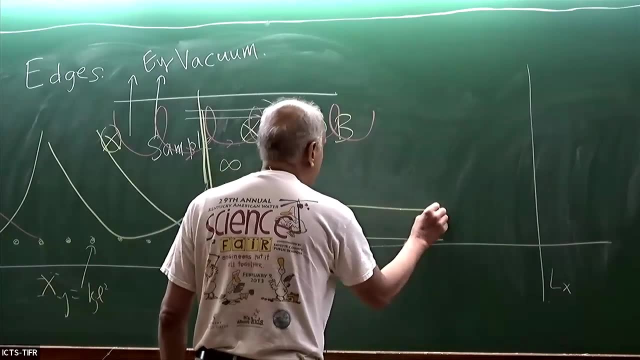 And then there is. so let me actually draw it slightly better. Let's say: this is 1 1⁄2 h power omega c. this is 3 1⁄2 h power omega c. this is 5 1⁄2 h power omega c. okay, 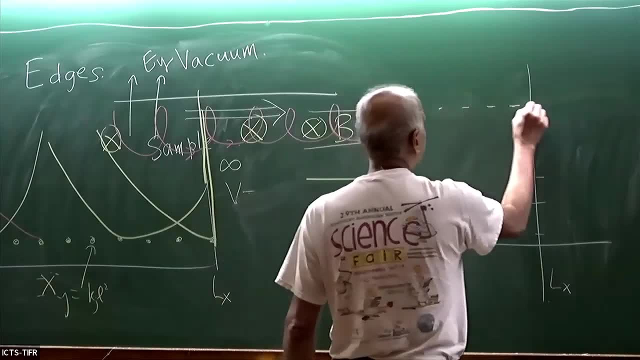 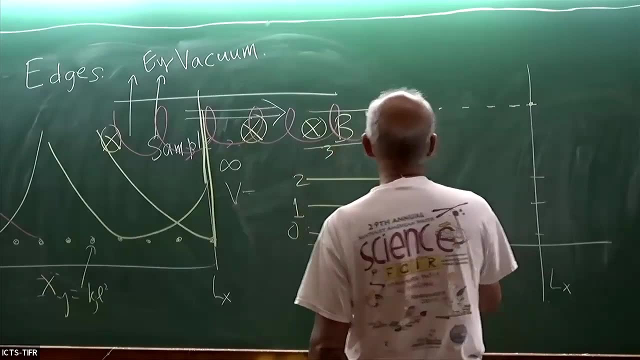 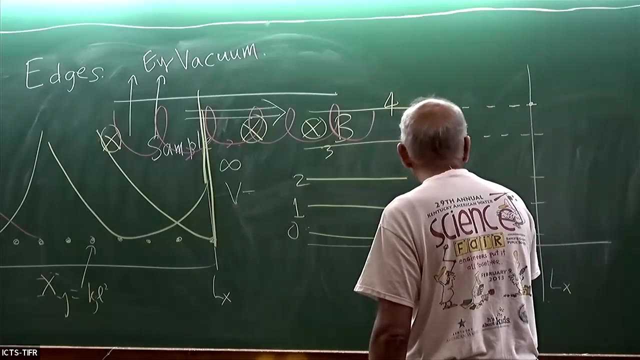 And this is 7 1⁄2,, this is 9 1⁄2,. this is the n equals zero. one, two, three and four landowners. okay, All right, very good. So I claim that this guy should end up here. 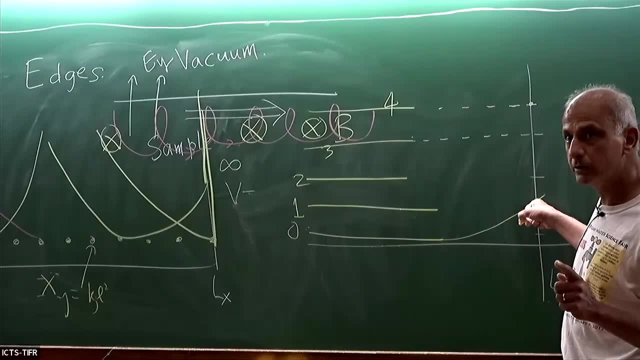 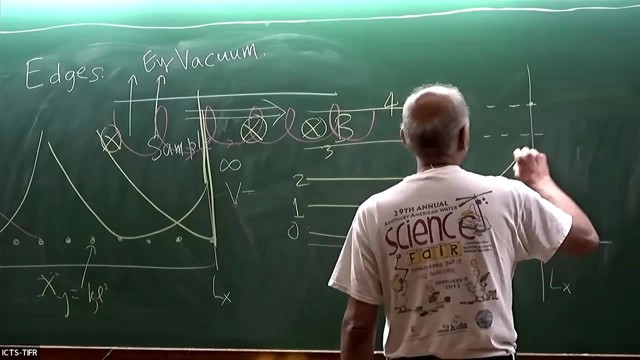 because this n equals one landowner. level is odd, it's an odd wave function. In the odd n are odd wave functions. the even n's are even wave functions. So this guy should go here, okay, This guy should go here, and so on. 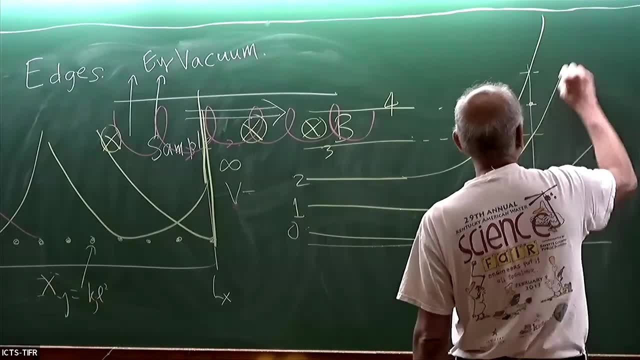 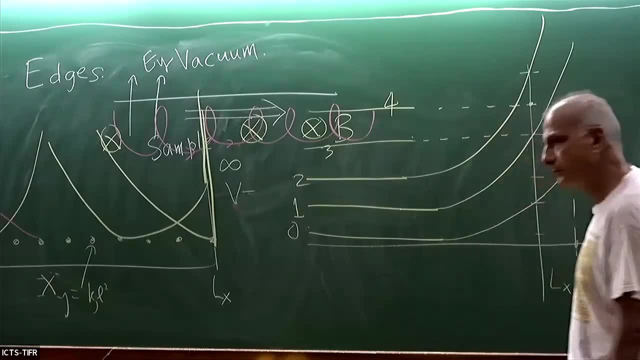 That's what should happen. Now. let me draw it like that. Now I've drawn these guiding centers over here. There is a guiding center here, right? What about this guy? That comes back to your question. there They're slightly different guys, okay. 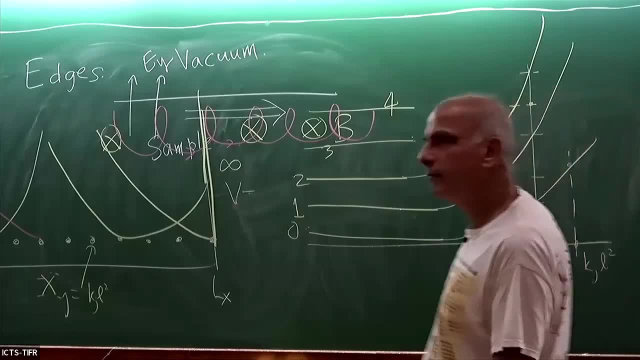 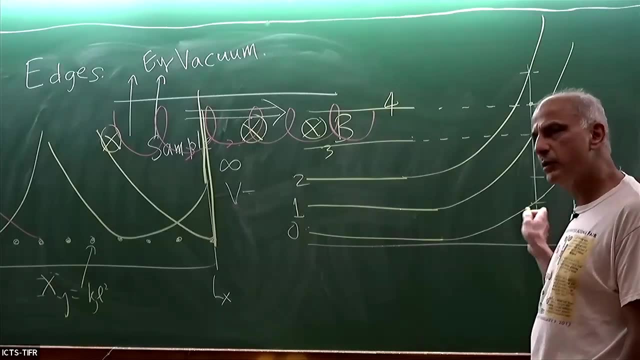 Does that guiding center even exist? How about this state here, which is, you know, the x sub j is sitting outside the sample? Can I have a wave function corresponding to that? Some part of the potential is definitely there, because if I draw my potential here, 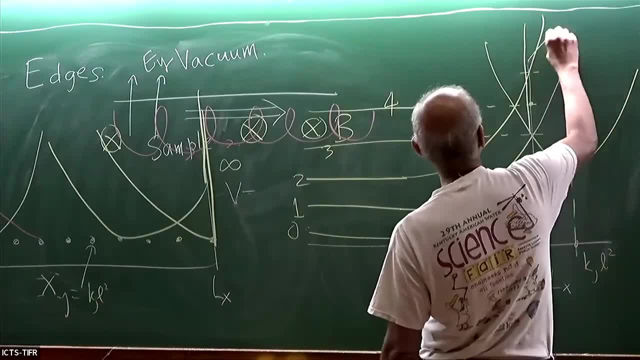 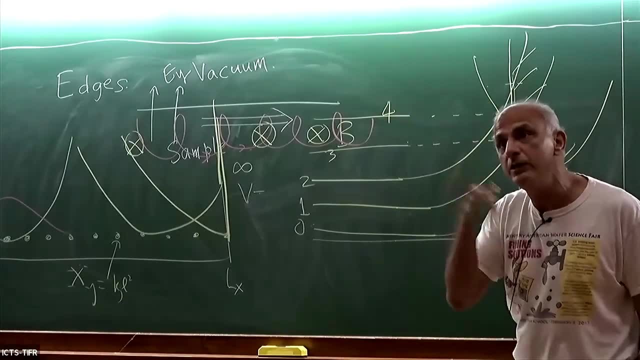 it will look something like this: and this: right, This is infinite. that is not infinite, So the wave function lives here. So, even though the guiding center is here, the wave function actually lives inside the sample, but its energy is very high. okay, 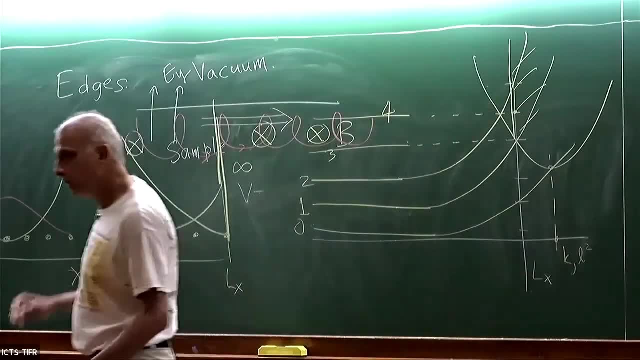 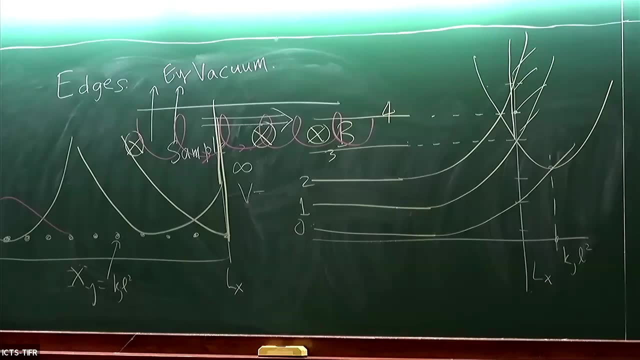 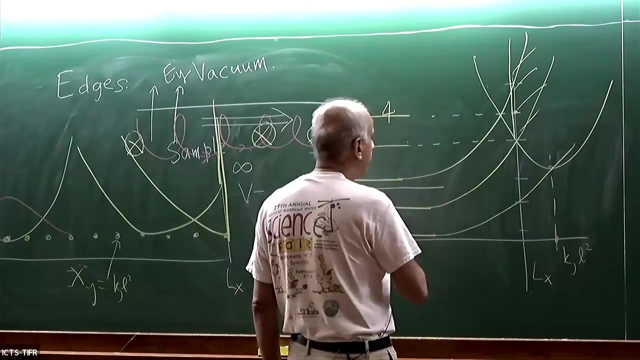 Good, So now let's imagine. so here's my spectrum, including the edge. Okay, now let me imagine that I have a system- Again, I'm forgetting about spin, So let me imagine that I have a system that, in the bulk, has two full Landau levels. okay, 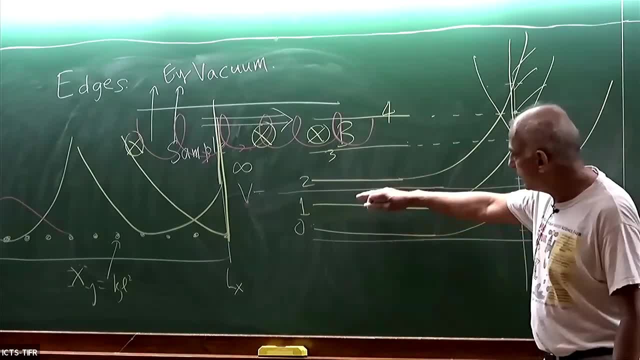 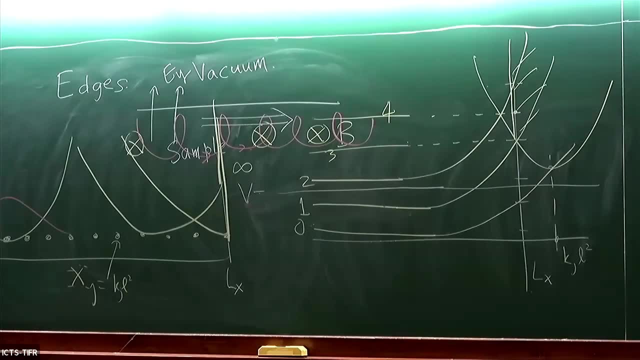 N equals zero and N equals one. And I draw my chemical potential somewhere here And I ask myself: what do I see at the edge? Well, if I want to add a charge or remove a charge from the system through my contacts, okay. 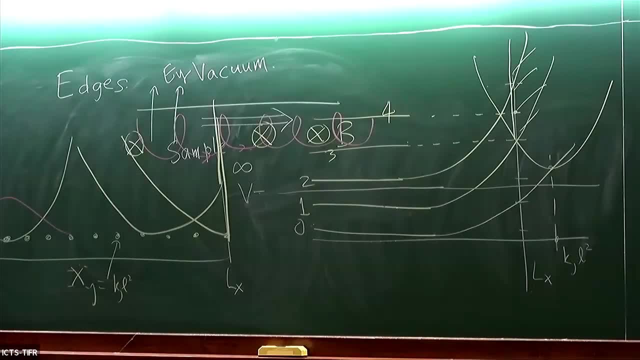 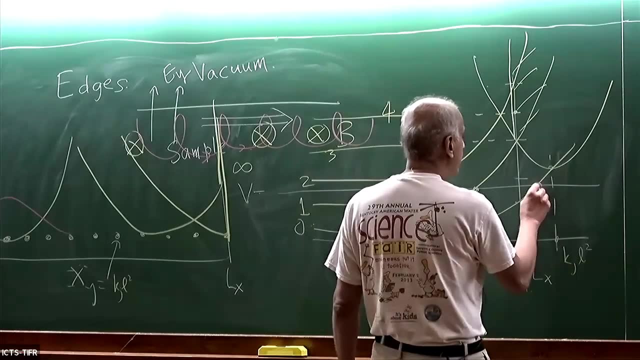 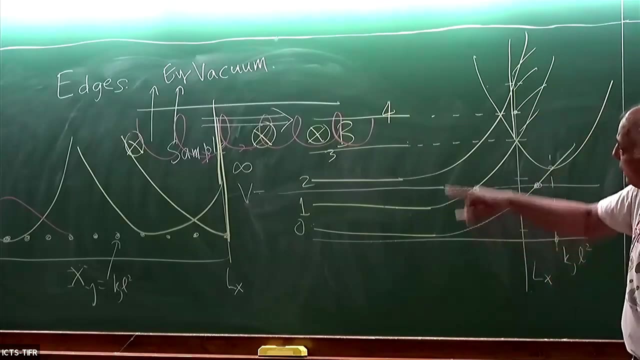 I have contacts around the edge. I want to add or remove a charge. I can do it at zero energy only at these points here. this guy and that guy, This guiding center is sitting outside the sample, but of course the wave function is still inside, right? 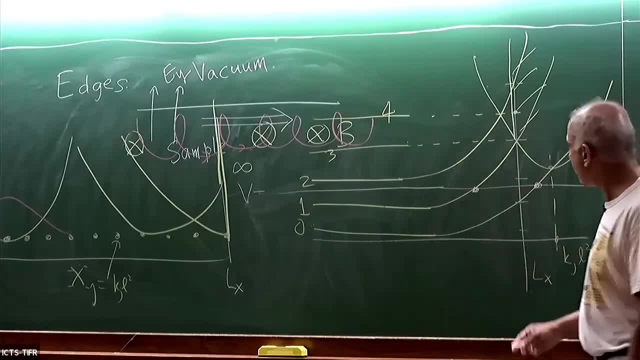 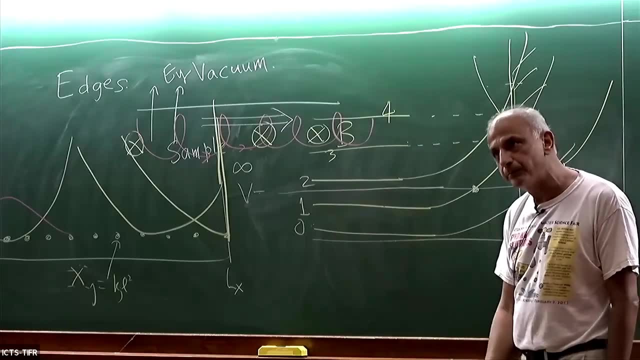 In the way that we just discussed. Okay, so now there are two points where the chemical potential intersects the spectrum: the filled part of the spectrum. So all this is inside the spectrum, right? Okay, so now there are two points where the chemical potential intersects the spectrum: the filled part of the spectrum. 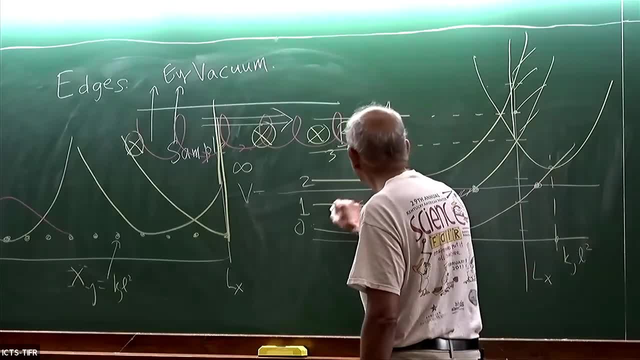 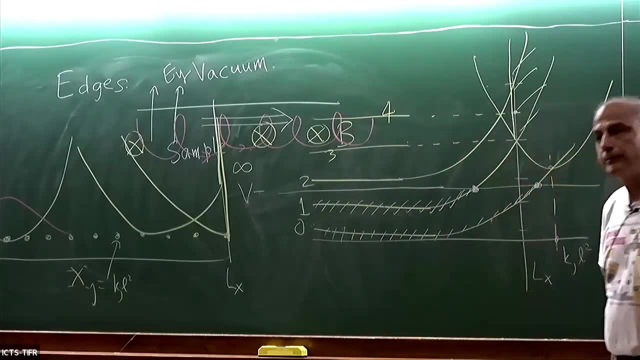 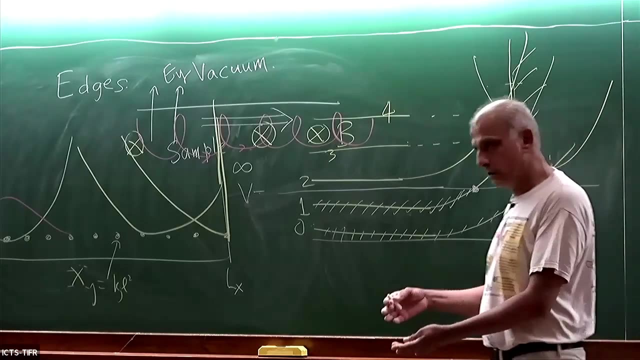 So all this part will be full in the system, These guys will be occupied and those guys will be empty. If I want to add a charge, I can add it here and I can add it there. So any conduction that happens in a quantum Hall system. 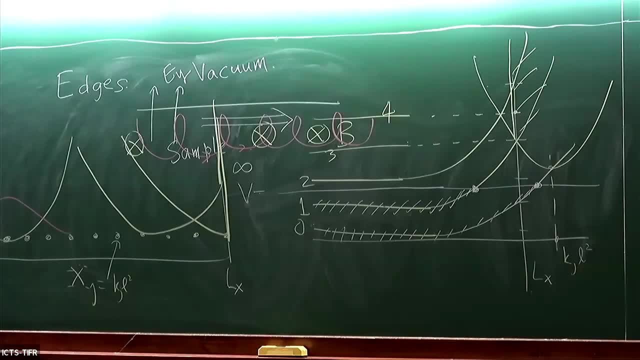 happens only at the edges. So in the insulator it's a sorry, in the bulk it's an insulator, at the edge it's a conductor. This is an example, one of the simplest examples, of a very general phenomenon. 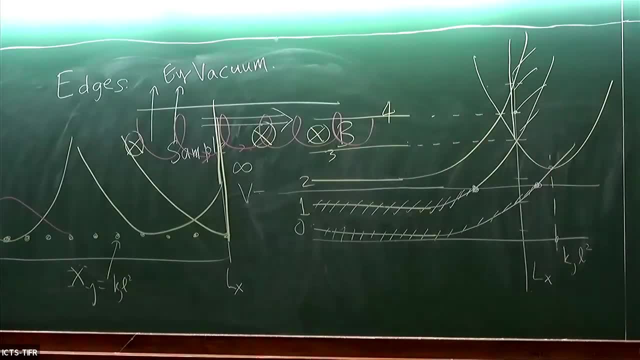 which you probably heard of at least. the buzzword is topological insulator. So this is the world's first and simplest topological insulator. So it has, it's insulating the bulk. there's a gap to all charge excitations. 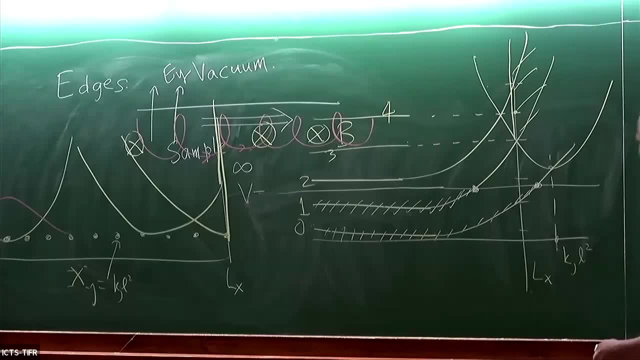 whereas at the edge there are necessarily gapless charged excitations. Okay, All right. Now somebody asked about thermal conductance. Yes, Because these edges, they transport charge, they can also transport entropy. So there is thermal conductance on these edges. 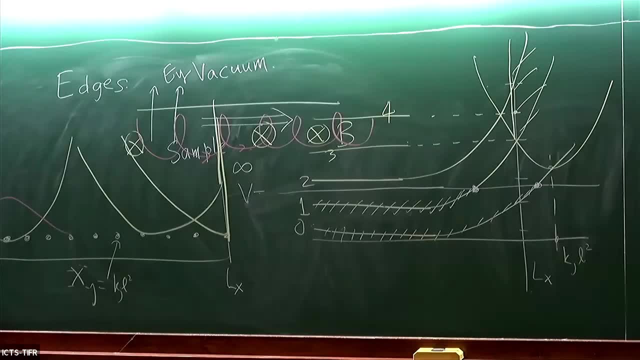 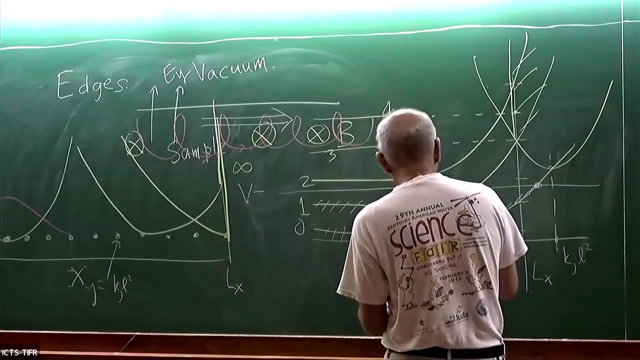 Yes, you are. Yeah, Yes, Otherwise there is a tiny gap. Yeah, Yeah, Did everybody understand what you all said? So there is a spectrum here, right? And as long as L-y is finite, there are these little guiding centers here, right? 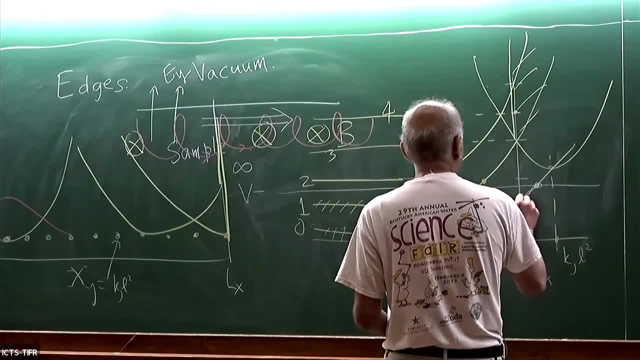 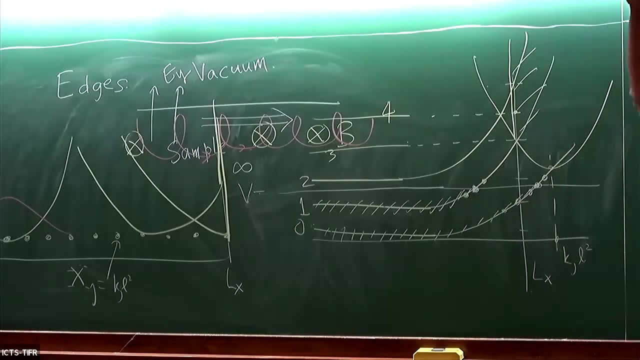 There's one here, there's one there, You know, one here, one here, one here, one there. So he's saying that there's some tiny gap here. whereas you make L-y bigger and bigger, this gap shrinks and the spectrum becomes continuous. 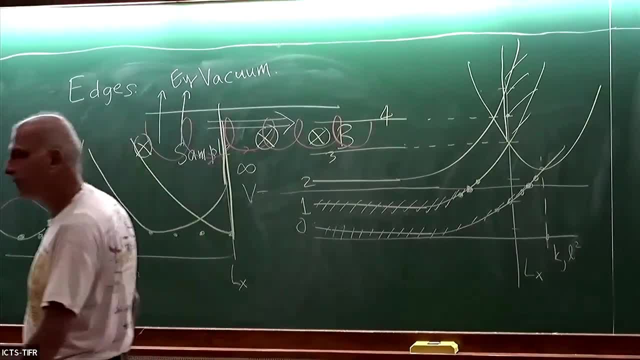 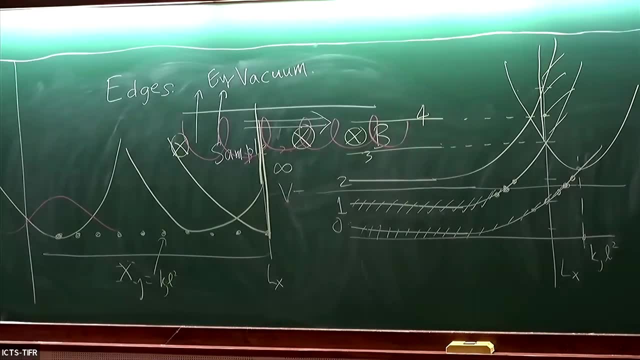 in the thermal architecture, in the thermodynamic limit. okay, This is true in a so-called metal as well, right? Because even in a metal there are various, you know, there's a Fermi surface and so on and so forth. 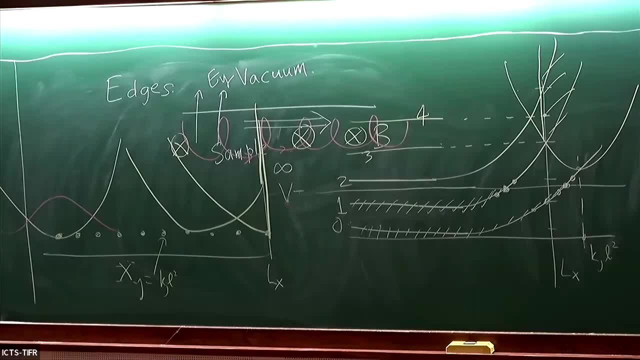 but then the K are all discrete in a finite system, And so in order to properly define a Fermi surface, you need to go to the thermodynamic limit. Okay, good Questions about the edge. So this is sort of the world's simplest edge. 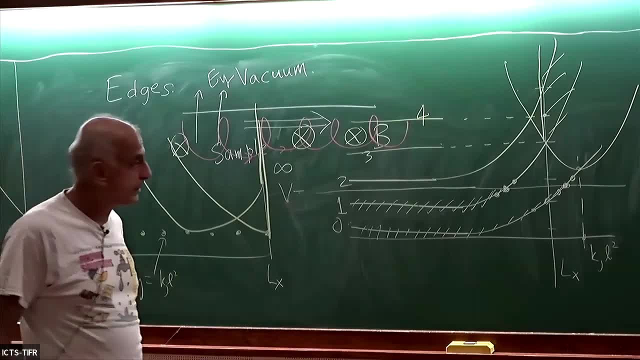 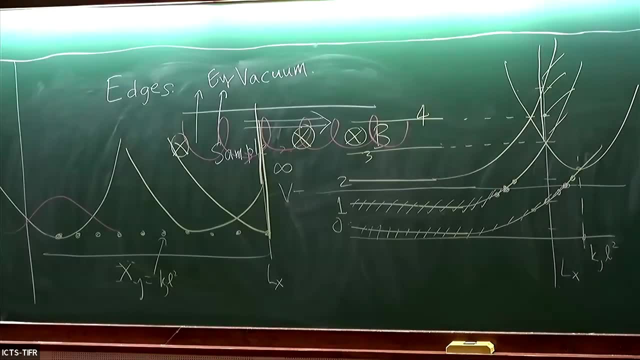 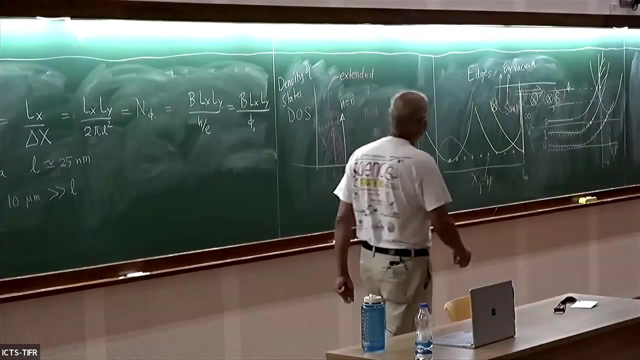 This was first discussed by Halperin, but Halperin in, I think, 1981 or 82 or something like that. Yeah, Very good, very good. So here's the issue. So if I put my chemical potential in, you know, 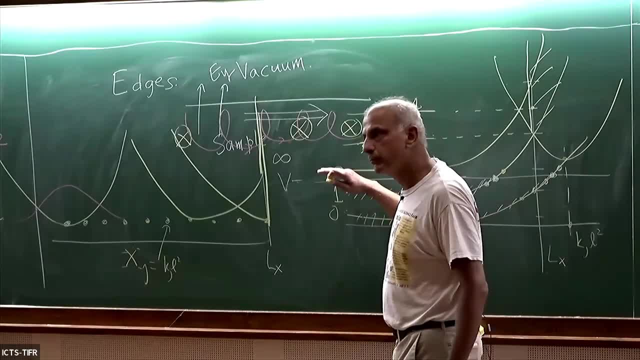 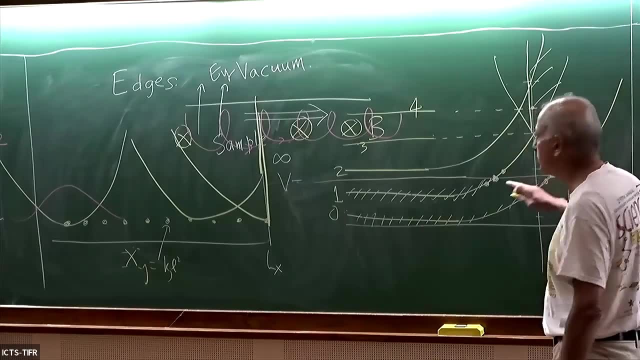 in the bulk between, let's say, N equals one and N equals two. and then I ask how many states are contained? right, You will see that all these states, even though they exist, they're not filled, okay. So therefore, the number of states. 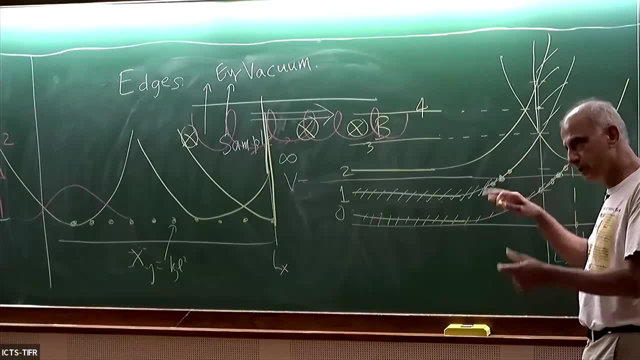 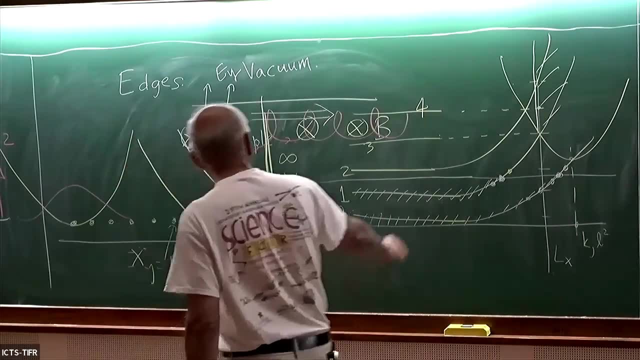 of course the details of the edge will change the states by a few, but they will not change it thermodynamically, okay. So even though these states are there, they're very high in energy, so they're not filled. So I'm counting only the filled guys. 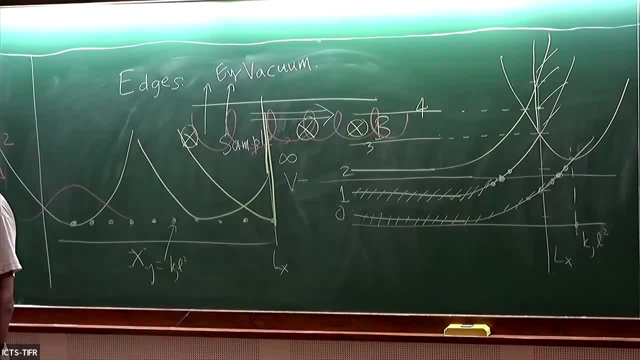 Okay, Yes, Yeah, Yeah, Yeah, Yeah, No, Because I'm taking periodic boundary conditions. I'm thinking of a tube. Okay, in a real system, of course it will vanish, But typically what happens is that in all this, 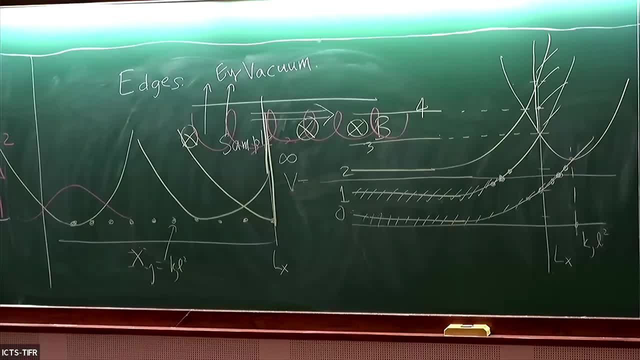 in the thermodynamic limit limit, while or somebody showed this in the in the 1930s- the thermodynamic limit, the density of states does not depend on the boundary conditions. okay, so the, the, the number of states per unit energy, there will be some small adjustments depending. 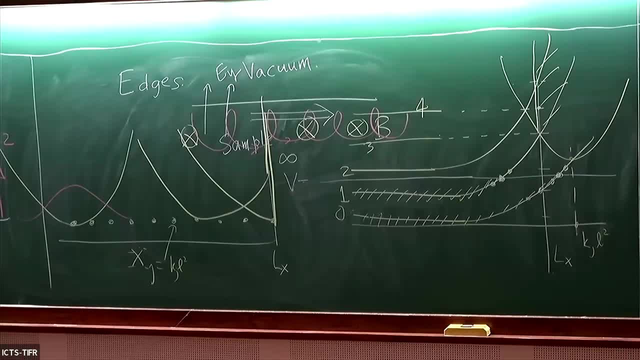 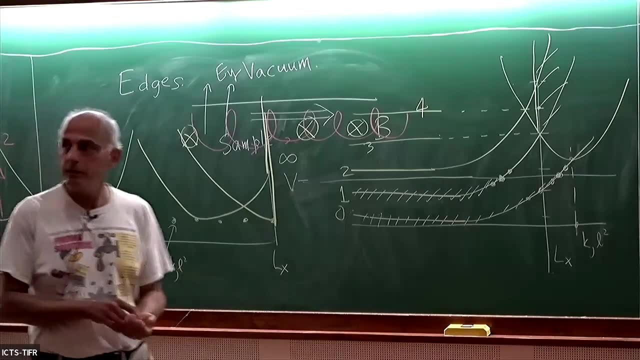 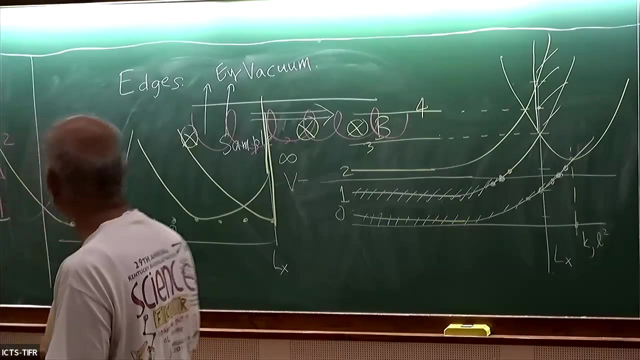 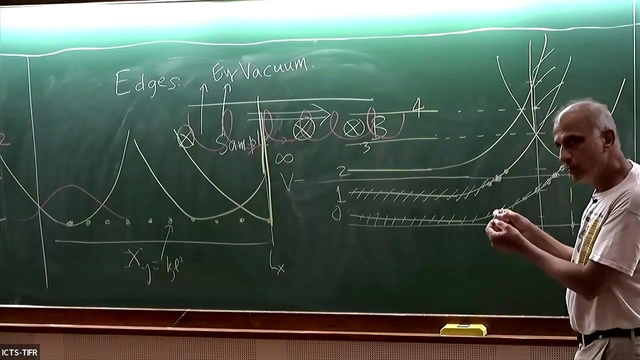 on the boundary condition, but the, the degeneracy will not depend on the boundary in the thermodynamic limit. all right, other questions? yeah, sorry, why did I call it gapless? because as Y, L, Y goes to infinity, these states get closer and closer right, and therefore I can add or remove a charge with. 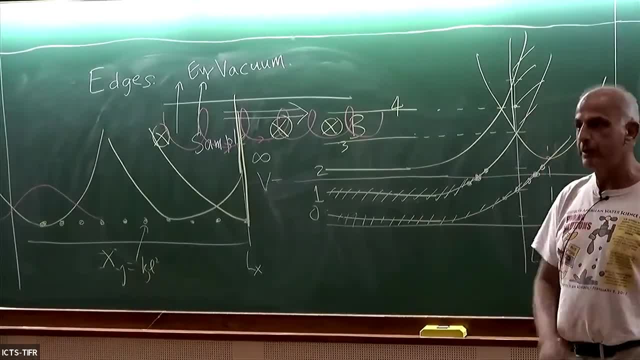 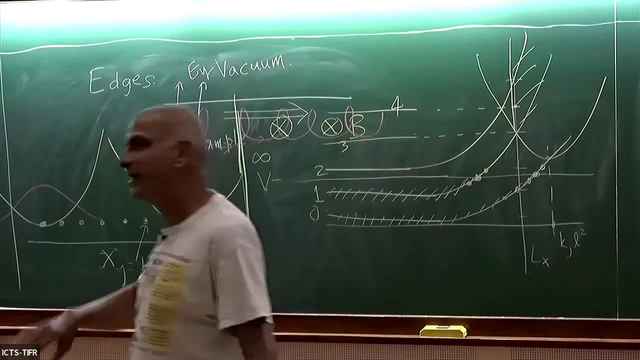 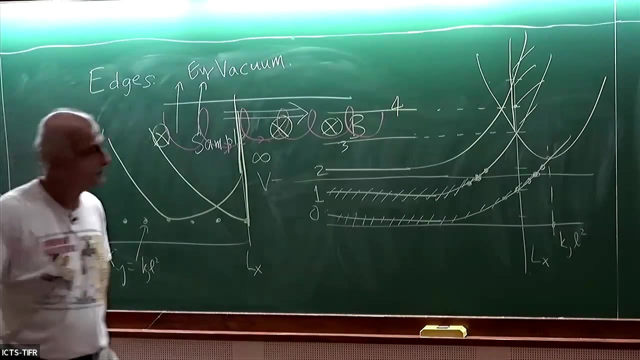 arbitrarily low energy on the system. that is why it's gapless wait. you've had your quota of questions for now, okay, so I want to finish the disorder and then, once I finish the disorder, then you ask a question. so remember, all right. so now in the last five minutes or so six minutes, let me talk about disorder. 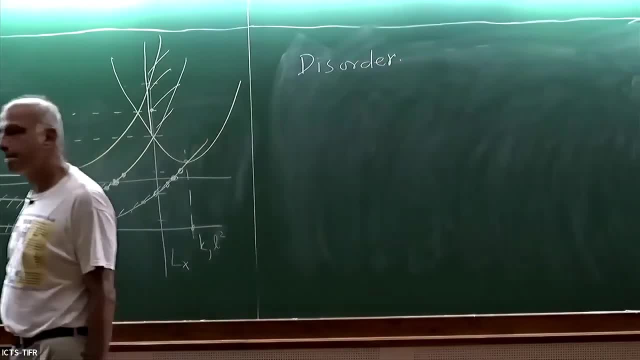 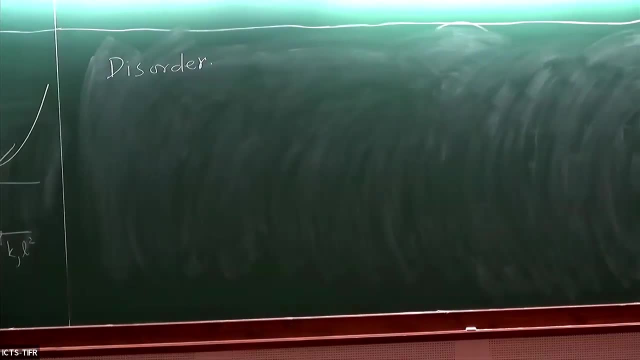 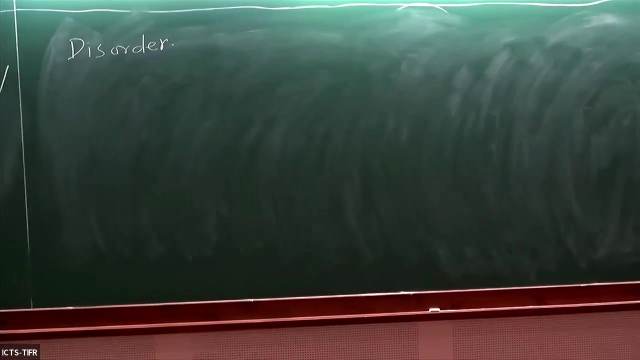 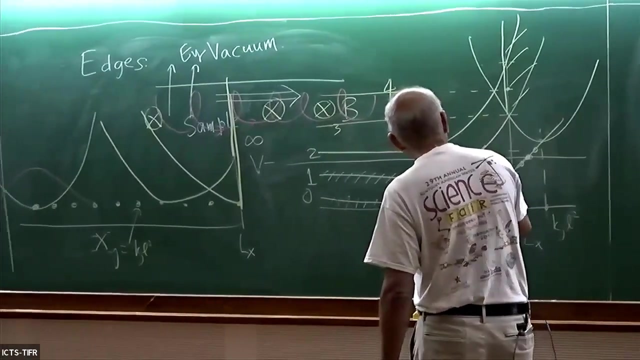 yes, very good, very, very good point, so very good. so the analog of this semi classical argument that I just gave you about why the thing moves along the edge right, this is cross B drift, I guiding center drift, the. the analogue of that here is fact that this guy has some BE by DK and this is a velocity in the Y direction. 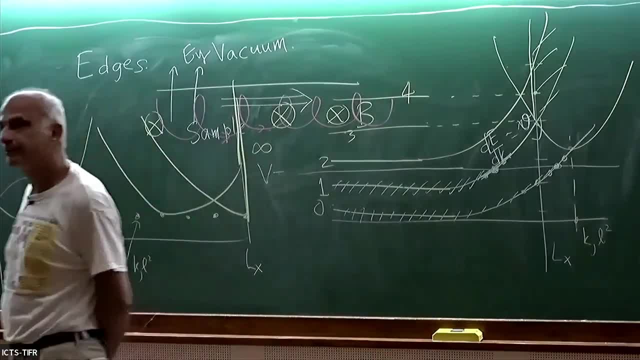 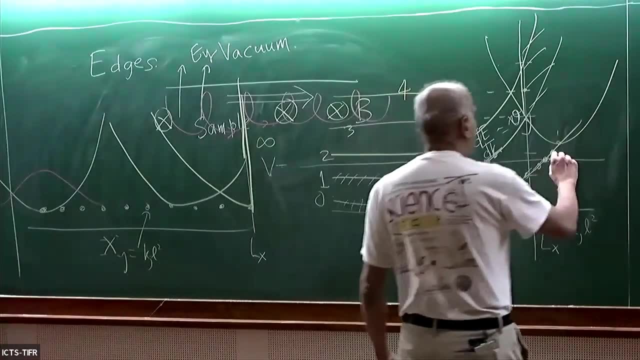 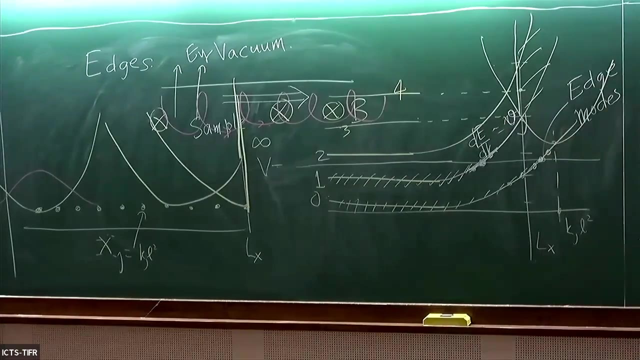 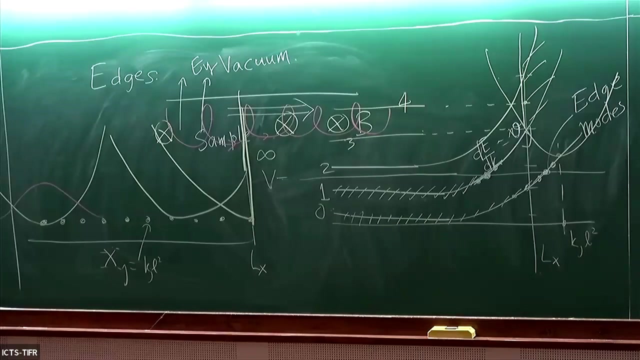 because K is a momentum in the Y direction, So there is a velocity to these edge modes. These guys are called edge modes, Okay, So they carry charge and they also carry entropy. They can carry heat. All right, Let's talk about disorder. So I'm going to take a limit where B is very large. 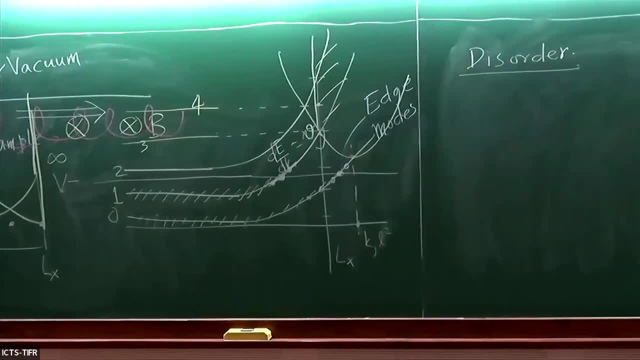 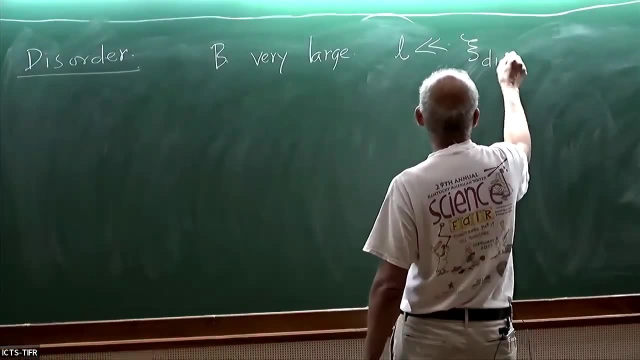 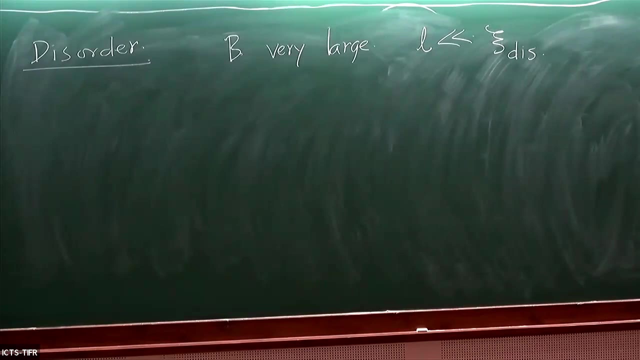 Okay, what do I mean by large? Large compared to what? Okay, what I mean is that this magnetic length is much, much smaller than the correlation length of the disorder. So the disorder has some scale over which it varies. I'm going to call that C disorder. 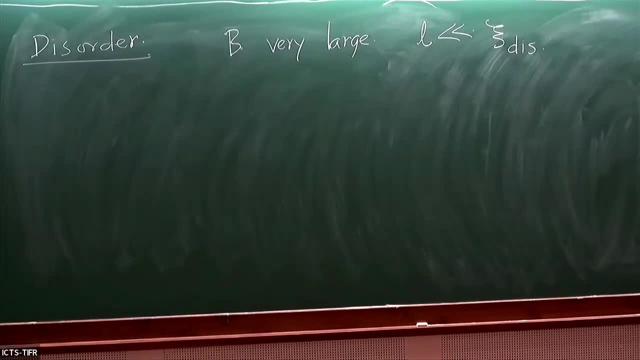 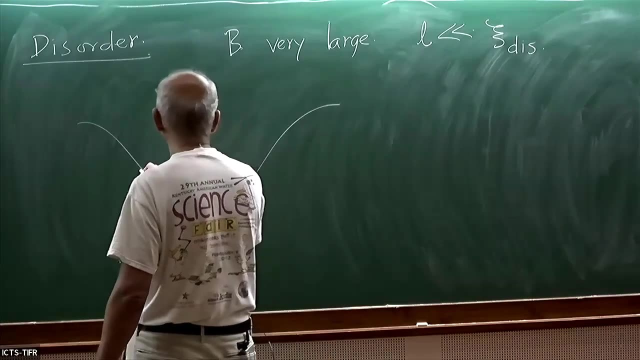 Then I can think of a solution. I can think of the disorder as being very smooth, Okay, on the scale of L. So let me draw a particular picture, Okay. so let's say I have a minimum of the disorder. It looks like this: 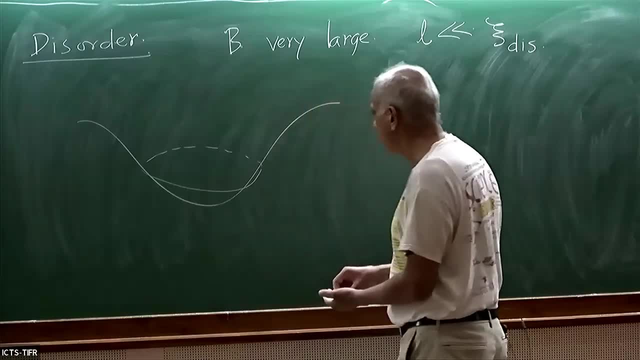 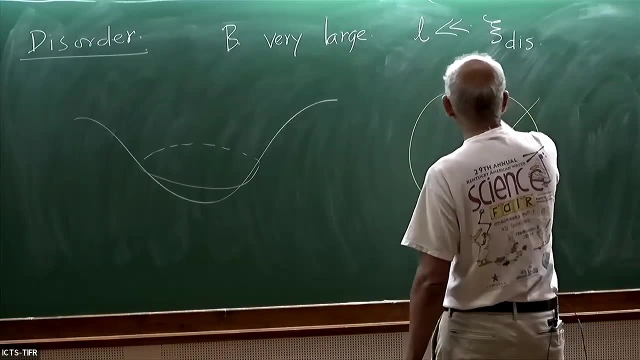 I'm going to look at it from the top. If I look at it from the top, what I will see is that the electric field- So I draw it like that right. The electric field is pointing inwards, right, Okay? 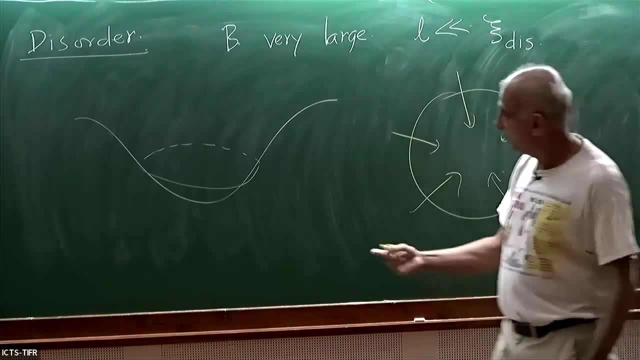 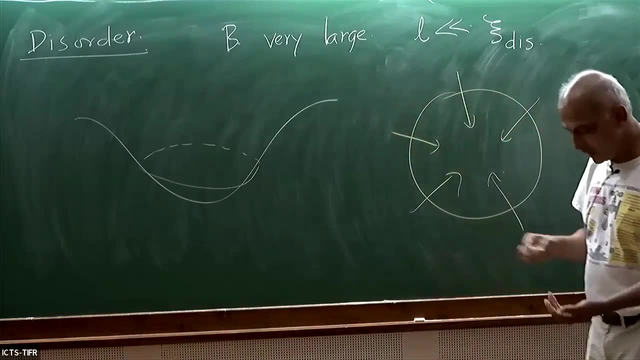 Now my electrons are doing guiding center drift right Previously, when there was no disorder, they were undergoing cyclotron motion. So let me think semi-classically right. So what's going to happen is that these electrons- an electron that's sitting here- will do something. 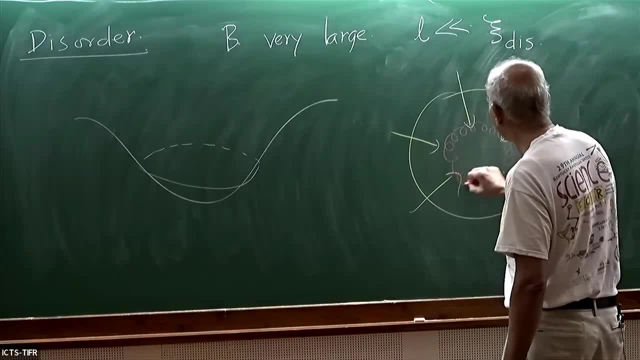 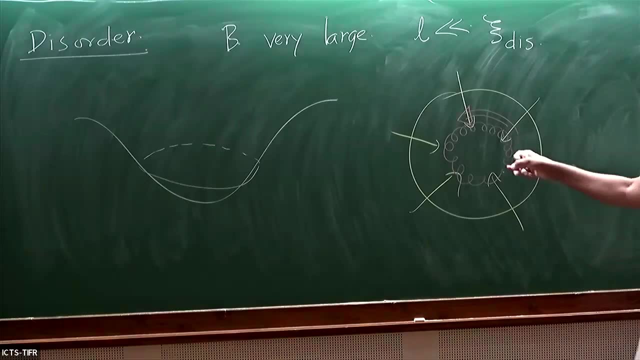 like you know something like that. So, overall, the direction of rotation will be like this, And I'm using this fact by saying that this cyclotron orbit size is very tiny compared to the size of the potential itself. That's why I'm using this condition. okay. 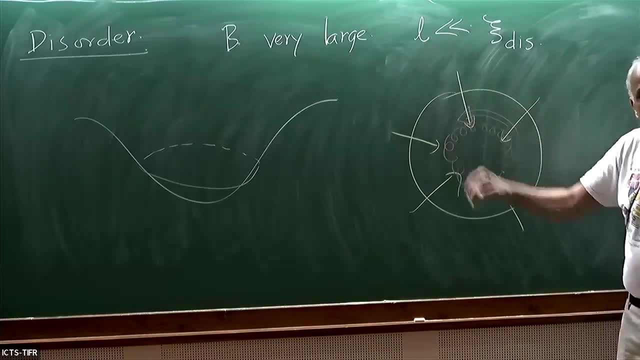 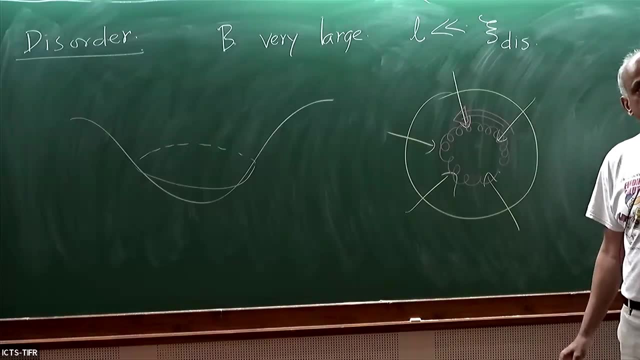 The size of each of these little squiggles is little l. The scale of variation of the disorder potential is that which is this? Is this clear, Okay? So what I'm going to do is I'm going to do some kind of Bohr-Sommerfeld quantization. 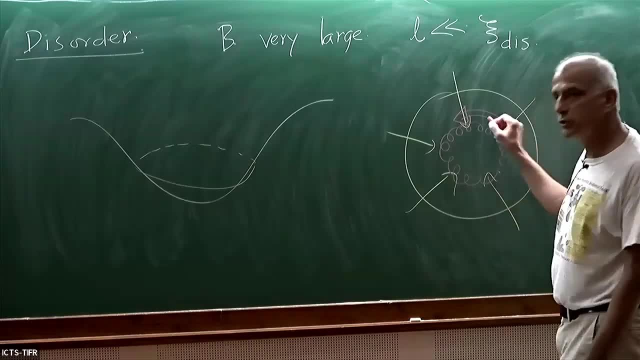 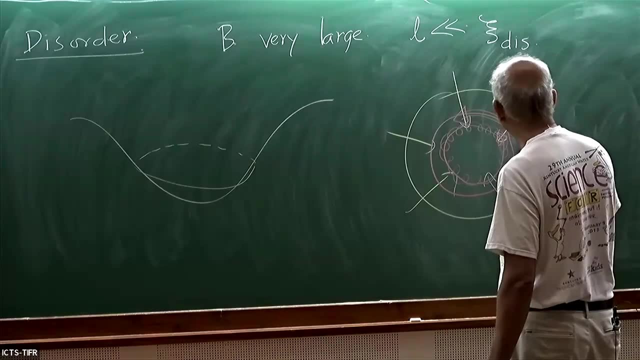 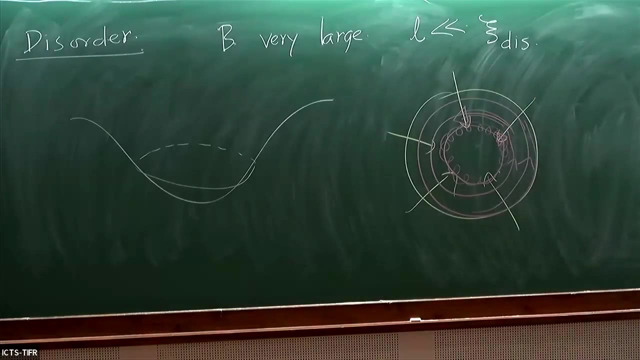 So I'm going to quantize this periodic motion, I'm going to draw some orbits like this. Okay, So let me draw this orbit here, there'll be another one here, there'll be another one here, and they will roughly follow the equal energy contours of this disorder potential. 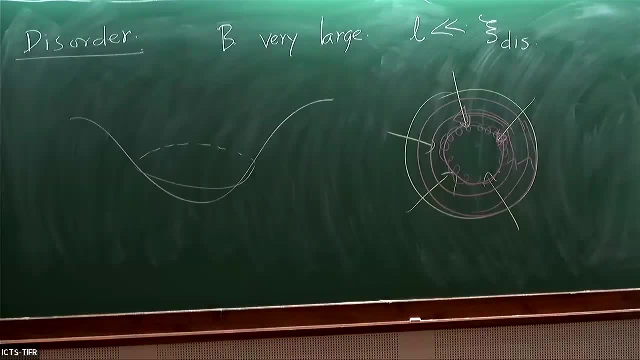 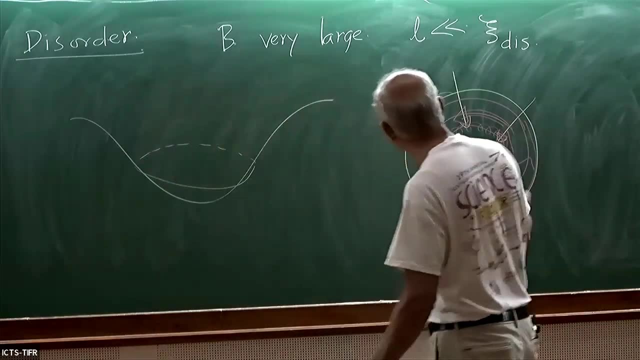 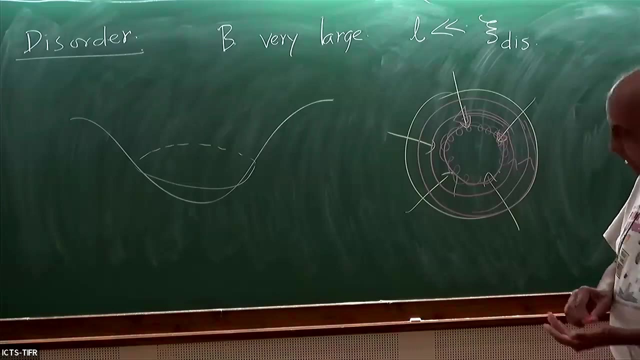 right, Because E cross B drift goes perpendicular to the electric field, which means it goes on an equal potential contour. okay, It's going on these equal potential contours, So that's near a minimum. Okay, We all know that near a minimum charges get localized. but in quantum Hall systems, something? 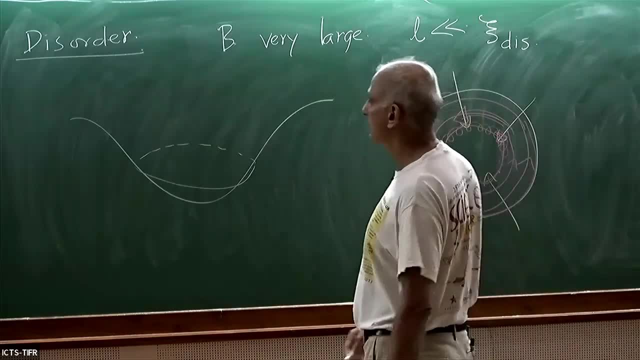 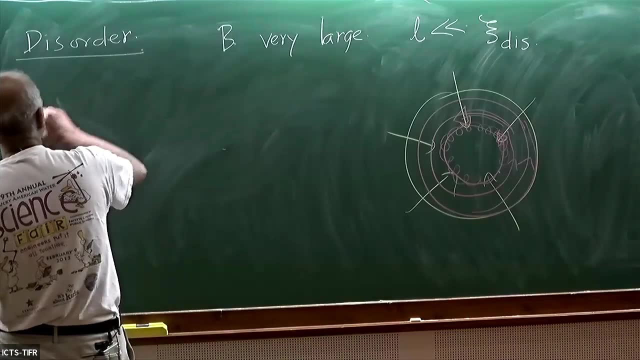 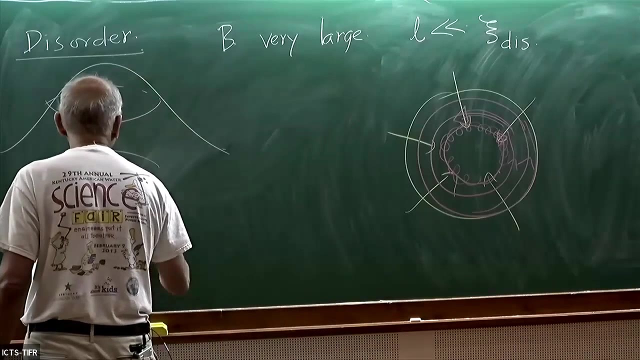 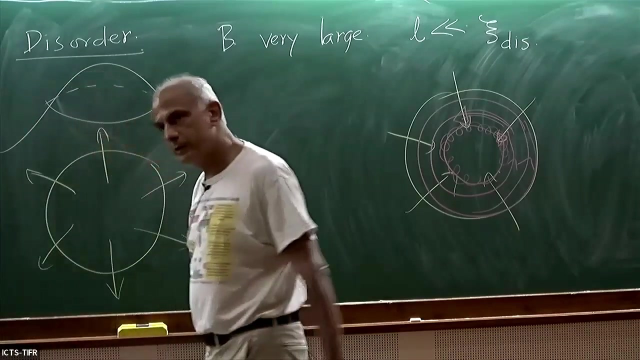 else happens. Supposing I now take a maximum, let me draw it here, use my space more efficiently. Supposing I draw a maximum like that: Now my electric field is pointing outwards, However, guiding center drift still happens and instead of going this way, the electrons 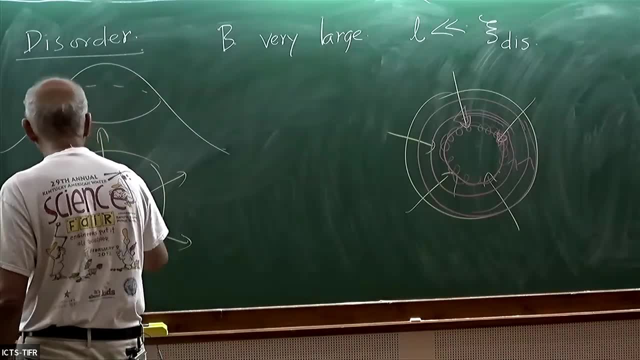 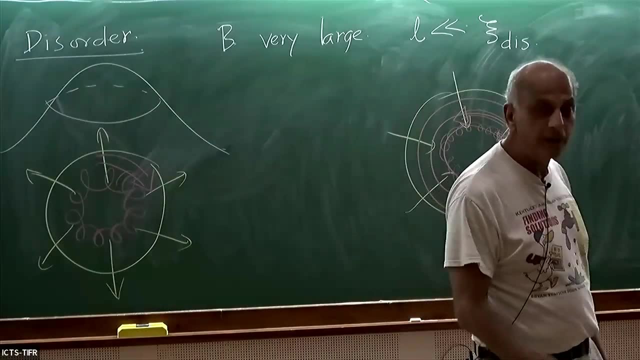 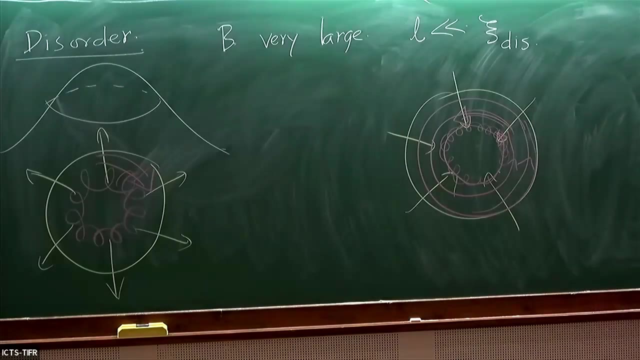 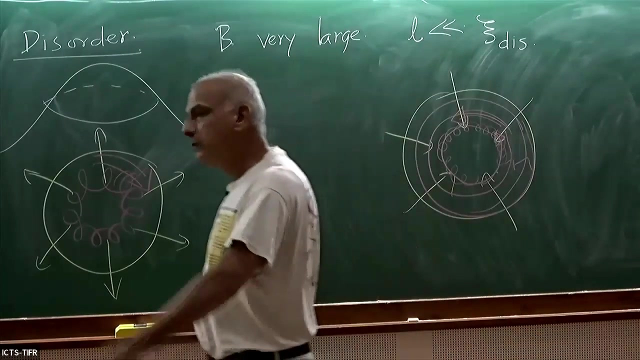 simply go this way, That way, They're still localized. So here's the funny thing about quantum Hall systems: disorder localizes orbits both near minima and near maximum. okay, So now let's think of a landscape. Now I'm going to ask you to imagine: okay, there's some landscape, there's some holes. 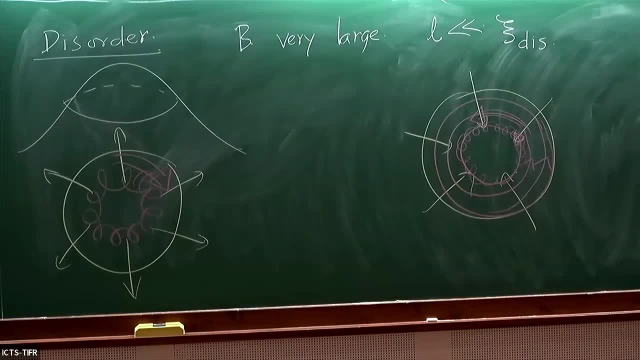 there are some big lakes, there are some hills, there's some mountain ranges, there's all kinds of stuff. Okay, Now I start filling the system with electrons. So first of all they fill the bottoms of all the lakes, right? 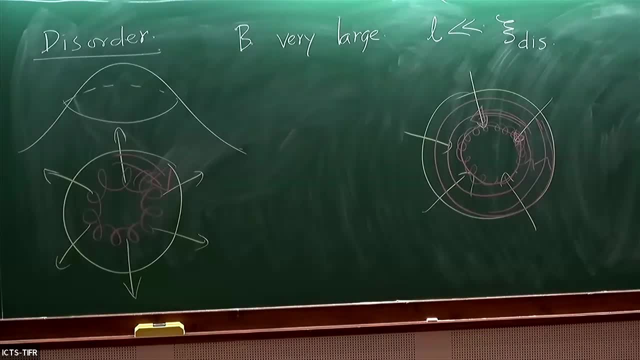 The deepest lakes get filled first, And then, at that point, you can walk from one side to the other side of the sample right By foot, because there's a land bridge across the entire thing. The lakes are all isolated. Imagine that you fill it almost completely. 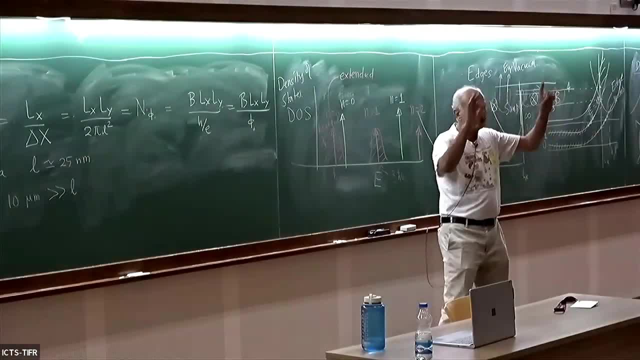 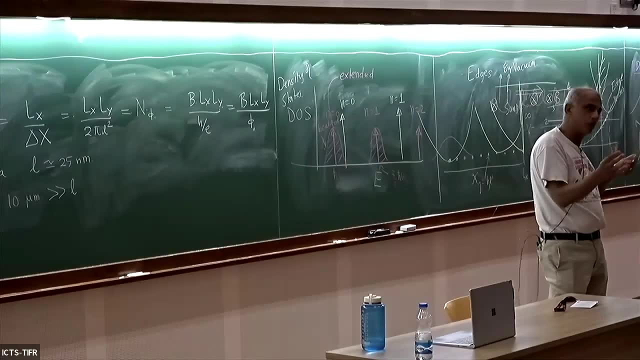 Then you have a sea of electrons and there are some islands that are sticking out of the sea of electrons. Now you can take a boat. right, You can take a boat. You can't walk across, but you can take a boat. 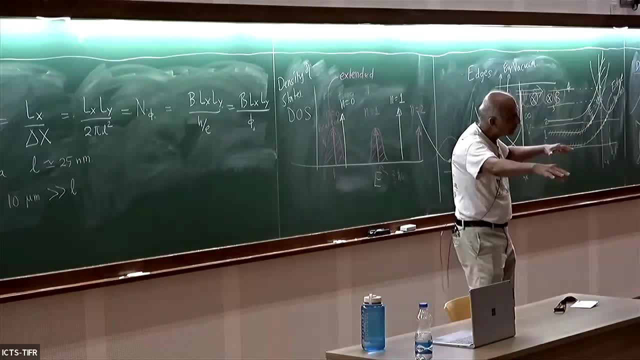 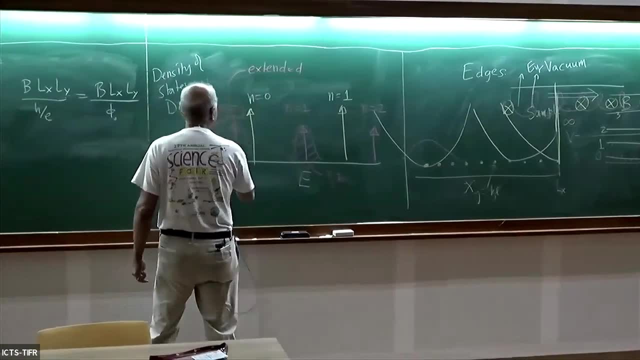 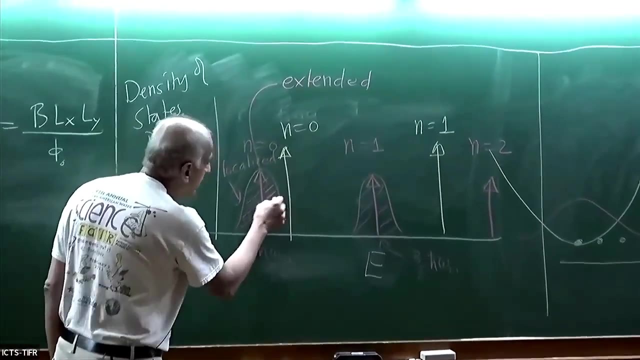 So at some point between when I can walk across and when I can take a boat across, there will be a critical point. That critical point is this state here, this extended state. Okay, So the states here are localized below the extended state. the state above are localized. 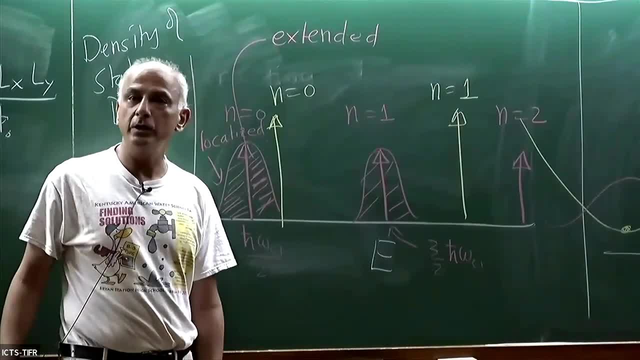 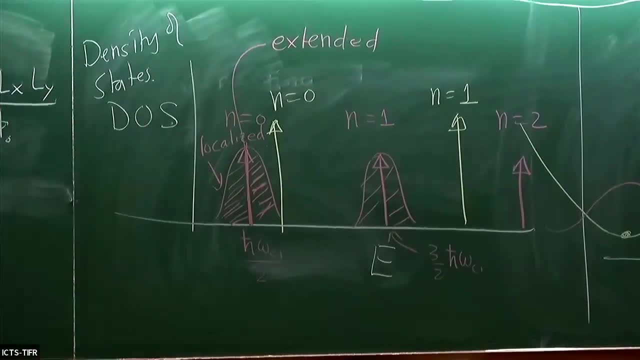 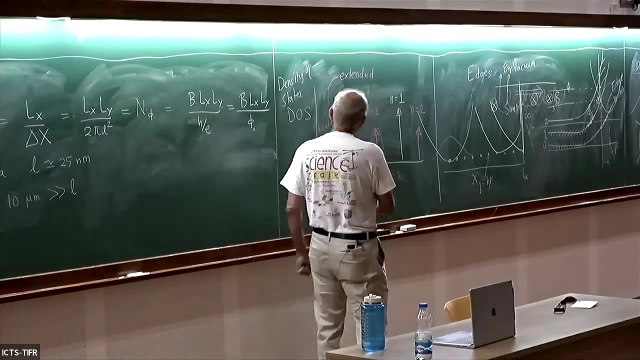 because they're localized around the maximum of the disorder potential as well. But the state right here, With that boundary, that interface between the states that are localized at minima and the states that are localized around maxima, that state is extended. So the picture is the following. 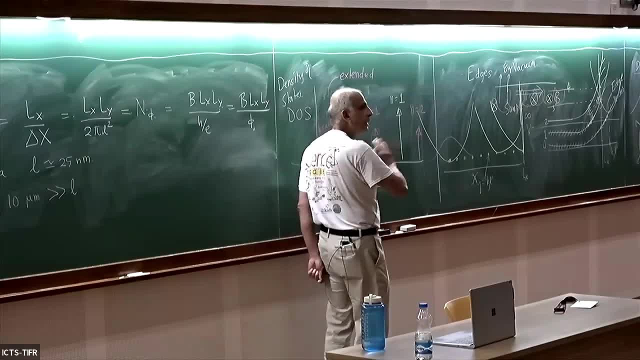 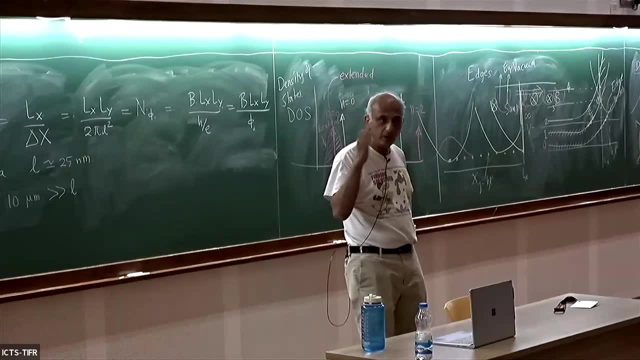 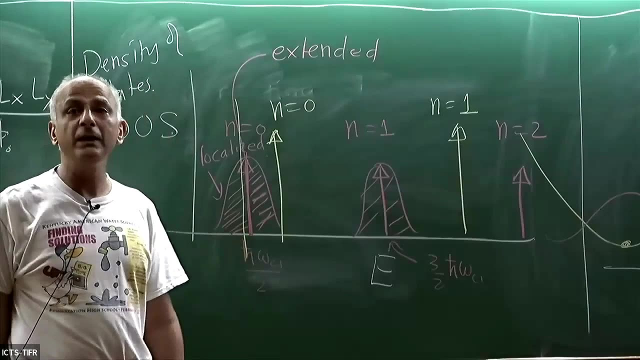 As I shift my chemical potential, I do something else than what I was saying earlier. Okay, I keep the magnetic field the same, but I change my filling by changing the chemical potential. What will happen is all the way up to here. I will find that the system is completely. 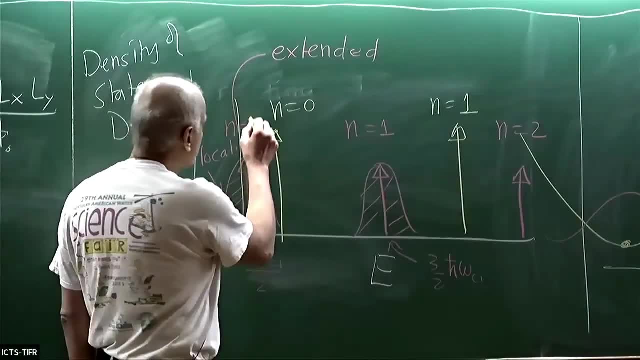 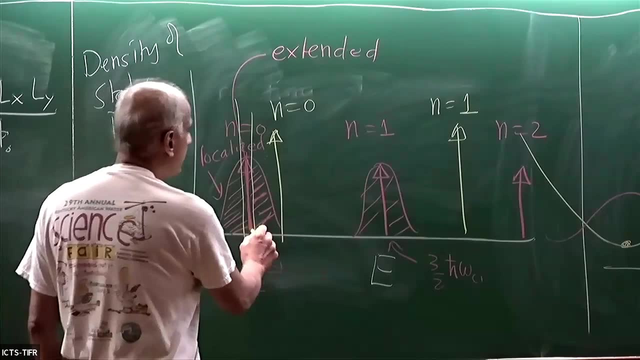 localized, There will be a quantum Hall effect. As soon as I cross this extended state, there will be a quantum Hall effect, And then it will continue all the way until I cross the next one, And then there will be a different plateau. 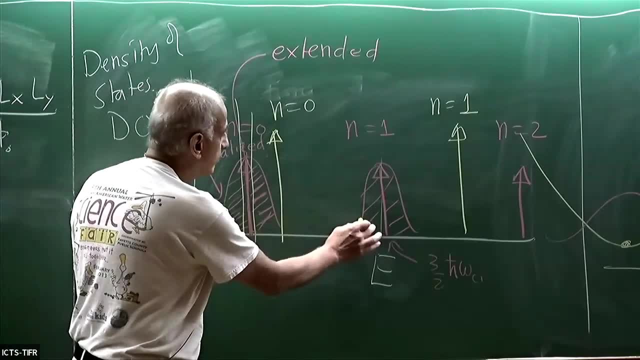 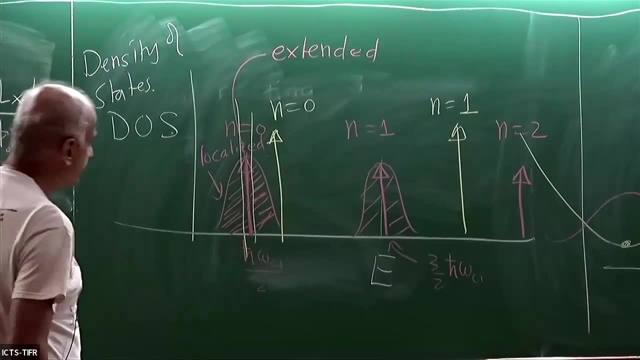 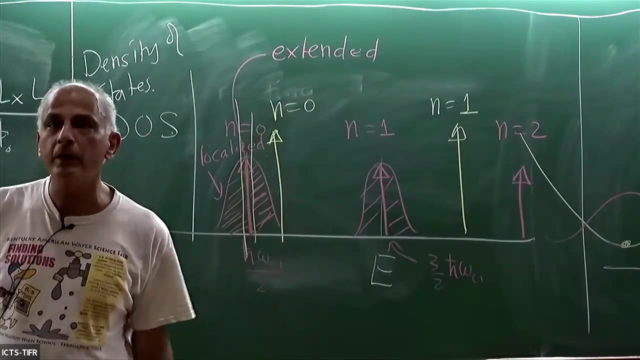 So the plateaus are the regions where the chemical potential is between extended states And the plateau transition is when it crosses the extended states. And the reason the Rxx- give me one more minute- The reason the Rxx is zero is because Rxx means there's dissipation. 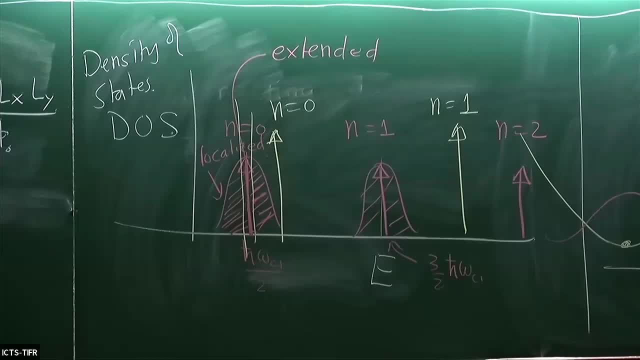 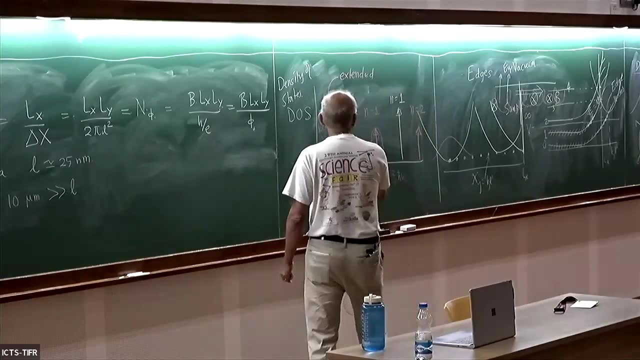 That means there must be some scattering at very low energies. Okay, So that means there must be some extended states at very low energies for the electrons to go into, But when the chemical potential is sitting somewhere here, all the states that it sees are localized. 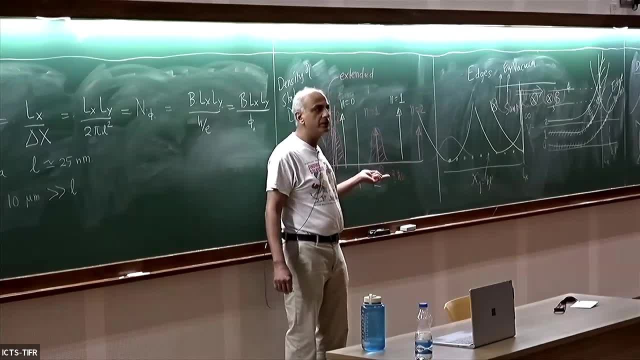 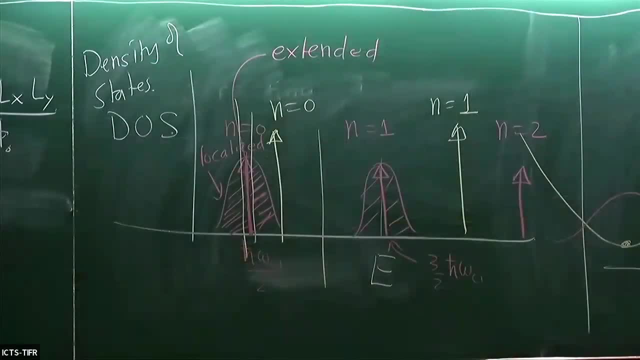 So it can't scatter into any extended state, So there's no possibility of dissipation. That is the problem. That is why Rxx is zero on the plateaus of Rxy, of the Hall resistance. This is why, in order to have quantization at all, if you okay, let me take a counterfactual. 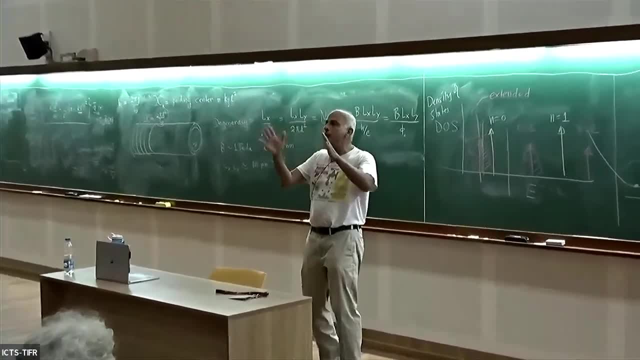 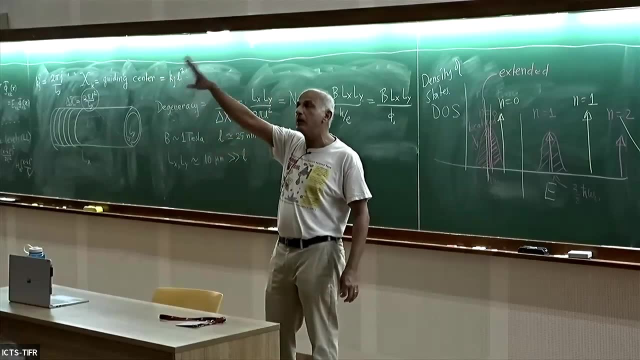 Supposing there was no disorder at all, there would be no quantization of the Hall resistance. In fact, you would go back to that straight line picture. You can show this by relativistic invariance. Take that as an example. Okay, 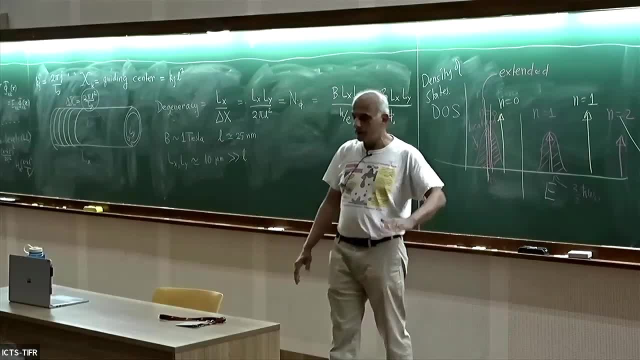 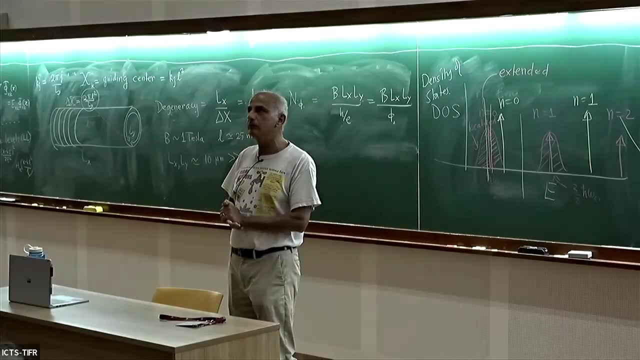 This is a homework, Okay, You can always go to a frame. So let's say your charges are moving. You can go to a frame where that velocity is zero and you can convince yourself that in fact the Hall resistance should exactly follow that straight line. 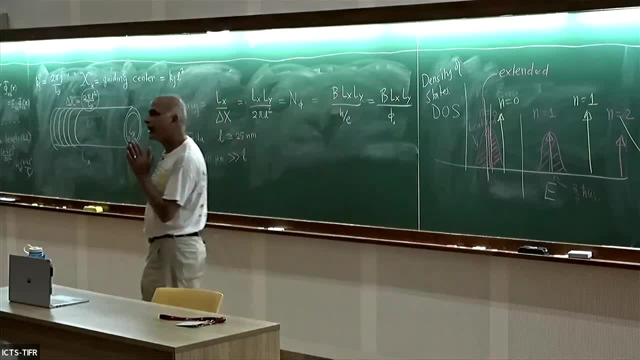 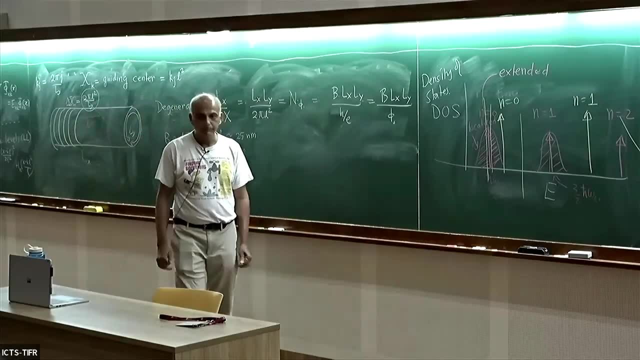 Okay, So it needs disorder in order to have the quantization of the Hall resistance. All right, I'm done. Now time for questions. More questions, Yeah, Okay, Thank you, Thank you, Thank you, Yeah Yeah, So in different situations they could be different. 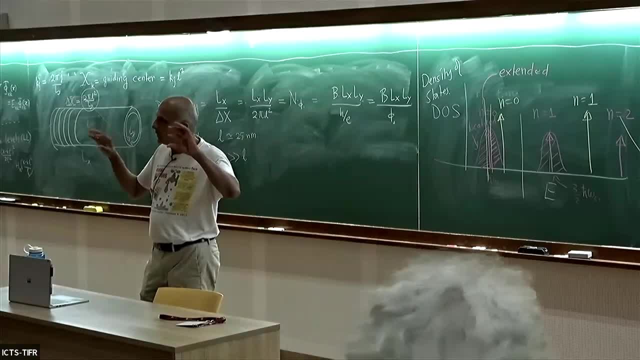 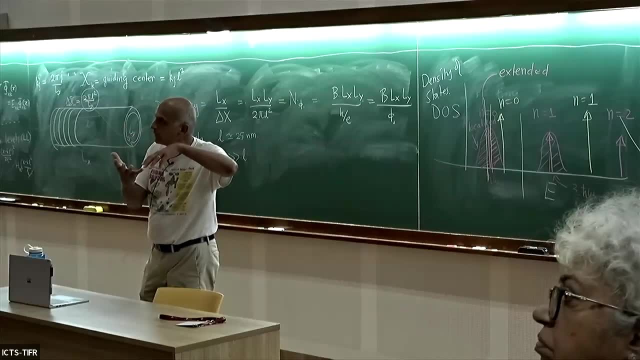 I mean there's some you know. so in these Gallium arsenide 2 decks they put dopants somewhere far away from the thing to reduce the disorder, but still they create some long-range pull-on potential And that's why this C sub disorder is large. 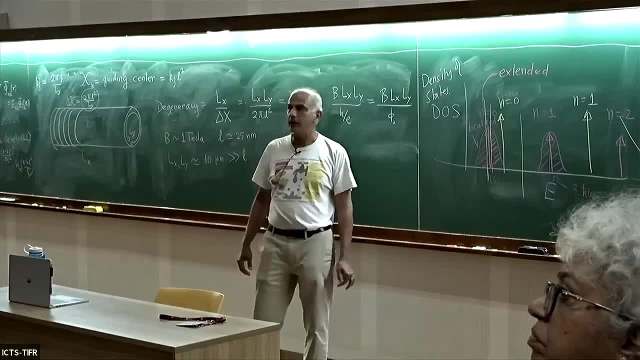 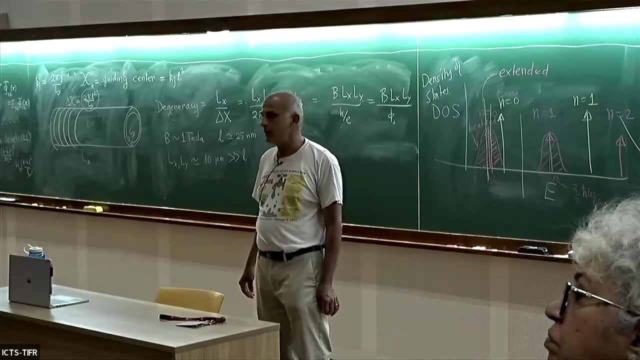 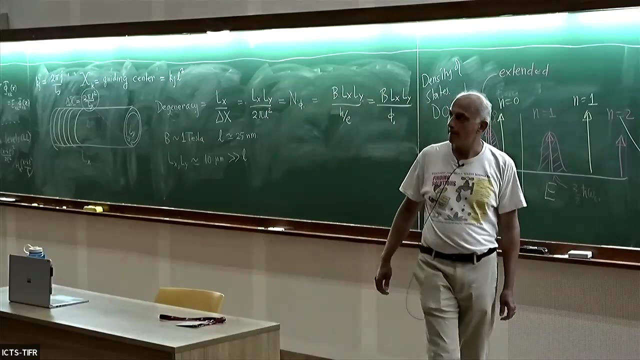 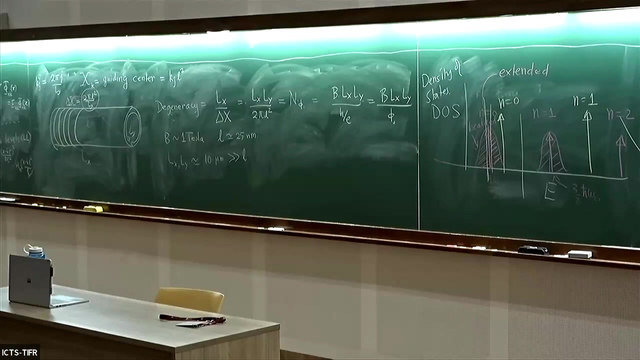 Yeah, the local electric peak Exactly, Oh, absolutely. But then I mean, how do you really see this kind of like you were saying, okay, it connects through the system, but No, the connection through the system is simply the interface between things that are localized. 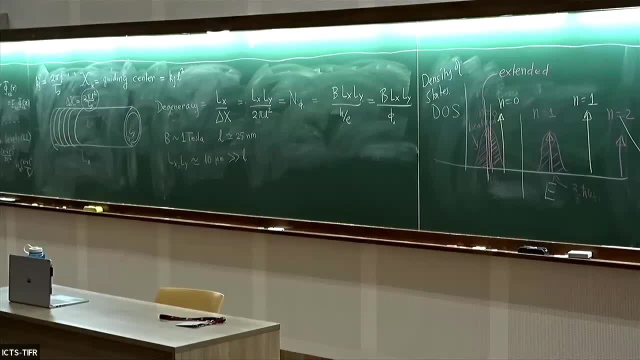 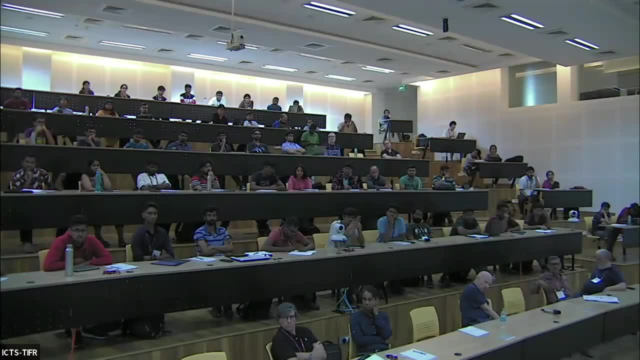 around minima. As I change the energy there'll be. I fill up the holes first, right, Right, The bottom, most holes. There may be some hills inside the holes as well. That's also possible. It doesn't matter. 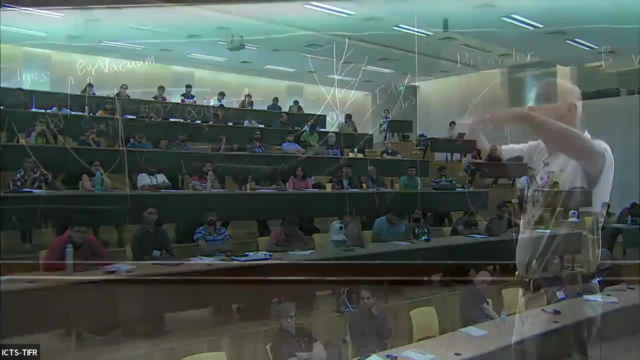 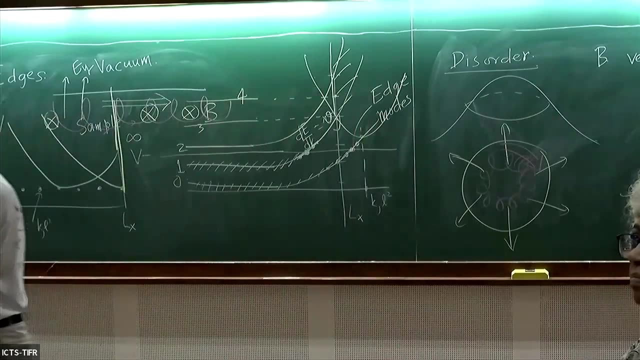 So at some point, if I fill enough, I know that I will not be able to walk across. Okay, There's some kind of percolation transition going on, Right, It's at that critical point of the percolation transition that you find the extended state. 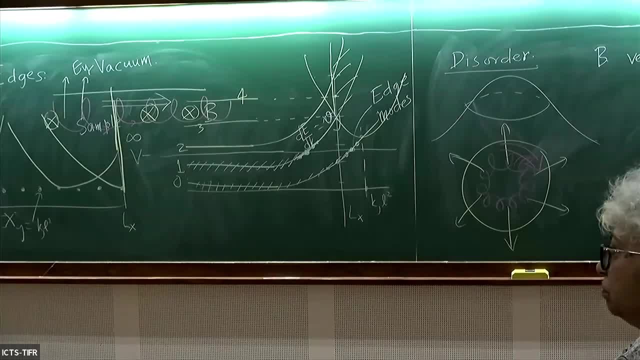 Right, It's a very complicated state. Okay, It's not a simple state. It depends on the realization of disorder: Some multi-fractal, some, you know some very complicated state. but it connects one edge to the other edge. 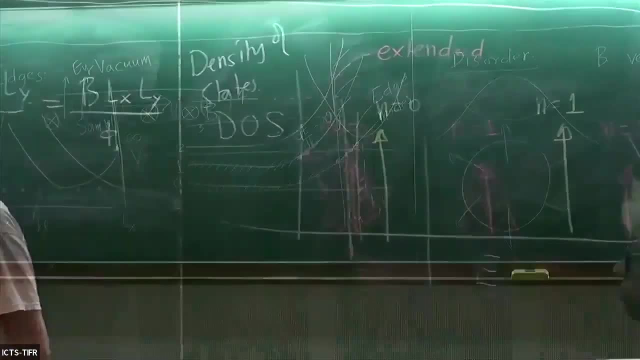 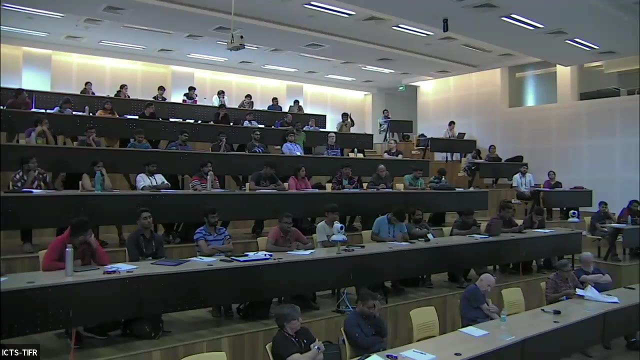 Okay. Another question is: so in presence of an edge, so you said that there are these velocities which you can have, Yes, So then I mean those are also states which are kind of extended right, Because these are going through the edge. 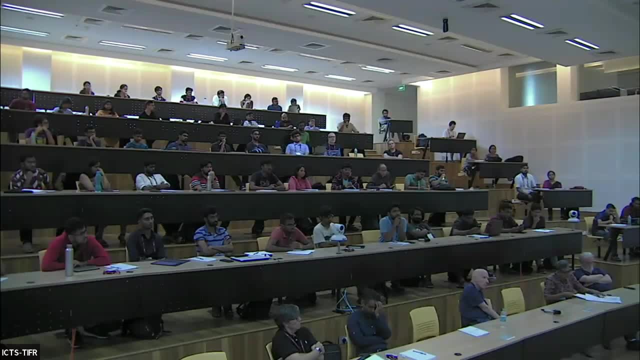 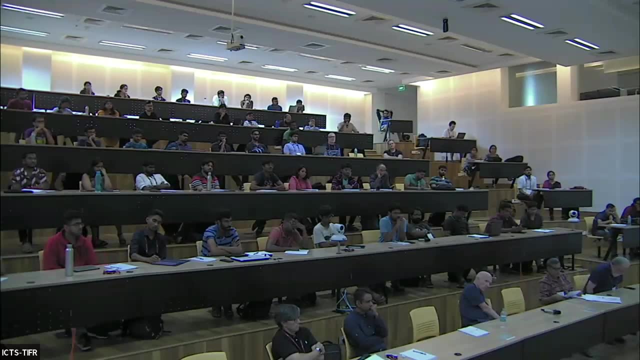 Edge states are definitely extended. That is why you can have transport through the edge states Right, Right, Absolutely, They're extended. Not only are they extended, they cannot be localized by disorder As long as the bulk state is intact. the edge states have to be intact. 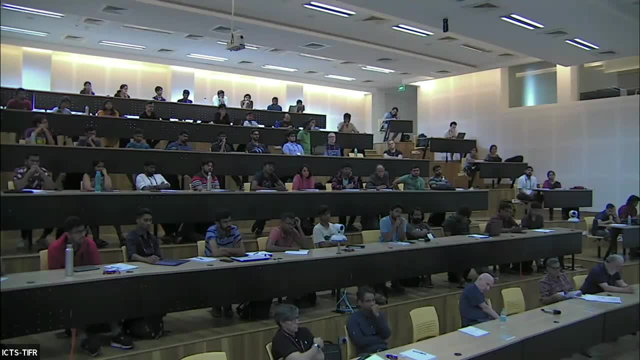 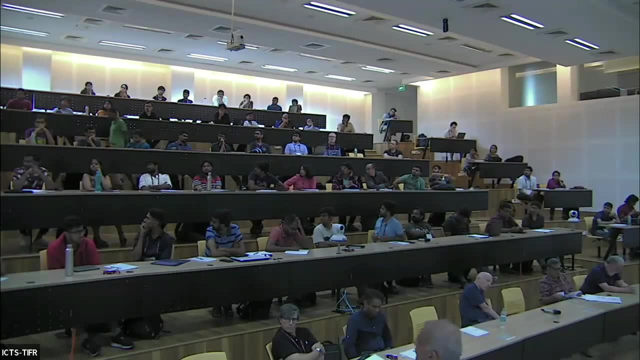 Okay, That's the topological property. Okay, Okay, Okay, Thanks, Yeah, Any few states which are, which are spread throughout the sample or which can go from one edge to the other edge, That is correct. That is correct. 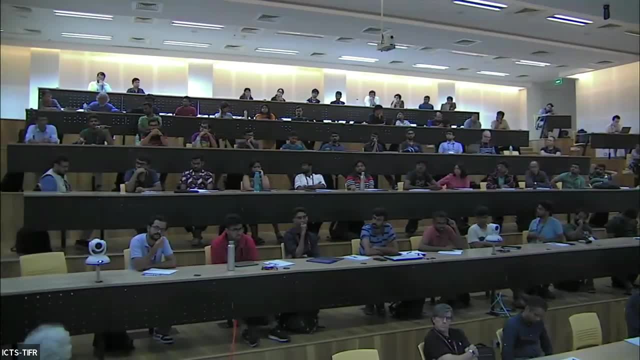 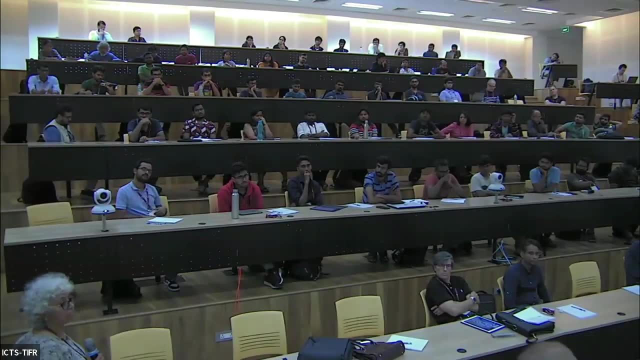 So does that number depend on the type of disorder you are adding in the sample? Typically there's only one state, Okay, There's only one state Now if you go to finite temperature, so around this state. so there's some, some complicated. 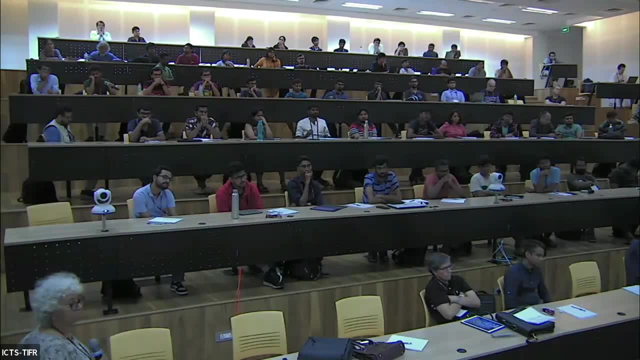 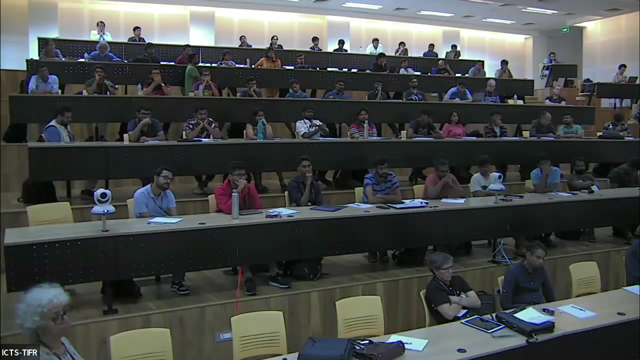 stuff goes on. Okay, So as you approach this energy here there's a certain size to all these localized states- Okay, That's called the localization link. That localization link diverges as you approach that energy. Okay, So, at a finite temperature, what happens is there's some little window here of order, kt. 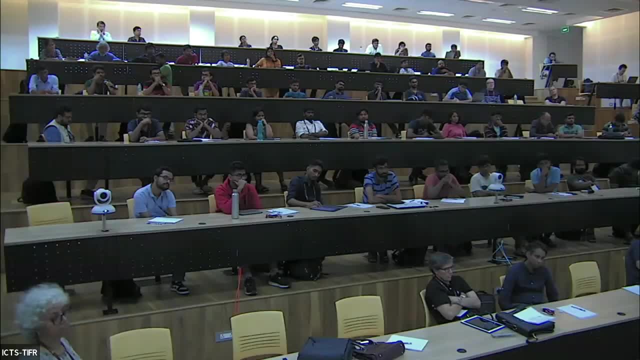 kbt k, Boltzmann times t, And those states can all scatter amongst each other Because of the thermal bath. Okay, So that is why the plateau transition is broadened with temperature. Thank you, Yeah, Yeah, Yeah, Yeah. 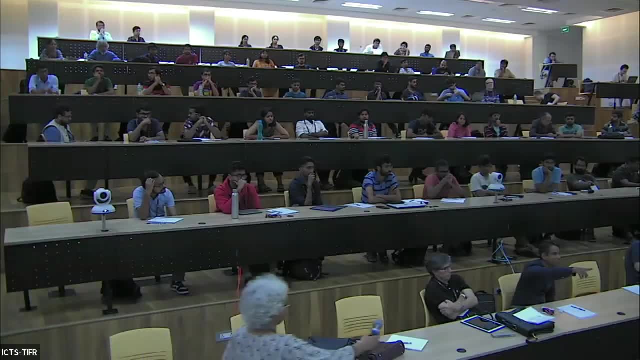 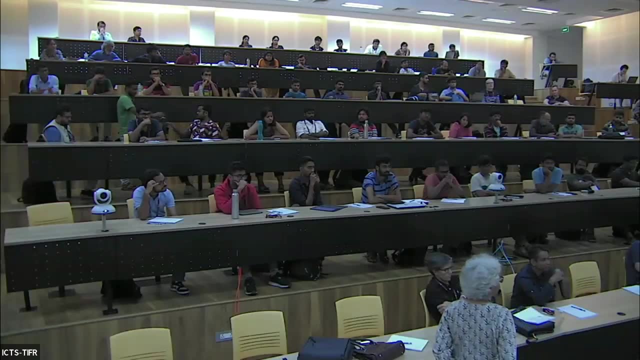 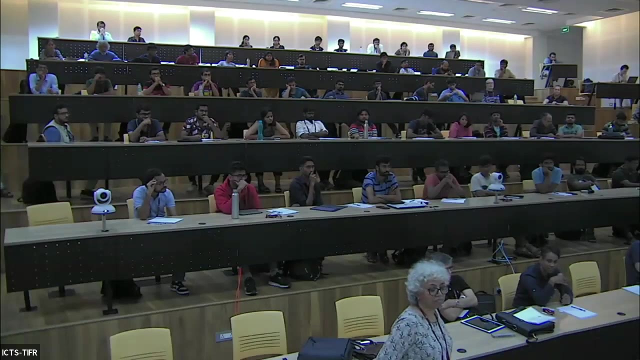 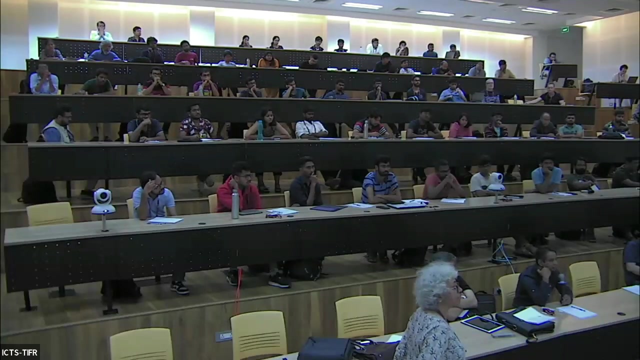 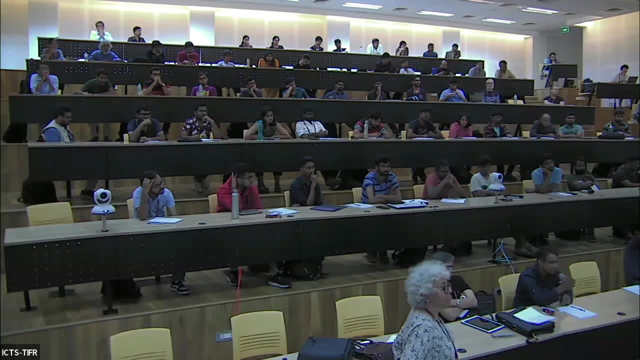 of the Landau band, the disorder-broadened Landau band. Yeah, yeah, in the field it connects to the edge. it's not identified with the edge. it certainly connects to the edge, but the point is that it connects from one end of the sample to another. but it's living. 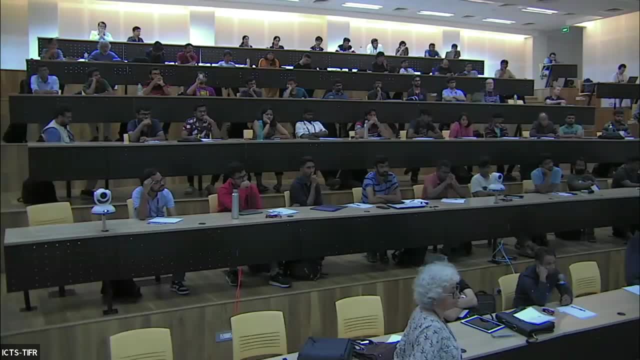 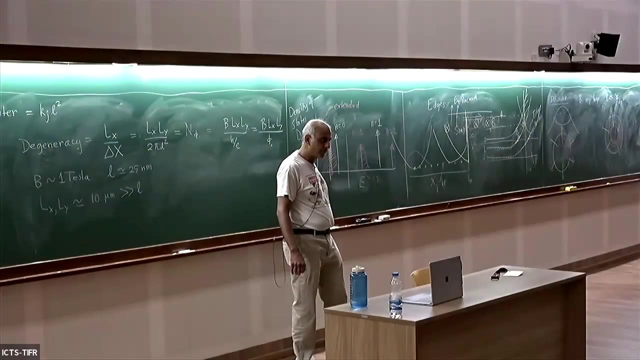 at this energy. Now let's say your chemical potential is here. okay, when the chemical potential is here, the only states that are conducting in the sample are the edge states. there's nothing else, all edge conduction. there's no bulk conduction going on, It's. 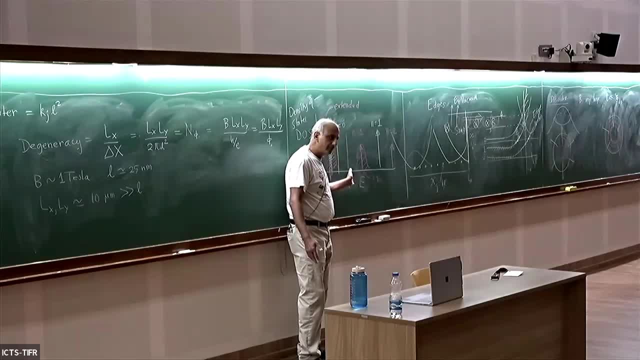 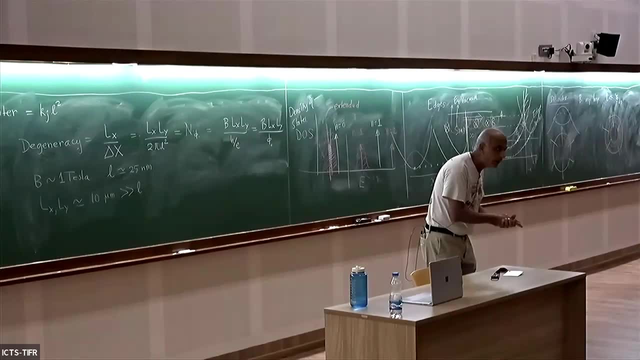 not sitting at the energy of the edge. Yeah, in a non-interacting picture there's a very strict division between the extended state, which sits in the middle of the Landau band, and the edge states sit in between Landau bands. so majority of the time you put arbitrary. 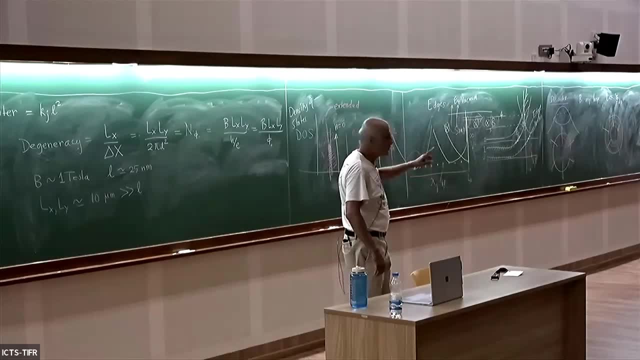 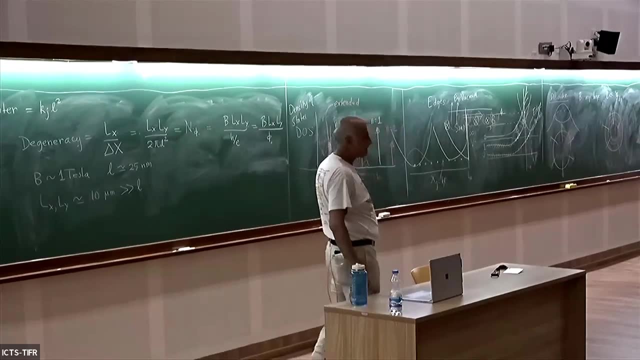 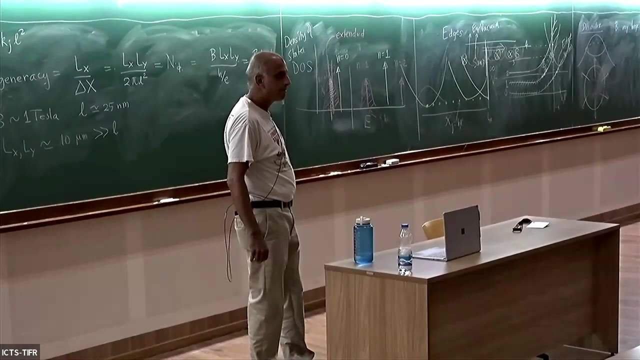 chemical potential. it will not hit the extended state. It will be edge conduction that happens. Yeah, you see it already in the quantum Hall plateau transition. Yeah, I do it, but then you always have to count this. Yeah, Yeah. 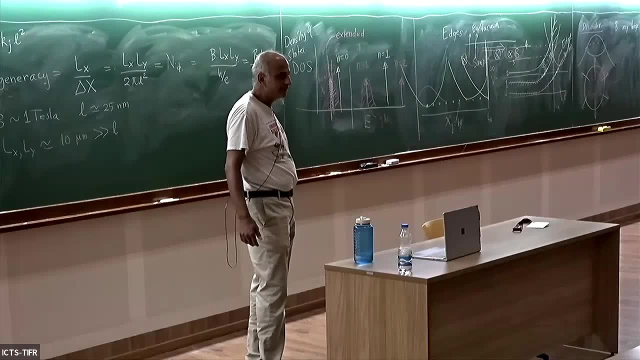 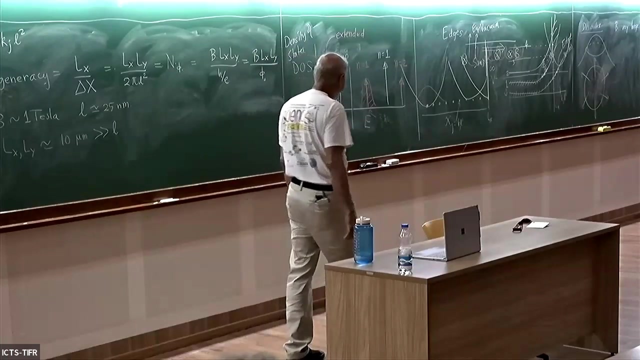 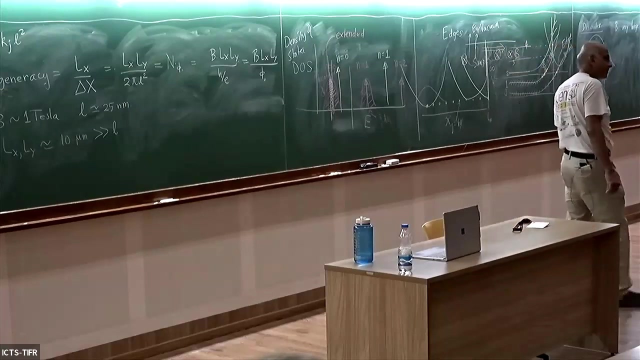 Yeah, Yeah. the threshold of the plateau transition is where the extended state lives. below that, all states are localized belonging to that landau band. right, the disorder-borne landau band. all states are localized below that chemical potential. above it they connect to the there is an edge state. yeah, yeah. so why does this rxx reach the level of uh rh at this at? 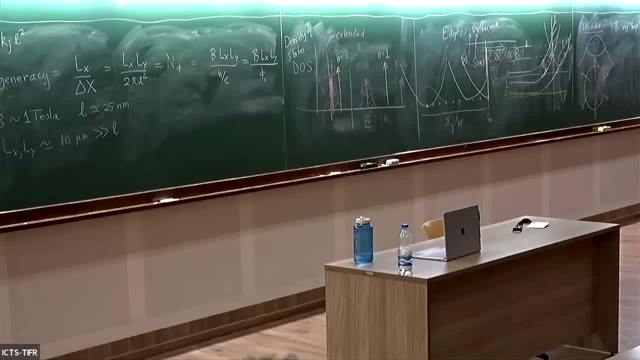 the transition rxx. yeah, so r? rxx reach this uh plateau, right, you, you draw, you were drawing this diagram right where these delta function. that that depends on the temperature and many things. okay, but look the the, the intrinsic scale of resistance in any quantum mechanical problem. 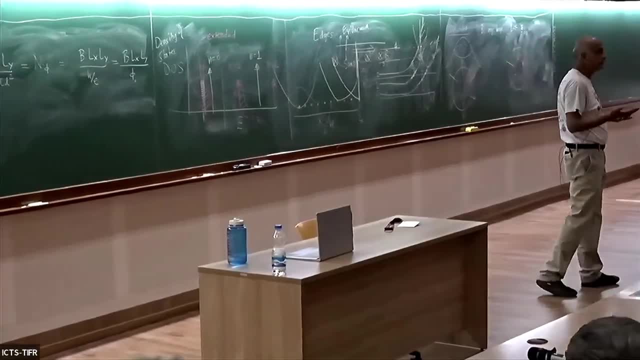 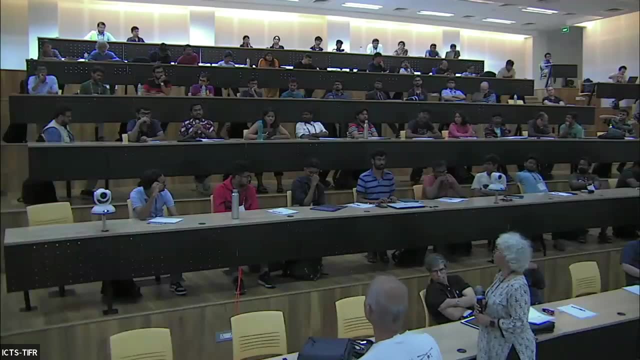 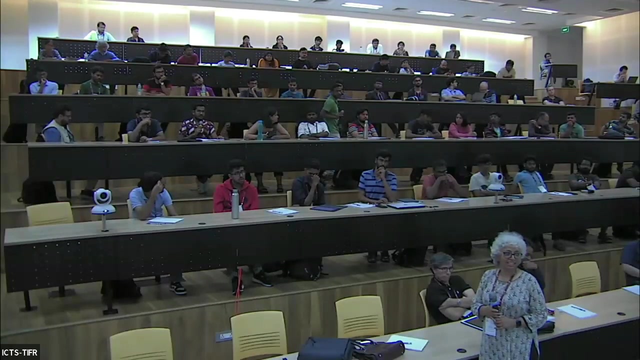 has to be h over e squared, right, there's no other scale, okay, but uh, but the dissipation, uh, rxs was happening because of the dissipation, and why it has to relate to h over e squared, then then my next question will, at a critical point, think about: so you're approaching some percolation transition, right? 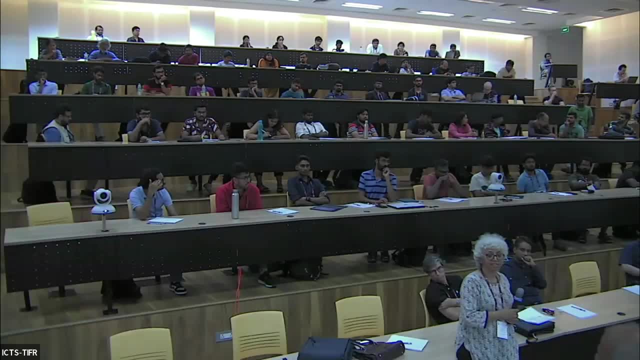 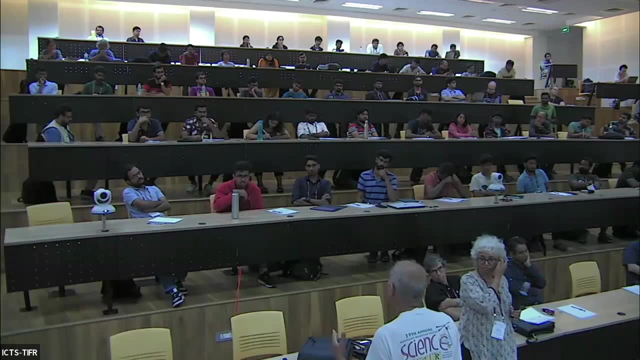 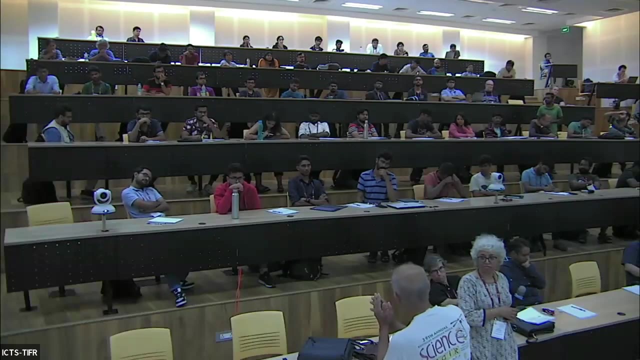 some critical point you think about. you know what kinds of things can rxx depend on. so, at a critical point, everything is scale invariant. right, there's no external scale. so now what you're going to do is you're going to relate rxx to some number of order unity times. 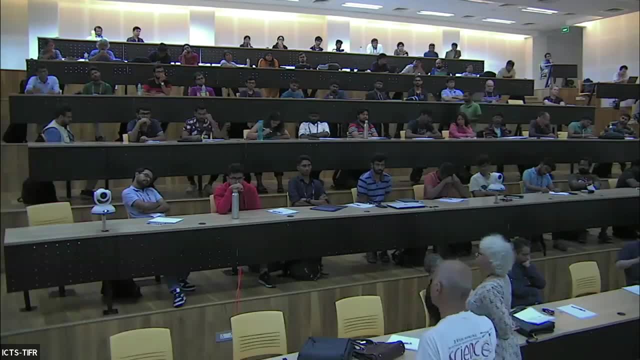 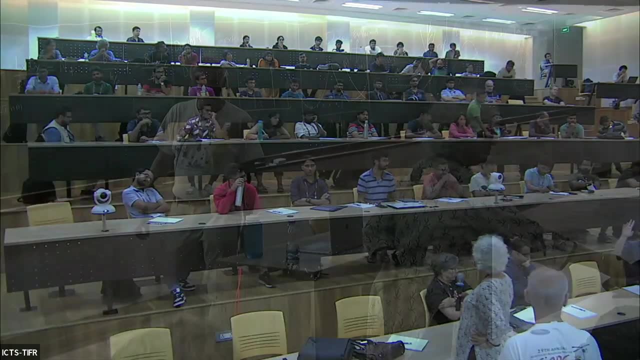 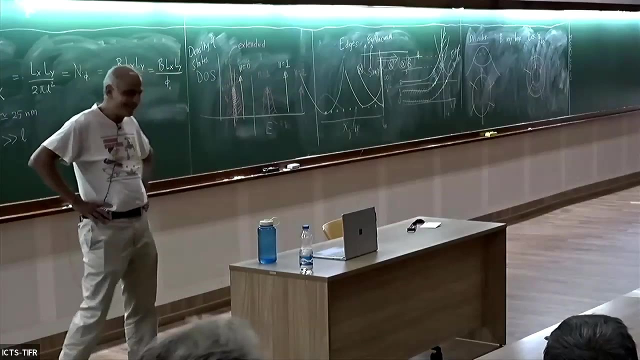 a fundamental unit of resistance. there is only one fundamental unit of resistance in quantum mechanics. that's h over e, squared, okay, i think. another comment: oh, my god, okay about this. uh, you talk about, uh, in the past, but how is it really important to have some simple? 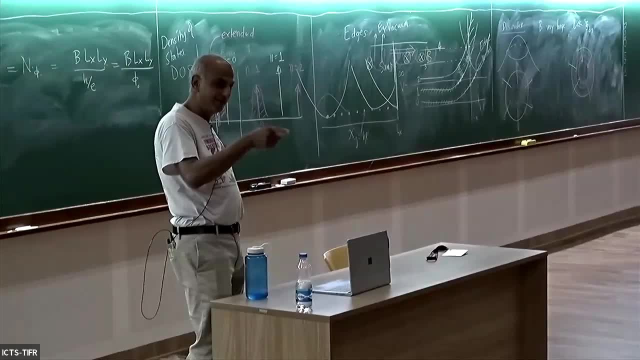 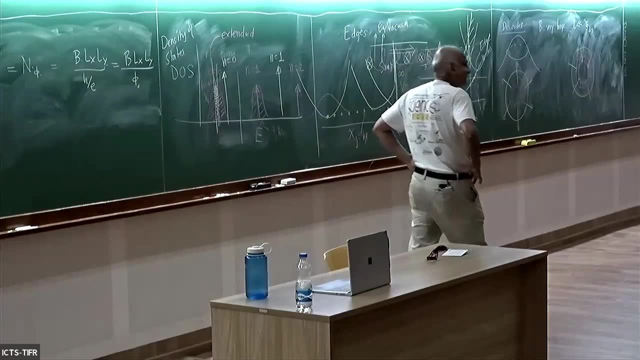 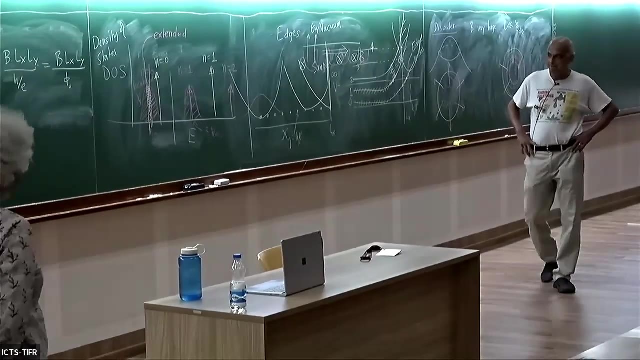 uh, expressions on it. the simple-minded picture- yes, just to avoid confusion- is already saying simple-minded. you're already casting, yeah, aspersions on it. uh, so, so, so we need to emphasize that, even if you are away from this. uh, uh, mid de-localized state. 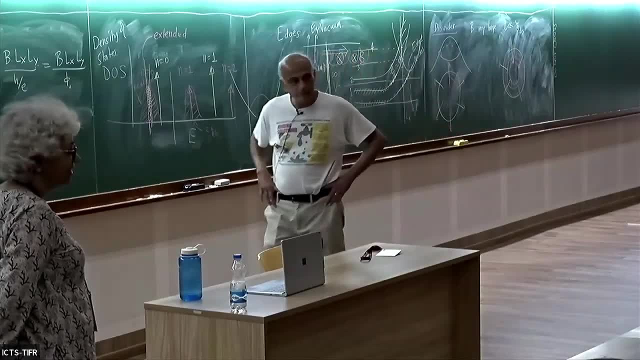 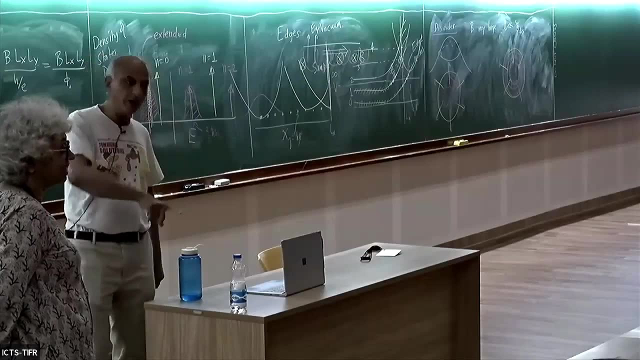 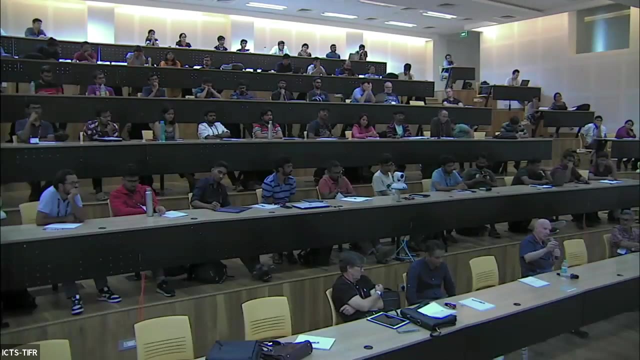 yeah, uh, conductance, in this simple-minded picture, conductance will be quantized Because of the edge: zero temperature at zero temperature. at zero temperature, Yes, will be a will be quantized and Actually even even a at a at a final temperature. Yeah, I mean, depending on the energy skills. 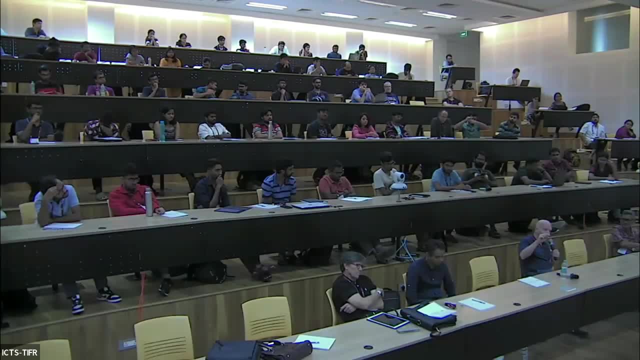 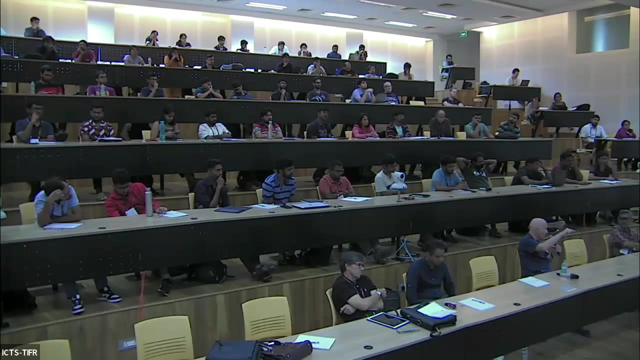 You will be quantized and actually what you would expect from this naive picture is if you a Scan the entire plateau. Yeah, then, at that particular point. Well, in addition to the air channels, the, the, this, the localized bulk state joins in, yeah, sort of a population a.